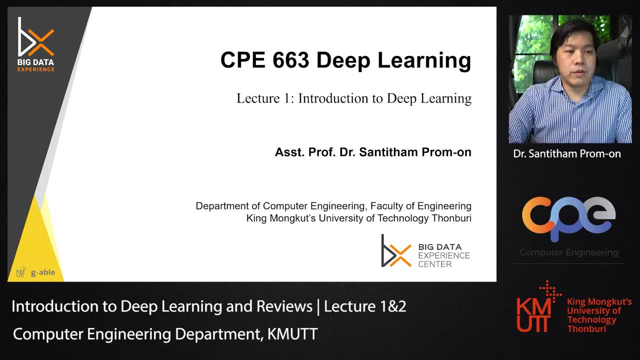 encounter throughout the course. Okay, there will be the reviews of concepts that I suppose that you have already known, which many of these are concepts related to linear algebra and how to write Python program related to linear algebra. Okay, so, in any case, let's. 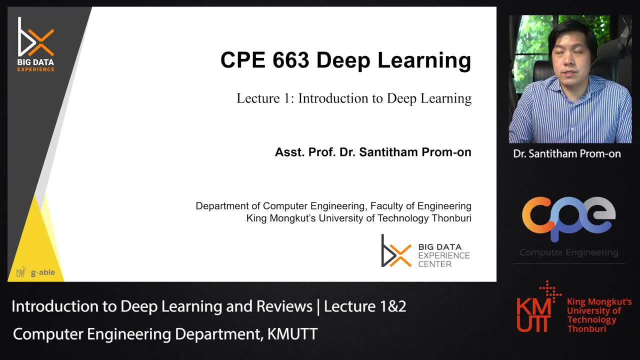 get started. Welcome to Deep Learning course for this year 2019.. We are still learning it online, like this, so I expect that some of you- that most of you that are here- are interested in the application of deep learning, as well as the insight of 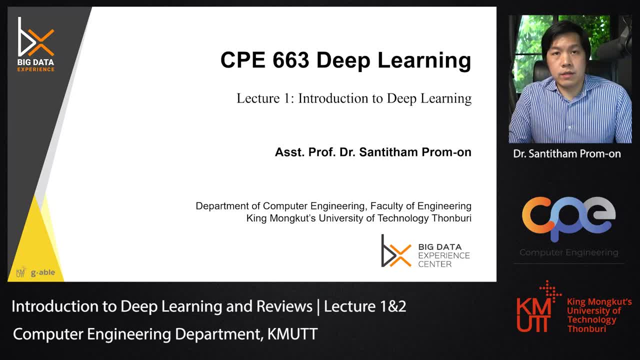 the deep learning models. What you encounter in this course will not be about how to write a program. It will not be about the special latest technique, But we will instead focus on the foundation of deep learning. We will look at how deep learning formulated and then we will further extend our knowledge toward some of a more 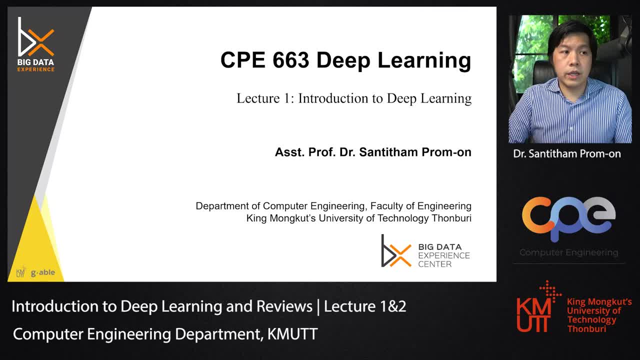 advanced architecture and see how are those. architecture has been described by the mathematical concepts. Understanding mathematical concepts are important if you want to be able to excel in the deep learning areas, So I suppose that you are in this course because of that. Otherwise, I guarantee that it will. 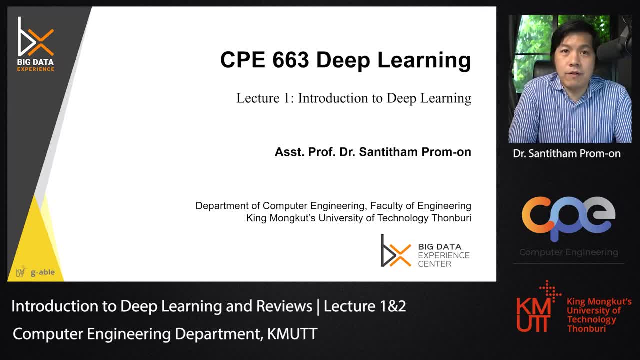 be a bit suffering because you will encounter lots of mathematical formula and the derivation of the mathematical formulas and extension to the application to do writing a program of it. So it will be like combination between both. We will also have assignments, which they are all coding, assignments that you have to write. 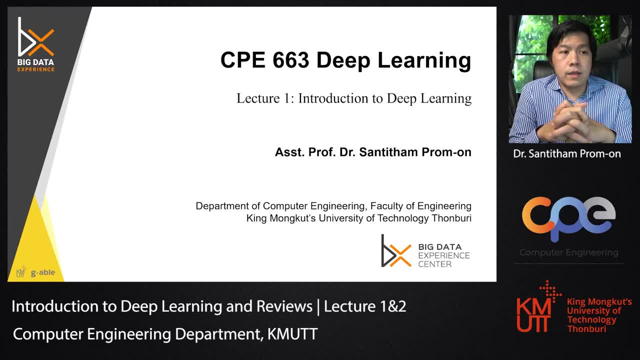 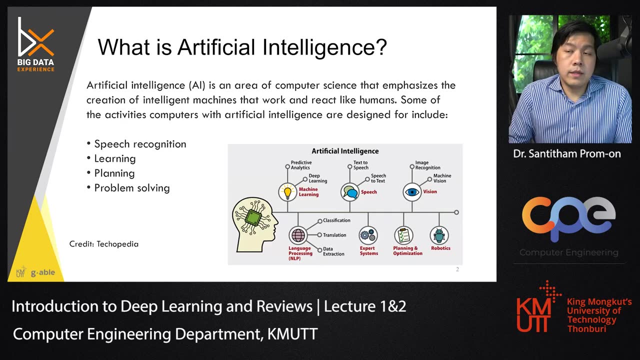 Some of them you have to write the program from scratch, write the learning application from scratch. Some of them you can use the library to do so. Okay, So let's start. You have in, I would say, in the modern era, now, today, that is where you usually use the. 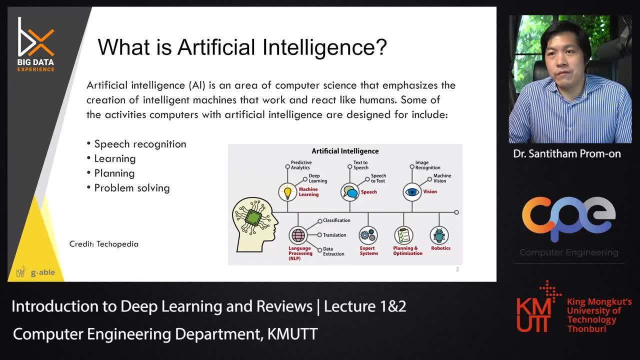 word right. So we have seen thatificial intelligence, AI has been part of us, has outside of us, been part of our life, and we all see that they have certain intelligence in them. how are they created like? what are they composed of? those would be the 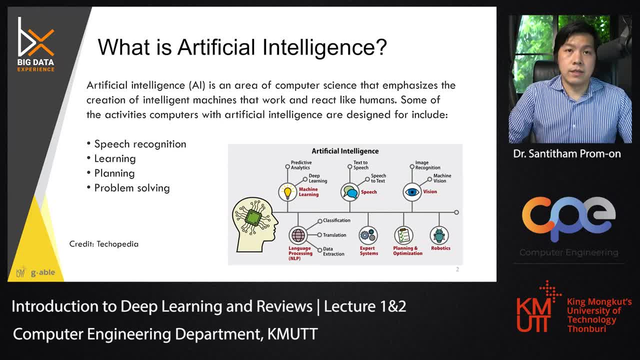 questions that we pursue in the more foundation perspective here. okay, AI is described as an area of study, as you may have known, that focus on mimicking human behavior, mimicking human intelligence. so we are creating a machine that should behave, that have certain cognitive intelligence like human. sometimes AI is also known as, in a larger field of cognitive computing, I 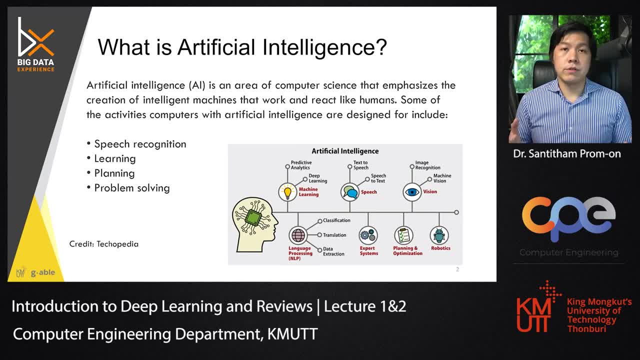 wish, may encapsulate not just in AI alone, but also other related topics like language learning, planning, optimization, problem-solving and other things. when we talk about AI, a certain task that we we know we expect them to, we expect them to perform, for example, in an AI. you might expect an AI to be able to match the pattern with. 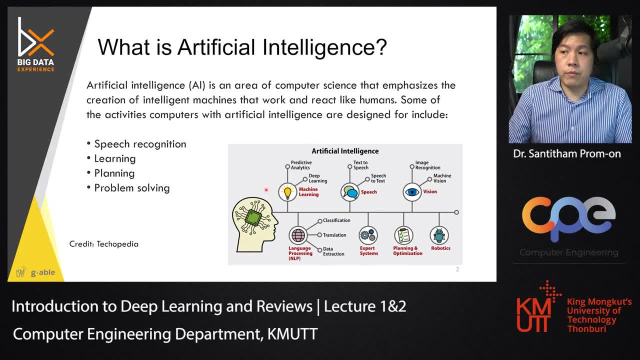 certain in certain output, match certain input with the output, and then we want them to learn the patterns from the previous, from the historical data. we know those, as we call the techniques like that, as the machine learning technique inside machine learning technique. they are like numbers of technique, number of methods that you can learn, like decision tree, land of forest. 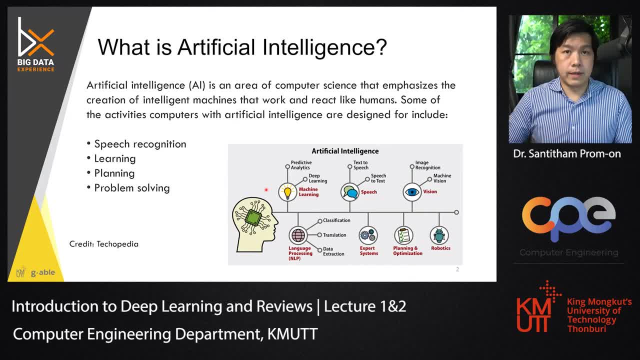 rain and boosting or even to to work deep learning and families of the deep learning technique. okay, in in the field of AI, there are application wise in AI as well, like when we talk about speech application, you, when we, when we create a machine that can generate human speech or can perceive human speech. 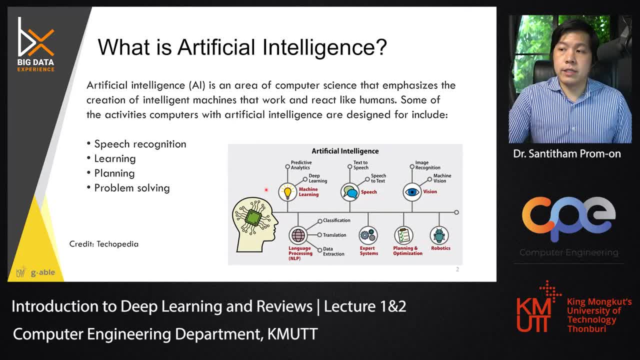 Those are the speech processing tasks, Or the machine that can evolve, evolve its speech pattern, that can mimic human, And on the other hand, you have an application that can interpret, image, perform tasks like human in something like human vision. These are the fields of computer vision, machine vision. 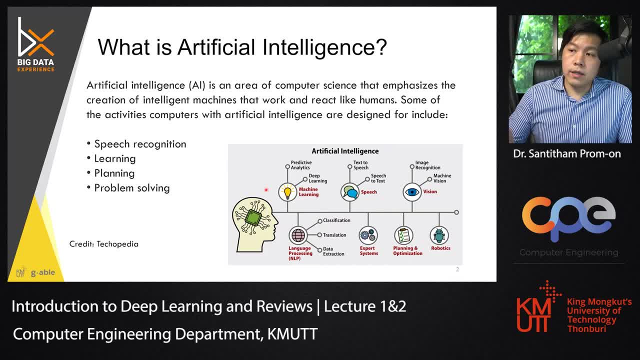 There are classes about this as well. If you are interested in those, you can take those classes and you will encounter models and techniques that will be different from just deep learning alone. Deep learning doesn't solve all the things, Although it is quite, I would say. 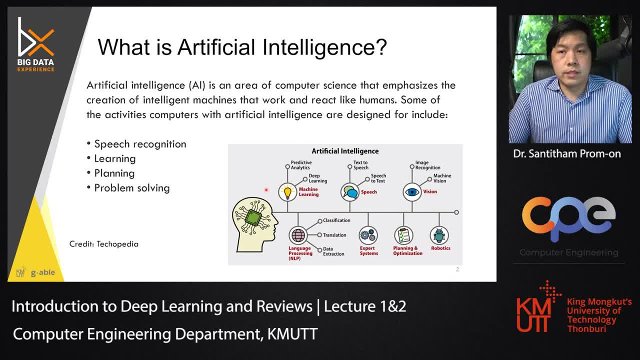 the novel approach in research. in a lot of application, deep learning doesn't reveal the inside of the process, But it doesn't reveal which features are important. It doesn't reveal which mechanisms and how it work. So if you want to create a model, 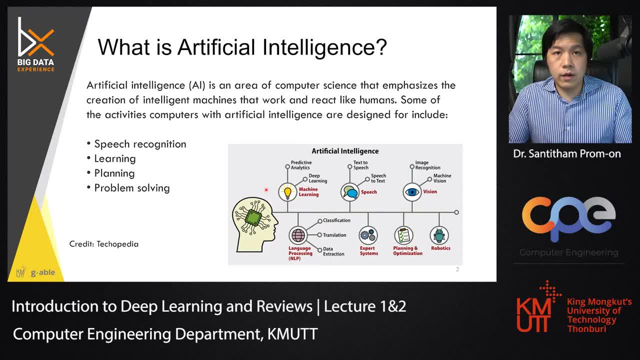 if you want to create a model, to perform simulation, perform something that close to human deep learning might not be the things for you. You might want to look at the model-based learning. You might want to look at other things. Okay, natural language processing. 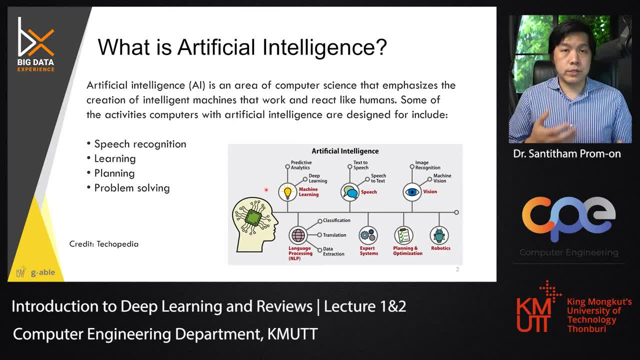 This focuses on how can we process natural language, how can we generate natural language? Right now, the field of natural language processing and the text processing is occupied by the deep learning technique, Although if we go back, like 20 years ago, most of the technique are heuristic technique. 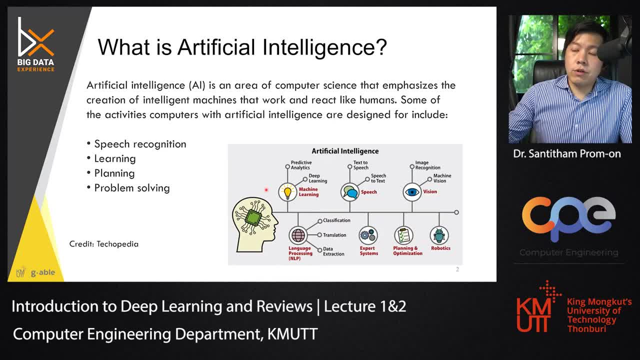 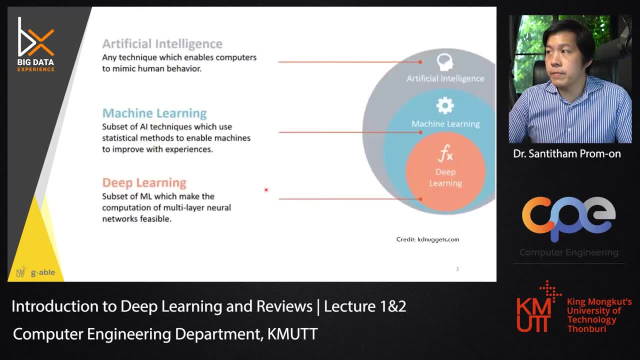 and some of the machine learning technique as well. And then there are also other field in artificial intelligence, like export system optimization and robotics. okay, Therefore, artificial intelligence is, like, I think, a tool for artificial intelligence. Therefore, artificial intelligence is, like, I think, a tool for artificial intelligence. 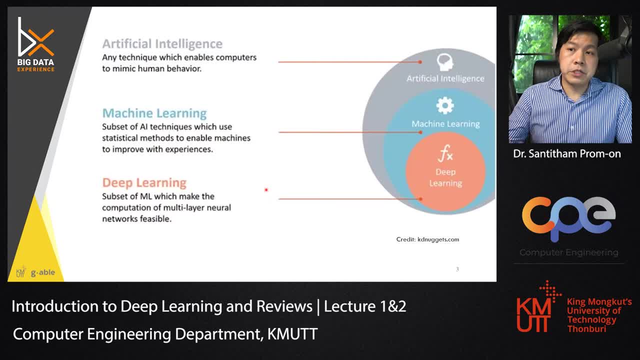 Therefore, artificial intelligence is, like, I think, a tool for artificial intelligence, And when we talk about machine learning, it is actually the subset of the AI, And deep learning is even a smaller subset of the technique, But even though it is quite a focus area. 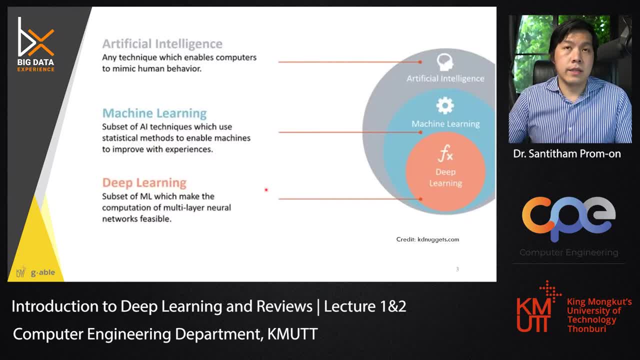 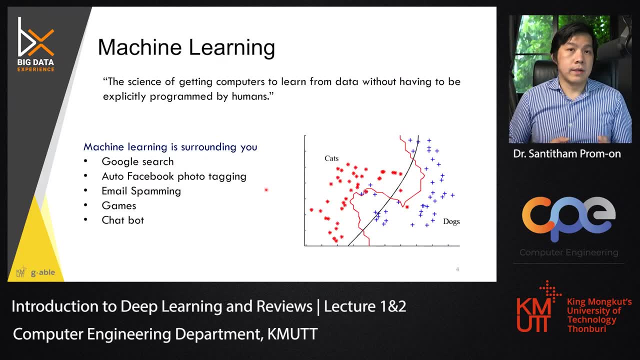 it can be applied in many fields because it's power in learning, the association between patterns. okay, So how do we define the deep learning? Let us first define machine learning. What is machine learning? Machine learning is like a technique. Machine learning is like a technique. 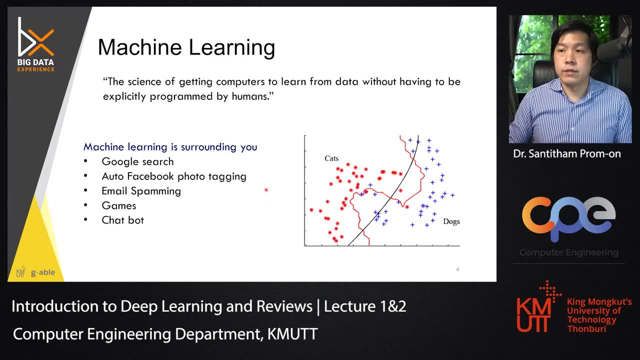 That you allow the machine to learn the pattern right. You allow the machine to learn how to associate between features and then do certain tasks, like distinguish between class, like what you see here, or perform estimation, like integration, divide the data into groups. 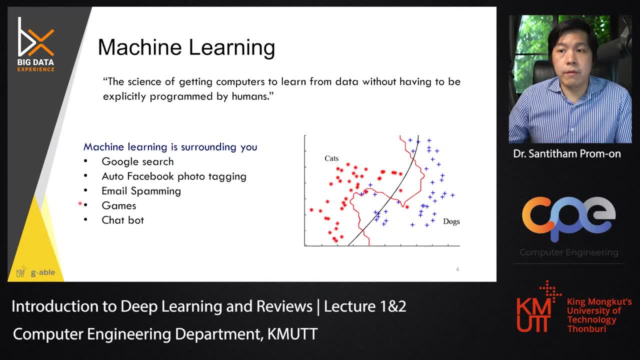 or do these things like tagging whether the email is spam or not. identify which search would you would like to see. identify which search would you would like to see or perform the chatting, perform conversational control like in the chatbot. 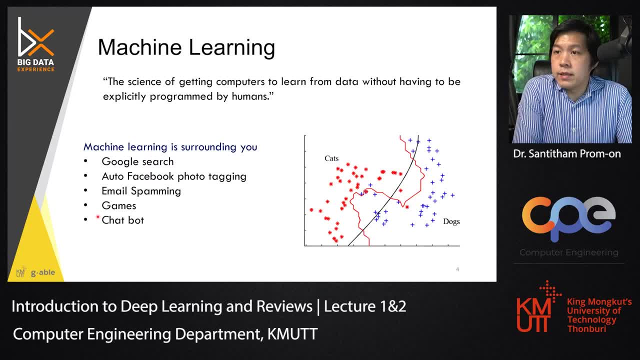 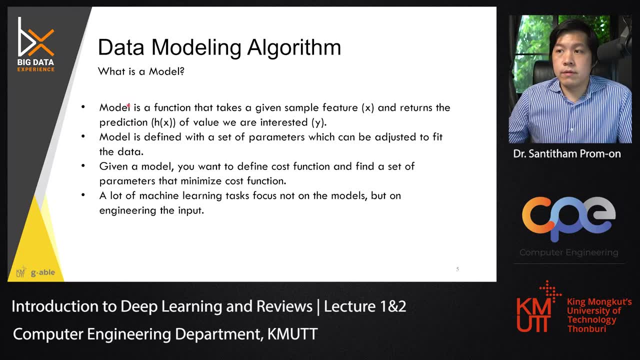 Now if we were to define deep learning mathematically, deep learning is a way that we want to find the function, or sometimes we call it a model, like a model that when we give the feature, the set of feature X, to the model, 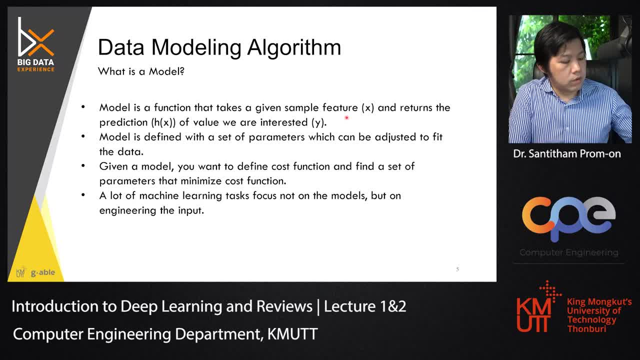 this feature X would pass through this feature. X would pass through the function F, X, and we got Y here Usually in the machine learning task and we got Y here. Usually in the machine learning task we would already have the X and Y collected from. 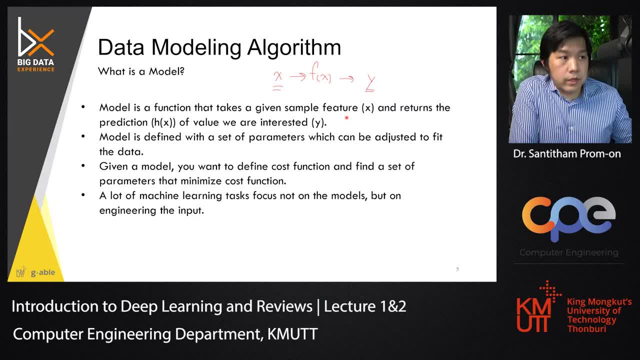 in forms of data, and then what we are trying to do is to estimate this F X by different methods, like when we use decision tree, by different methods, like when we use decision tree. by different methods, like when we use decision tree. 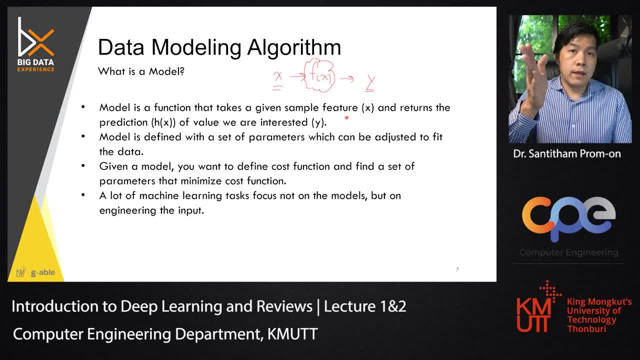 we try to infer that this F X should be partitioning based. we try to infer that this F X should be partitioning based, like the model that based on partitioning, the discrete partitioning of data. When we use regression, we are trying to explain the association. 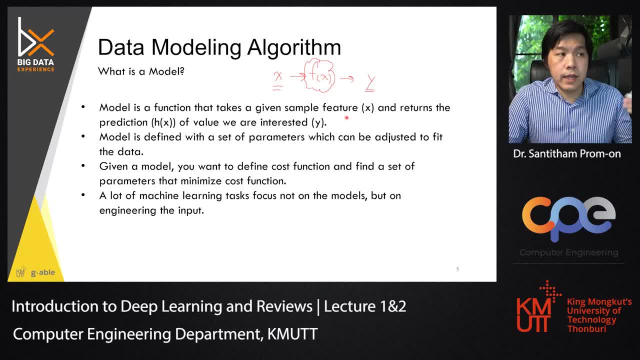 between X and Y as linear combination. That means X has to somehow linearly correlated with Y. And when we use other technique like random forest and gradient boosting- like random forest and gradient boosting, we are trying to infer that they are linear combinations. 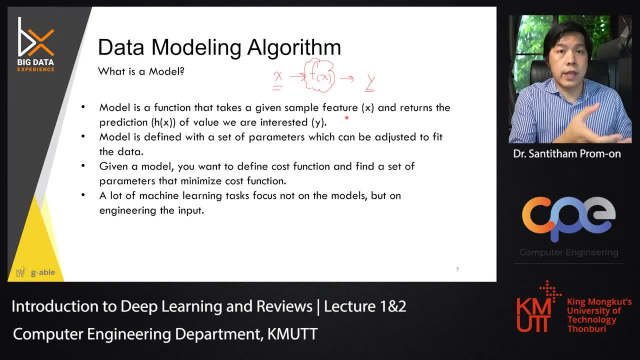 that there are certain quite complicated subset and association that informs of partitioning as well between x and y, And also different method would based on different assumptions. For example, suppose your data x is a sequential data and y is a class. f should be something. 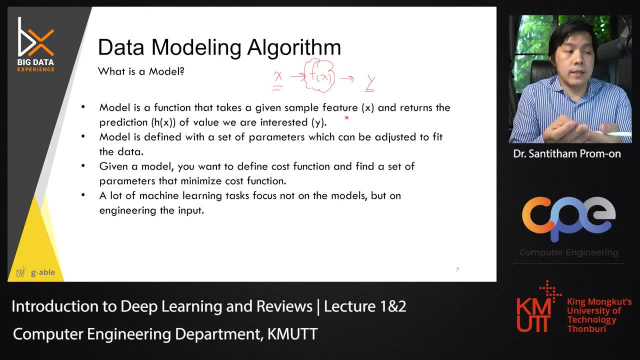 that is suitable for this type of data to explain the process. If you use decision tree to map between them, can you do that? Yes, but f might not represent the actual process. But if you were to use something like hidden Markov model, conditional random field or 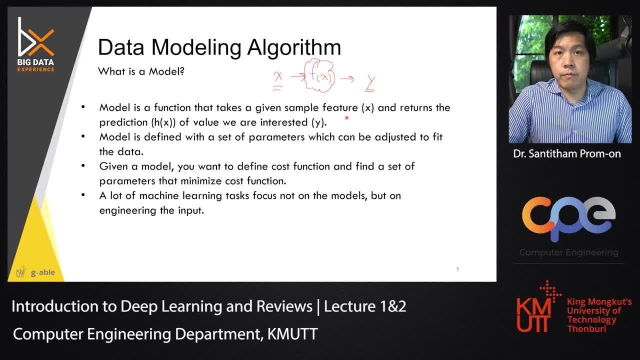 the RNN, then association between x and y will be more proper. The task that is to identify the model that are suitable for this type of things is belonging to the well modeler. I usually call myself a modeler, although I'm not associated with any type of modelings. 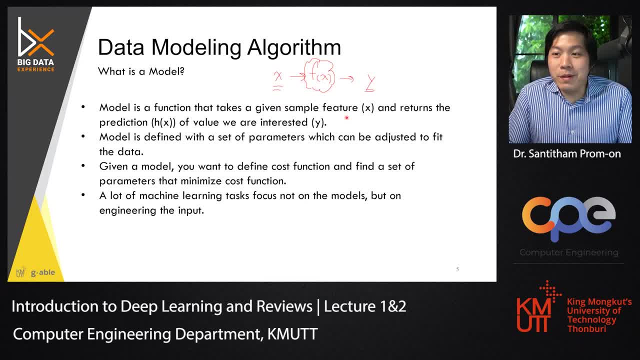 in the modeling sense. you know that right. But well, now, today, we, we have different names, Like scientists, AI, engineer, whatever. I'm still calling myself a modeler. I like to. I like to create a model, although my model is the mathematical models, that kind of finding. 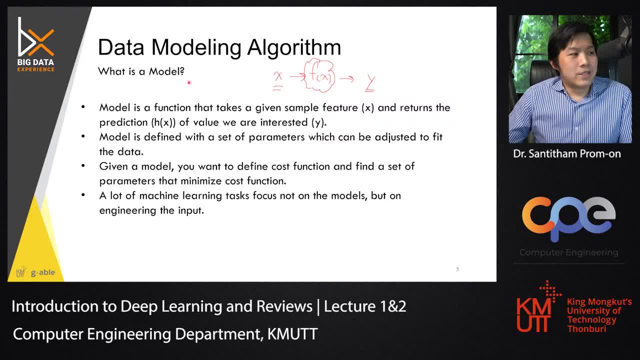 associations between things that you see. Okay, so when we talk about model, a model is a, set, is a like a defined, defined formula, a defined structure that you that have a certain set of parameters, Those set of parameters to explain the association between data to have in the model. you even 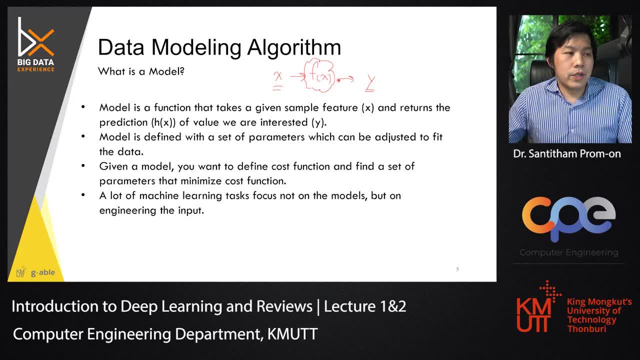 you want. the menu wanted to be learned that you need to have a certain something that is called cost function or objective function. All the other function. Well, the same thing on the last function. Okay, then you can use the function, Then you can use, then you can use these as a criteria to optimize the parameters. Okay, 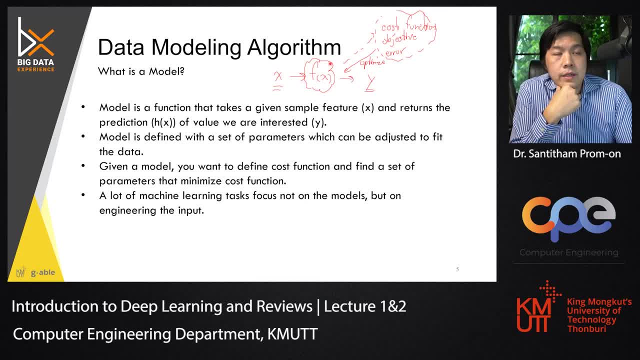 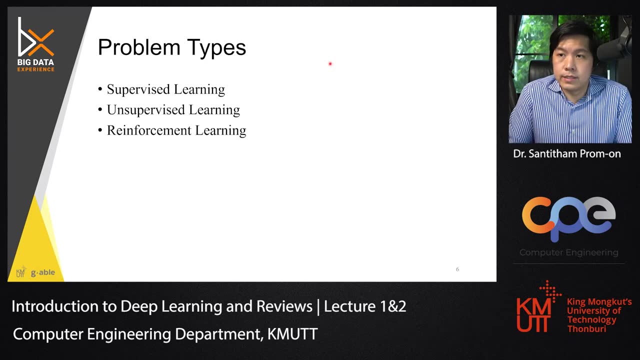 so it's like the basic concept here Now. we will talk about it in more detail in the lecture of machine learning, which we will learn about the machine learning concept. mathematically, The form of learning can be different depending on the task, depending on the situation that 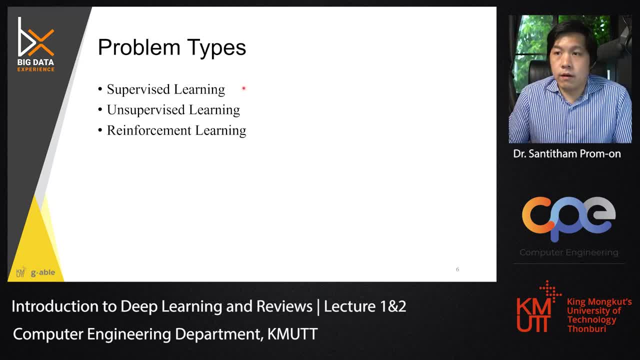 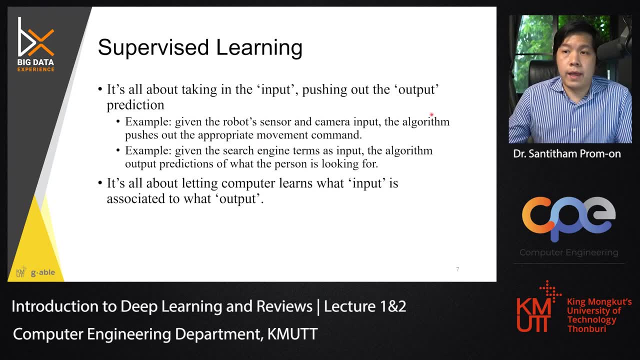 you have supervised learning or unsupervised learning or reinforcement learning. In the supervised learning we have input and output pair. what we are trying to associating. what we are trying to do is to associate input and output together. Sometimes output might be the thing. 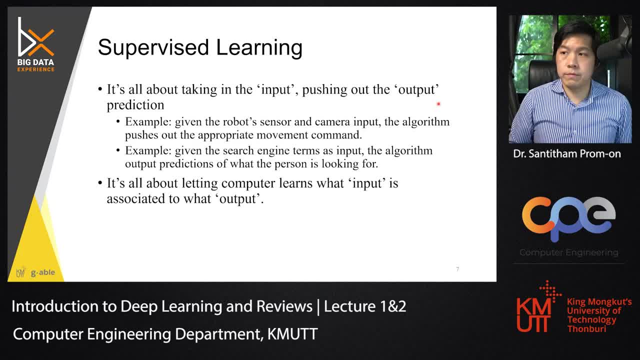 in the future and that we are creating a predictive model. But sometimes output can be the thing that is now, And what we are trying to do is to create a system that can interpret the data, like seeing the image and deciding what to do. Okay, So something like this: given the robot sensor camera input. 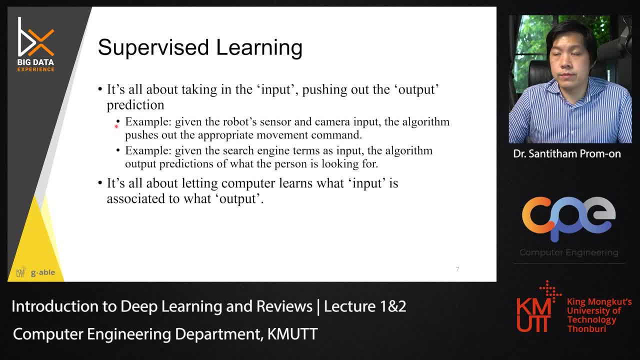 you want the algorithm to kind of find the movement that it should do, So that's not future, that's something that it has to do. or creating a search engine that when you query the search terms, then it identify, maybe, products that are close to what you are searching for. So here you need to teach the system. 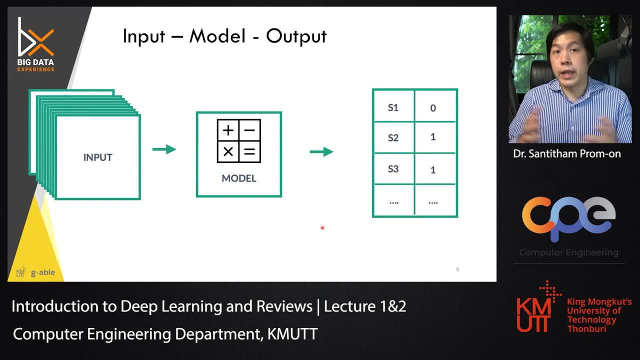 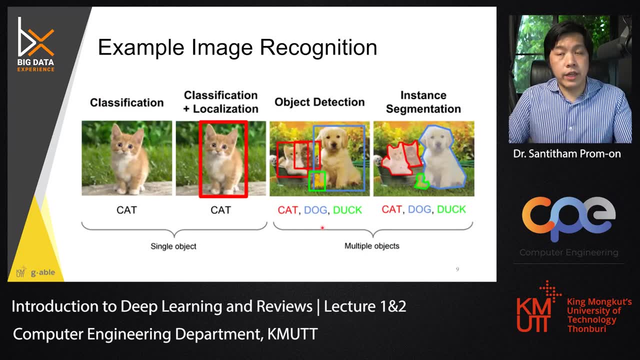 input and output. okay, have input and have output and then trying to associating them together. These are supervised learning. The tasks are supervised learning like classification tasks, localization tasks, object detection and segmentation, Although some of these are like combination between, I would say, the combination of the two. So, for example, the 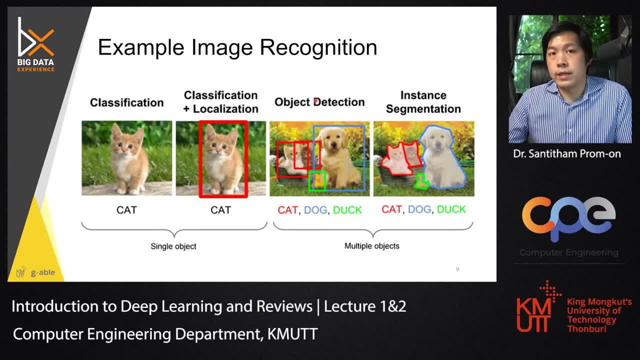 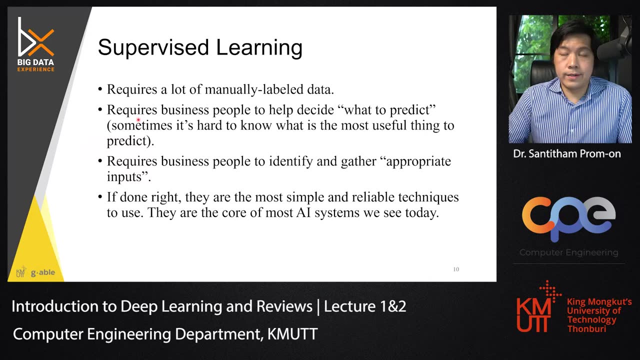 combination between supervised and unsupervised that trying to like, minimize the region. But let's put it this way: like classification is supervised learning in this case, Okay, Okay. so for the supervised learning, what do you need to perform the task? you need to have a lot. 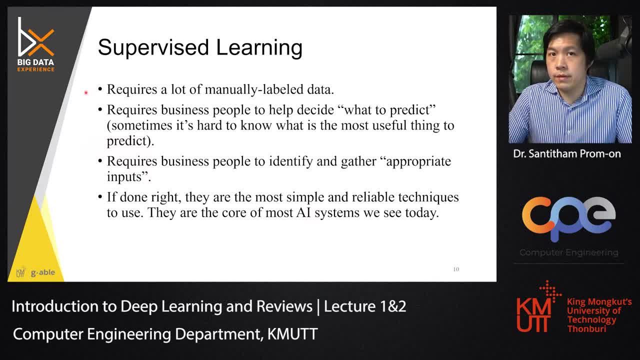 of label, a manually label data. This is important. you need to have the manually label data, All the data that are labeled, not based on certain criteria that you want to use them as input, but based on all the things. It might be based on criteria, but those should. 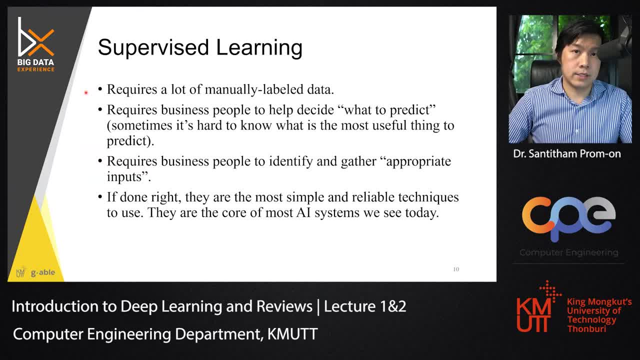 be the criteria that you are not including in your X, Otherwise you will generate- and I was sometimes you call this overfitting, but I usually like to call it in more philosophical terms, Circular reasoning. you are putting the output to reason as the input to produce the output. 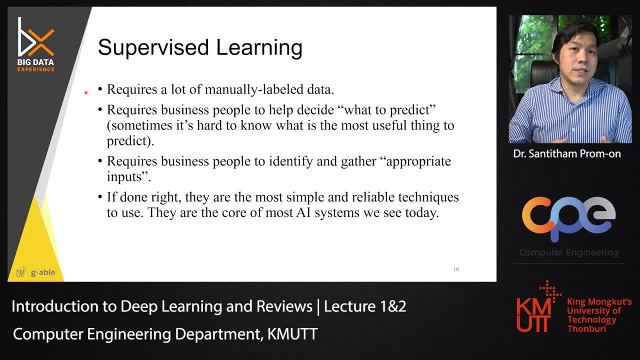 And that is circular reasoning, And circular reasoning is not acceptable. In reasoning, you should not use your, your end goal, as your assumptions, right, So so? so, that's the philosophy related to to model. Okay, so that's the philosophy related to to model. 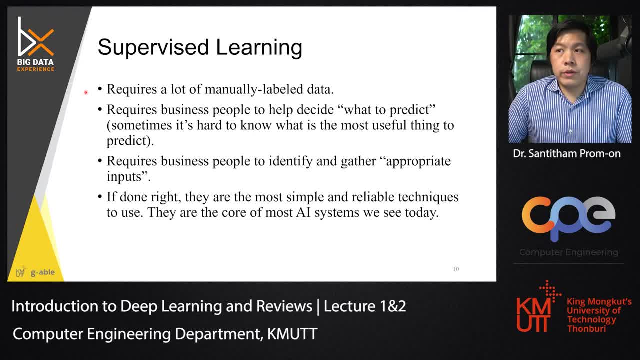 Okay. so when you are building the supervised learning, you need to have certain, certain, certain thing that you aim to predict, And those are the target. And identifying your target is actually very, very essential to solve proper business problem. If done right, then you will have 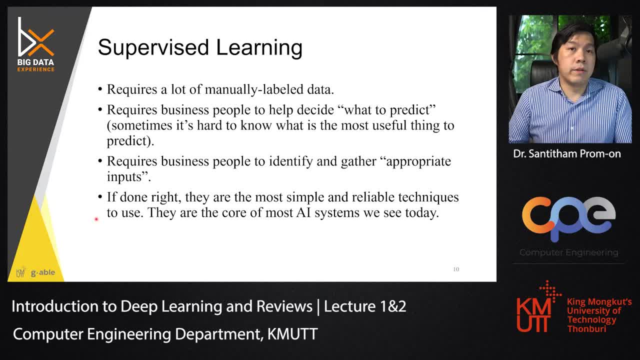 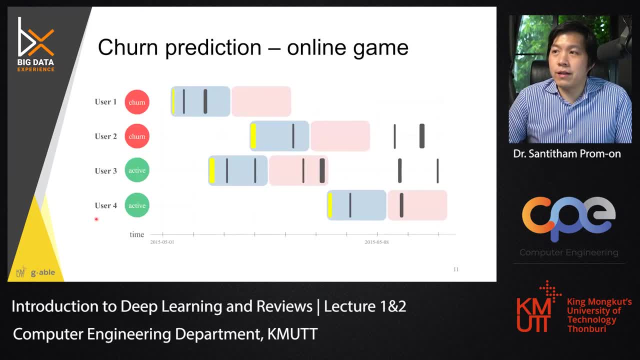 a simple model that is powerful If done. if you perform it wrongly, then you have a model that you cannot use In any case. right, For example, might want the task like churn prediction or like game churn prediction. you may want to predict which 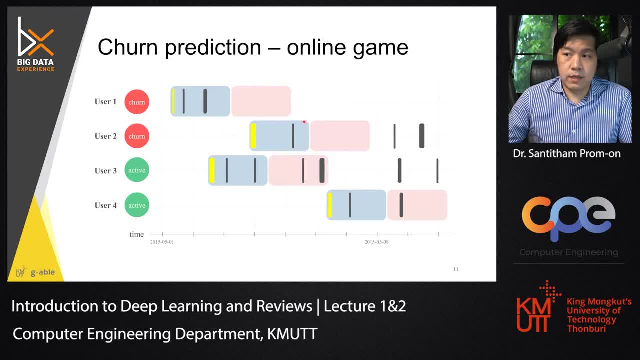 user will churn or not returning to the games based on the playing pattern. in that case you have the label as churn and not churn, active and not active, and then you have the previous historical data of those users playing the game in the session in the credit risk scoring this. 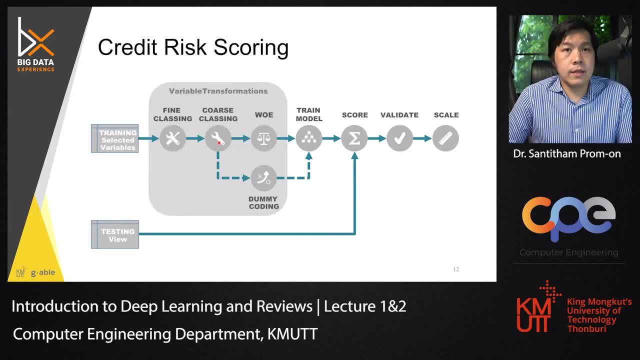 is also another example of supervised learning. you need the data comparing between those who have problems with credit not paying and those who have- uh, those who are okay, paying on time and whatsoever. then you can train the model so that you have the model that is trained based on a certain. these are by the classic method in in credit scoring. first you need to identify. 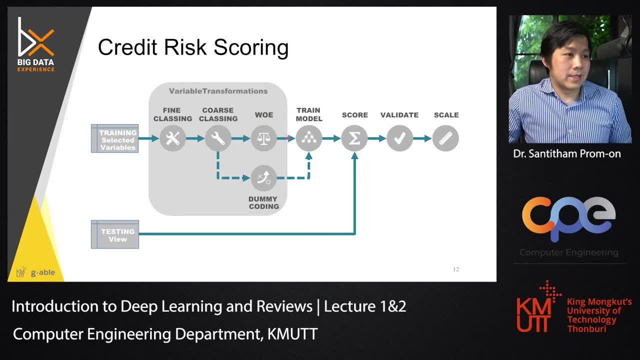 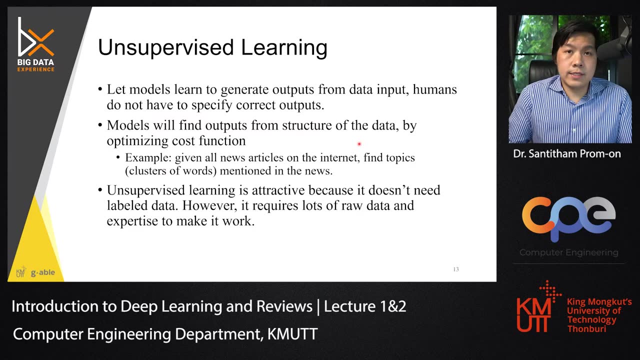 the variable based on the weight of evidence. once you get the set of variable, you can train the model and then you can predict using the score. you can use the test set to validate whether the result is okay or not. these are the tasks of supervised learning. the unsupervised learning relies on similarities, co-occurrence. 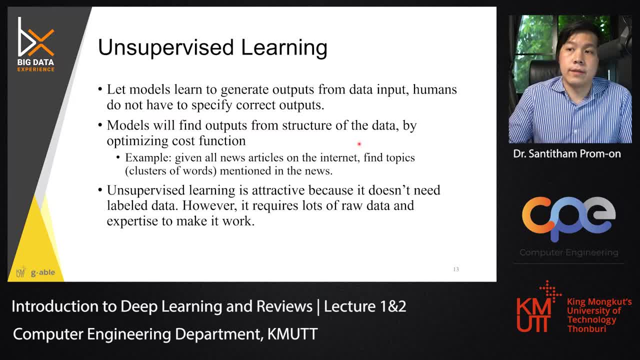 something that say they are close together. okay, so there's the unsupervised learning technique allows the model to identify patterns and those patterns are something like the consistency pattern in the datas. so it will find some structure out of the data set, like in clustering technique, which will find the cluster of data that are close together in the graph clustering. 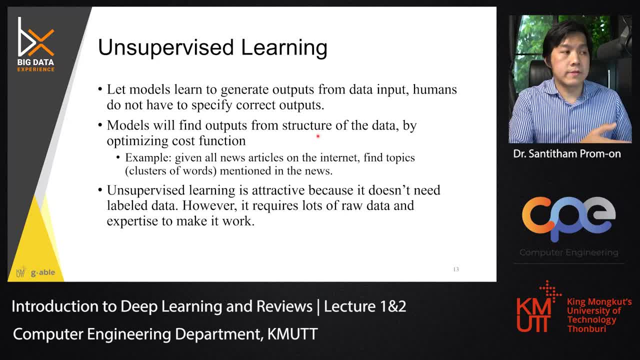 it might find the the graph cluster that have certain associations between them. okay, as a wise, Hetal is a quite attractive technique when you want to look at the arrangement, the structure, the outliers, the group of data that occurs together, like in retail you might want to see. 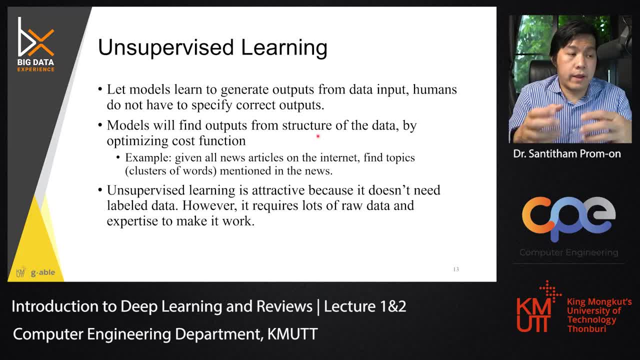 whether customer on on would f i buy the products, whether they would buy the product together in a set and and, and which product is usually bought alone. so understanding this, which product is usually bought alone, so understanding this, or which product you have to recognize, that is very lot. to understand this how. I wish you can make an перек here to so understand where you go from that to say, some work into the Villanova design, like so returning theитай to a classic model, that, for example, amiory mediaah here to existing model, like on speculation aboutill. 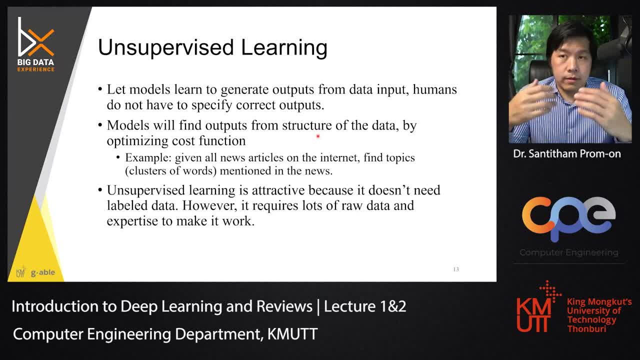 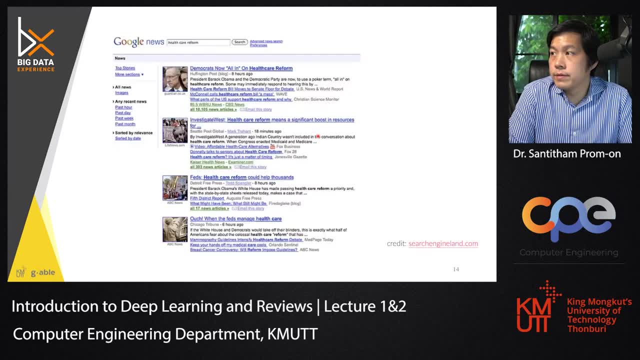 glass into history, inight details like you can uh on screen: which course, which skeleton. understanding this would allow, like the marketing people, to come up with some strategy to sell the product. Examples are like the news story. News story comes out. news comes out every day, right? 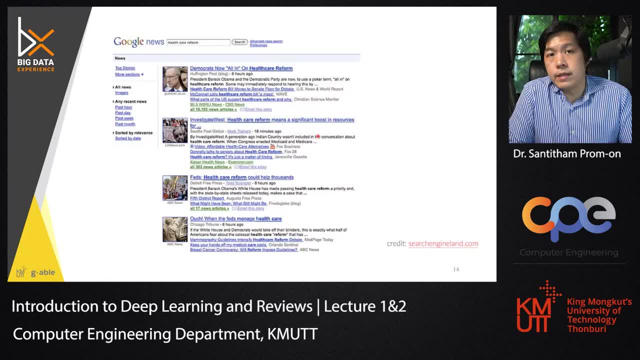 And in order to process the news nowadays, there are a model that can group the news together if they belong to the same category. right, Performing something like text clustering or topic modeling will allow us to identify that the news are close together and they should be grouped as the same group. And if those groups contain certain labels, then 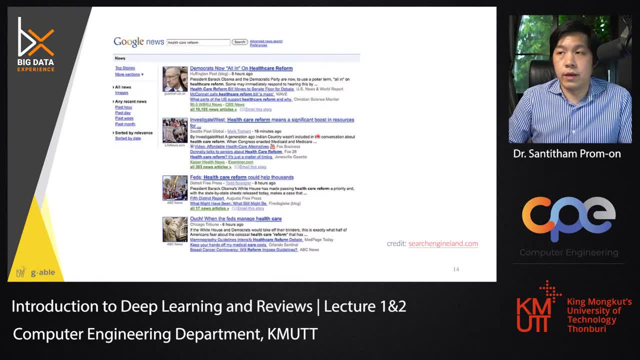 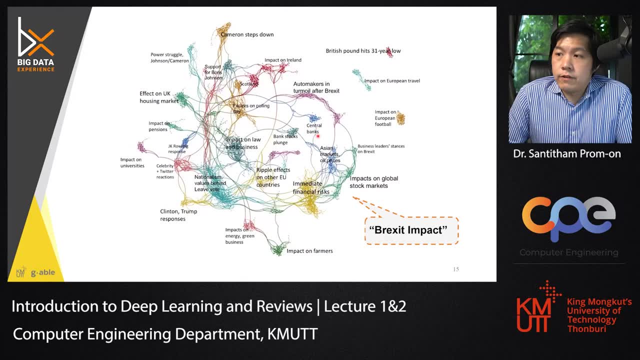 you can certainly propagate those labels to those that you do not know, that you do not know which topics they contain. This is an example. This is an example of the study on Brexit. Oh, this is quite a long time ago and I still 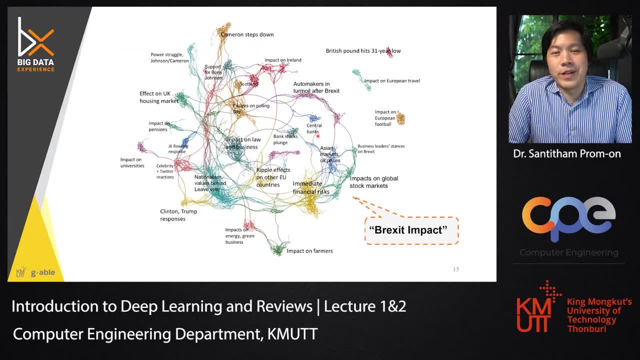 use this like man. maybe I should do something like COVID-19,. right, That would be more of the latest, Never mind. So these are the topics that are on the news article that are related to one another in COVID, using a technique called topics modeling and graph analytics. 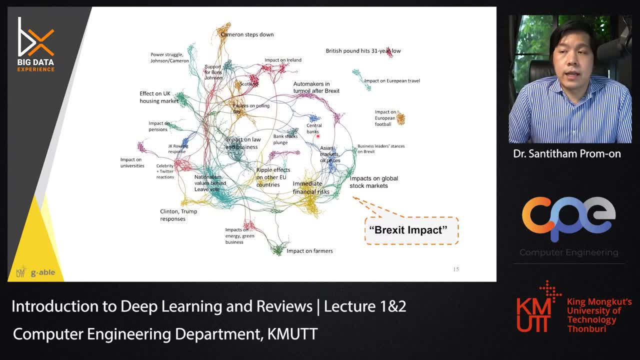 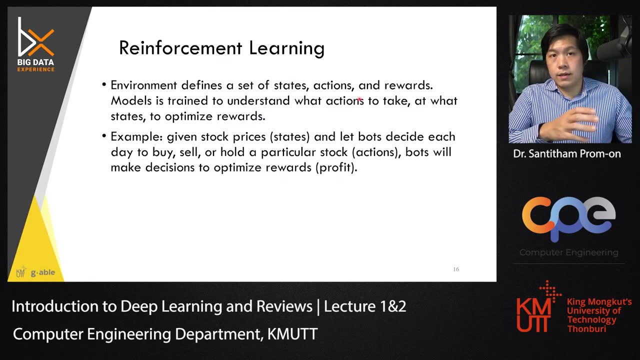 together And then you can identify that certain topics are associated, that are associated with each other, with one another, and then you can see that there are certain isolated topics that have been discussed but are not linked to others. okay, so these are. the first is the supervised learning, unsupervised learning, and this is 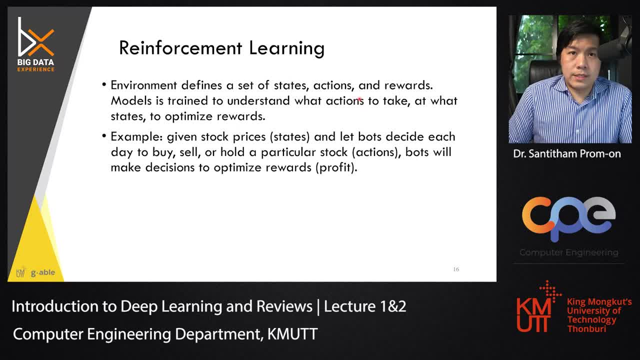 reinforcement learning. reinforcement learning used simulation right, quite exciting. use the environment that you need to define. the environment contains the state, action and reward. you need to define all of this so that the model that you train can learn from this environment. so it depends on the environment that you create which will allow you to train the model differently. 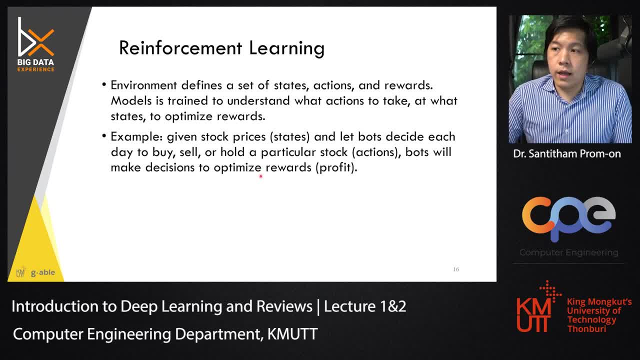 for example, if you were to create a very realistic stock simulation and you let the bot decide whether to buy, sell whole or doing the stock actions you, then the bot can decide whether to take action or not, and then it will take the reward as the objective. 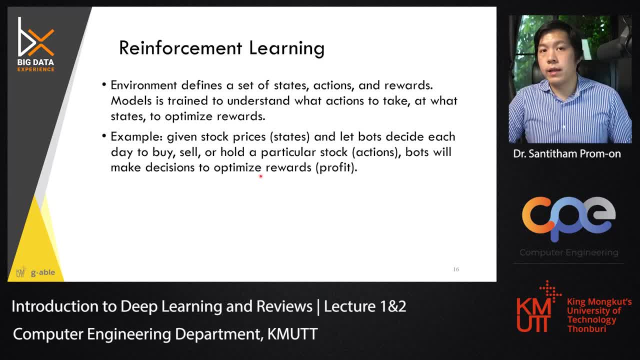 and then let the bot learn what to do And then afterwards you can then use the bot that is learned, based on the virtual environment, to deploy in the way of things. So hopefully it would work. Let's take a look at some example here. 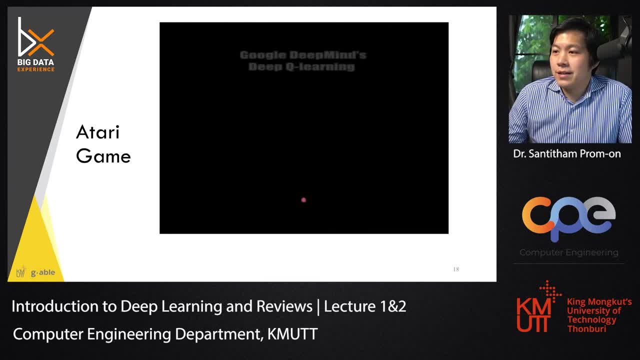 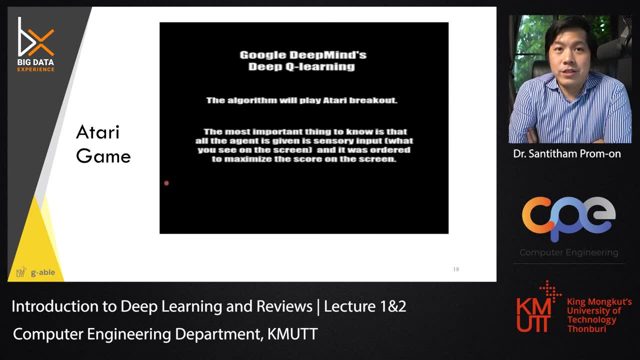 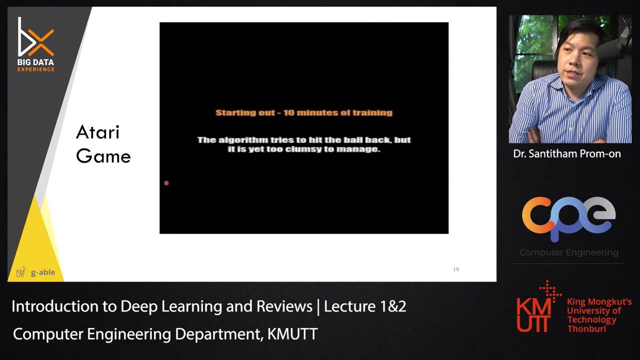 This is an Atari games, Yeah, that use deep Q learning to learn the action, whether it should go left or right and how much. Yeah, let's take a look at this, Okay. so these are the first 10 minutes of learning. 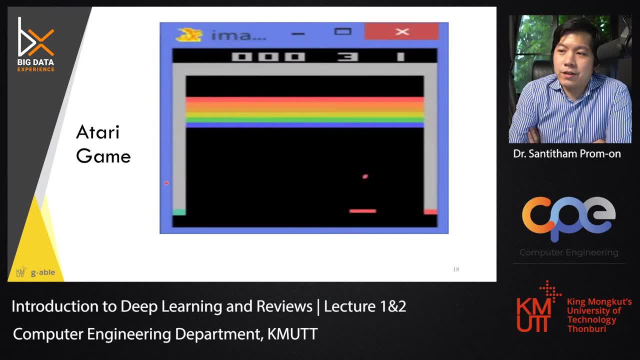 and you can see that the bot still cannot control very well. so it missed a lot right And once it missed it will be like there will be penalties to the objective function. If it can receive that, it earns some score. 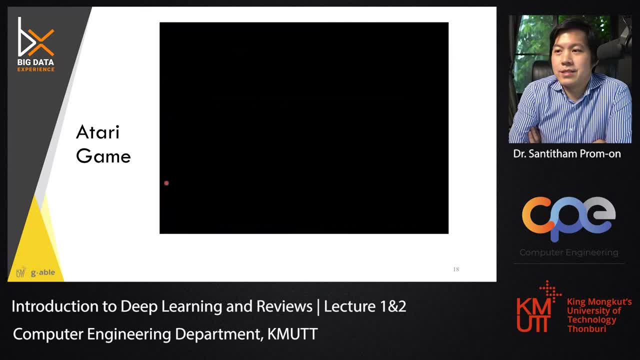 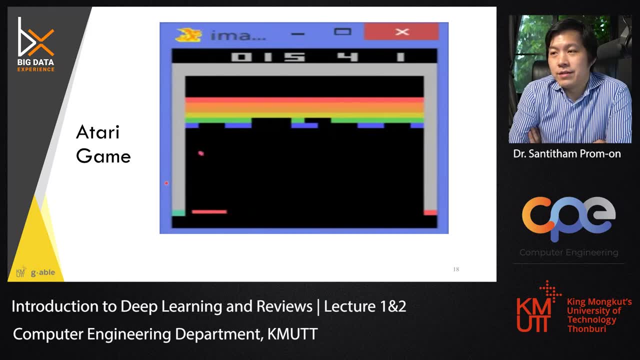 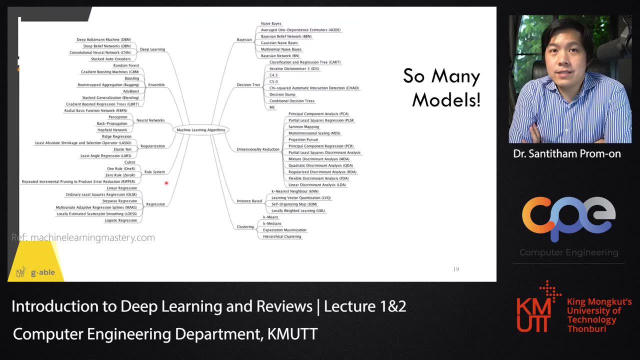 After two hours of training, doesn't specify what type of computer it use. you can try it yourself using deep Q learning to write the gameplay And you can see that the bot is able to do a lot of different things. So that is reinforcement learning, okay. 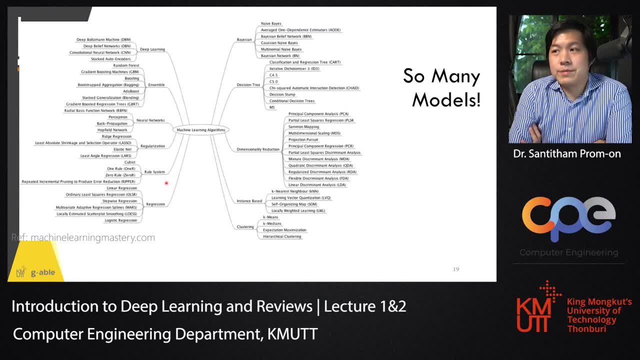 And there are all the types of technique, many models in machine learning. Some of you may have already encountered some of this and learned it with me in the other courses. like there are techniques on the Ensembler-based models, on the Bayesian, on the technique to reduce the data. 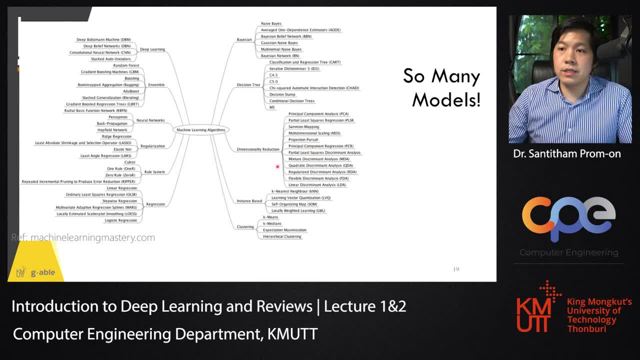 to compress it based on dimensionality reduction. on the Bayesian. on the technique to reduce the data. to compress it based on dimensionality reduction. on the Bayesian. on the technique to reduce the data. to compress it based on dimensionality reduction. 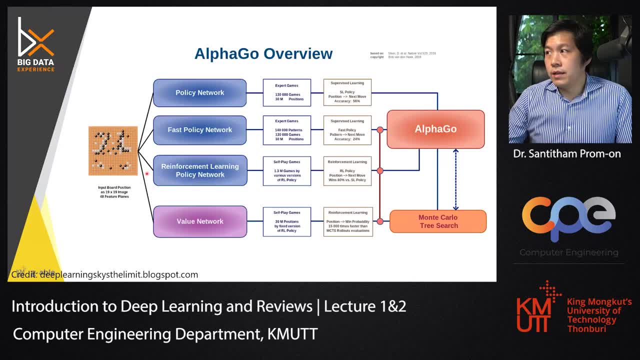 and other types of techniques which will be suitable for different tasks. An example of the combination of deep learning and reinforcement learning is the AlphaGo. The AlphaGo has different types of network that perform differently. Some of them will be the policy network, which select the policy to perform. 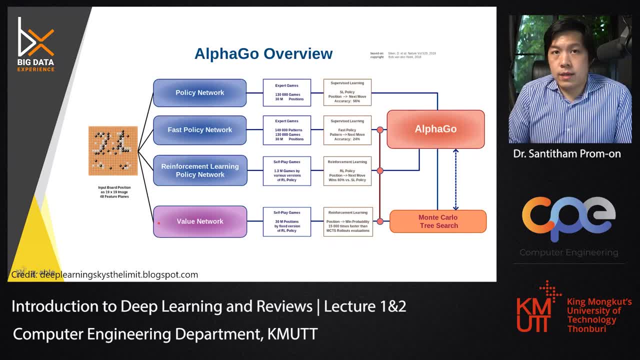 Some will be the value network, that based on the value, based on the actual perceived value, and then shows the action. Then, combining the result of all of these, the AlphaGo make decision on what type of thing that it should do based on certain Monte Carlo tree search. 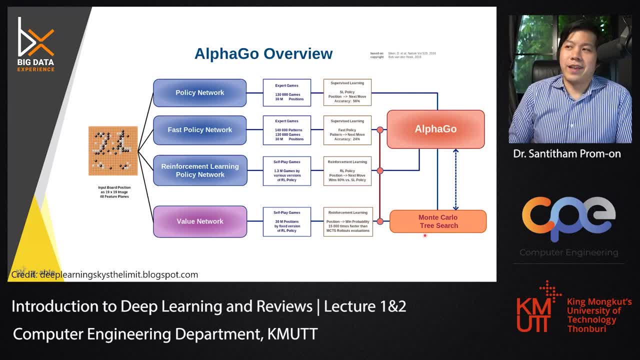 So there will be certain randomness in the movement. If you are interested in the AlphaGo, in the reinforcement, learning and combination, all the combination of different type of network together, you can find the link in the credit here. I would suggest that for that. 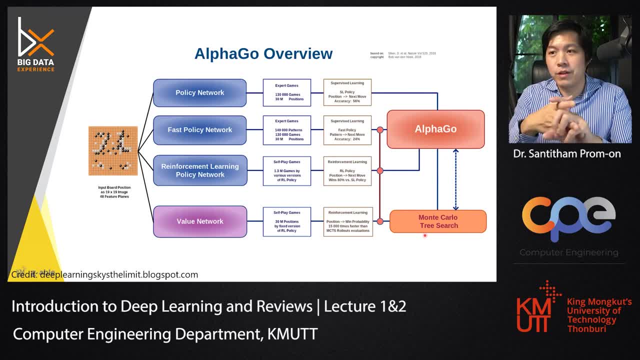 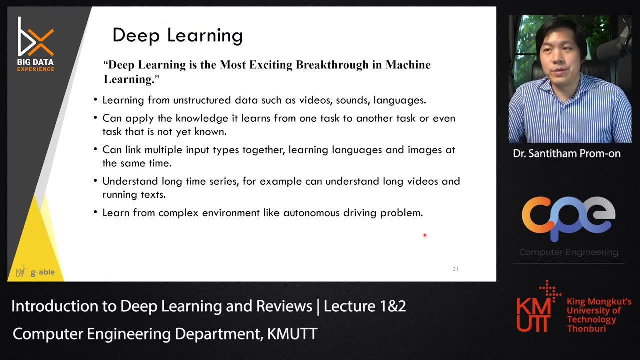 you should understand how to create a deep learning model here first, and also how to do reinforcement learning. then combination of them will come afterward Right. so that lead to here, to the deep learning. Deep learning is one of the exciting technique. 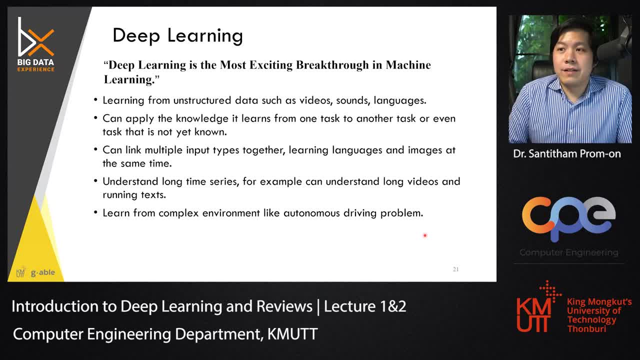 one of the exciting breakthrough in machine learning. It learn the. it can learn structured well. it can learn the goodness of deep learning. It's not its capability in the tabular data, in the structure, the structured data. no Structure if you have structured data. 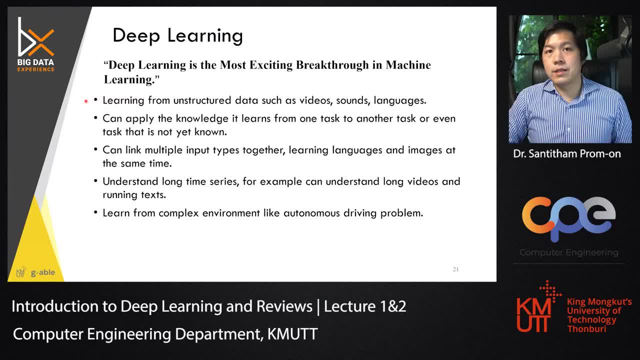 you better use general machine learning like decision tree, random forest, the gradient boosting. But when you have the unstructured data, those machine learning technique would be struggles to beat deep learning techniques. Why is that? Because there is one essential things that deep learning can do. 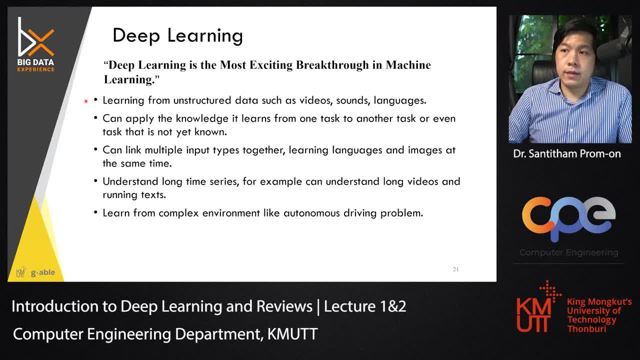 which is to extract features automatically, Right. That's why it is good for the unstructured data. It can learn the representation of data right. This technique can apply the knowledge that it is learned from one task to another task as well, And you will see that in the latter, the latter section. 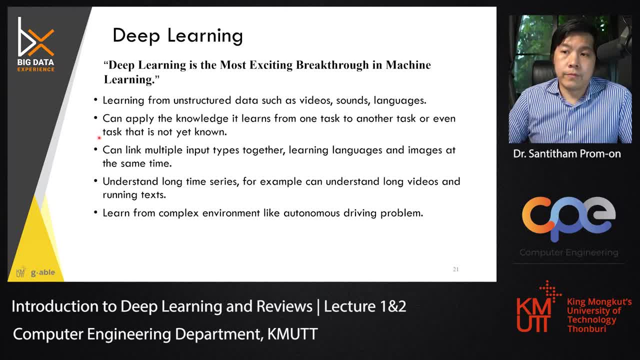 especially in the technique like embedding in the technique that compress the data in auto-encoder- I will look at that later on. You also link multiple input at the same times and it can also understand different types of unstructured data- the series data- and then can be used in complex environment. 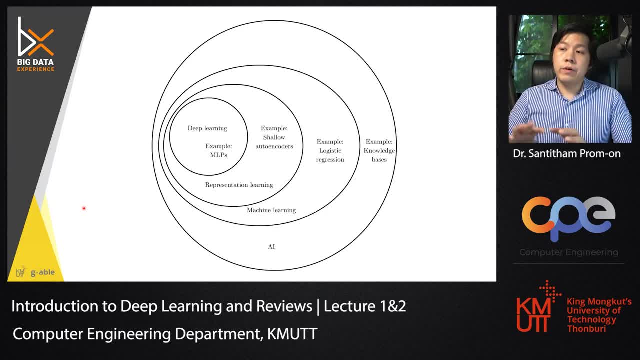 if you train it properly. So if you were to build a deep learning and AI association, AI is like the general fields, that contains lots of technique. Reasoning is also one of that, not related to deep learning or machine learning at all, But the logic, the logical operator. 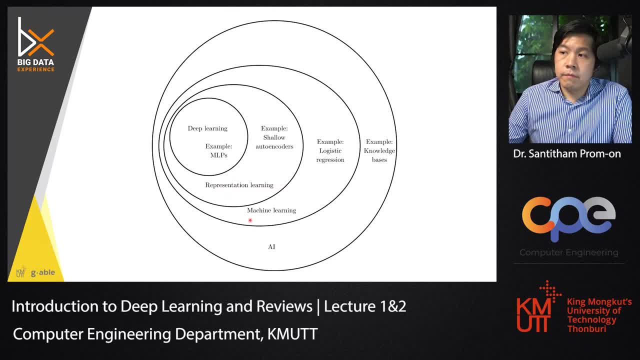 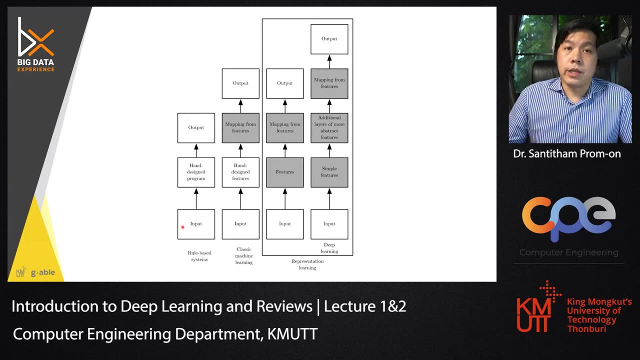 that is actually originally part of AI. Machine learning is like subset of deep learning and deep learning is part of the technique that learn the representation Right Inside here. Okay, What is representation learning In the system? right, if you were to go outside? 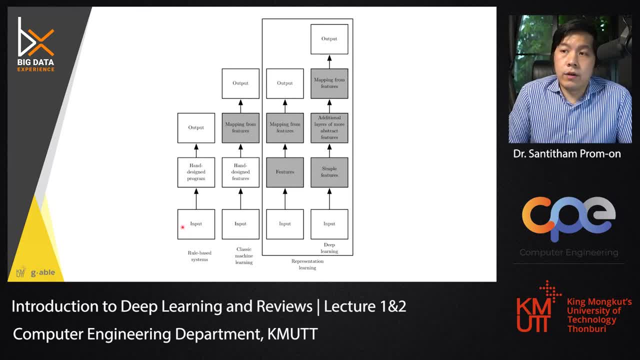 and then look at if you work for the company and then look at lots of system in the company, you will see that Right now the state of AI in the company mostly relies on the hand-designed program, on the threshold, on the logic. 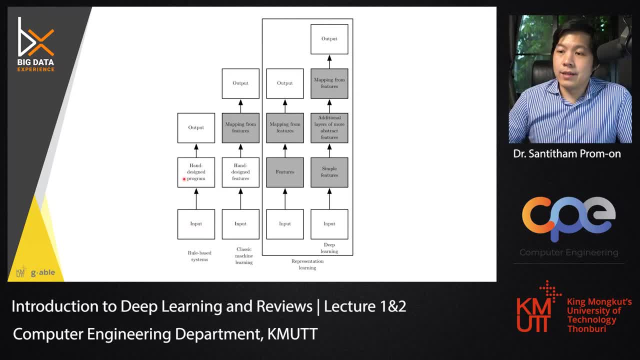 on the if-else tree that has been decided. This is the rule-based system, right? This is one of the classic artificial intelligence that we are trying to incorporate the criteria into the system so that it can make decision based on those criteria. The reason I call this an AI. 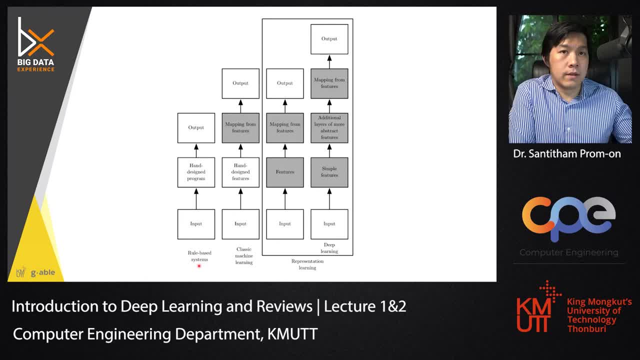 because if you go back like 20 years ago- or, yeah, 20 years ago, the field of AI actually encapsulates those type of things as well. When you want to make reasoning judgment decision, that is part of the AI. 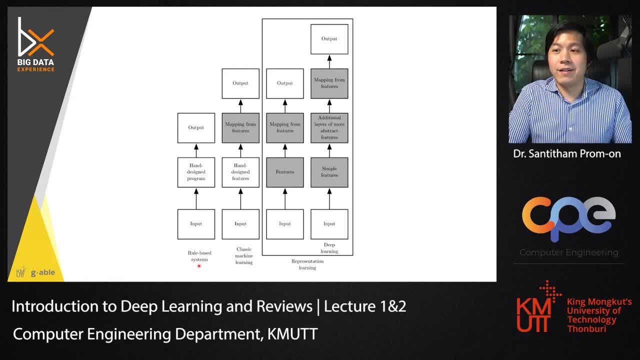 And, if-else, is actually part of the AI. on the original AI, the expert systems Move on to about the years 90s to 2000,. the technique on machine learning has been advanced, partly because of the power of computer and also the algorithms itself. 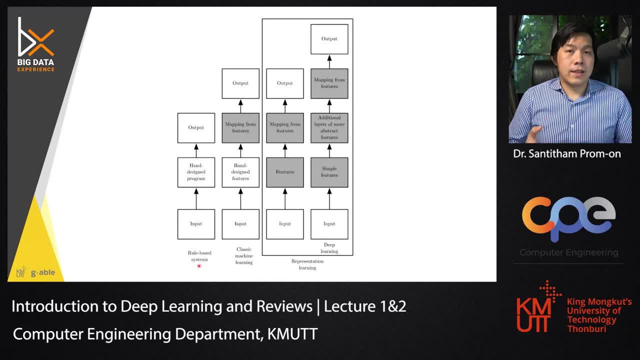 We have lots of techniques that can map between input and output. Actually, my early studies were driven by these types of things as well. Back then it is called pattern recognition. I have a book called Pattern Recognition back then- and then it is mostly used with like signal data. 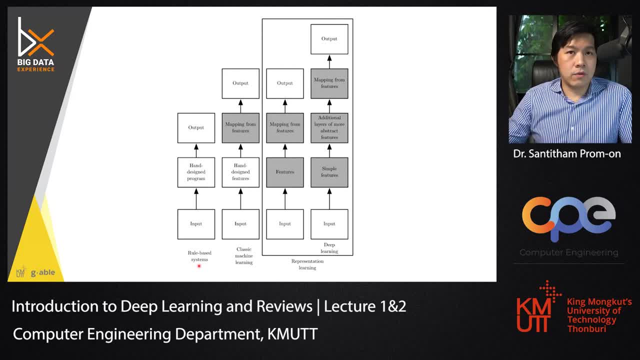 image data to perform different tasks. that is not quite commercialized yet, But now today because of the general framework that anyone can use. so now we can apply the machine learning to data And then part of the data science is a study, by creating a model based on the phenomenon as well. 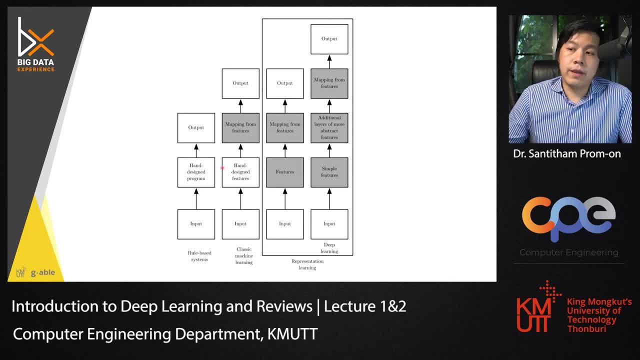 So these are classical machine learning You need to have like hand-designed features, like extracting features of this month, comparing to the last month as a tabular data, and then let the model learn from those tabular data and then make decision later on. 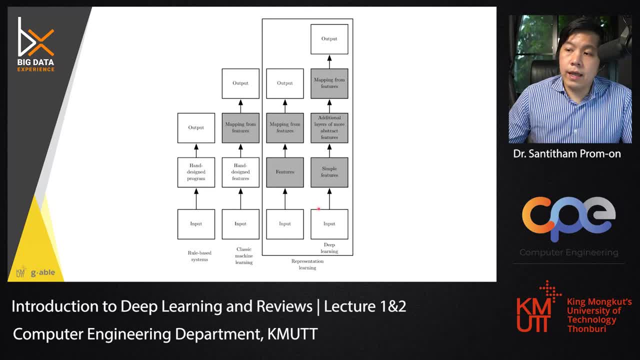 For the deep learning and the representational learning. you have input and output, but you want the model to learn all these things. It needs to learn the features and learn the mapping And, in the deep learning sense, it needs to learn the additional layer. 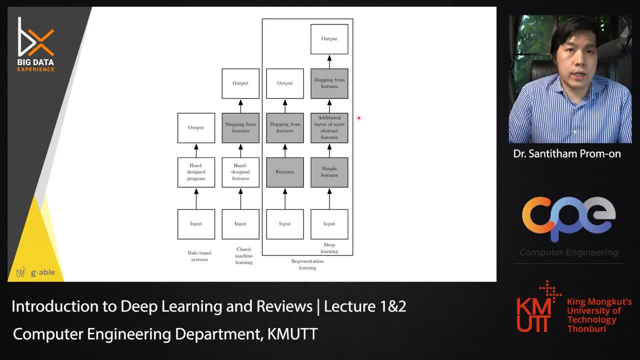 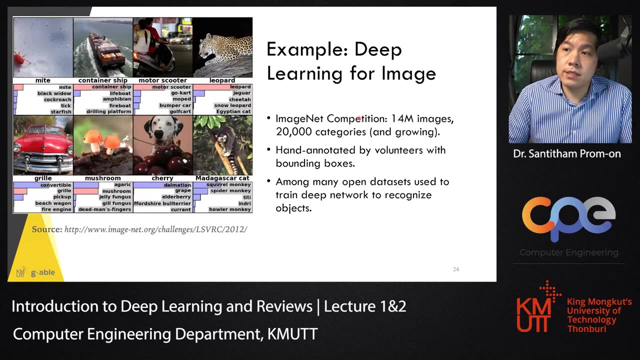 It needs to learn which layers are important, which are not, and then make sense, and then trying to kind of prune them out themselves if possible. This is representation learning. So deep learning has been applied to different types of tasks. This is one of them. 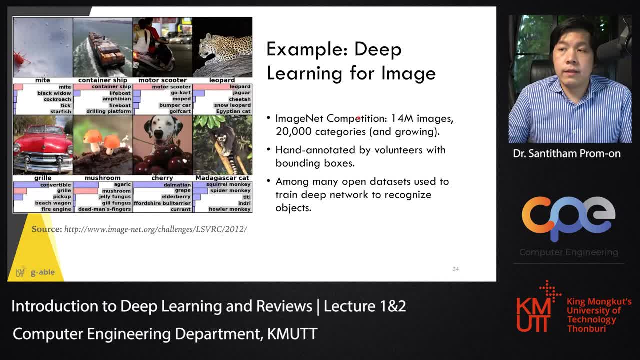 It can be used to perform image classification In the deep learning. in the ImageNet competition the participant has to classify like 14 million images of 20,000 categories, And these images are annotated manually by humans, So we can be sure that they should be correct. 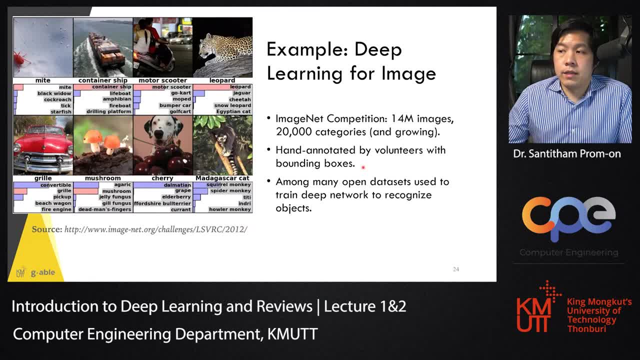 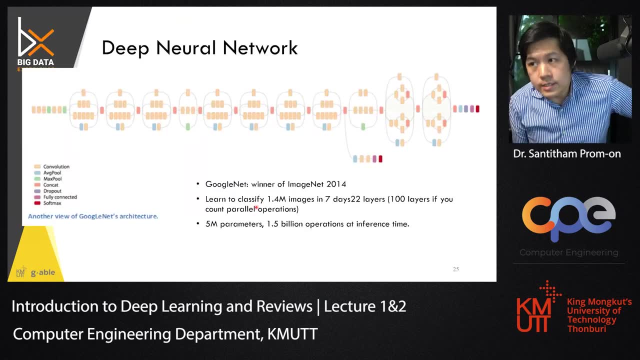 And it has been tested on many sets and some of the model is quite powerful that you can even deploy to on. Once it learns the ImageNet, you can actually transfer it and use it on other tasks as well. So it looks like this: 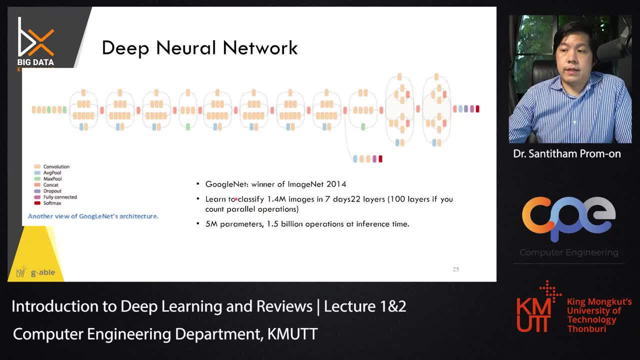 This is one of the. This is a GoogleNet right. There are many different types of network, like the VGG, the ResNet, which we will talk about it later in the convolutional neural network lecture. So you will understand why are they working. 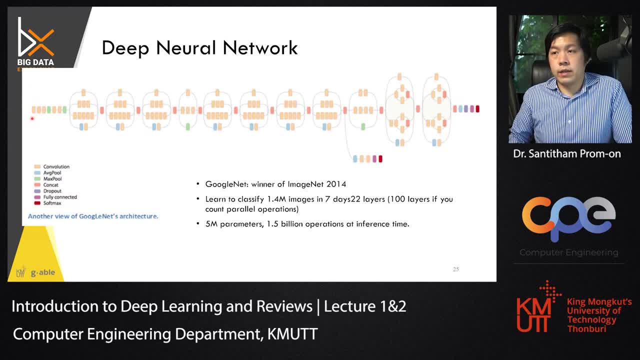 and why the usual feed-forward are not working. So it looks like this one. It contains lots of convolutional layers and other types of layers which, if you do not know right now, it's fine, We will talk about it later. But yeah, it's called deep. 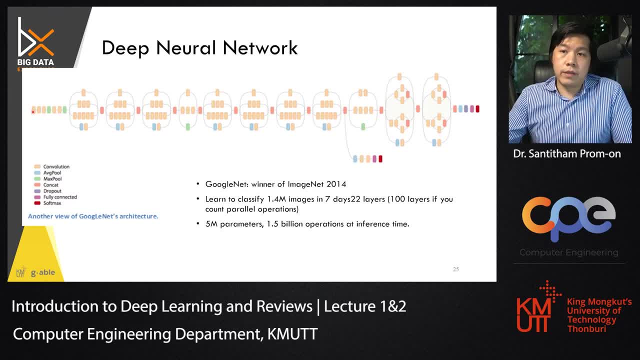 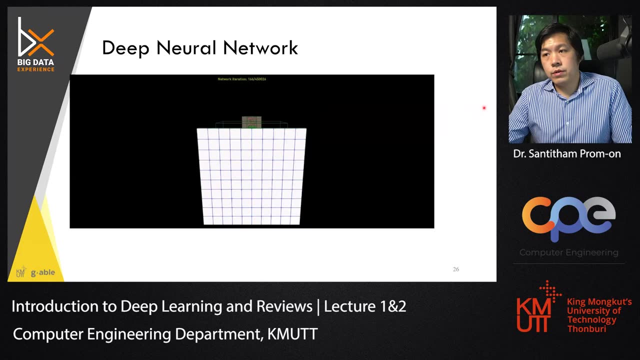 because it contains lots of layers from input, left-hand side here- to output here that you have the softmax and fully connected to perform classification at the end. Okay, And the deep learning model has to, has to expose, has to be exposed to. 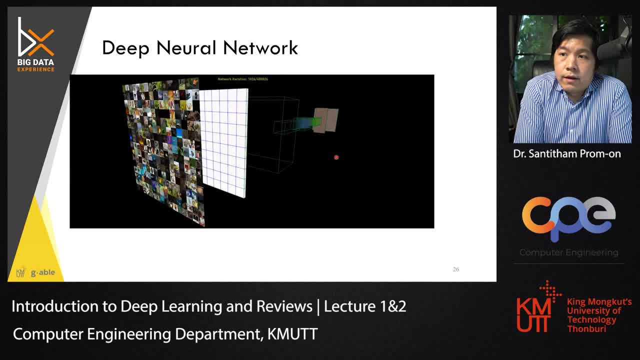 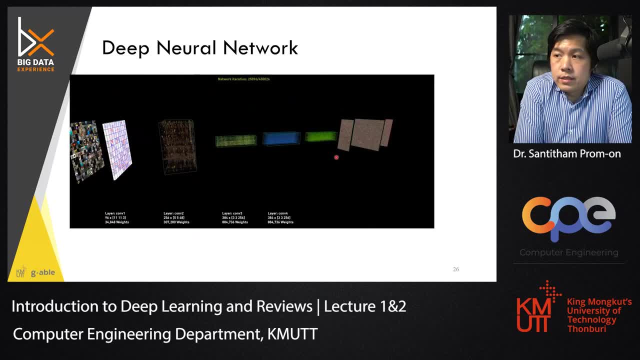 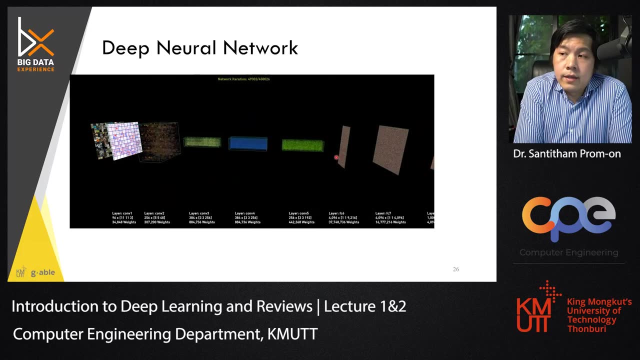 lots of input and then, when it is exposed, the weights in the model will be learned at different layers. Each of these layers can be extracted to view what happens there And actually when you learn further in the later lectures we will extract this feature map out. 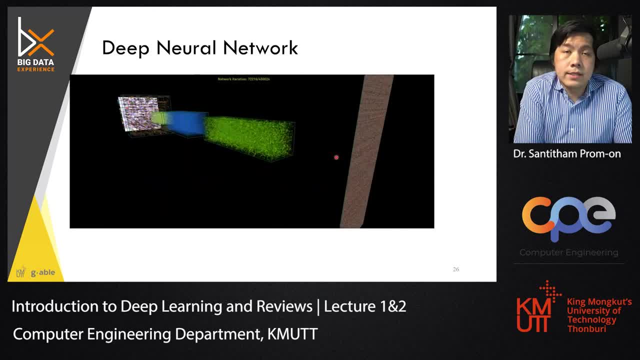 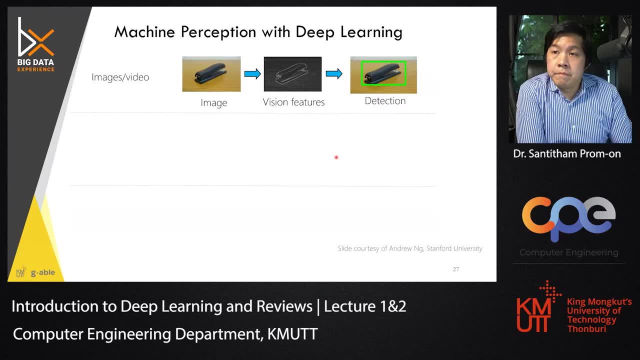 to see what actually happens there and why does it matter? Okay, So we can use deep learning to perform machine perception. Actually, you can use. This is live image that tells you the story about the usual machine learning In usual machine learning. 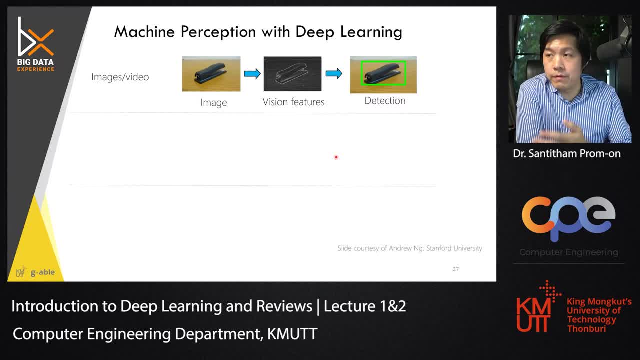 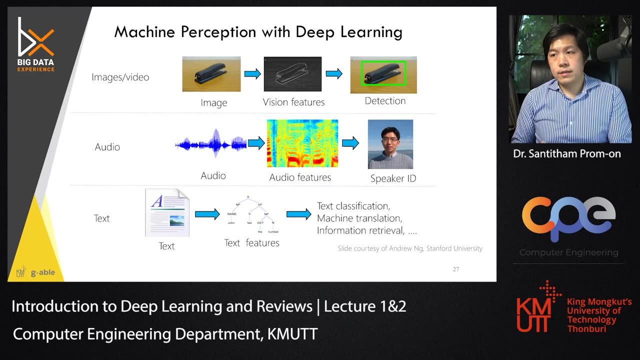 you have image, You have to extract vision features, then perform the task In the speech audio. In speech audio, you have to extract audio features and then perform the task. In text, you have to extract the textual features and then perform the task. 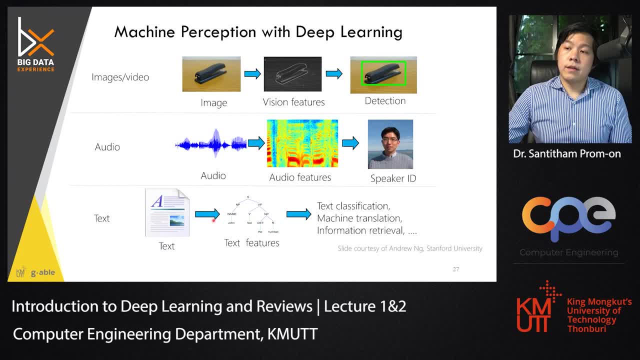 But in deep learning you are kind of including these feature extraction in toward the model, So the model will have to do the task entirely. But that's not always true. For example, when you study about this further, you will see that 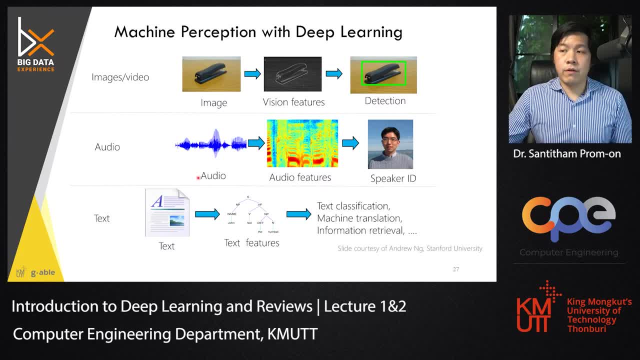 sometimes pre-process the data before putting it to deep learning is a good way to do the job. For example, if you work on speech processing, putting the whole audio file into the model is not a good idea because usually the speech content is in form of frequency movement. 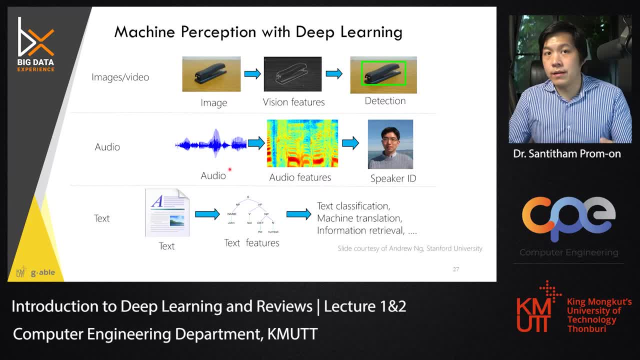 So you might want to convert it into the spectrogram, Convert it into the filter banks of the frequency, Or, if your task is to extract, Well, an image is quite obvious, so I'm not going to talk about it here. 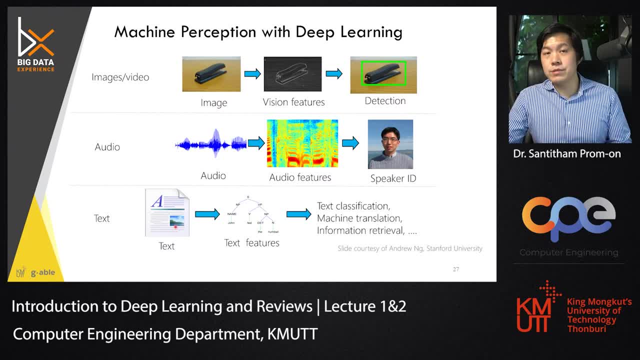 For the text. you need to process it somehow So that the data- Like, for example, you need to actually tokenize the text first, Like, for example, to do the Thai text processing. tokenize the text first before doing all the tasks. 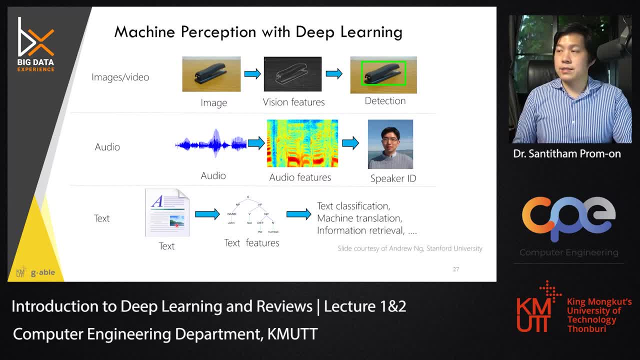 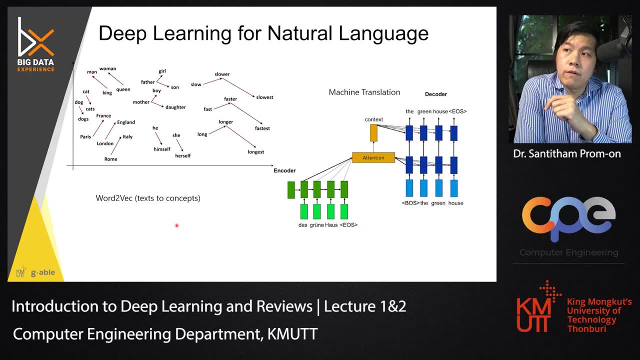 that related to text analytics there And deep learning can be applied to different work. You can see that it works for image. It also works for natural language processing. There are lots of work related to natural language which I cannot co-create, So I'm going to cover it here in this course entirely. 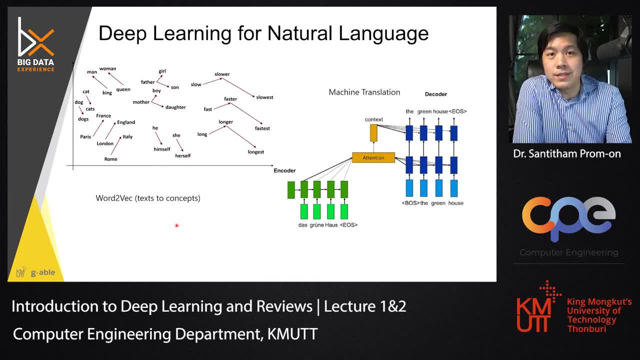 So usually I would have the text mining course separately, but this year I opened it for the undergrad to dump it down to the coding level. But I think there is a course called natural language processing. If you are interested in the detail you can register for that course. 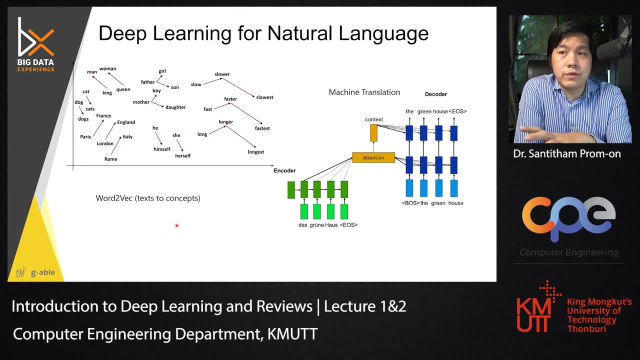 For this. I would just want to mention that you can use it with natural language, And we will briefly work on this in the language modeling and in the sequential data in the recurrent neural network later on. Okay, so learning the representation allows us to identify the words. 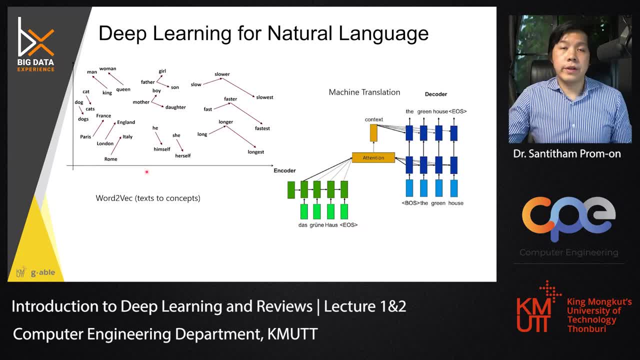 that have similar contexts, like the word to wake, that train on the basic, quite basic, quite basic structure, But it can learn the association between words Or the machine translation, the attention, the transformer, the latest technique that allows you to perform the sequential model. 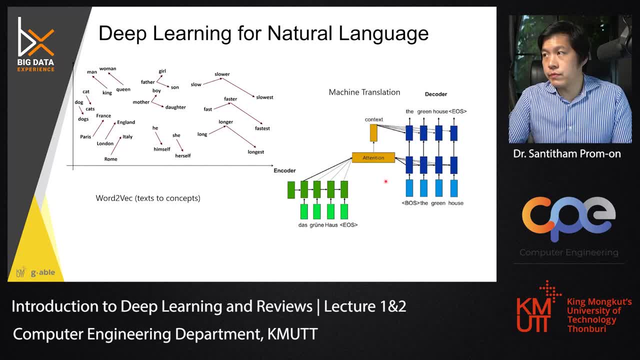 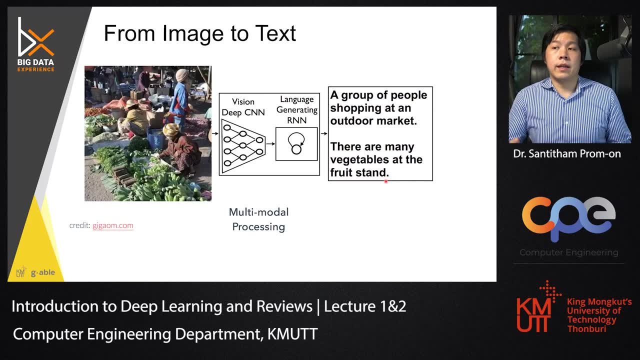 that captures the context in the sequence as well. Combining them together, you may have the model that learn from image and then generate the language by plugging in the structure, the convolutional structure, with the recurrent structure. Let the model learn itself on how to translate from the picture. 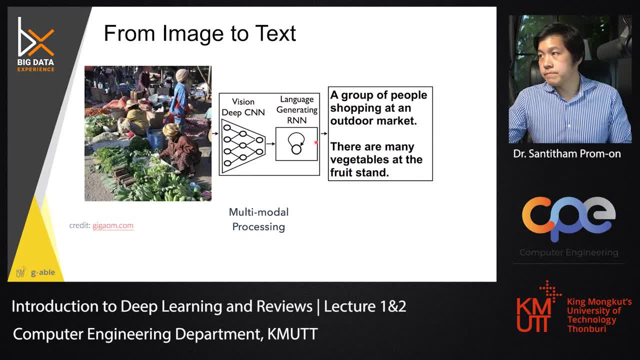 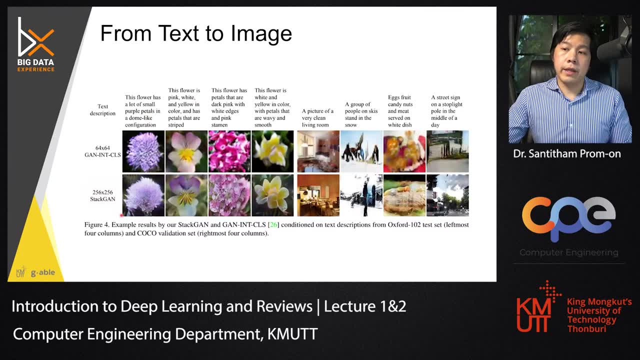 into the sequence of data here, From text to image, that when you describe it as text, you can generate image based on certain generative model, like GAN, the generative adversarial network, which is quite an interesting concept that can be used to do the generation. 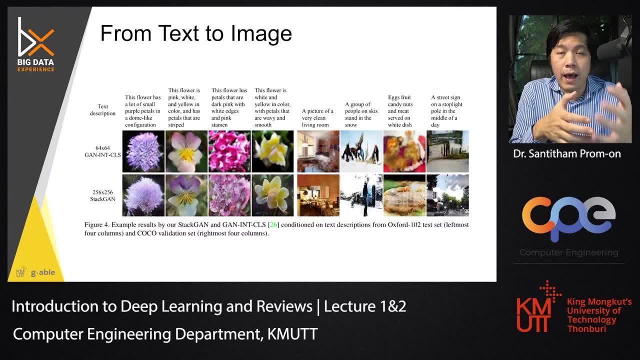 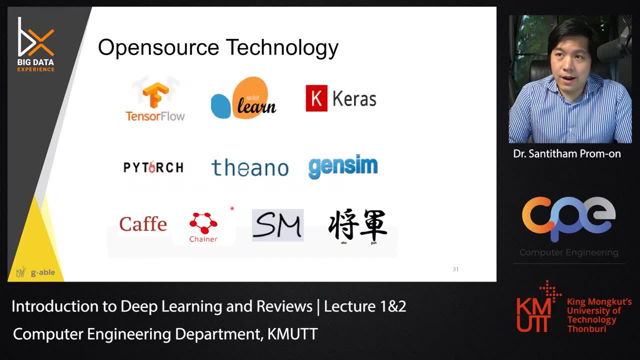 as well as to perform, to be part of of the analysis system, to train the model, To use deep learning now, today is not that hard. There are plenty of open source that you can use. These are not limited to. these are some examples. 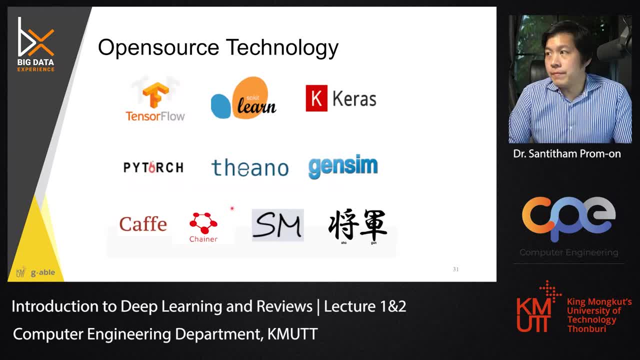 and they are quite like the leader in the fields. In my course, I usually use Keras and TensorFlow, which, well, is quite simple to access, But feel free to use PyTorch and Authors, because our course will not be about coding. 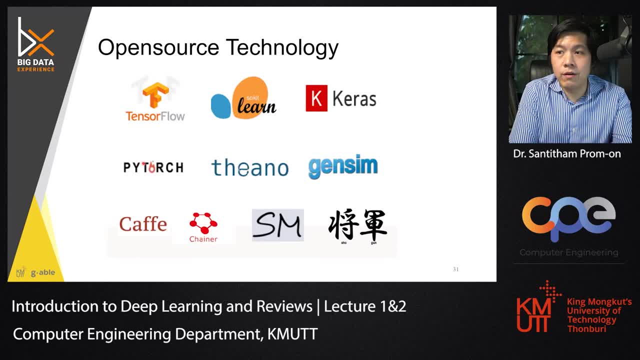 Some of you have passed us already in coding in the AIs. Our course will not be about coding entirely. Our course will be about the inside of the model, So it will be about the mathematical foundation of the models. So here are the learning outcomes. 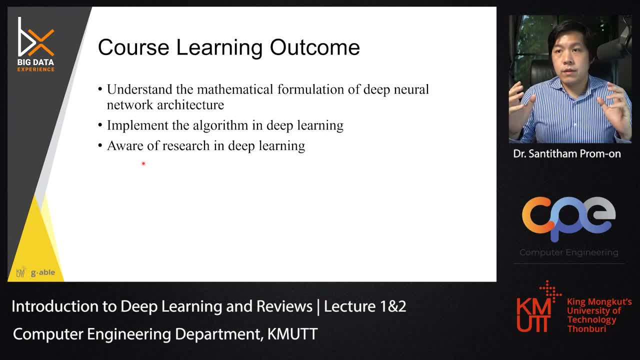 The learning outcome in this course is to understand the mathematical formulation of the deep learning neural network architecture, Deep neural network architecture, And you will also implement an algorithm in deep learning. But mostly you can. well, you can use libraries later on, But I think first two lectures. 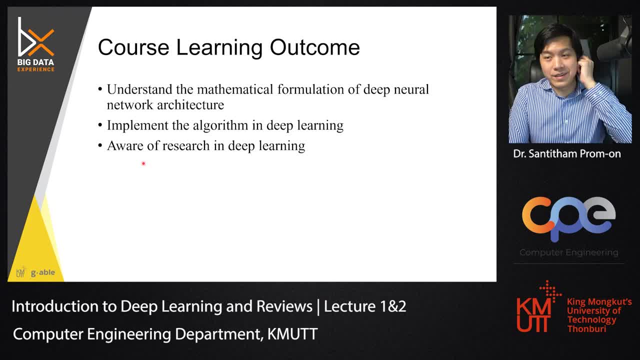 you need to write it your own, if I remember correctly. And lastly, you have to do the research in deep learning as well and then present the papers to the class as the term project. I usually not call it a term project, It's actually a term paper. 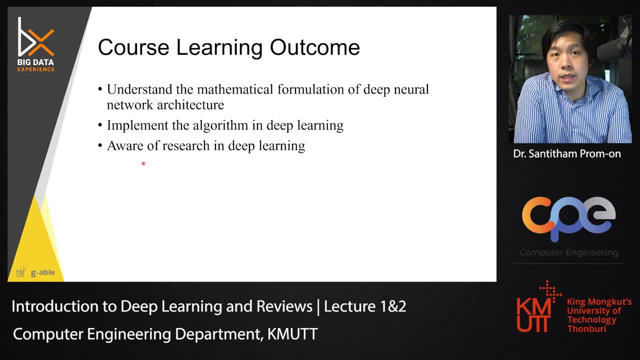 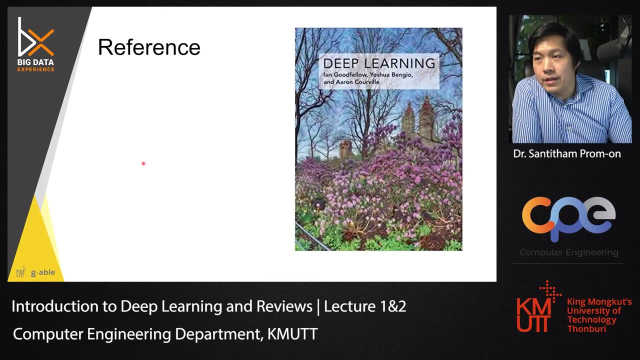 You have to select one paper, one interesting paper, that you would like to study, and then present it to the class. Your score will depend on the intelligibility of your presentations and how well you teach your peers about those techniques. Here's the textbook. 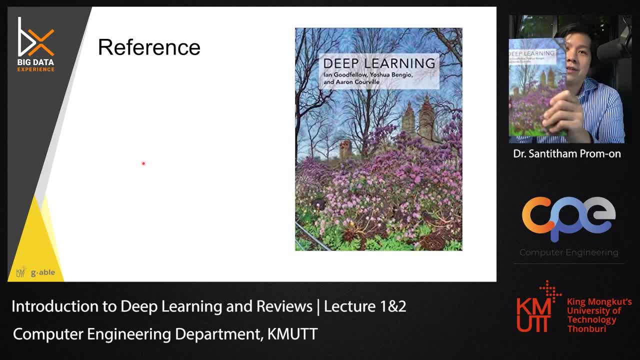 the reference book that I use, Quite a hardcore book by Ian Goodfellow. In this book there are no codes, But there are actually lots of equations. Yeah, Lots and lots of equations. So, yeah, we will use this as. 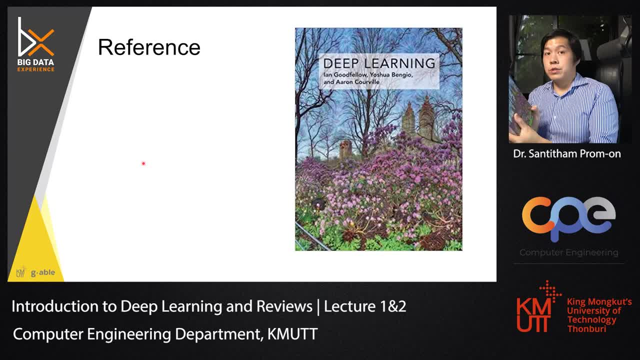 the textbook in this course. If you want to read through this, I would. if you are a new beginner, as a starter in deep learning, I will not recommend this book. Okay, Because this book is very, very difficult. It contains quite a lot of. 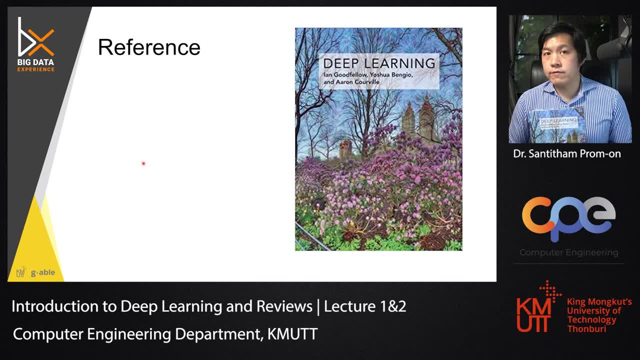 mathematical concepts that you probably need to have certain backgrounds before we proceed further. But if you want to start in the foundation of deep learning, this is one of the books that you must have. The simpler one would be Deep Learning with Python, The simple Deep Learning with Python. 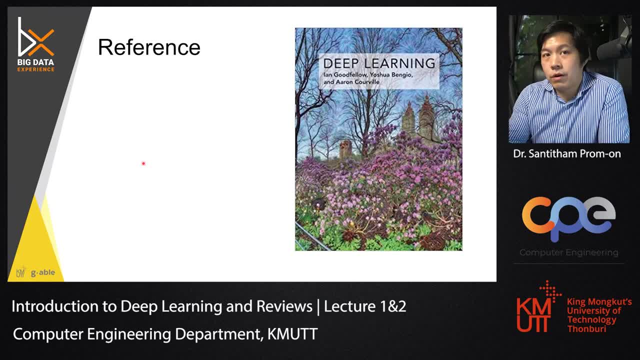 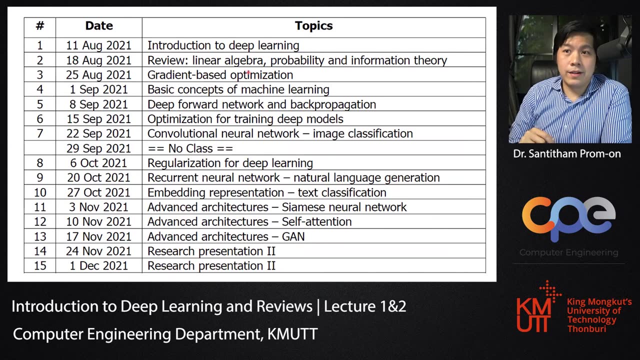 by the one that wrote Keras, or the tutorial online that you can find on the Keras and TensorFlow and PyTorch website, And the topics that we will cover in this course include the introduction to deep learning- is actually this one, And it's from the last time. 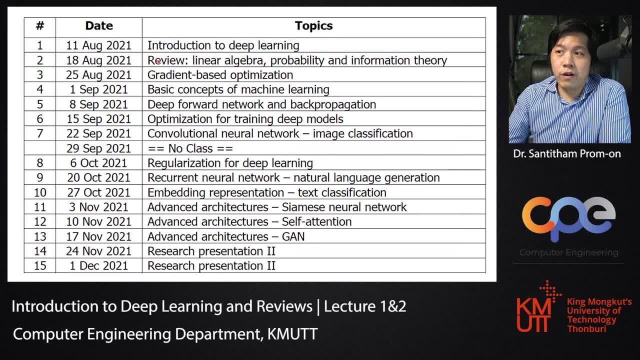 And this time we will cover the topics of the review of all of these theories, which is quite a lot. I will move along with the topics quickly, although I think I spent lots of time here. No, it's still fine. I still have about two hours to cover. 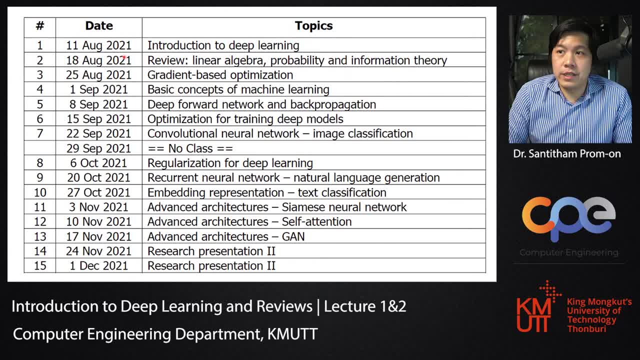 And the next time we will then jump to the gradient-based optimization, which you have. the first assignment: to write a program to do the gradient-based optimization. Then you learn the basic concept of machine learning. No, we are not learning about Decision 3.. We are going. 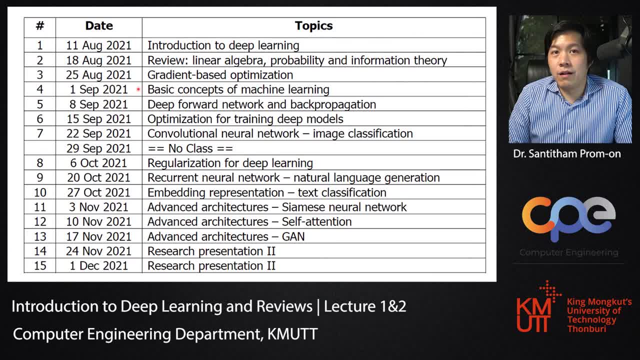 to learn about the basic of machine learning, About the loss function, the posterior probability and others, And optimization as well. And then it will be about the default and backpropagation algorithm and optimization of the deep learning. We will learn about the Adam-Nadam-Nesterov. 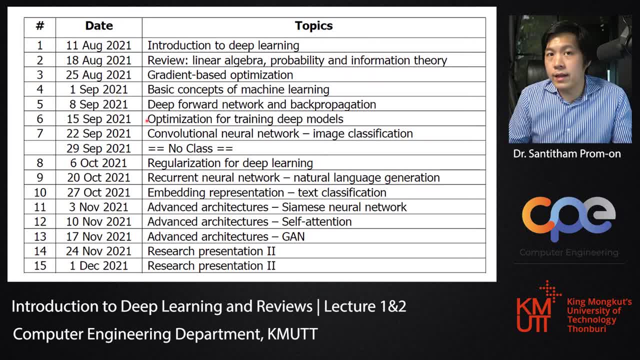 criterion, the adaptive moments and others. Why does it matter and how does it work in mathematical terms and in the library, which already have this thing to input as parameters, And afterwards it will be a class about convolutional neural network And then a simple image. 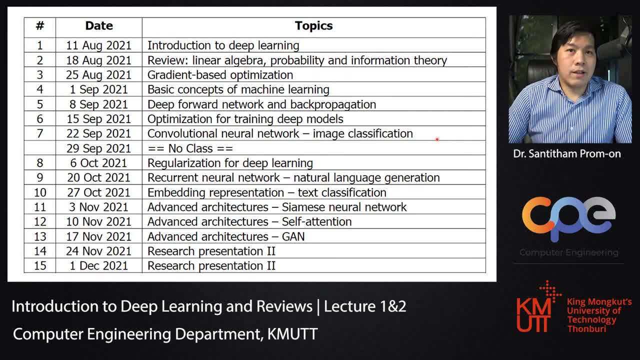 classification. If you already take coding in AI or deep learning course, this will be like the first one that you work on, But it will be a separate lecture and what you forgot on is not actually in terms of implementation. Implementation itself is quite simple, but 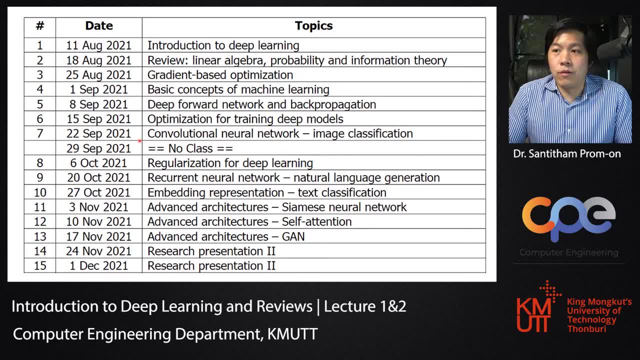 I want you to look at the detail on why does it work in the convolutional sense. Maybe you will create something that's similar to convolution later on. Okay, And then no class because of the midterm. After that, we will learn about. 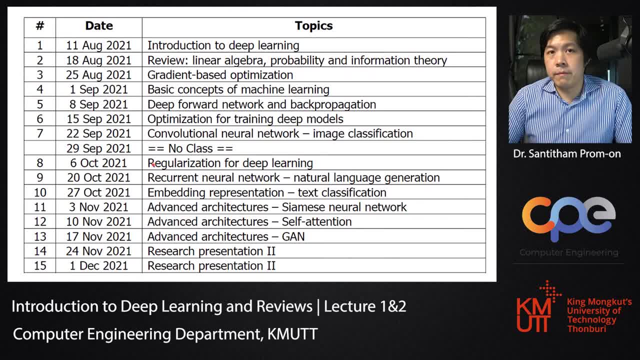 regularization. Dropout is one of that, but you can create different type of regularization based on the structure. We will look at that here, And then recurrent neural network And embedding, which is an classification here. Then there will be like three lectures. 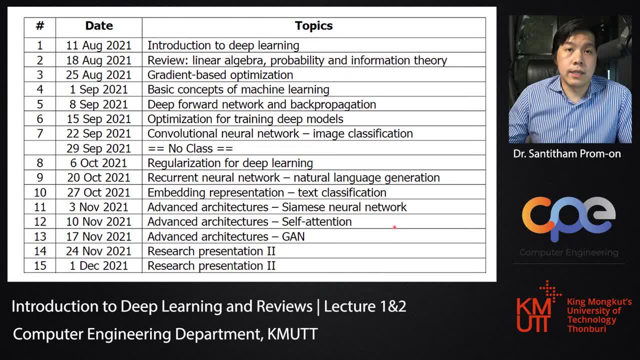 which I will cover the three concepts, three advanced concepts here. Last year I covered the Siamese neural network- That's why it's here- And for this year we'll talk about the self-attention here to learn about self-attention a bit. 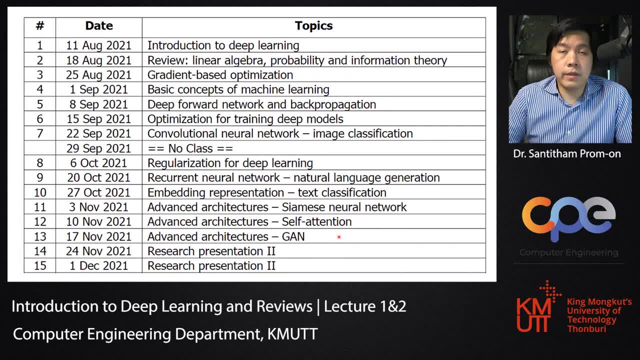 And GAN, to learn about GAN here in the advanced topics. Advanced topics can be changed if you want to learn about something else, but at least I will cover this And it can be reduced as well- hopefully not reduced. So yeah, about these three. 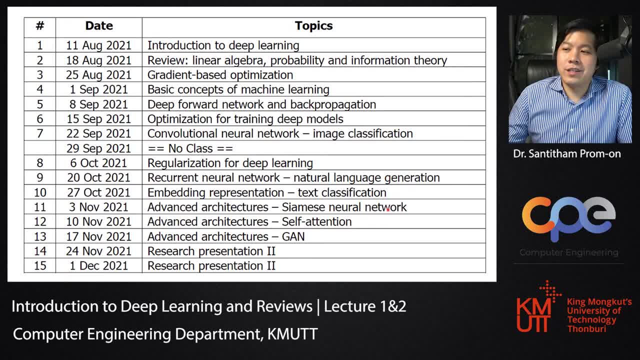 the advanced topics for this year. These are usually changed year by year. Last two years these are not there. So in the past year I covered something like autoencoder And I don't remember, But because we can talk about autoencoder, 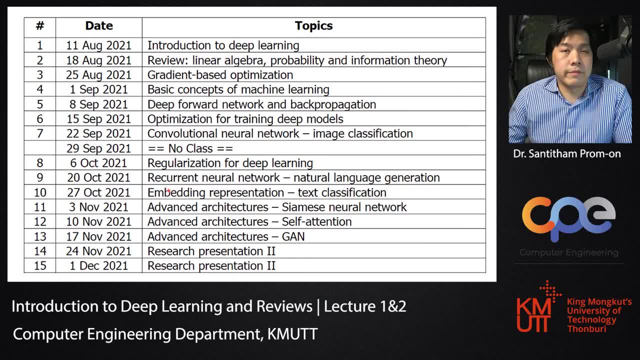 here as well in the text, in the embedding representation. So I kind of compress it a bit to cover something else for one-shot learning and self-attention and GAN, And then lastly the last two slots. here you see. 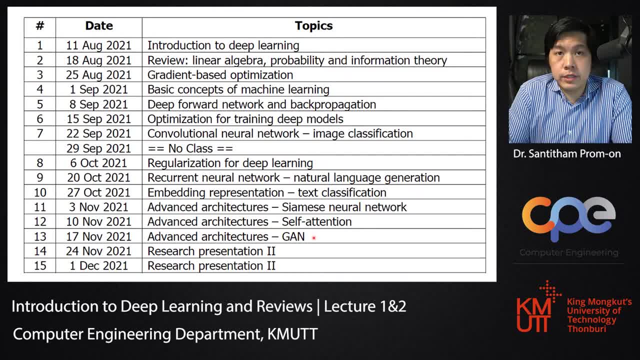 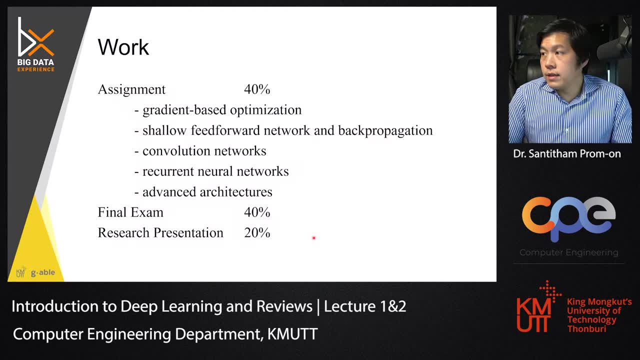 that we have the research presentations which you present- one paper to the class, Okay, And each of you have about 20 minutes or half an hour to do the presentations and present the work to the class. The score for this class comprises three parts. 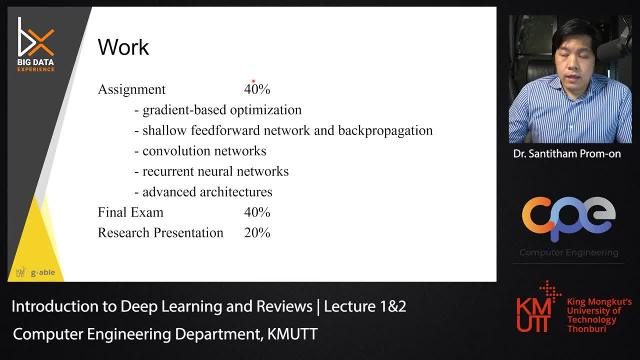 First is the assignment. In the assignment, you have to implement these five models. Although I said implements in the implementation, you need to also solve the equations. Because, for example, you want to perform gradient-based optimization, you need to solve the. 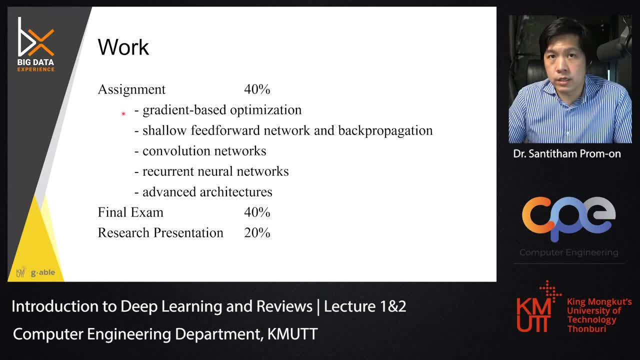 cost function, show the loss function and then take the derivative of the loss function to determine the gradient and then perform gradient descent. So there will be both mathematical formulations and the task itself in these assignments. There will be five assignments and in total it comprises of: 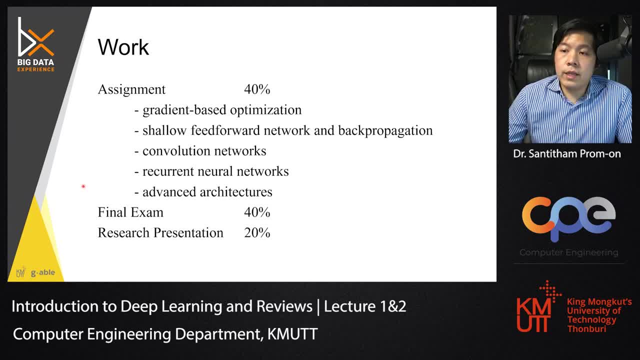 40% of the score here, Another 40% comes from final exam And the last one is the research presentation. Okay, So this is all of the work in this course. Do you have any questions about it first, Otherwise we will. 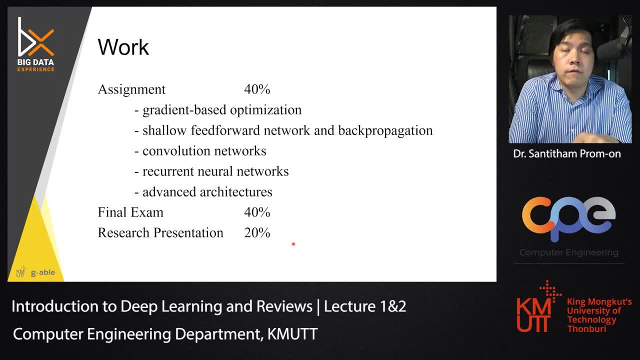 take a short break and then come back with the review of the mathematical concepts required for the class. Any questions During the class? you can chat in to ask questions. You can open the microphone to ask questions. I don't mind, Both are fine. 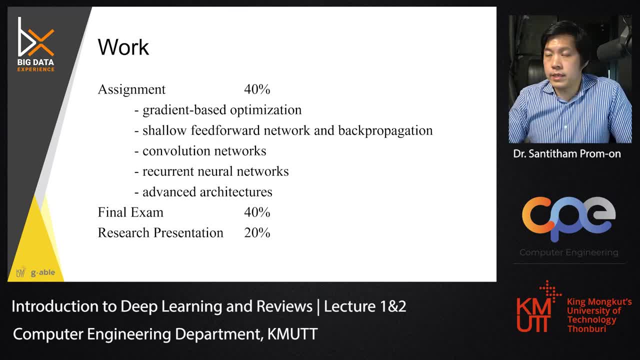 And we will start the class on 6 pm, Except if I have an emergency, like last time stuck in traffic. I came back like 7.30 something. So yeah, that's not practical for starting the class there, Right? 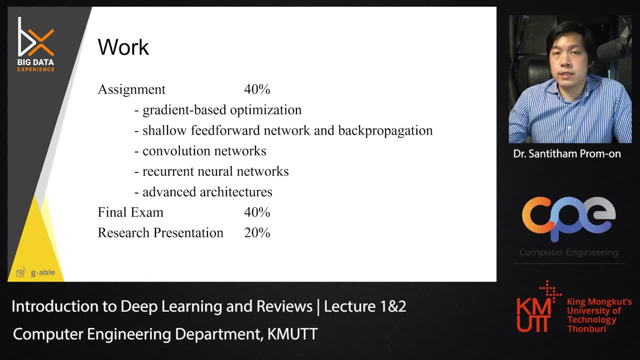 So if there are no questions for now, let's take a break and then we will start the review on 7 pm. Okay, If you have questions before, then, please put the questions into the chat box. Okay, Let's take. a break. 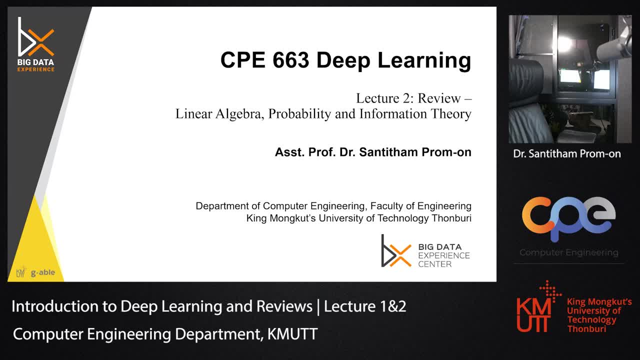 Online learning is mainly done on computers and electronics. You might think you're in a classroom, but at school. but instead of going to school, 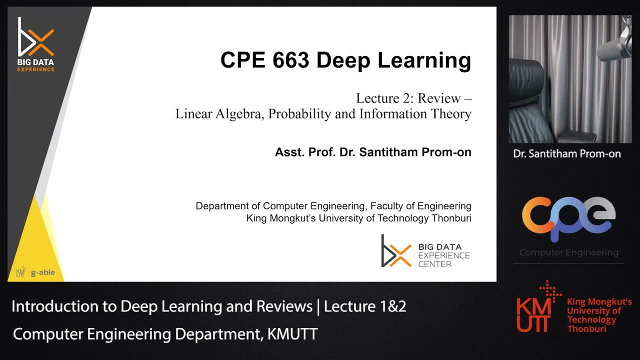 you will learn online on computer and called Google Meet in Microsoft. In fact, the questions are typically done by students and at school. it can be done by anyone and it can be done by anyone. Let's see if it works. I can't see. 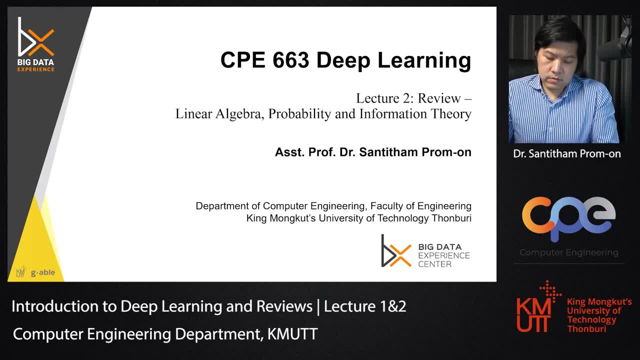 All right, welcome back. We are then going to proceed with the review of the mathematical concepts you require for this course. Okay, so I hope you are already here. All right, so What we will learn afterwards will be about linear algebra, probability theory and the information theory related to the course. 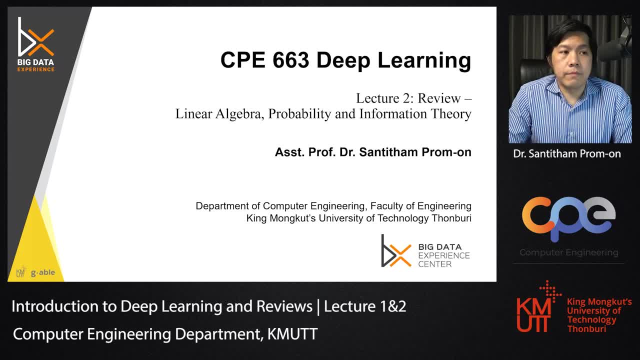 You can follow the code here, but I'm not going to particularly type them here so you can review the coding later on. I put it here in the slide as well, if you want to practice. afterward You can see what types of features that Python has toward addressing different types of problems here. 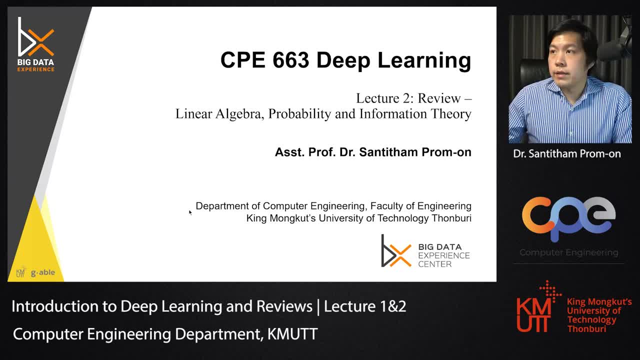 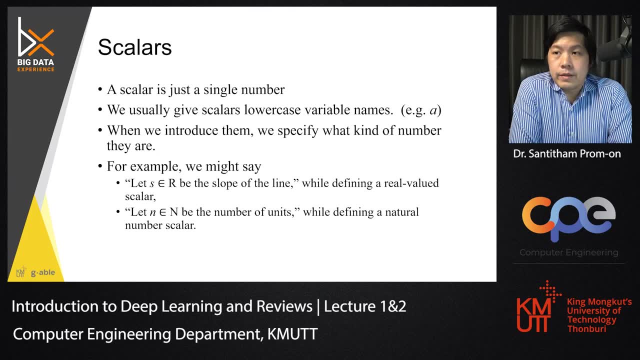 Okay, let's start with scalar. Okay, scalar value. When we talk about scalar value, we are referring to just a single number, Okay, Okay, Usually in the course, And in a lot of books, we usually use the lowercase variable to denote the name of the variable or the value related to the scalar values. 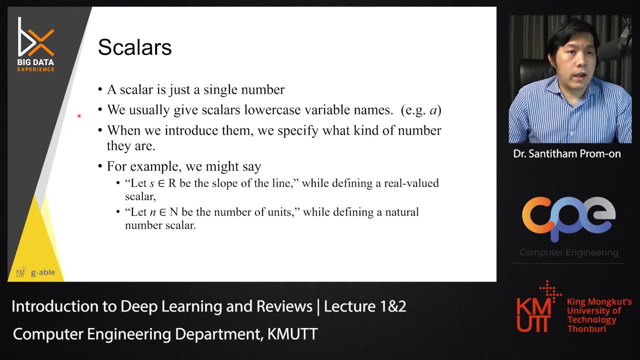 When we refer to scalar value, we usually define it as certain types of value, like it will be the real value or the natural number, depending on the set that it belongs to. Okay, once you combine the scalar value together in the form of the structure, you have vector and matrix. 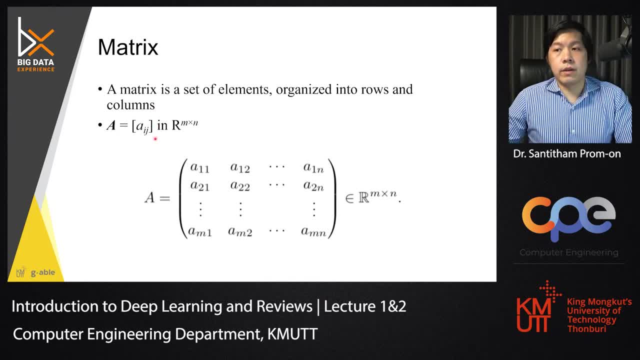 Okay, Metrics is a set of elements, that you organize them into row and column. Usually it is written as this: a equal aij in the square bracket. This belongs to the rm time n, which means that you have m row and column. 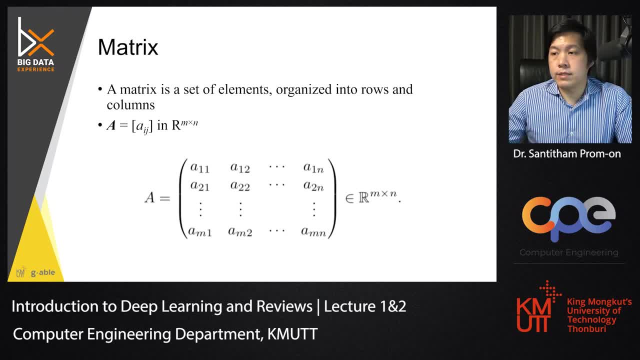 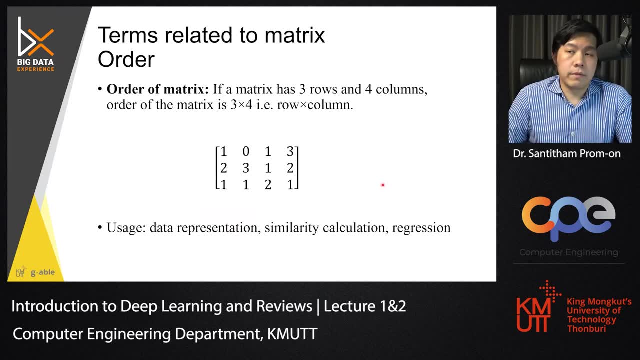 Okay, m, row n, column. That's why we have indexes like this. Okay, we call the matrix an order, We call an element of the matrix an order of the matrix If it refers to the number of row and columns of the matrix. right, we have the order of matrix three times four, which are the row times, columns, right. 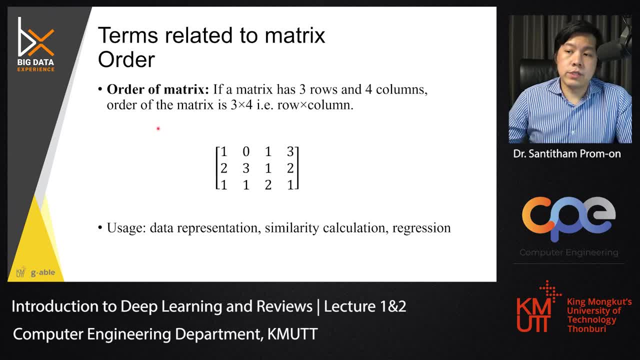 Three rows, four columns. right Order of matrix is used in referring to the data, the shape of the data. When you create a model, you have to be sure that the shapes are right. right, You use shape in Python. 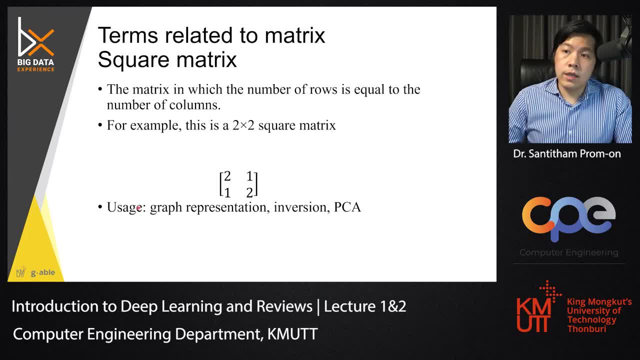 It is related to the order of the matrix. A square matrix is a matrix that has: We have the same value in both dimensions, in both row and column. We usually use square matrix in different places, like in graph representation, in the principal component analysis, in the matrix inversion, in the pseudo-inverse case. 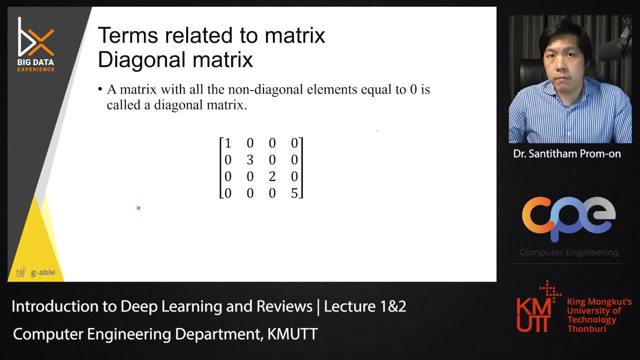 Okay, The diagonal matrix arises when you combine the values, something like an eigenvalue, or extract the eigenvalue from the characteristic equations, And then you encounter the diagonal And then you encounter the diagonal matrix that they are the matrix that have like the values in the diagonal line. 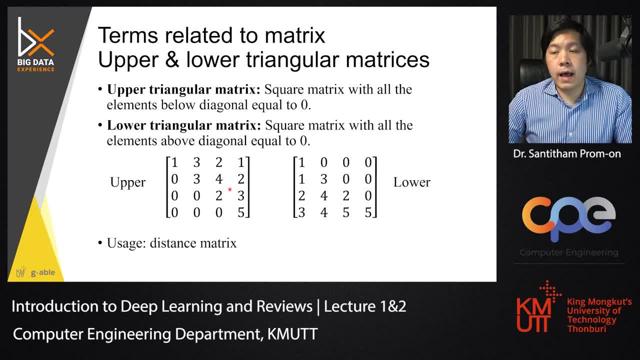 Sometimes you have a matrix that contains values, just parts of them, like in the upper triangular matrix. you have the matrix that have values only in the upper part or the lower part, here called the lower triangular matrix. These matrices are usually used in representing distance matrix from. 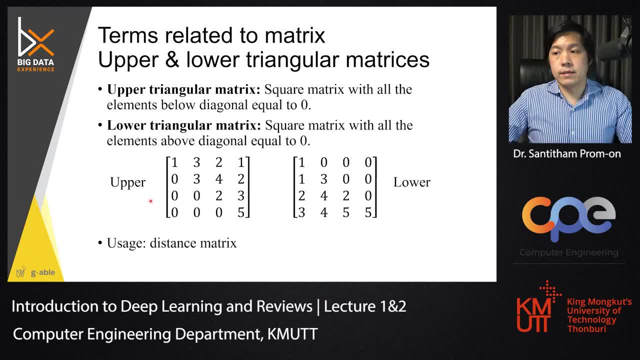 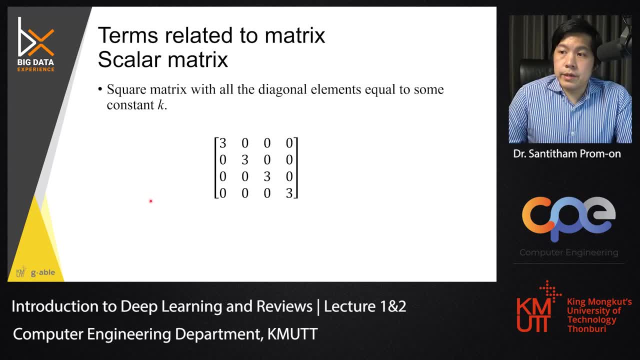 Come from calculating The difference or the similarities between data. Scalar matrix is a matrix that have a That is like combination of diagonal matrix times scalar values, You get the scalar matrix It is usually used to represent like a scale value in the matrix form. 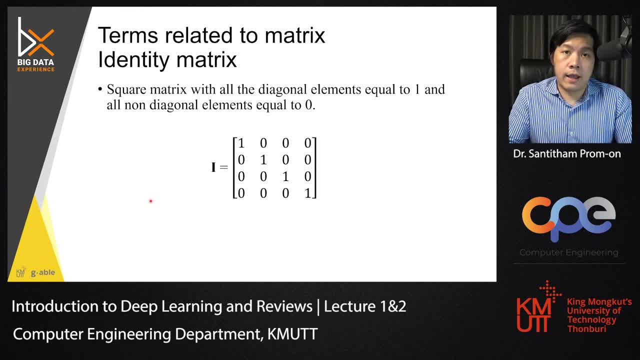 Okay, Identity matrix is a matrix I that have certain specific criteria, that you multiply it with anything, It results With the square matrix, it results in the same matrix, So it is Behave like one of one. So identity matrix has the one of one in the diagonal line and zero elsewhere. 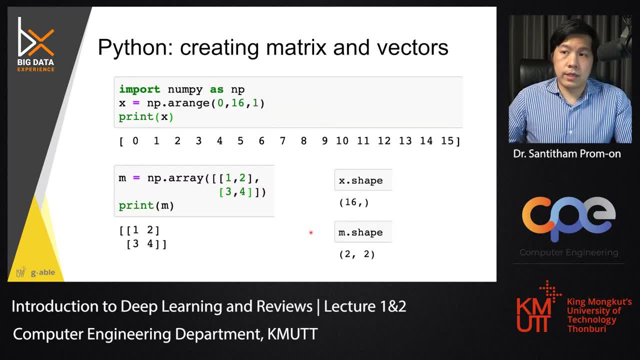 You can create matrix in Python and then play with them, like using NumPy. using Arrange, You can create a vector, one time number of dimension that you want to generate. And if you create a two-dimensional matrix here, something like this: 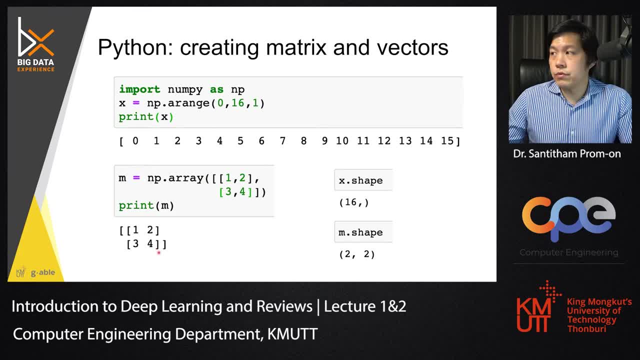 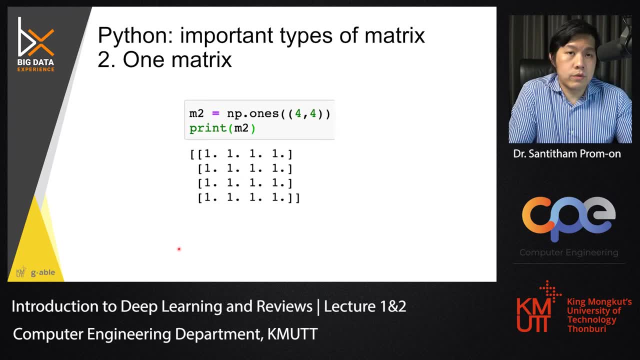 You can. You can create a list, nparray. you have the matrix in two dimensions and you can use a special type of function in NumPy, like zeros to create a zero matrix, one to create one matrix, and np to the identity to create identity matrix. 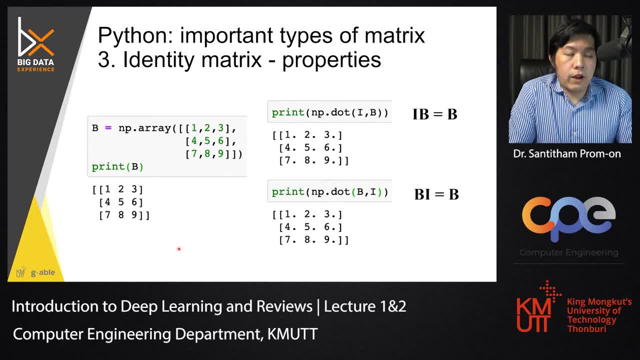 NumPy also has the function that you can multiply matrix together, like npmatmau and npdot. This allows you to multiply the matrix, the two-dimensional matrix, together. So if you have the matrix B, you can multiply it with I that we generated earlier and then get the results as the same matrix. 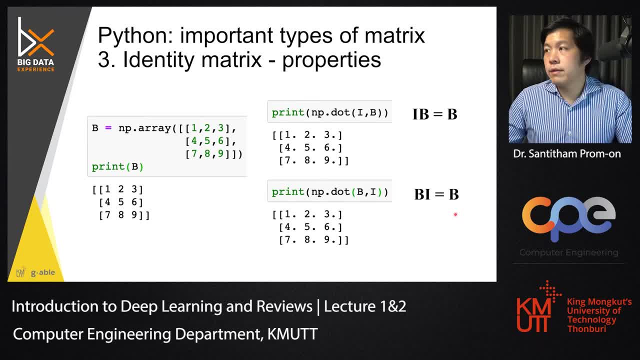 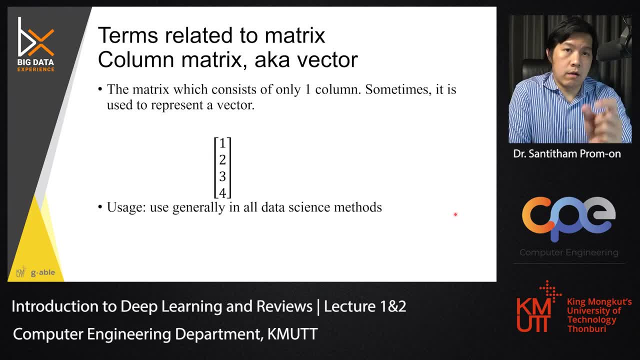 So I times B equals B and B times I equals B. Okay, when we have a matrix in one dimension, particularly in the column dimension, we usually call this a column matrix. A column matrix has been found in lots of applications because when you represent the Y values, 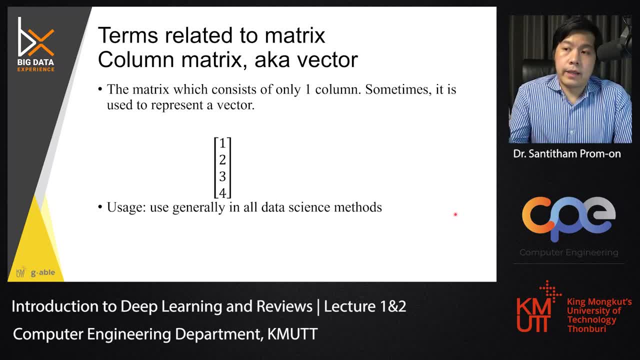 sometimes we call them a column vector as the set of values and it might be arranged as a column vector And this column vector would represent certain values that you want to associate with, And in lots of techniques, a column vector also represents different things, like we will see later on in SVD. 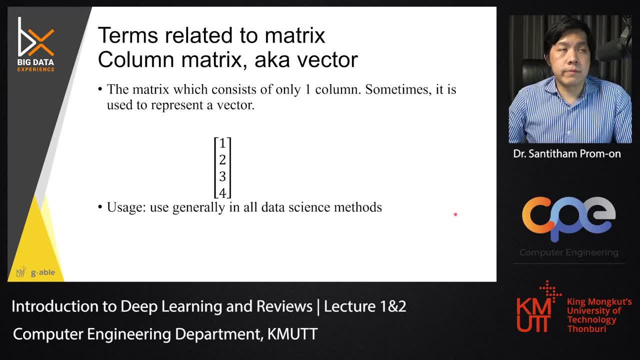 in the singular matrix. So in the singular matrix the column vector can be extracted out to get the eigenvectors of the reduction, of the reduction process, Okay, used in general data size concept, here the column vector. Now it comes to the vector. 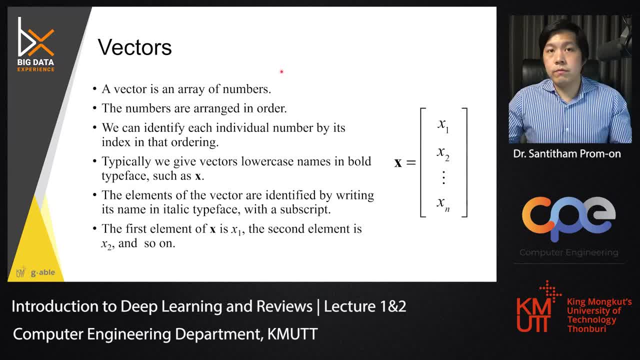 When we talk about vector, what is it? It's a scalar. it's just one value matrix. you have two dimensions. Vector is actually a matrix, an array of number, right? Just that. It's a random matrix. There's a range here. 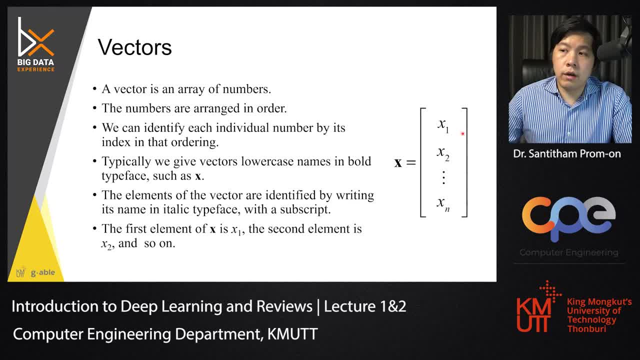 Think of it as a column vector. It is arranged in order. the orders are important, right? You can identify it by index. Usually, in mathematical terms, you would write it as a lowercase bold letters To denote the vector. okay, 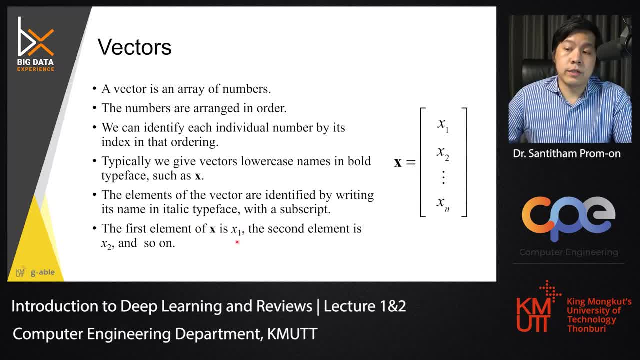 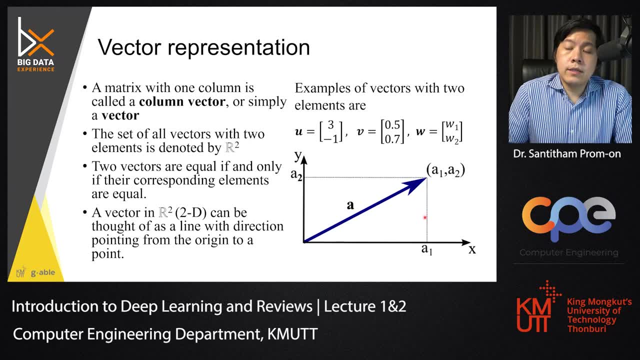 So elements in a vector will be denoted as a subscription here. like this is X1 and X2 and so on. like this, What is actually a vector vector or the column vector can be thought of as the in the geometric representation terms. it can. 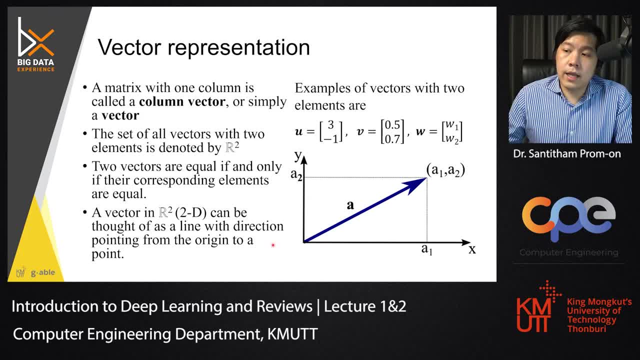 be thought of as an arrow here, like this, that point starting from the origin to the point of the value that you want to represent. this is the two dimension, uh, with a vector in in 2d, that representing the, the direction, or actually the direction and size, from origin to the point. 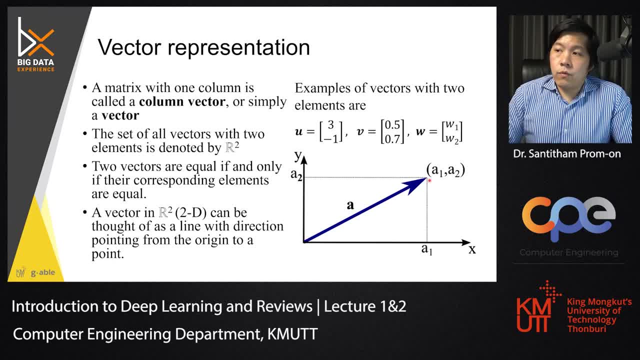 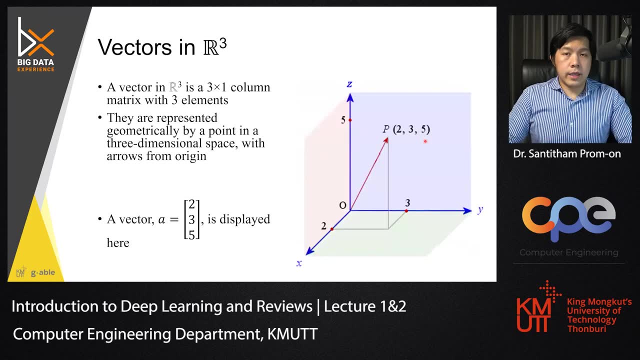 of interest. okay, when you have vector like in 2d, like this, you can write it as like the two elements, vector like this one, and they say these, these two are also two elements, like v and w. like this for the vector in r3, in the three dimension right, this is also just a. 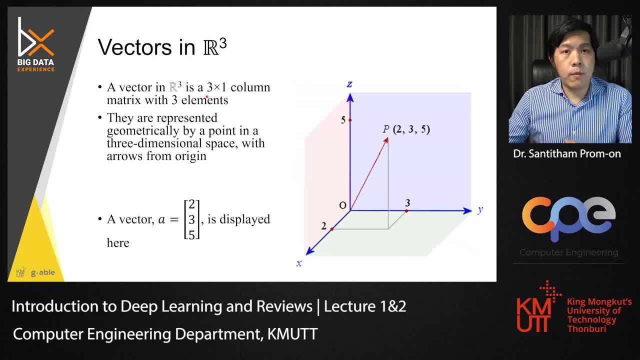 column matrix, just a column vector. this is three times one vector with three elements like two, 3, 5, it is the vector would point starting from origin to the point 2,, 3, 5,. or you can think of it differently and start from 1, 1, 1, and then point 2,, 3,, 4, 6, and it is still. 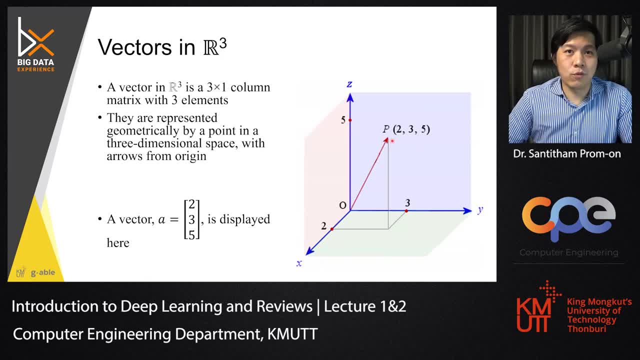 the same vector, But that is like high school math and I'm not going to go in that path. So at least here, yeah, the vector in R3 can be represented as like a set of values, like three values that you've written all together It represents the direction and the movement. 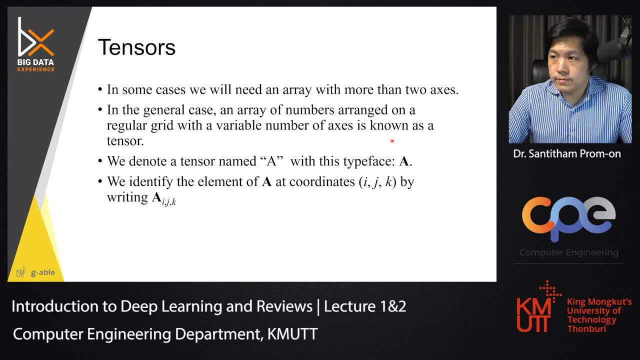 toward that direction. Now, in some case you need more than just one direction, You need more than just one vector, You need more than just one x. Sometimes you need an array that is more than two x's Right And, and then you need to like: suppose that we have just just a point right starting. 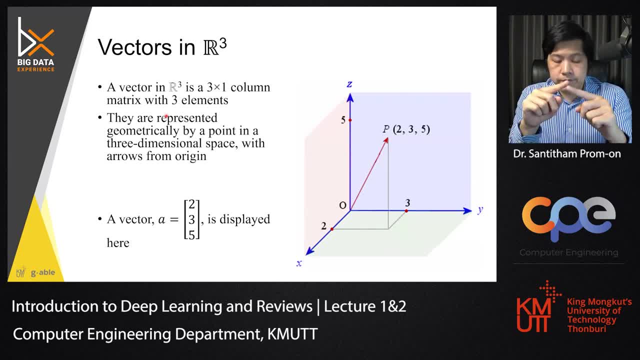 from a point. When you have a point, it's like zero dimension. When you draw a line, you got a one dimension data, Oh and a line. think about it as having a set of values, like in the vector. Once you have a line and then draw in two dimension, you can have an. 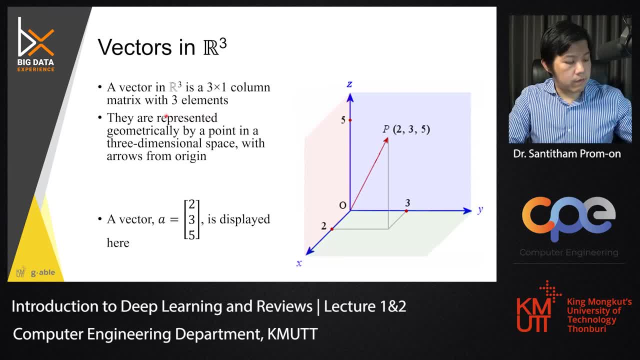 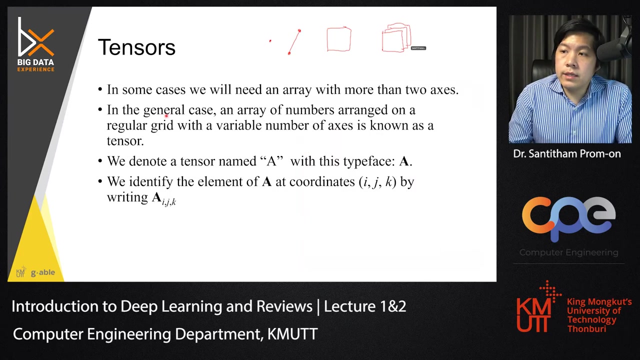 image, like an image in two dimension, Right from the point to a line, to an image. Now, how about if we need something more than this, like we need to have an image with a lot of layers? In that case, here it is denoted. 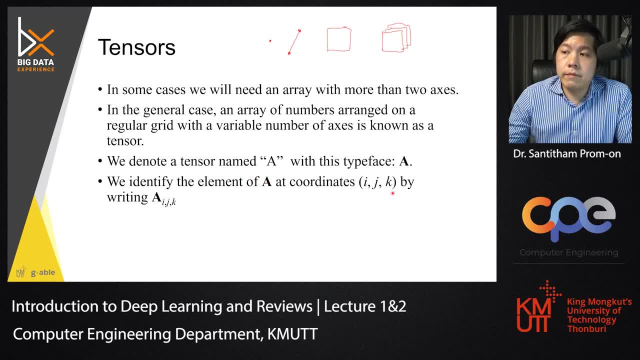 as a matrix like A, but you have an element K, Right, Yeah, That element K denote the layers that it has here. This in this course, but particularly for for this one. for mathematical sense it is referred to as tensors. That's why in 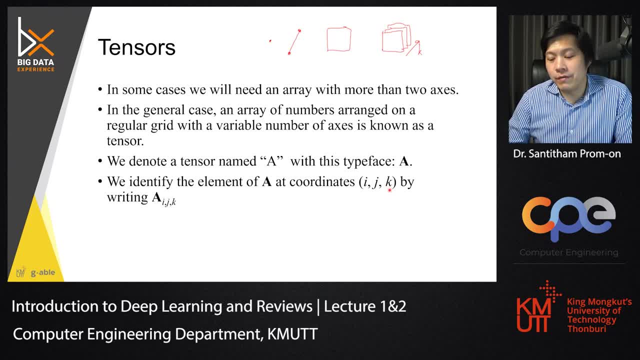 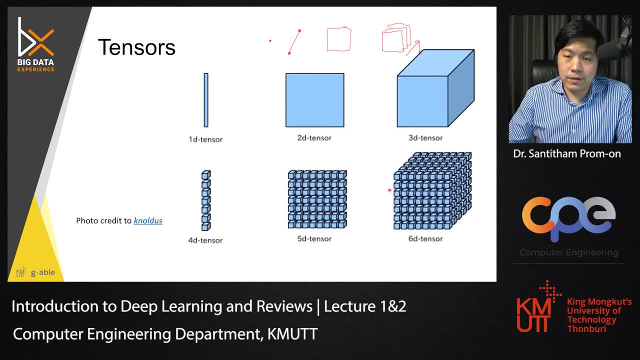 TensorFlow, the, the, the algorithm, well, the, the well widely used algorithm, TensorFlow. yeah, it is these tensors that they are talking about. So in tensors they are like 1D tensors or just a matrix in one dimension. 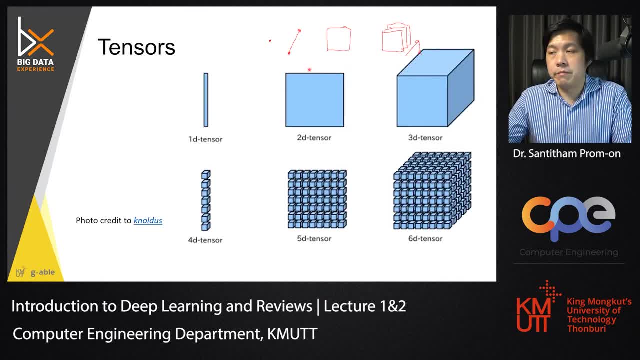 An, an, an array in one dimension: 2D tensor, an image 3D tensors. think about you have an image layer and have multiple layers. I J K 4D tensor is like you have multiple cube. 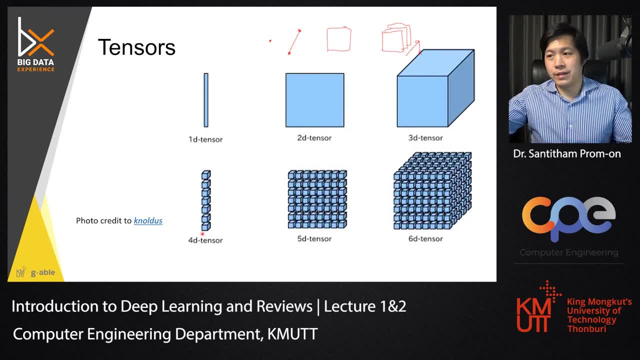 and 5D tensor multiple cube in diagonal in in the and then also in the what. what should I call this? Would be like something like a sub-spatial domain, like the spatial domain of the space Right. 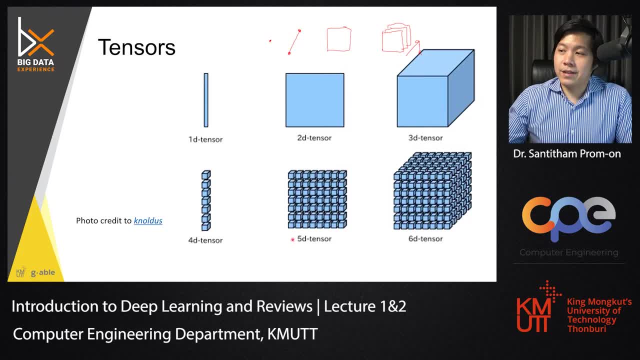 Spatial domain 6D sensor You want. you don't want to imagine something about it, but well, you can configure deep learning to have these type of architectures. And- and you can see that from the earlier image- convolutional neural network looks like 3D tensor, right, So that means TensorFlow would process. 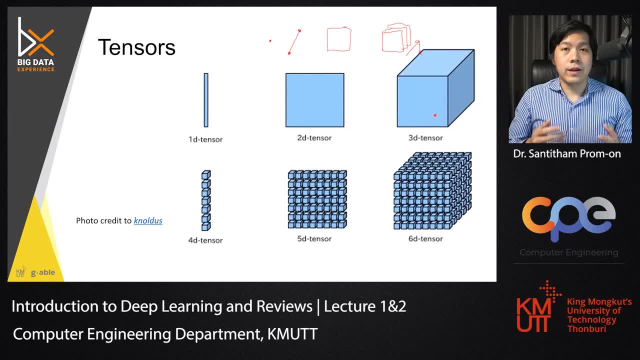 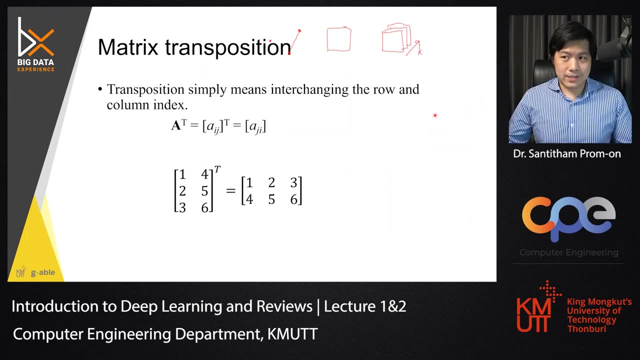 would perform computations very quickly based on the tensor processing matrix modification, But instead of just metrics would be tensor multiplication. Okay, now let's come back to to the real world that we talked about vector, then we let's extend it further to the metrics When you 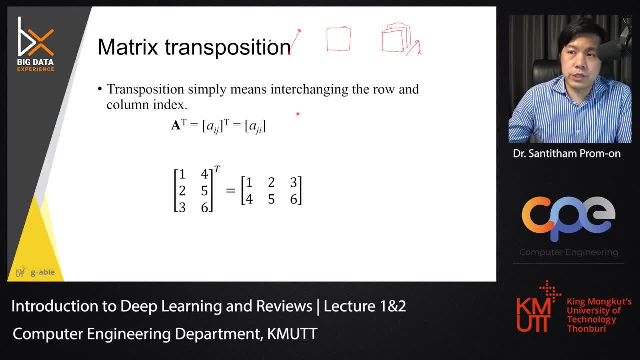 have metrics, you can perform operation like matrix transposition. this T metric transposition will inwards, the will move the index from I to J and to be to J to I and basically just flip row and columns. So the transpose of this matrix can move this matrix away from. 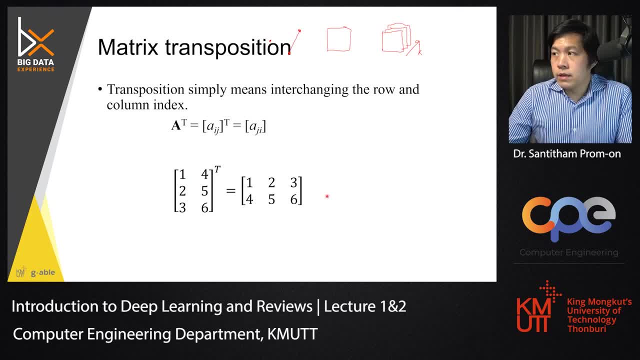 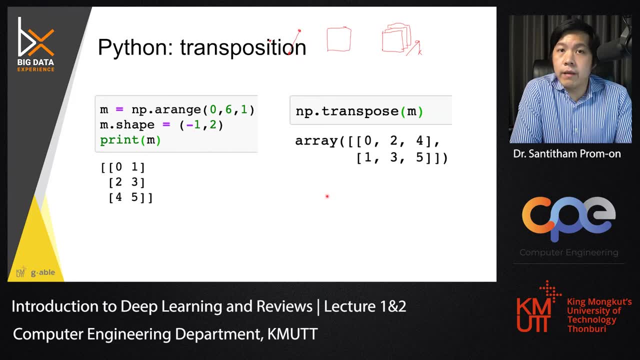 of this matrix equal to the right hand side here. okay, transposition can be done in python. just use transpose, nptranspose and then, or if you have data frame, just dot t, then you get the transposition of the data frame for the matrix. use nptranspose, it would transpose the matrix. okay, let's take a. 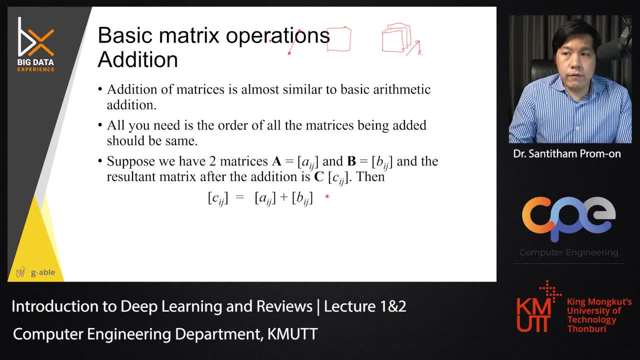 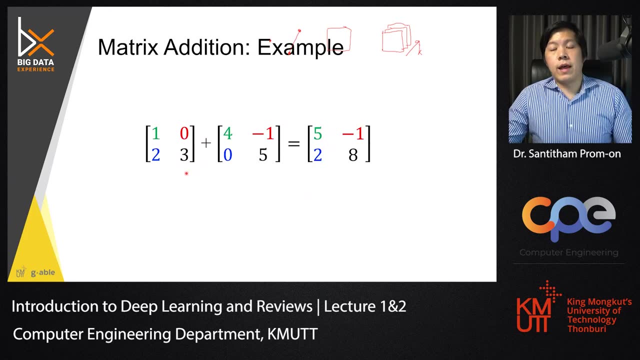 look at the matrix operation as a review. if you have the message matrix with the same orders, you can add them together to perform matrix addition. in the matrix addition you are actually adding the elements, performing element by element addition. so if you have a matrix like this, one, two, zero, three and four, zero minus one, five, adding them together you get five, two. 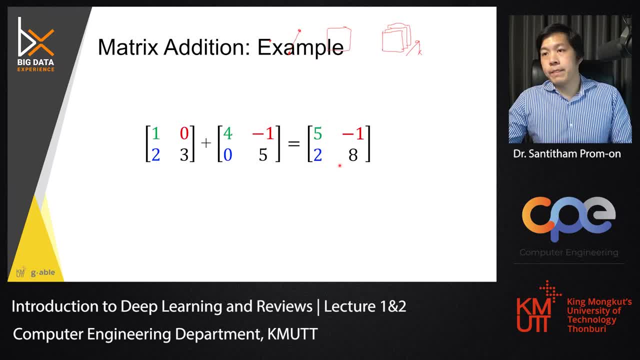 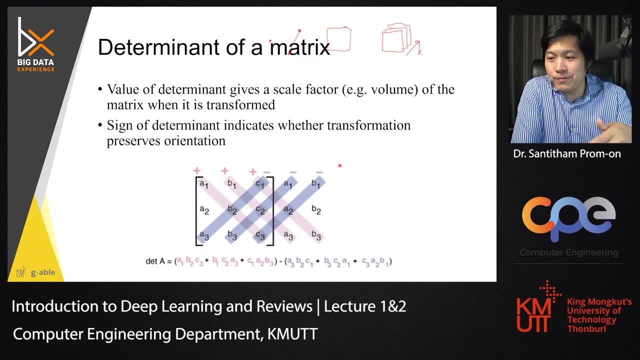 minus one, based on addition and eight. okay, that's the matrix. addition, the determinants: another topic, some metrics. i'm going pretty fast here to review the concepts that you have already known, but well, maybe let's skim through some of them, if you are. if you have questions, though, please, please ask. put it into the chat, okay. 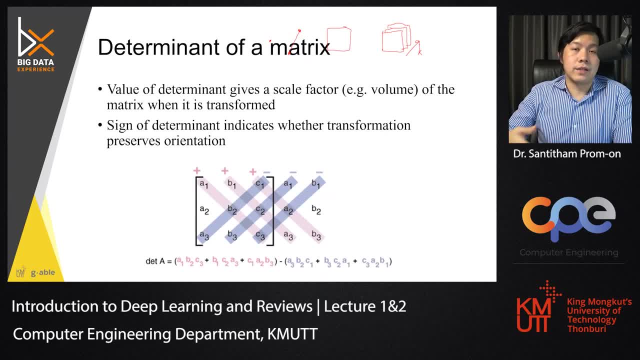 if you have questions after the class, like review the contents, and you have questions afterwards, post into the group, i will answer the question for you guys there. okay, determinant, what is determinant? determinant is best described as the volume of the matrix, like what you can think about determinant best when you evaluating the transformation matrix. 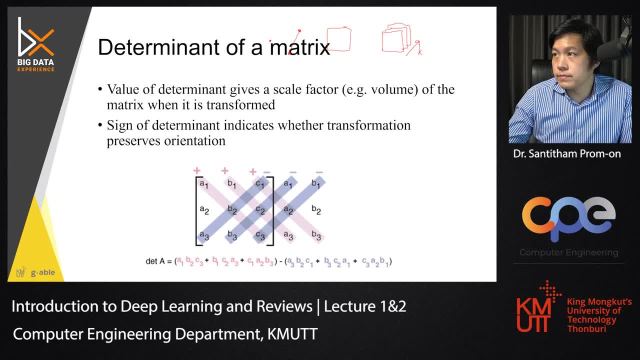 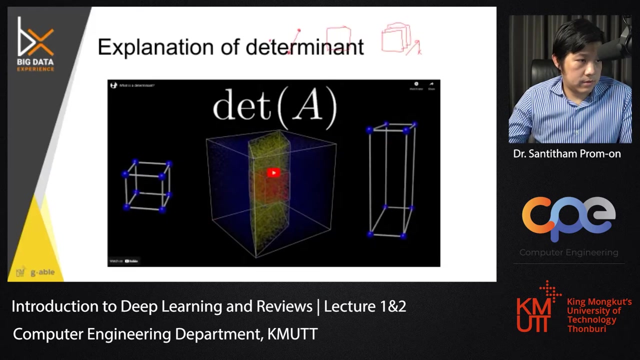 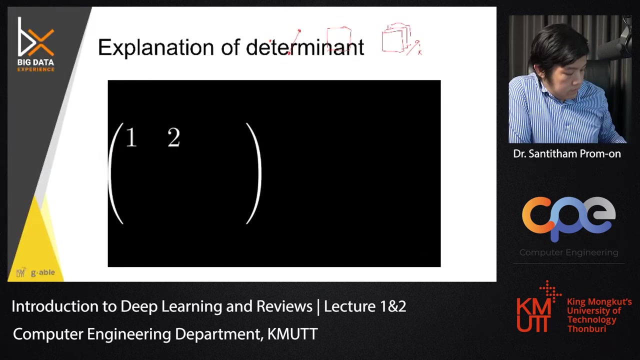 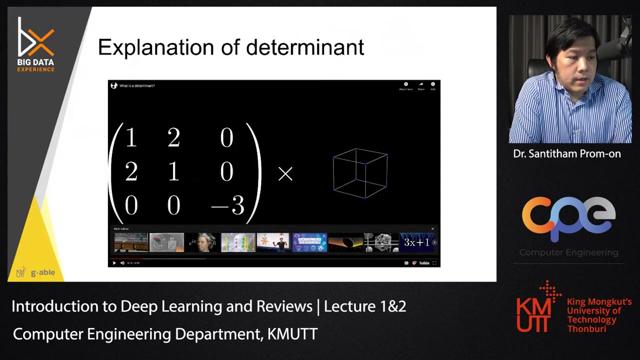 let's take a look as example here. okay, so calculation of determinant can be done by multiplying down, you have the positive terms, and multiply up, you have negative term. right, the what is determinant? let's take a look at this video. what is this? when we talk about, matrix, transformation is actually the 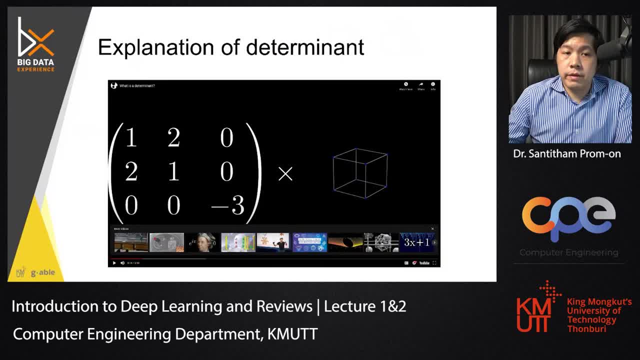 multiplication of the, the adjustment matrix, the transformation matrix, transformation matrix and and coordinate in in computer graphic. when you learn about the computer graphic you will see that you can kind of process the coordinate in the, in the, in in the graphical sense and the coordinate in a three-dimensional world into different perspective. right those? 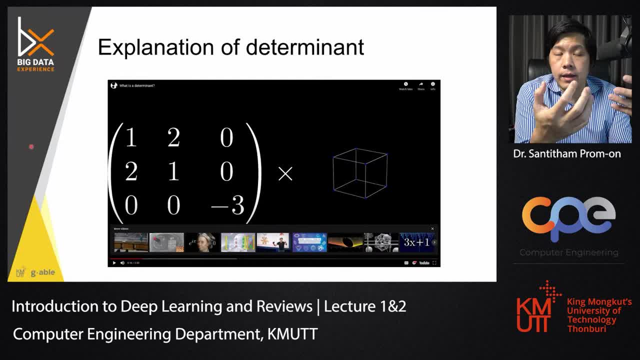 those projections can be done by multiplying the transformation matrix to the points and then those coordinates will be transformed according to the transformation matrix. okay, so if you, when we think about determinant, let's think about you- have this matrix that you are going to transform the point and the price is like a cube now, and what is that? what is determinant? 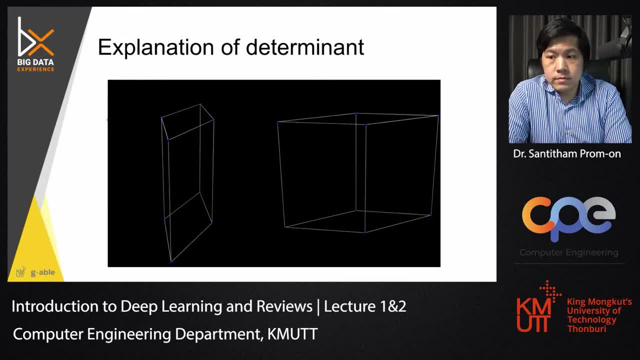 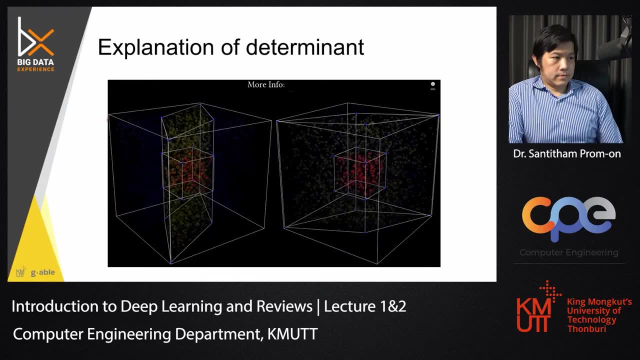 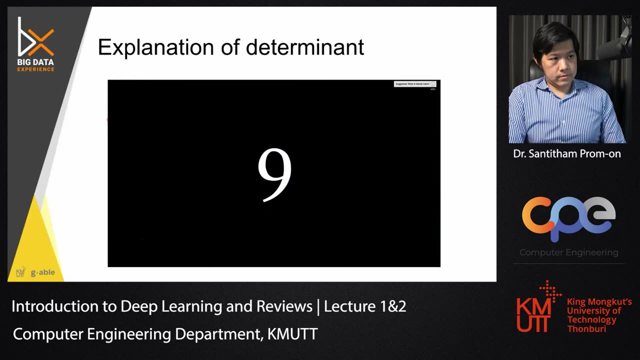 how much larger is this new transformed object? we could solve this problem with numerical integration by encapsulating both objects in a larger cube and performing monte carlo integration. after integration, we can say that the larger object is about 9 times bigger than the unit cube. 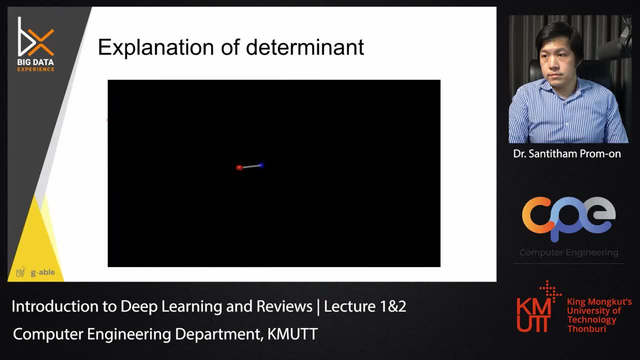 Now let's think of this problem a little differently. During matrix transformation, most vectors will stretch and rotate. However, there are certain vectors that only stretch and do not at all change direction. These vectors are known as eigenvectors, and the amounts by which they stretch are known as eigenvalues. 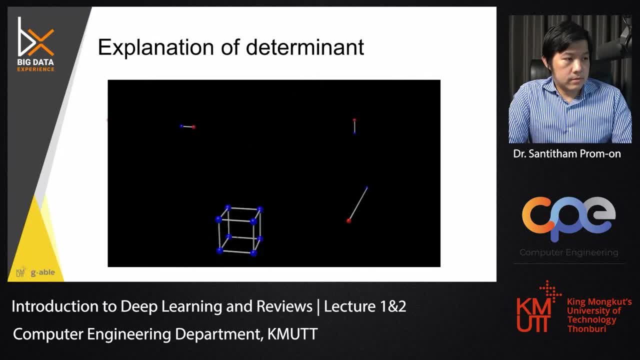 If we align the sides of our unit cube along these eigenvectors and perform a matrix transformation on each vertex in the cube, we'll find a rectangular prism that has not been skewed at all. This makes finding the ratio between the new transformed object and the original unit cube kind of trivial. 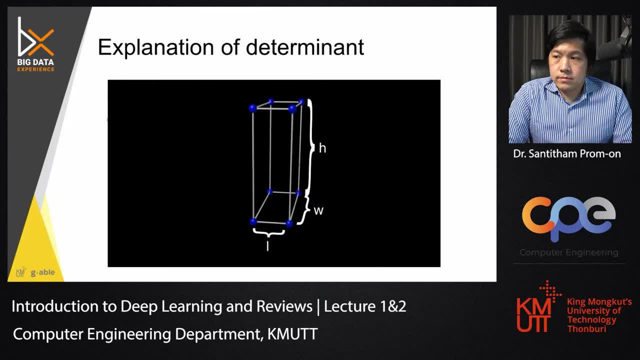 It's simply the length times width times, height of the new cuboid. Now, because we aligned the unit cube along eigenvectors and each side of the unit cube is of length 1,. after transformation, the new length, width and height are all eigenvectors. 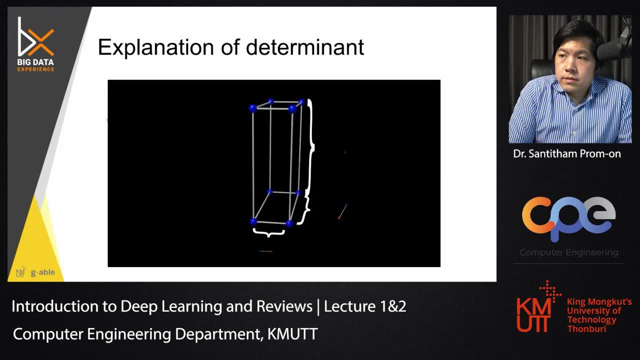 So how much bigger is the object after transformation? Well, it's simply a product of all the eigenvalues, which in this case is exactly 9.. Here I suppose, it makes sense that any object's volume will increase by the amount of stretching in each dimension. 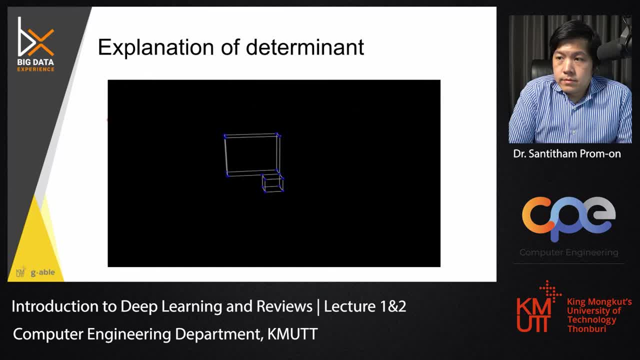 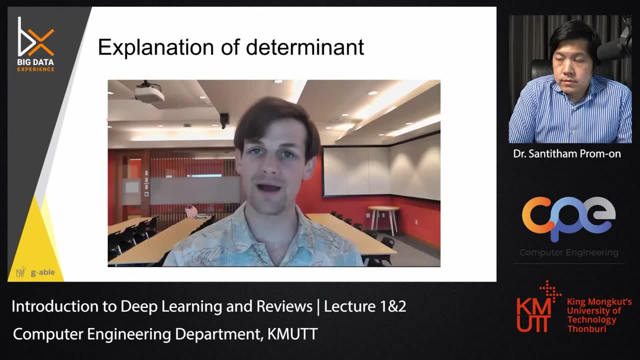 which is exactly what we said before. The new volume is a product of the eigenvalue. Now, at this point you might be thinking that we're pretty clever, but mathematicians have at least one more trick up their sleeve: Determinants. 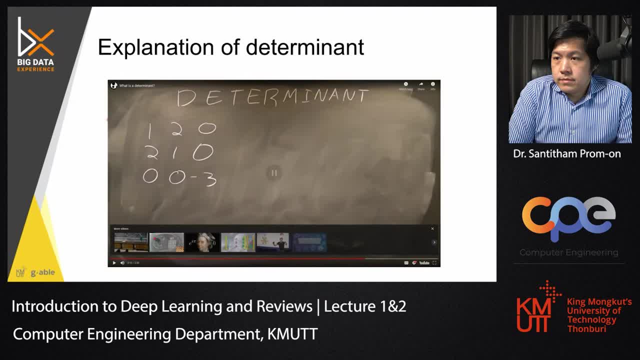 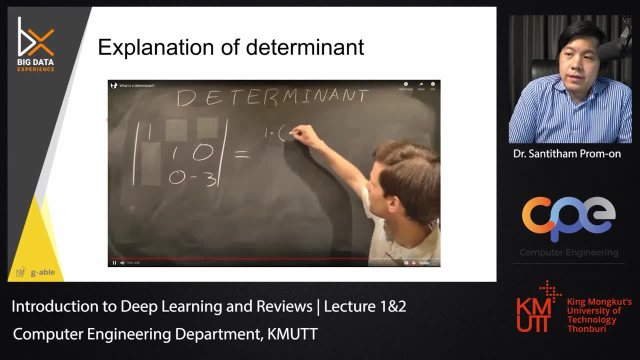 So let's do it. Let's find the determinant of our transformation Right. the determinants of this matrix would be: It would be 1 times 1 times negative, 3 minus 0 times 0, subtracting 2 times 2 times negative, 3 minus 0 times 0,. 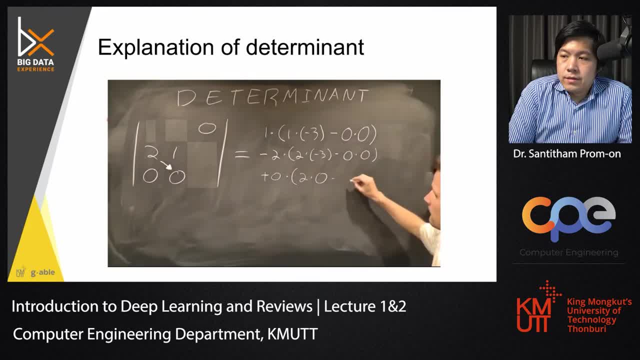 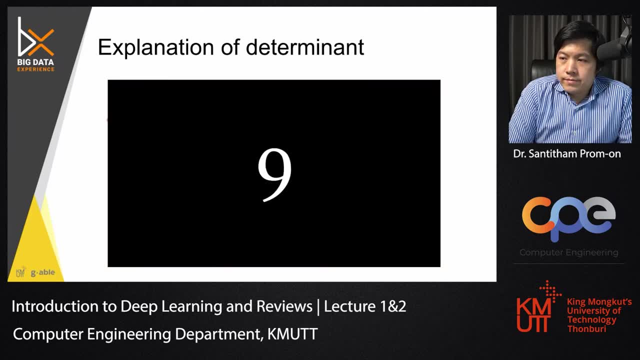 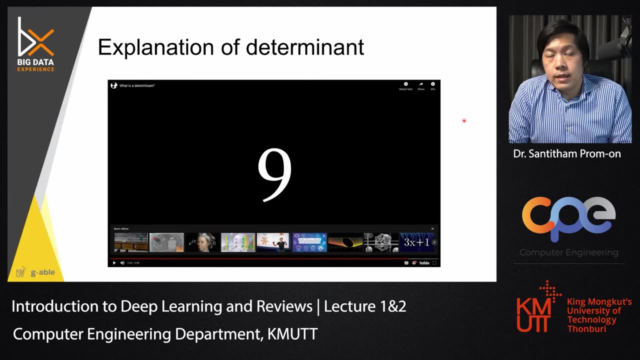 plus 0 times 2 times 0 minus 1 times 0, which is equal to negative 3 plus 12, or exactly 9.. That's it, So you can think of determinant as the modifier, as the factor of the matrix. 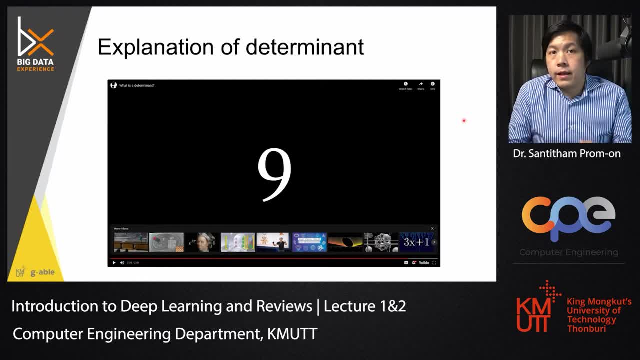 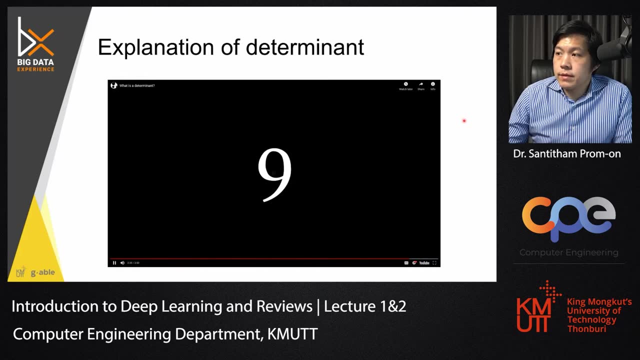 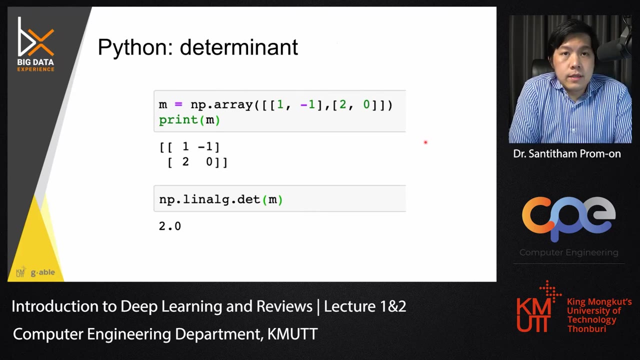 that when you transform the points in the cube it would kind of modify the volume of the cube to the amount of the determinant Right And you can do the determinant calculation by the method mathematical method. in Python You can use the nplinearalgebradet to find determinant. 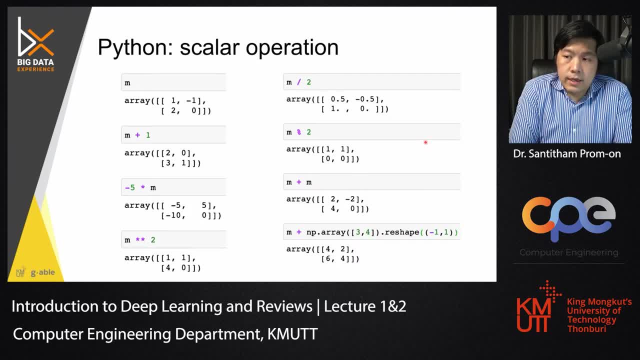 Then in Python you can also perform all the scalar operations to add time and do other things. What happens underlying is it was broadcasting, so Python would perform broadcasting of the 1 times 1 vector of the 1 times 1 matrix. 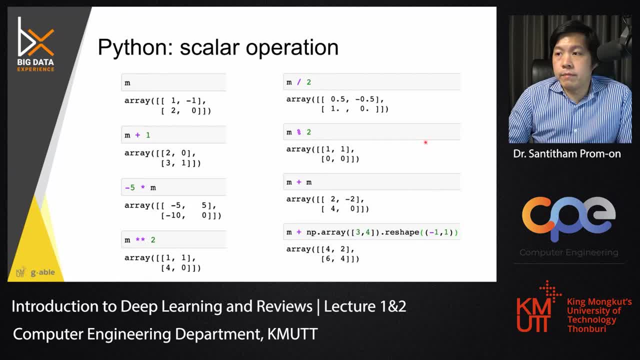 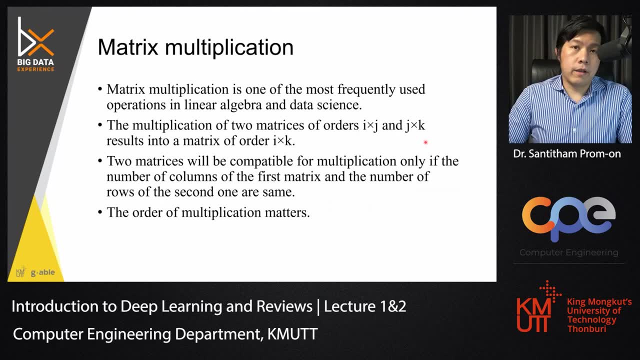 to increase it into the size of the m matrix. That is for scalar operation. Matrix can be multiplied together, not elements by elements, but in terms of matrix multiplication. In matrix multiplication you are actually projecting the one, the row matrix, with the column matrix. 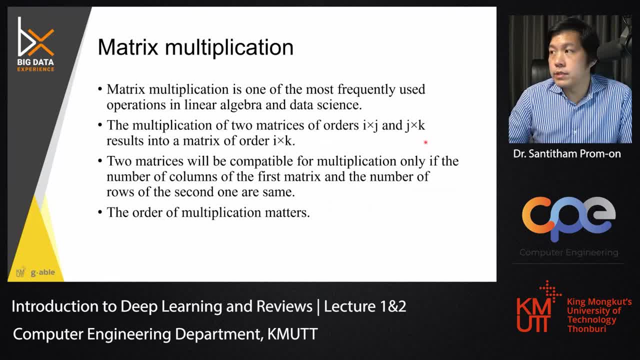 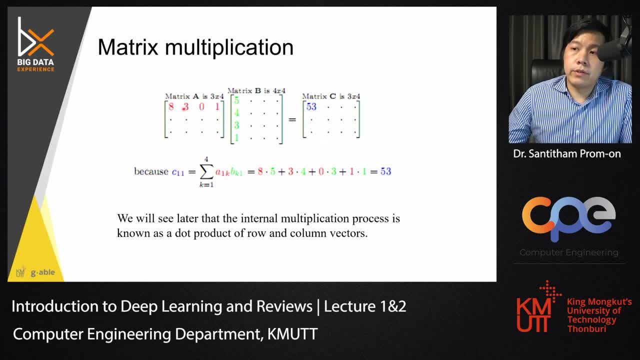 Dot them together to get the results. So you have learned this in, I think, high school and afterwards. So when you multiply the matrix, you have to multiply row with the column. This multiplication is actually the dot product between the row vector and column vector. 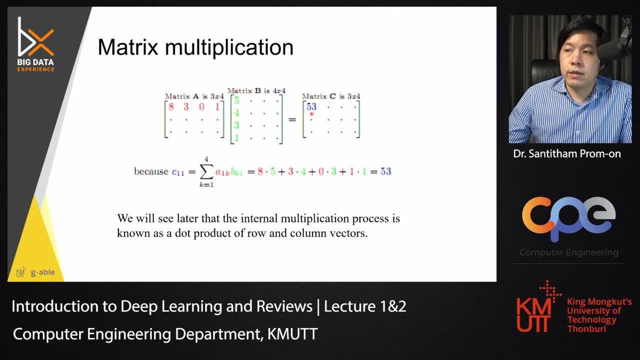 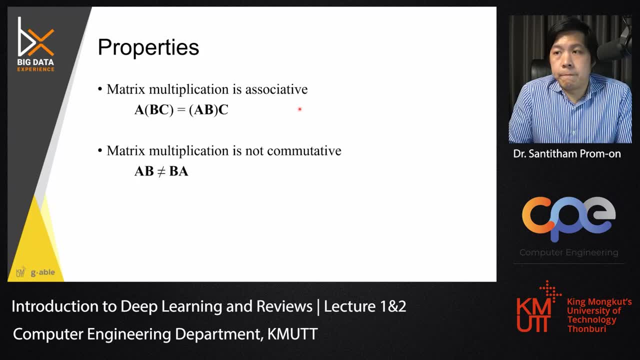 Multiplying each element and then sum them all and then you get the value at that element. Matrix multiplication has certain properties. that it is. it is associative but not commutative. You cannot switch sides, but you can group them, multiply them in order according to what you want. 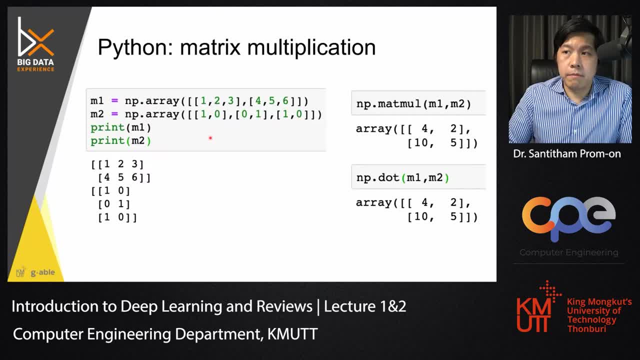 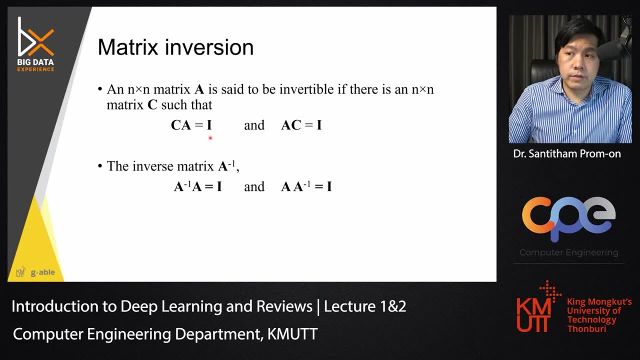 In Python you can use npdot or npmatmult to perform matrix multiplication. They are both fine. Lastly, for the matrix: matrix inversion, Matrix inversion, because you cannot kind of putting matrix in division- It's nonsense, right, Putting matrix in division there. 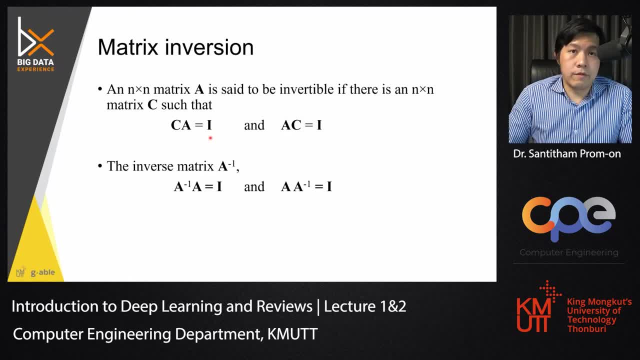 But you can perform inversion of the matrix by what is inverse matrix. right, We can say matrix A is invertible if it has matrix C, that when you multiply C with A you get I, or A with C you get I. 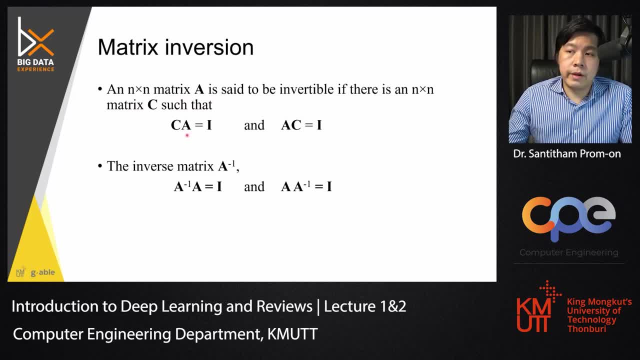 That means you can inverse the matrix A. if you multiply matrix A with the A inverse, Then you get I or A to the A inverse matrix, And you get I. That means that inverse matrix would, when you multiply it or project it to A. 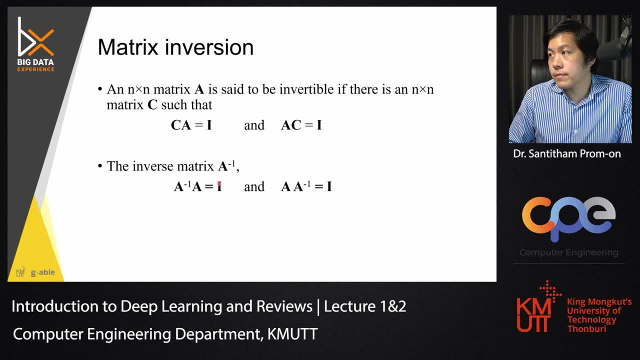 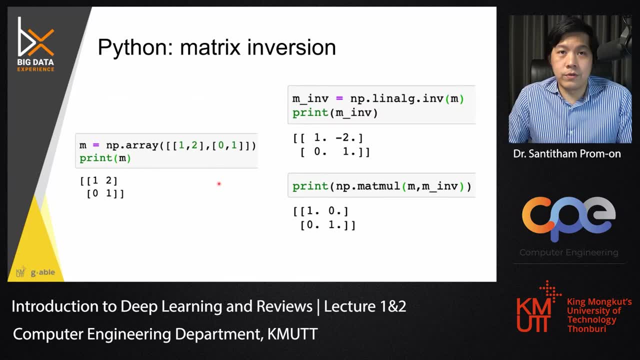 then you get- I So finding inversion in mathematical terms. I will leave that to your previous professors that teach you about the matrix inversions. There are quite a number of methods to do so. In calculation you can use Python to perform inversion. 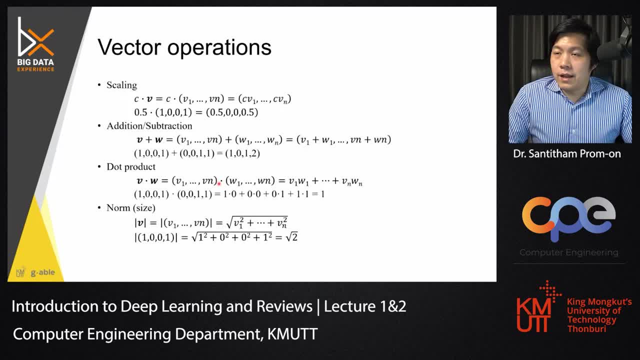 So I will use Python to perform inversion here. Okay, so, in summary, there are certain operations that you can perform on the vectors, like scaling, multiplying with the scalar, addition and subtraction, which will perform elements, while addition and subtraction the dot product. 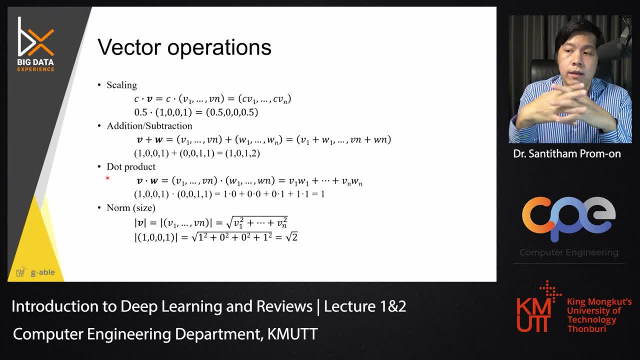 which will calculate the projection or the dot calculation between two vectors, and the norm which is calculating the size, the size of the vector. This is the L2 norm. The L2 norm is referred to as the like. you get the element square. 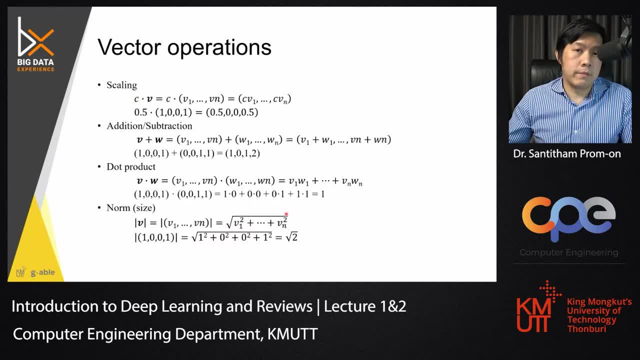 and then put them into the square root here. This is L2.. Later on you will see other L as well: L1 norm and L2 norm, the, let's say, the size of the vector in different criteria. Okay now, how do we use metrics? 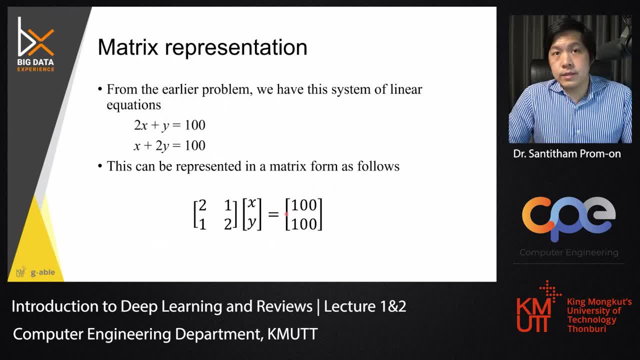 You can use metrics to calculate the size of the vector. You can use metrics to represent data. You can also use metrics to represent the association in equations. If you have a system of equations like this, that it explains the association between X and Y. 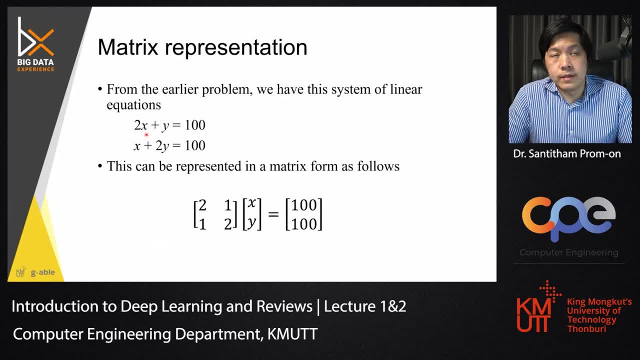 like you might have this from the data that you have input. you have parameters that you want to estimate. These are X and Y- And you have input data as 2 and 1, pairing with 100.. And 1 and 2 also pairing with 100. 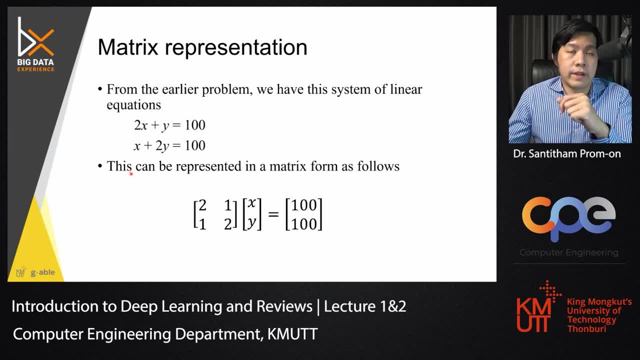 And then you are trying to solve for the value of X and Y. This is the system of linear equation. Solving system of linear equation would yield different results depending on the order of the equations that you have or the order of the coefficient metrics that you have. 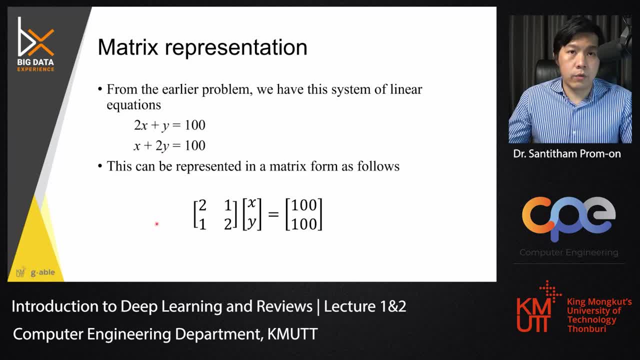 You can represent this system of linear equation as this metrics form: Like multiplying 2, 1 to X Y, you get 2X plus Y equal 100. And down here is like X plus 2Y equal 100. Now you can have different types of solutions. 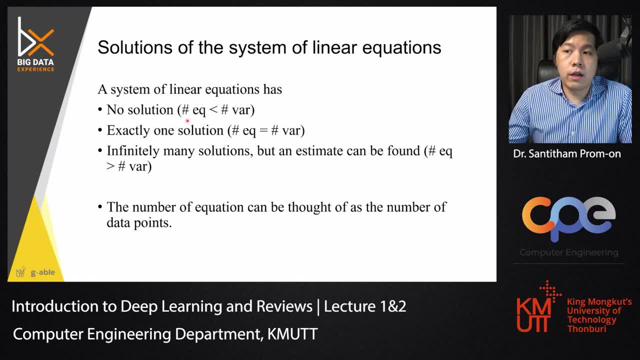 You can have the solution that there is no solution at all if your equation is less than variable. So, seeing this, remember this. And then if you build your model and then you have very little of samples but a lot of variables, you can expect to get into trouble here. 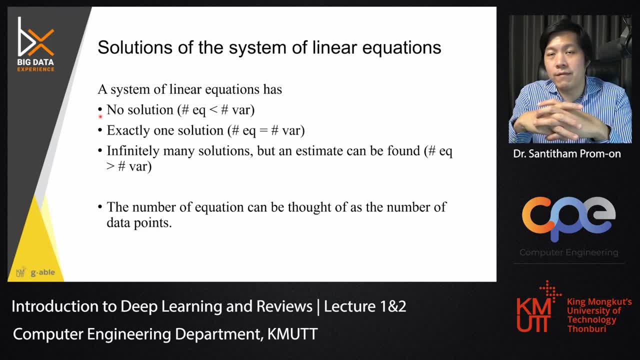 So no solution if you have less data, less equation than the unknown variables. You have exactly one solution if they are equal to one another And in a lot of cases that you work with data, you have many solutions if the equation is more than one. 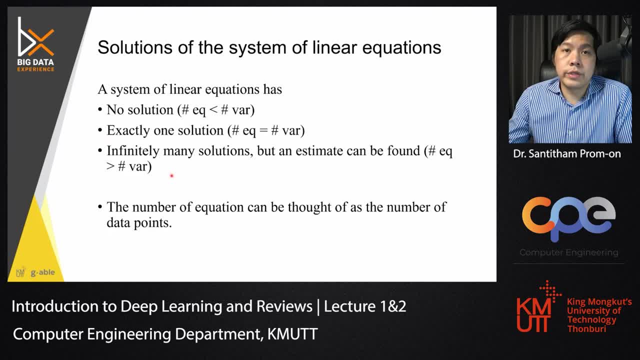 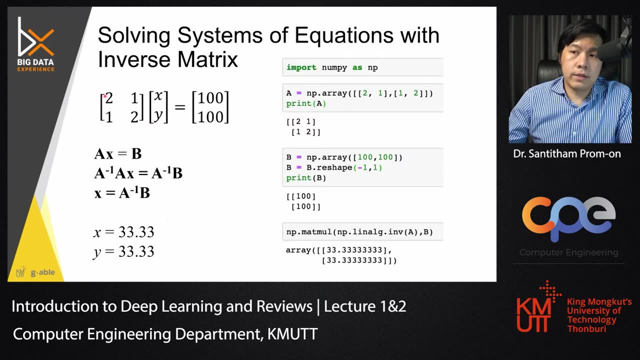 So you need to estimate the solution instead of having an exact solution. In the case that you have the number of equation equal variable, you can solve this metrics by finding inverse. By representing this as AX equal B, you can multiply the inverse of A. 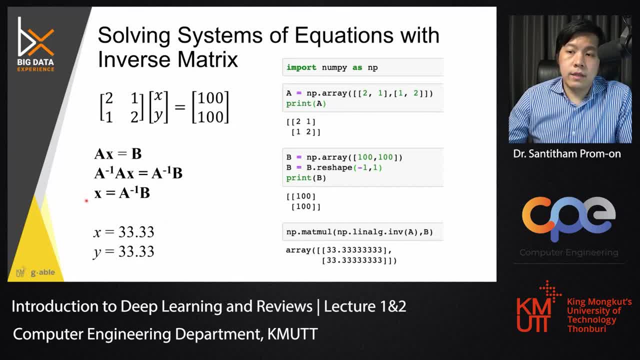 to this metrics, And then you get X, equal, A, inverse and B. This is what you learned back then. So here I created metrics A, and then here is the metrics B, And then multiply B with inverse of A and then get results of 33 and 33.. 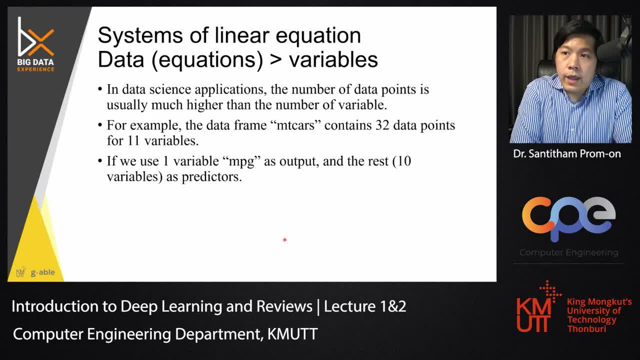 Simple enough If you have equations of data more than variables. in lots of data science applications, this is the case that you have often encountered. Okay, For example, in a data set empty cars, there are 32 data points and 11 variables. 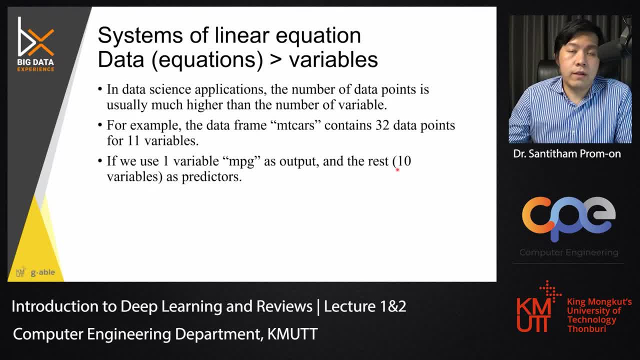 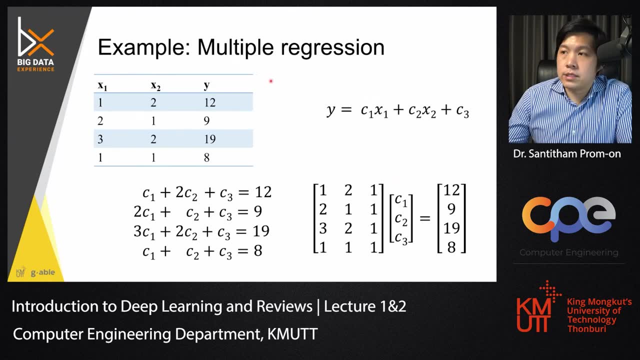 If you use one variable as output, you still have 10 variables as predictors, And then you still need to find 10 parameters, 10 coefficients associating with each predictors. Okay, Let's take a look at this simple example. This is a multiple regression example. 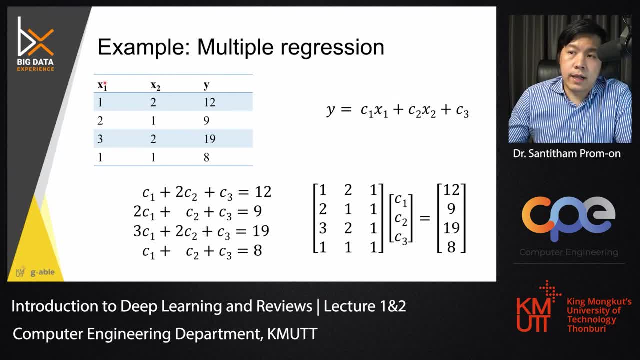 Suppose we have the data like this: X1, X2. And Y, And we want to fit them into this equation: Y equals C1, X1 plus C2, X2 plus C3.. Okay, We got X1 and X2,. 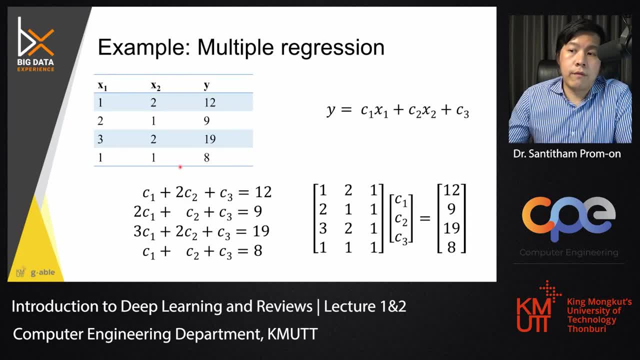 and the coefficient, three unknowns, And we have four equations. If we put the data into equations, we have this set of equations. This is the system of linear equations. But well, you have more equations than the unknown. It doesn't mean that you cannot find the answer. 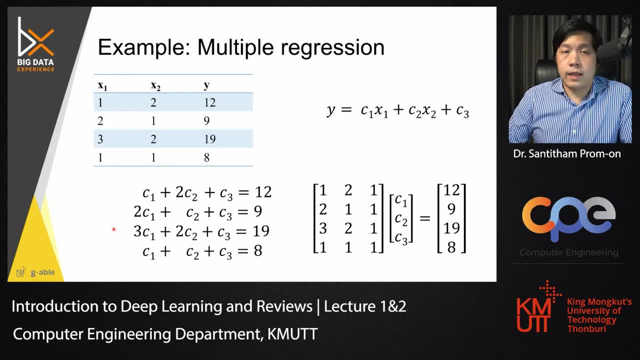 but you need a way to estimate- estimate for the best solutions of C1,, C2, and C3 out of this. Okay, There are many ways to do the job. The one that I will just show you here is the method called pseudo. 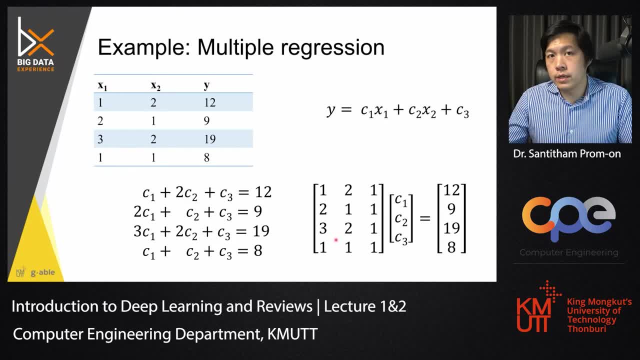 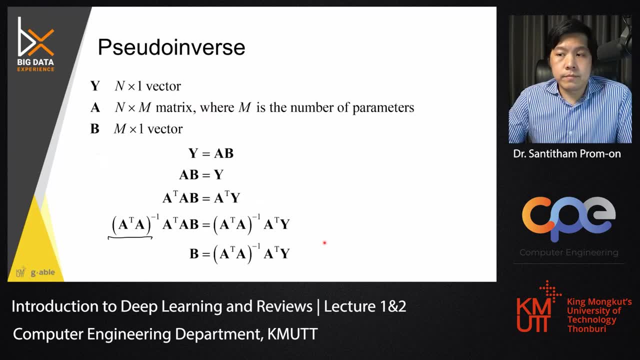 because you cannot inverse, you cannot multiply it with inverse. There are no inverse here, But you can find the pseudo inverse, Pseudo inverse. take, take into consideration of the rank or the order of the matrix, That is, A is N times M. 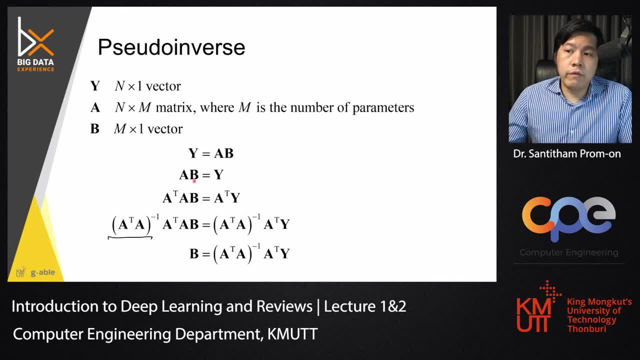 which is not a square matrix. So we have something like AB equals Y, Y is like output and A is a coefficient And B is something that you want to know. You can find B by first, because it's not a square matrix. 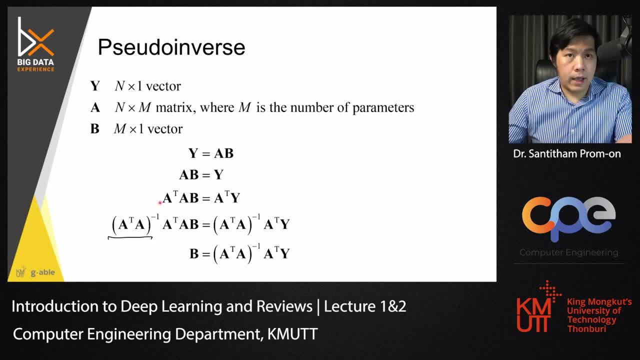 we need to make it square How We can multiply both sides with A transpose. Once you multiply this with A transpose, this with A transpose, then the A transpose times A will be a square matrix, right? If you wonder if that is the case, 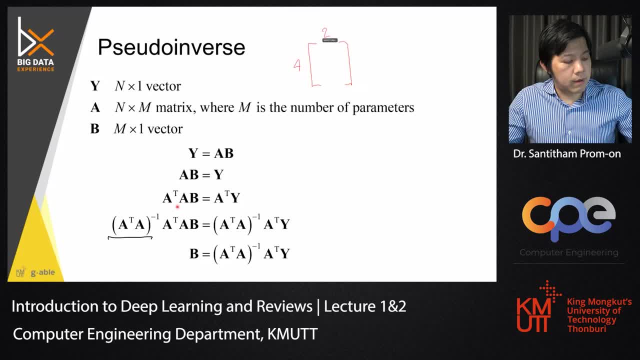 just imagine this like: suppose you have 3, 4 times 2, and then you multiply it with 2 times 4, the resulting matrix will be the dimension of 4 times 4, right, It will become a square matrix. 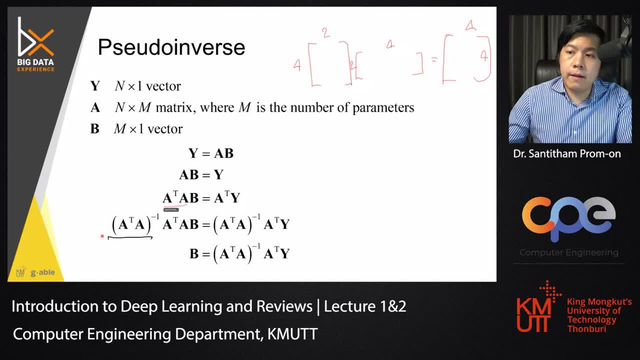 And once this becomes a square matrix, you can multiply the inverse of it to the whole bunch, And this would cancel each order out to become I. And here is the formula that you have to do In order to solve these equations. Okay, 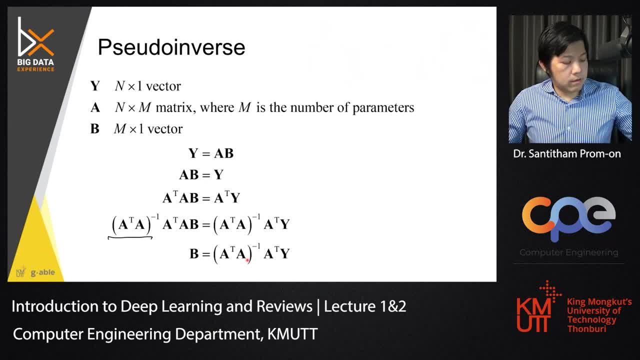 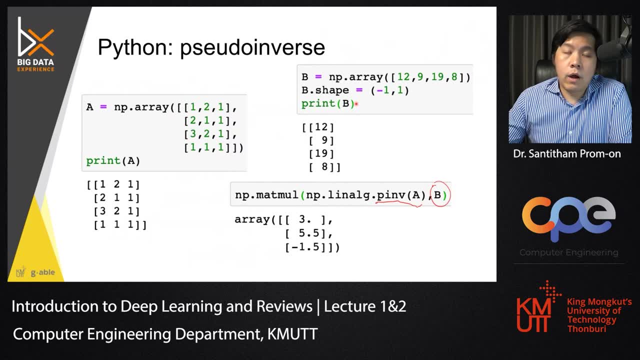 So here let's implement it Here. I have the array of A and B and I want to find the X and C1, C2, and C3.. How do I do? How do I work on that? What I did here is to use the P inverse. 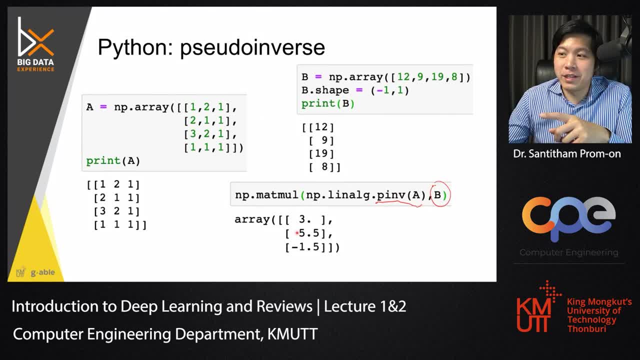 P inverse is a pseudo-inverse, So the inverse of A multiplied by B and you get 3, 5.5, minus 1.5.. You may call me shit, because well, P inverse is like 5D, pseudo-inverse for you guys. 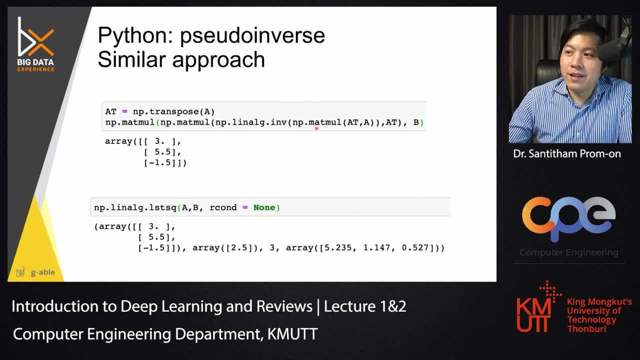 So here is the full form. This is the multiplication of A transpose and A right, And then matrix inverse of the A transpose and A and time: A transpose and time, the Y, the output, and then you get the similar values. 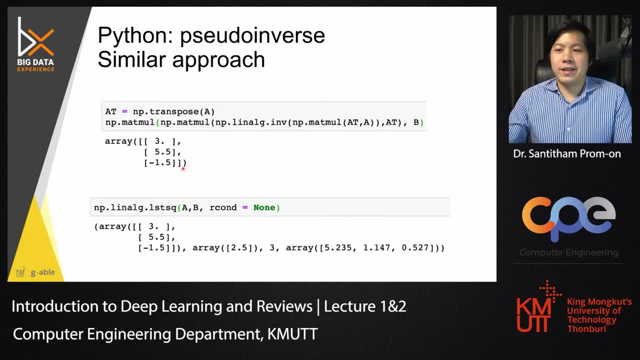 3, 5.5, and minus 1.5.. Okay, You can also solve it another way, using the linear algebra and least-square method. The least-square method would solve using the similar technique and then find a solution like this. 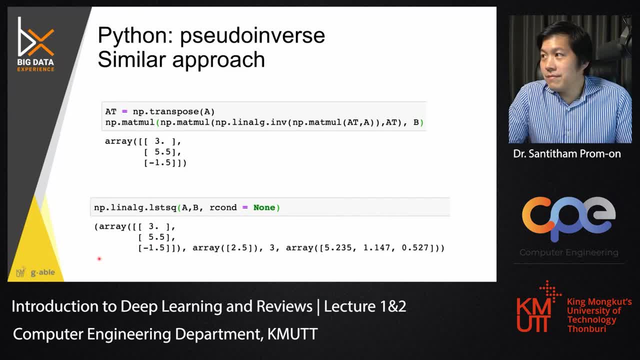 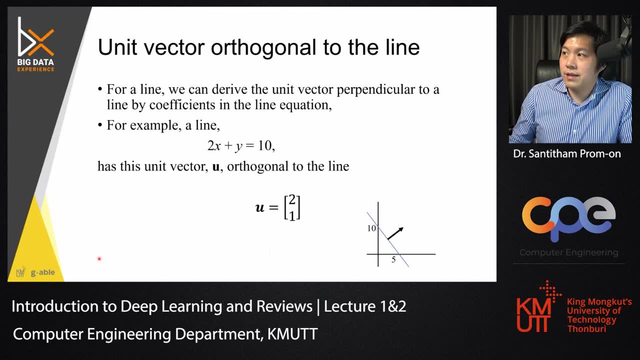 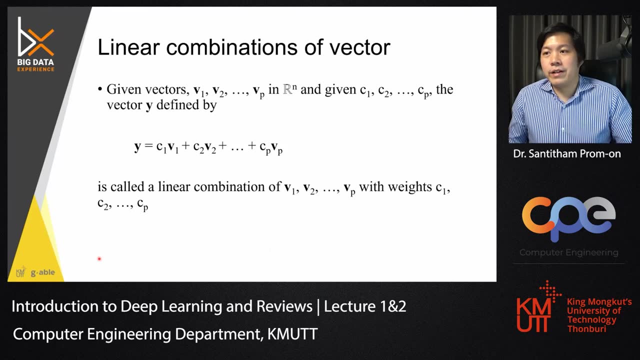 Okay, Almost done for the matrix and vectors. I think, Yeah, Almost all of that. Okay, Some of them you have already learned. so if you are not sure about the concepts, try to review the old contents or you can ask here. 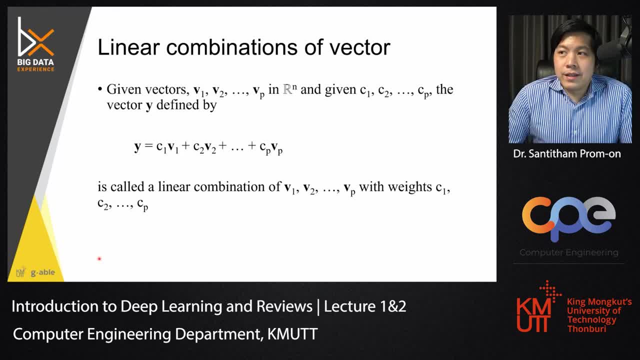 or ask in the group. Okay, We call, Well, we call a linear combination, a set of vectors, a linear combination of vectors. Suppose we have a vector v1 to vp and we have coefficient c1 to cp. Say, if we have y equals c1,, v1, c2, v2 to cp, vp. 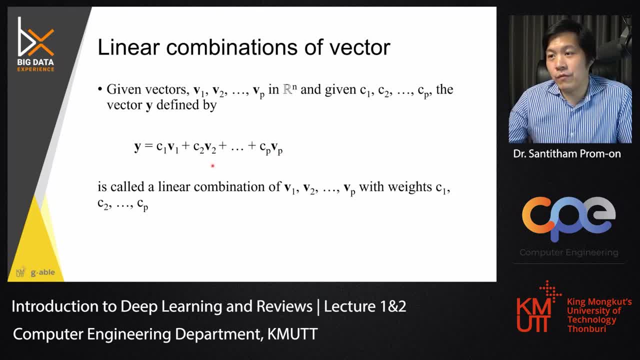 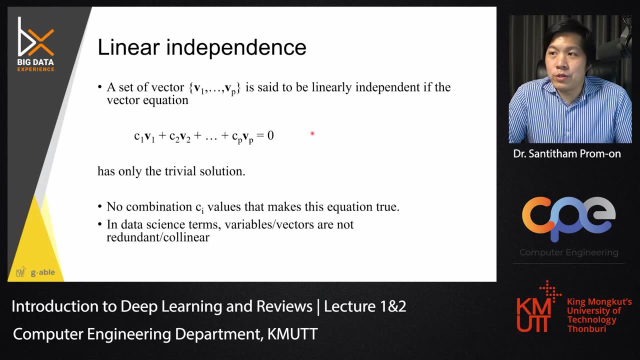 we call this a linear combination of vectors because they are linearly combined. That's why they are called linear combination of vectors. Why do you need to know this? It's because of the next concept: The linear combination of vectors. Suppose you have a vector like this: 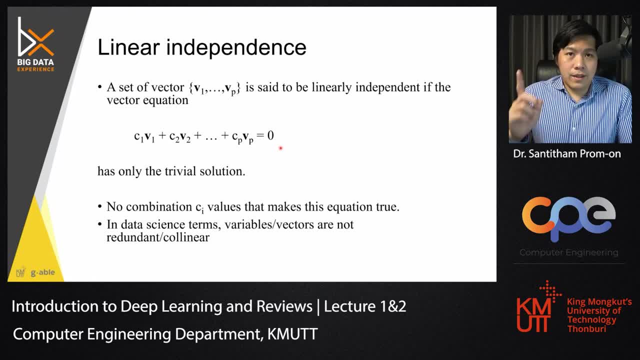 in linear combination. If, If you can equate this c1 to cp to 0, and has only And this work, And this work only in the trivial solution, What does that mean? You cannot combine the vector And make them 0.. 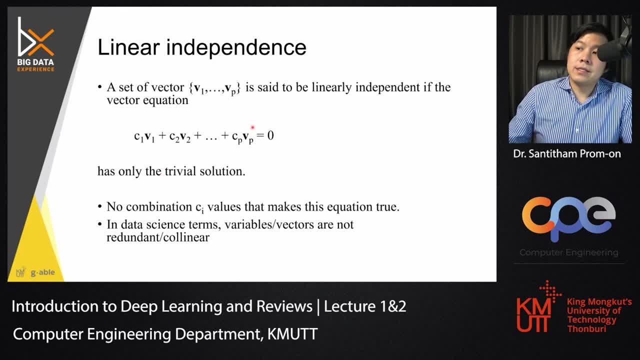 If that is the case, then it means that these vectors are linearly independent of one another. They are not dependent on another vector. Independent, For example, like this one: c1, 0 and 1, plus c2, 1 and 0. 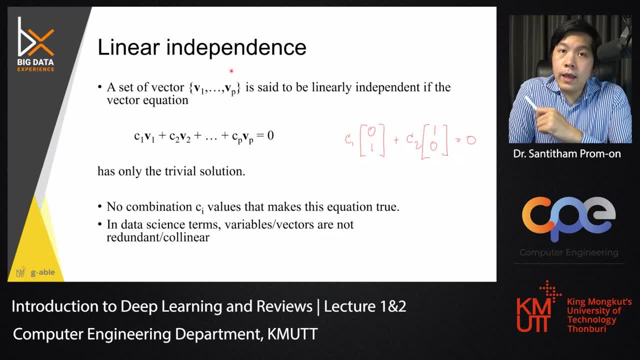 Equals 0.. Can you find c1 and c2 that are not both 0 and work? You cannot, Right, Because they are independent of one another. One is going to like x-axis, Another is moving toward like y-axis, So that's the case. 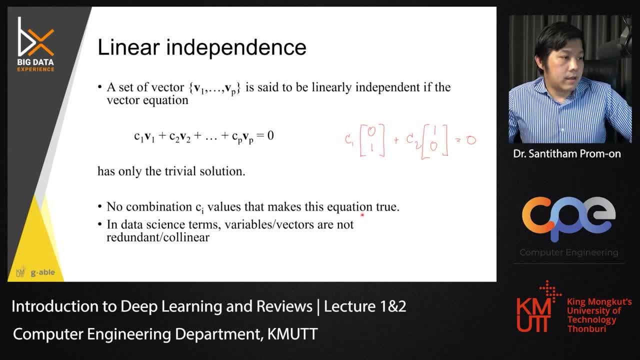 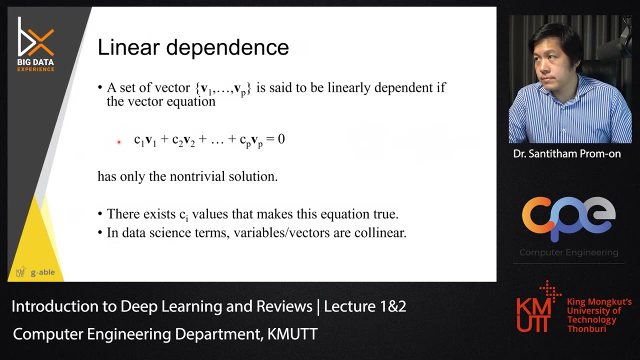 And in many, In many data science applications. we want to determine this Because if, In some cases that you find the solution here, it means that the vectors may be collinear or redundant, You might not need them in your model. 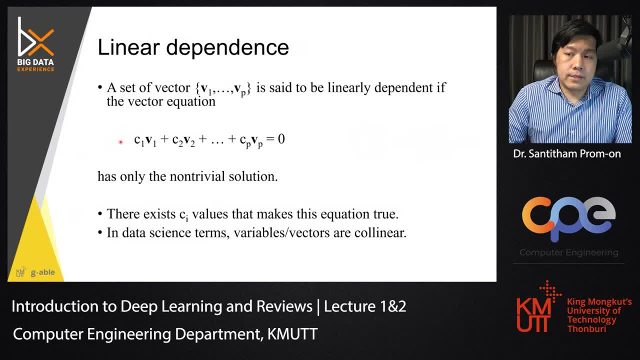 And that's the case for the linearly dependence. If you can find a solution- the non-trivial solution in this case- that exists, the values. that makes this equation true. we usually call this the collinearity. They depend on one another. 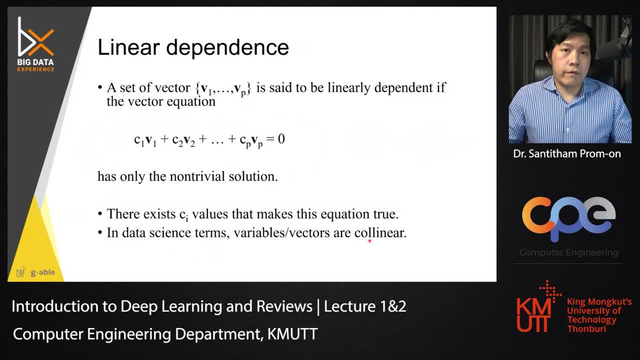 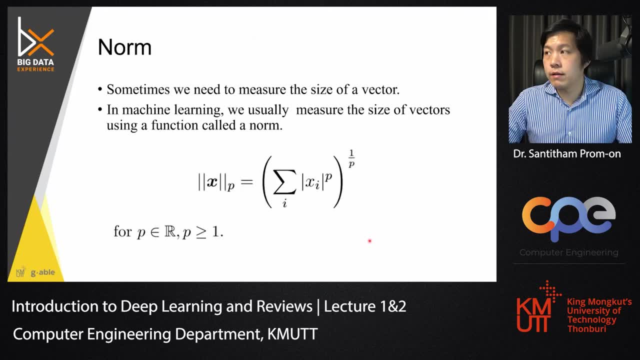 And you can kind of remove them out from the equation, Although for deep learning you might not have to do so by yourself. But well, this is the concept of independence and dependence. Now let's move on, The concept of norm in vector. 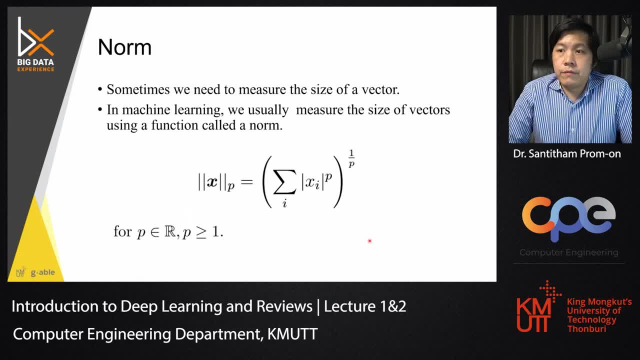 Norm is referred to the size of the vector. We usually call the function norm as the norm of all the p, The norm of, And usually we use like L1 and L2.. The norm of all the p can be found by this equation. 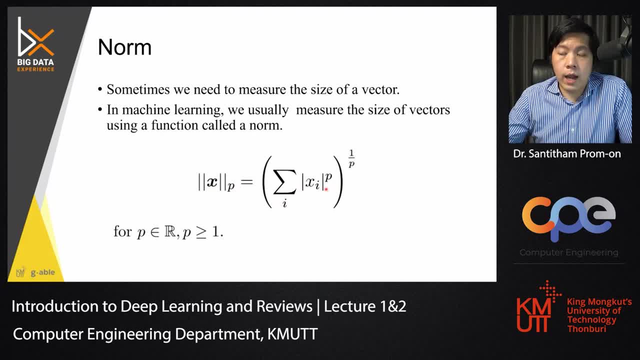 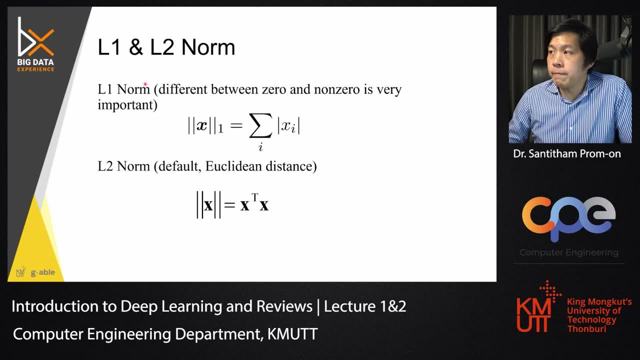 It's actually a summation of the value to the power of p and then 1 over p. So for the L1.. For the L1, L1 norm will be the size of the vector with respect to each of the sides of the vectors. 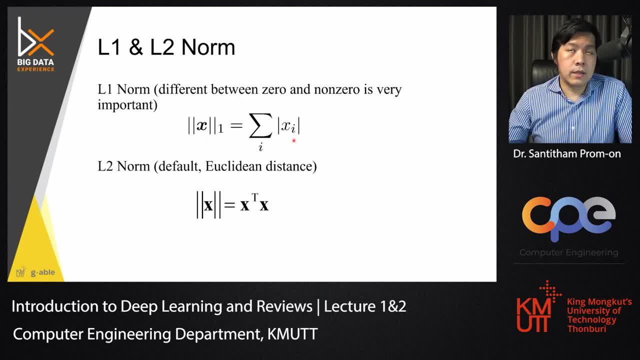 each of the eigenvectors, each of the coordinates. distance L2 refers to something like Euclidean distance can be found by the dot product between two vectors. And then you get. It is actually not true. You have to have the square root here as well. 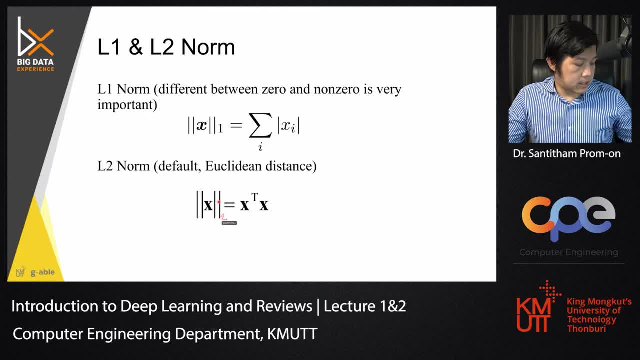 I think it has to be something like this: Yeah, To be correct, Because the L2 norm will be the square root of the L2 norm, Will be the square root of the x1 square plus x2 square, plus dot, dot, dot plus n square. 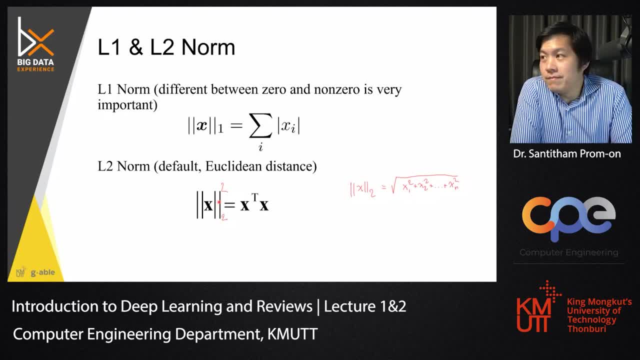 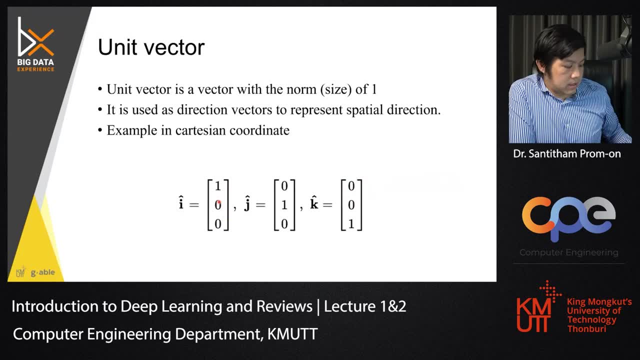 So the dot product between them would be the square of the norm Right. This is the L2 norm. Next, In terms of vector, we call a vector a unit vector when it has a norm of 1.. Has the L2 norm the size of 1.. 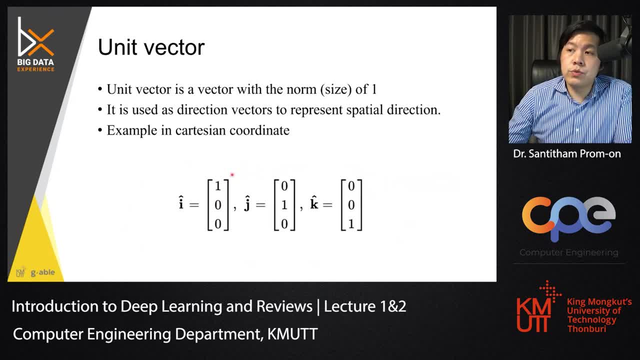 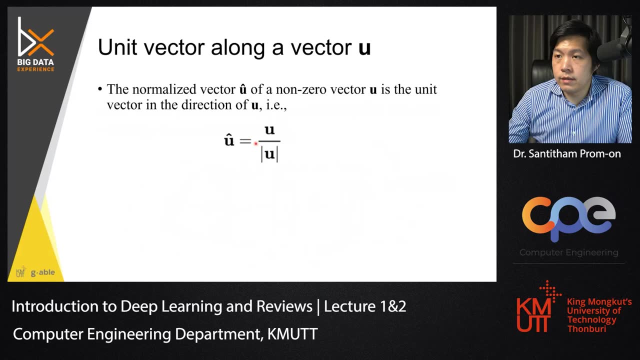 Okay. It is usually used to represent the direction of the direction because it has the size of 1.. We can find the unit vector along a certain vector by taking that vector and divide it by the norm of the vector. Then you get the unit vector moving in that. 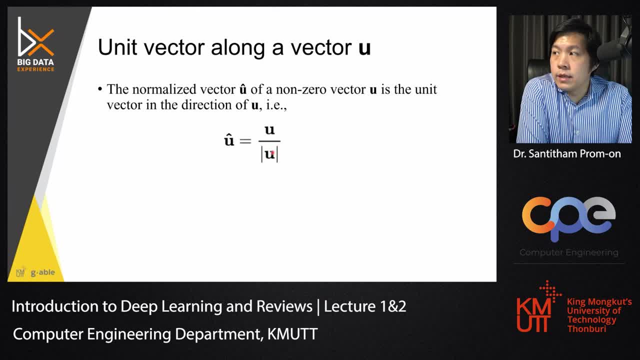 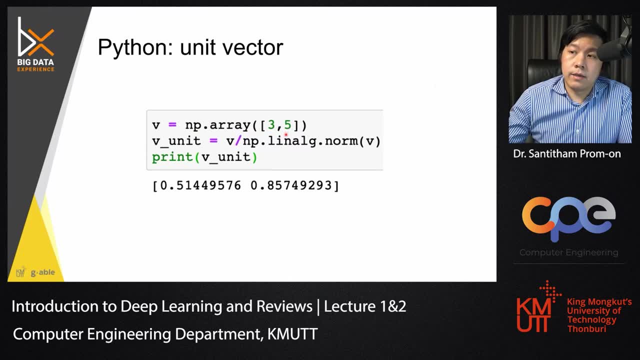 the same direction as that vector. In Python, if you want to find the unit vector, you can do it by taking like this: one is the the vector 3, 5.. And then, if we divide the vector v by the norm of v, 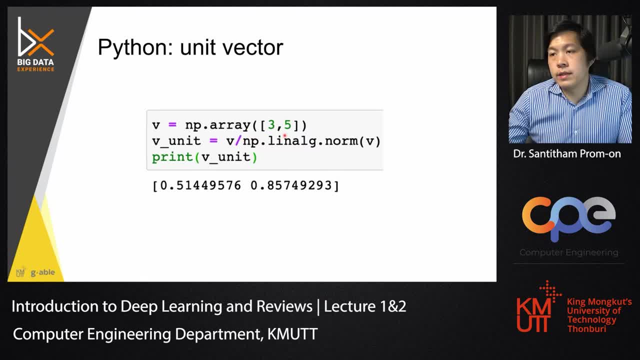 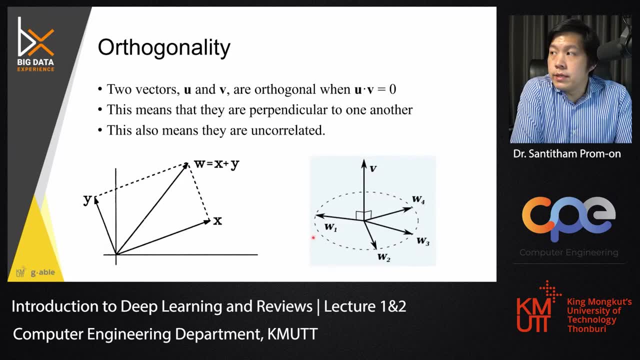 we get the unit vector of v. This would move in the same direction as 3, 5. Knowing the unit vectors allow us to determine the that the vectors may be. well, when we have vectors we can represent, we can determine whether the vector is. 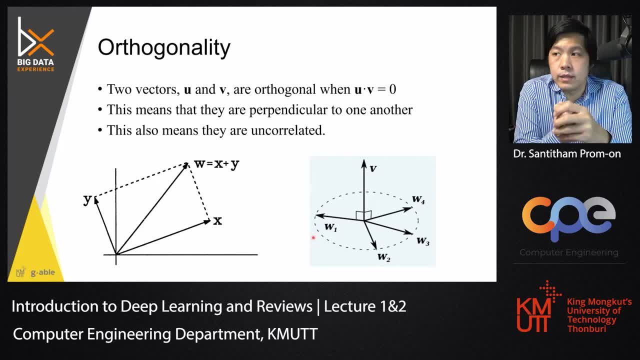 perpendicular to one another. We usually call this perpendicularity of the vector as octagonality. The two vectors are octagonal if when you dot them and then you get the value of 0. Why is that the case? Think about that vectors are. 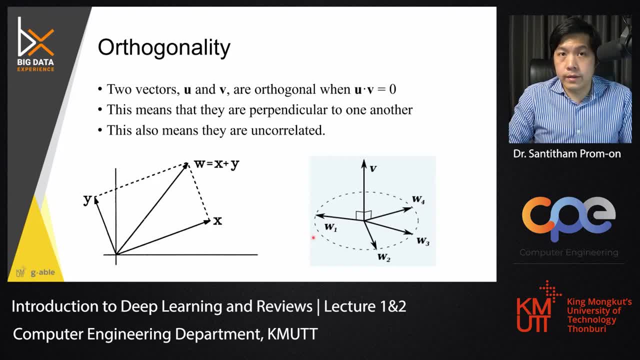 when they are perpendicular to one another. they are not related to one another, Like the vector that moves in the direction x and the vector that moves in the direction y. When x moves, it doesn't affect y. When y moves, it doesn't affect x. 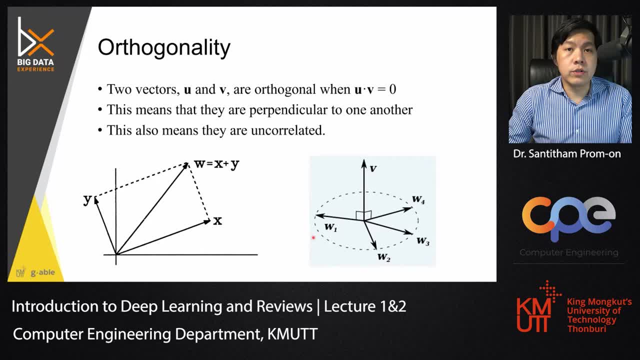 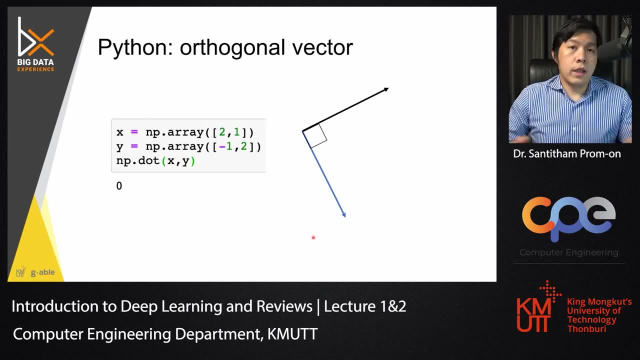 We usually call this orthogonal to one another or they usually are unrelated to one another, Like these two vectors, 2, 1 and minus 1 and 2.. If you perform dot product between them, you get the value of 0.. 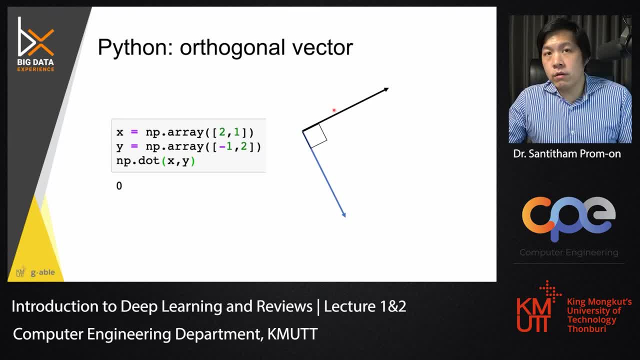 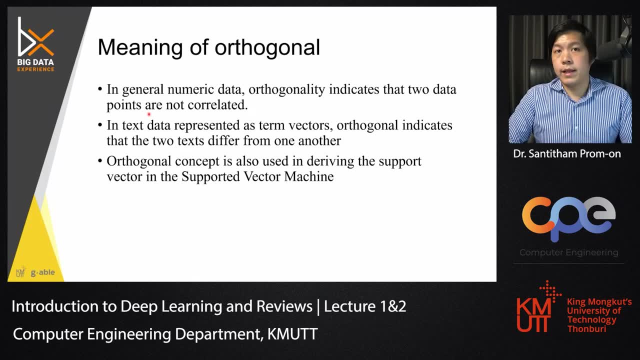 And these are orthogonal vectors. Orthogonal has certain meanings. You can think about orthogonality as in the numerical sense. they are just not correlated, not related to one another. But think about it as suppose that you talk about text data. 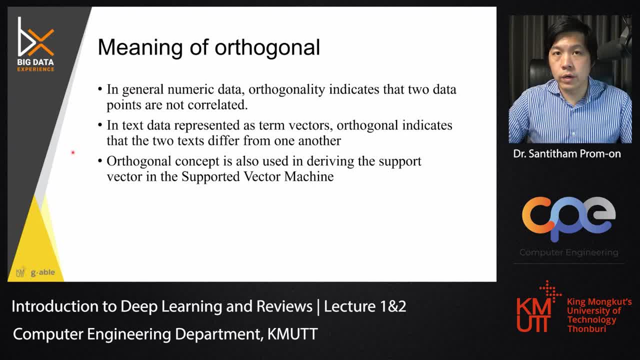 If you have two vectors representing the keyword extracting from two different, two different documents, and then when you're calculating the orthogonality between the two vectors, you find that they are orthogonal. When you dot them, you get 0.. And that would mean that 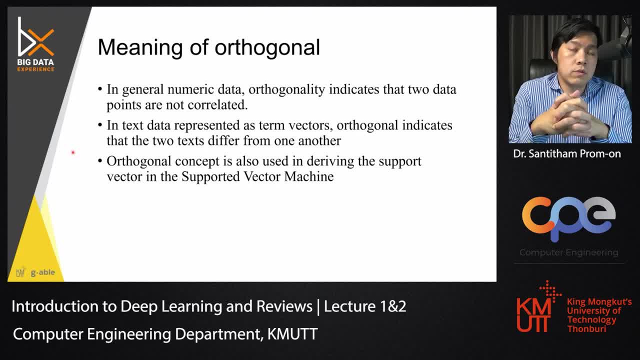 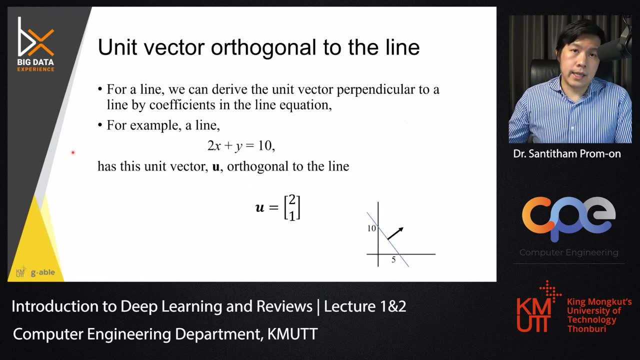 the documents belonging to different topics, potentially So. orthogonality is used in lots of concepts in data science, in SVM, in finding similarity and other things in PCA as well. We will talk about that later on. The unit vector aligns. 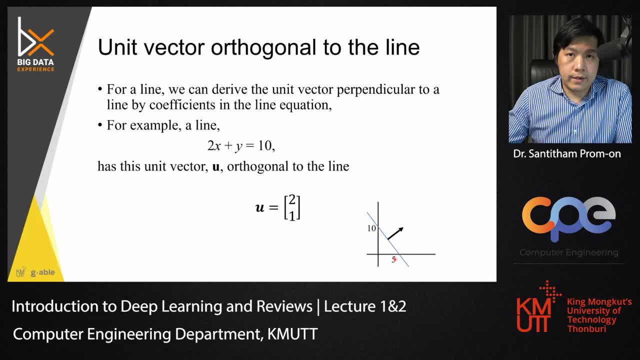 If you have a line like this, 2x plus y equals 10.. Here is the line. You can get the vector that is orthogonal to the line by just taking the coefficient, Like the 2 and 1 will be a vector that is orthogonal to the line. 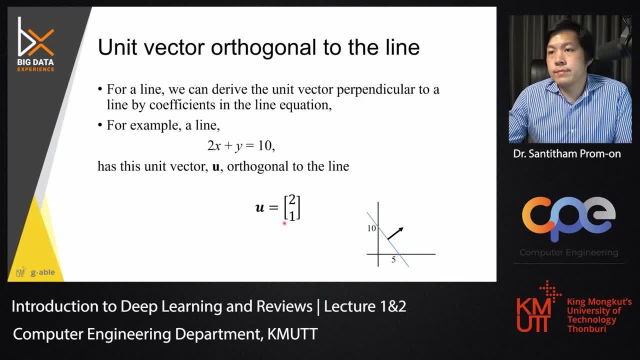 perpendicular to the line. This is 2, 1.. So that's all for the review of the vector concepts and equations before we move on further to the next topics. Mostly, these are the things that you have already learned in your undergrad level. 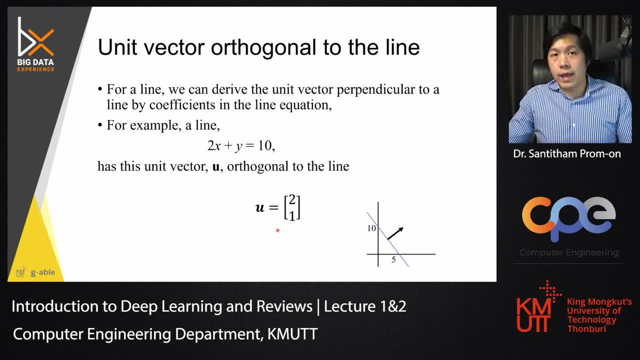 Some of them might be before, that might be in your high school level, And I know these are quite a long time till now. but you will have. this is a chance that you will use all of them And you'll see later on in the subsequent lectures. 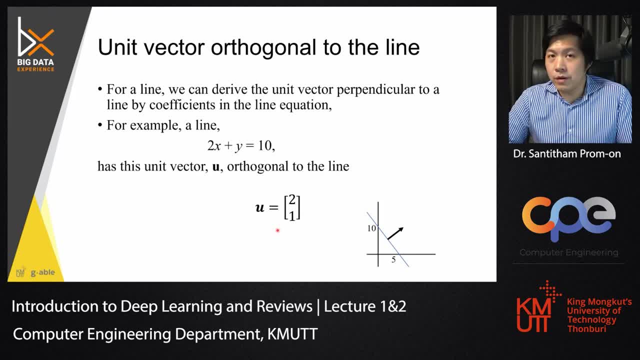 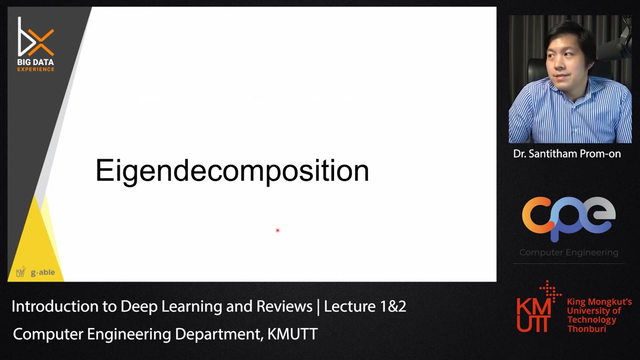 that some of these play very important roles in learning, in learning deep learning. Any questions about the vector and the matrix before we move on to the next topic? All right, No questions then. next It's the eigendecomposition. 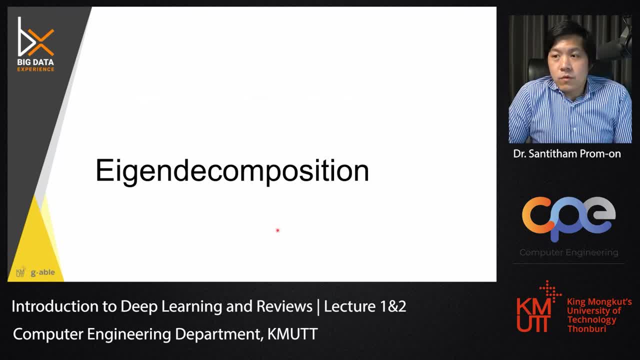 What is eigendecomposition? What is decomposition? The concept of decomposition comes from that. we can think of the data as the combination of multiple patterns. We can extract those patterns out to have different types of consistent patterns. There are many techniques that allow you. 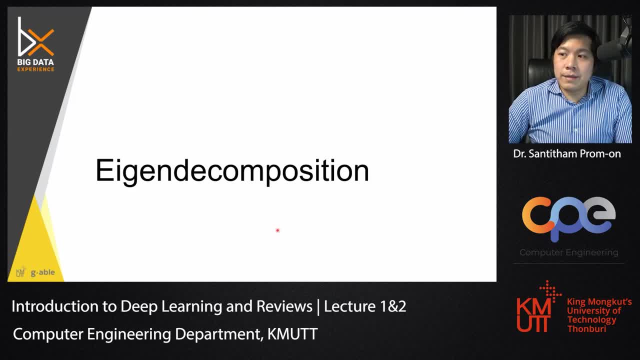 to extract those out, And some of which relies on the mathematics, some relies on statistics. In a lot of machine learning techniques, we use statistics to identify which variables are important. Those are also decomposition, the regression technique. Now, what is eigendecomposition? 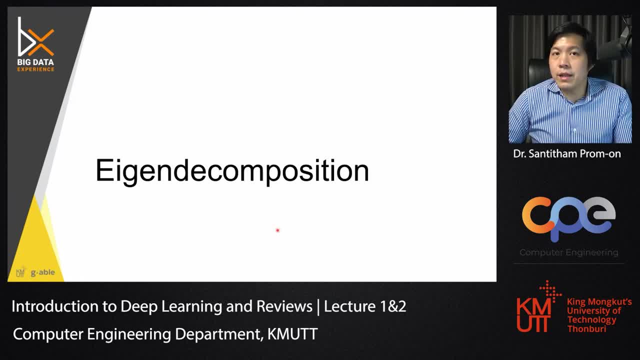 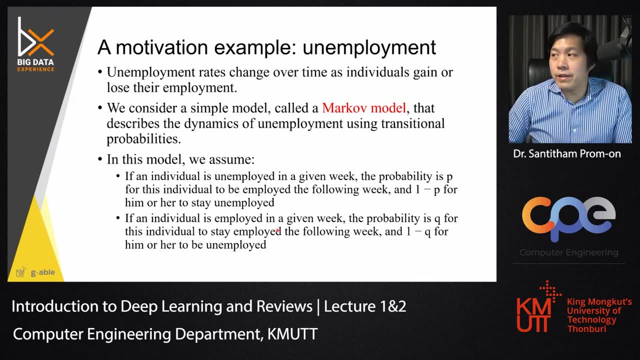 Let's take a look at the concept first, And then it might allow you to see that eigendecomposition plays very important roles in the development of Google, in the graph theory, in other things. Let's consider this situation that we are talking about: unemployment rate. 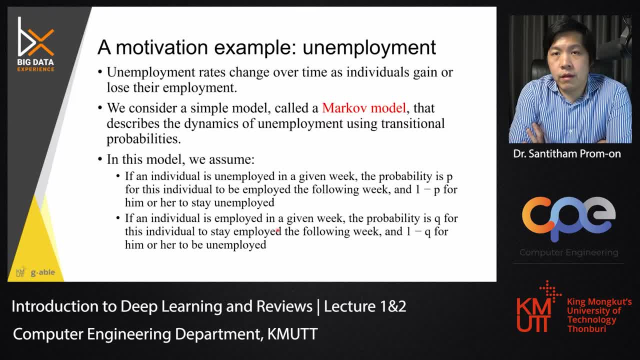 And then we want to describe the unemployment and employment, the rate of unemployment and employment. We want to create a population-based model, like in game theory, using the model called Markov model. The Markov model explains the transition between states as the dynamical process. 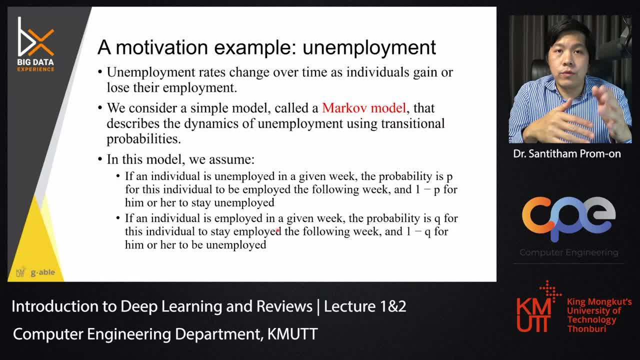 What does that mean? It means that when you are at one state, you have a chance to transit to another state. Okay, so suppose that you are currently unemployed. An individual is currently unemployed. There is a probability P for you to be employed in the next week. 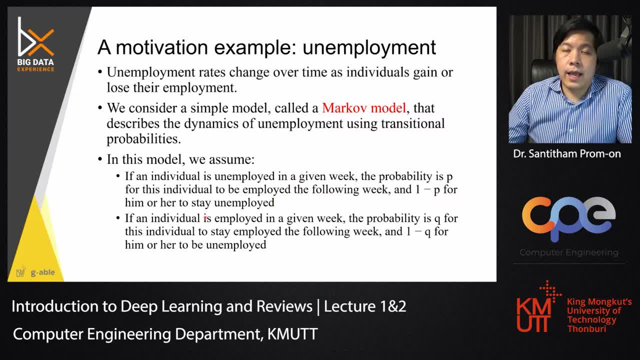 and 1 minus P to stay unemployed. If that individual, if the individual is employed in a certain week, there is a probability Q to stay employed and 1 minus Q to be unemployed. Okay, hopefully I'm not confused now. So let's see if the variable is correct here. 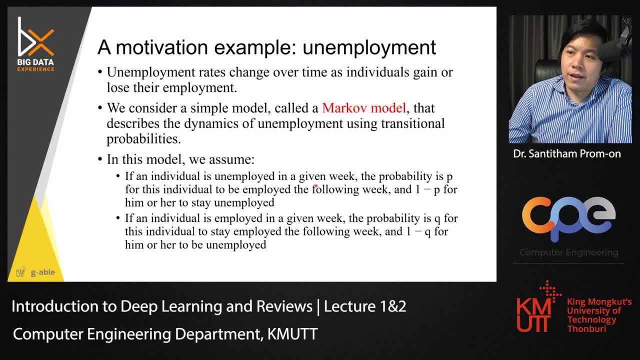 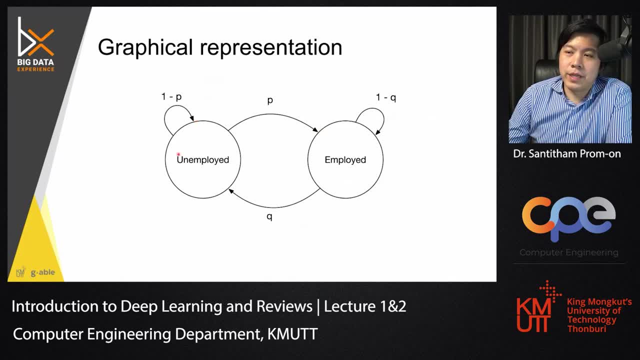 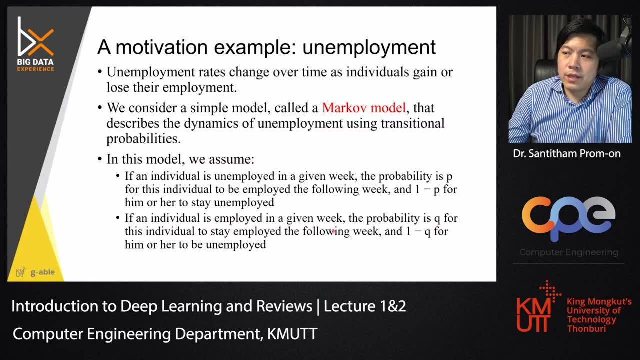 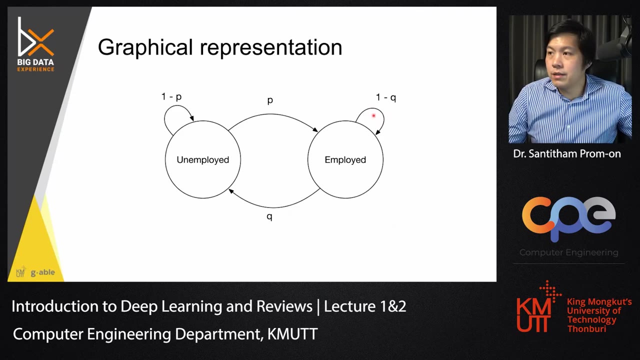 So we have here: if we are still unemployed, then probability P to be employed and 1 minus P to be unemployed. Okay, this is correct. If at a certain week that individual is employed, then probability Q for stay employed. Q for stay employed. 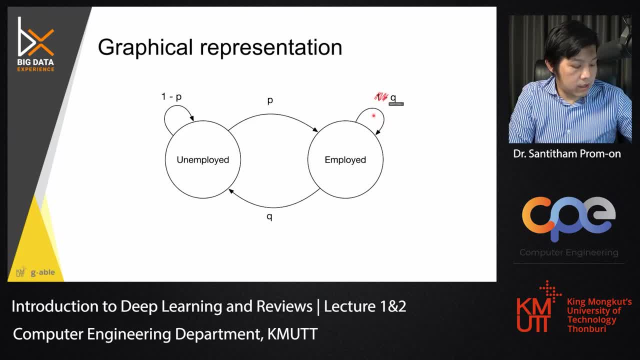 Q for stay employed. Maybe I should use this one, So it will stick to the slide. Let me Q for employed 1 minus Q for transition to the P to be unemployed, Right, And then we can write a Markov model. 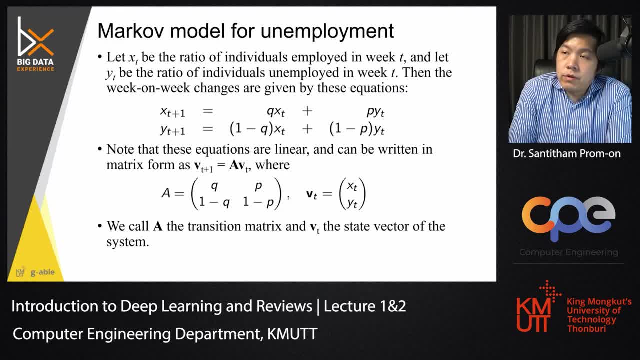 for unemployment like this one. Suppose we have here have X as the individual, the number of the ratio of individual being employed at week T and YT becomes unemployed. Then at a certain week the number of employment for XT would be QX here. 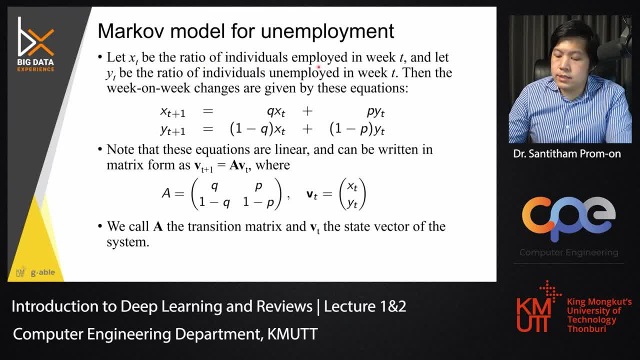 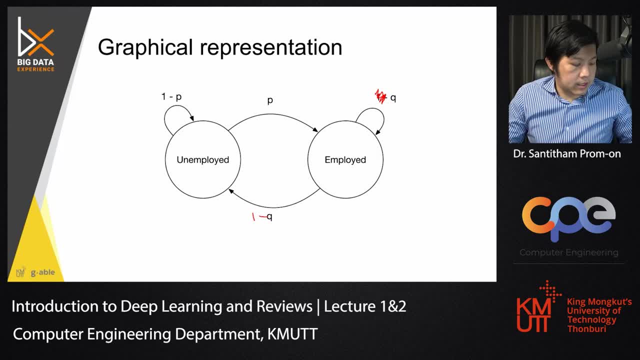 Q times X. So X is the number of the ratio of individuals that is employed. right, This is XT, so I should write like this. Let me like it here: Employ is X, Unemploy is Y, So the number of X would. 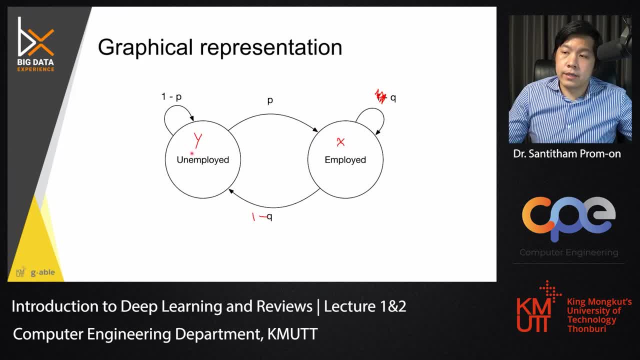 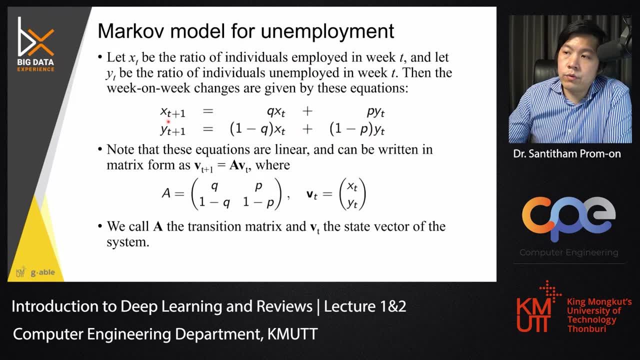 comes from. just look at the arrow sign. X would come from transition for unemployed to employed, So P times Y and Q times X. That's why we have this. X at T plus 1 would be Q times X at T and P times Y at T. 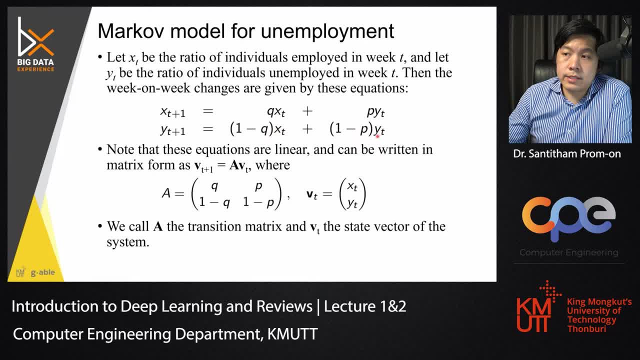 And Y at time. T plus 1 would be 1 minus Q times X and 1 minus P times Y. This is called the dynamical system because it's changed according to times. Now we can represent this as the. 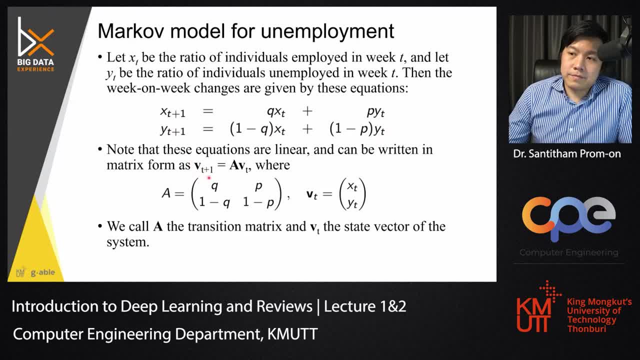 as matrix like this. So it means that V at time T plus 1, equal AVT right, And V at time T plus 1 is XT plus 1, YT plus 1.. V at time T is XT and YT. 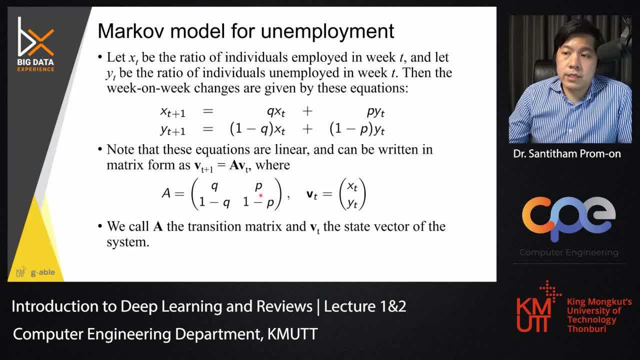 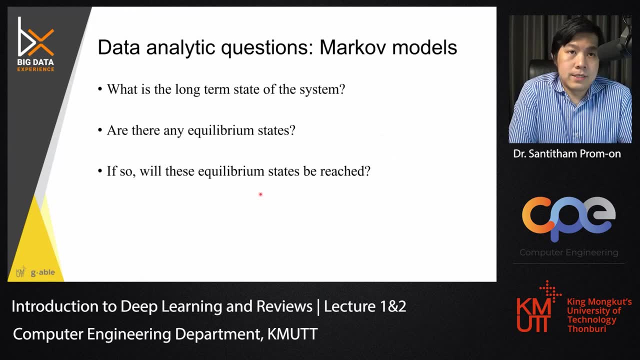 And the coefficient is Q, P and 1 minus Q and 1 minus P. Once we reach this stage of the model, we can determine the behavior of this dynamical system, of this game theory, to determine the long-term state. 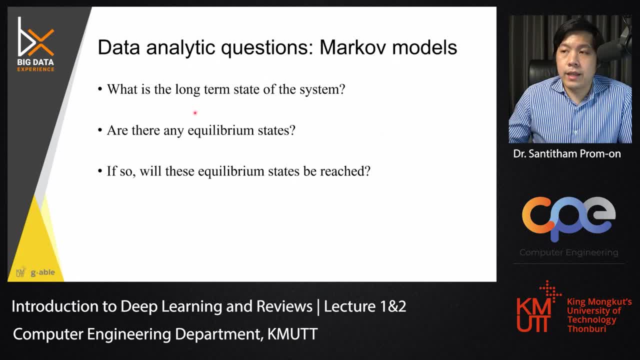 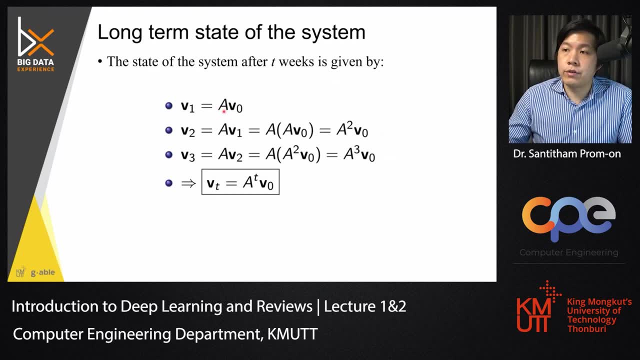 This is called the equilibrium. where there is an equilibrium with the model, How do we determine that Computationally, you can multiply the transition? Think about that, because if you multiply it one time, that's one week, Two time. 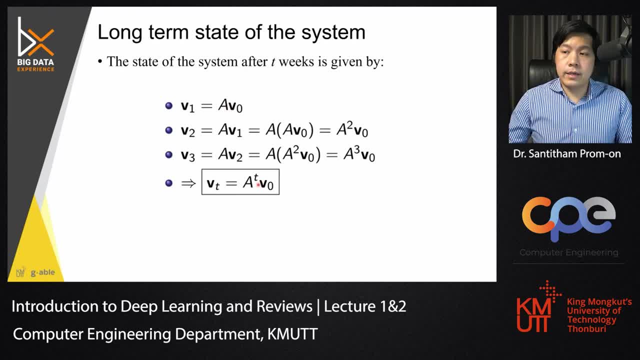 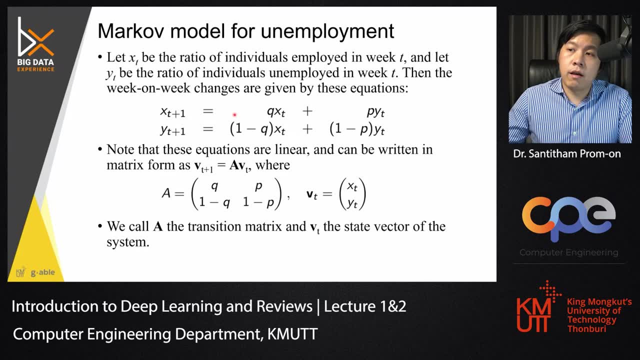 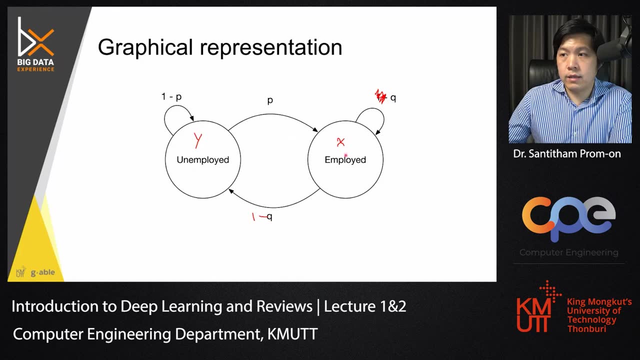 two week. So you multiply it T time, then you get the transition for T week. Suppose that at the start we have the P as the probability of of what P is probability of getting job. right Yeah, of getting job. 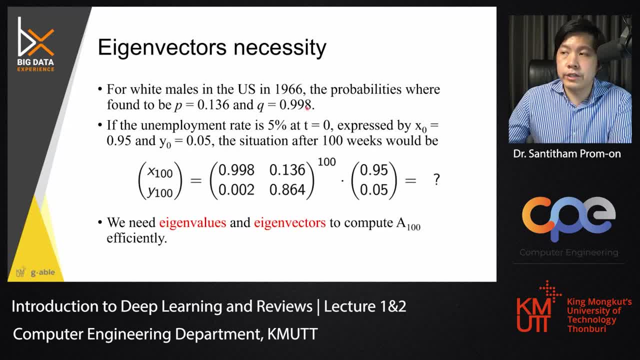 Q is the probability of retaining job. We have one of P and Q like this. one Have 99% to retain the job, has about 14% to get the job And then, at the current rate at the moment, suppose that the X0 is 0.95. 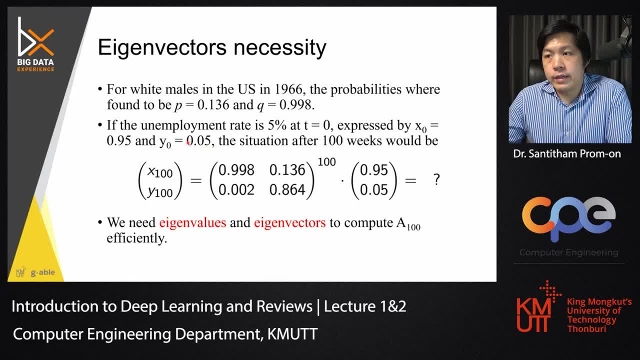 and Y0 is 0.05.. These are the unemployment rate. unemployment rate After 100 week. we can make projection on what would be the values. Right, You don't really need to do this. You don't really need to multiply it 100 weeks. 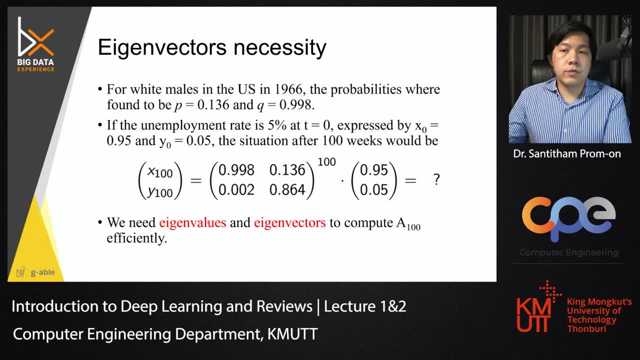 or 1,000 weeks, because you can actually decompose this matrix and find eigenvalues and eigenvectors and then know the and then know the equilibrium, the values, if you multiply it 100 or 1,000 times. Okay, 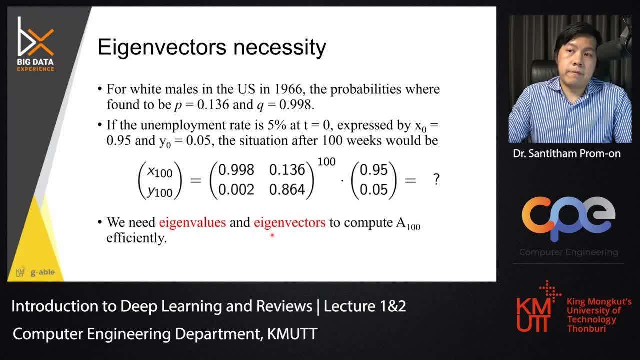 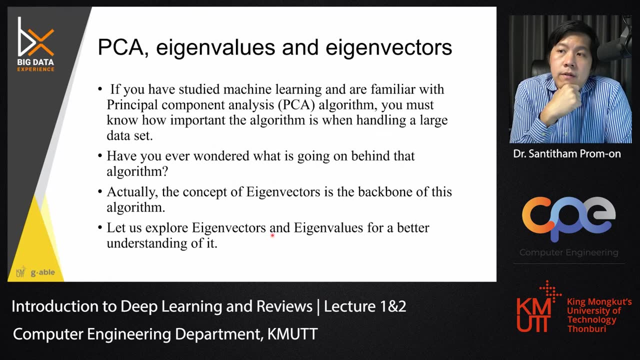 Eigenvectors has been used in other technique as well. Right Eigenvectors are something like the core, the core X axis of the, of the matrix, of the vector of the data. So it's best to imagine in terms of the PCA technique. 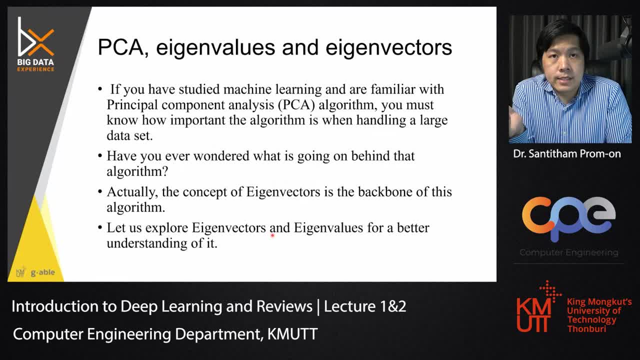 The technique called PCA or principal component analysis. it's a technique that allows you to identify the principal component or the eigenvector of the data And, instead of representing data as it, you can projecting the data onto the new axis so that it would be represented better. 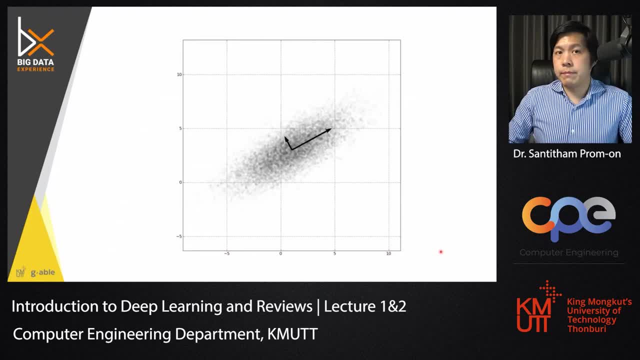 than the current coordinates. For example, suppose you have the data in X and Y like this one. This is X, the X axis and Y axis, And you can see that X and Y are somewhat collinear, that they are like. 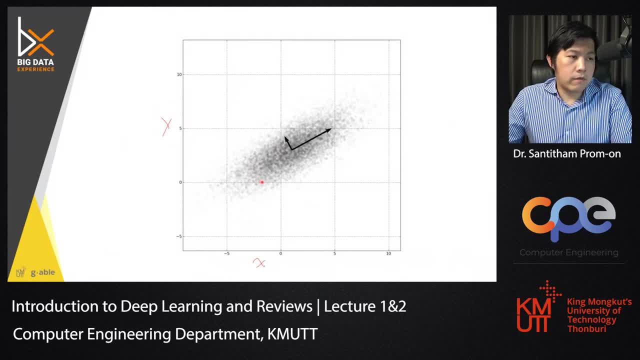 if you look at the dot in the scatterplot, they are kind of going in the same direction as one another. So techniques like PCA allow you to identify. the PC allow you to identify something like X prime and Y prime, The axes that are not depending on one another. 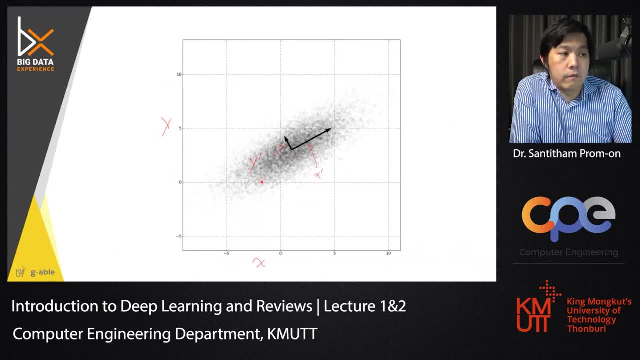 these are the eigenvectors of the axis And the eigenvalues. these are the spread of the data, And PCA allows you to identify this and then projecting each point onto the new axis. So this is the reasons that eigenvectors and eigenvalues. 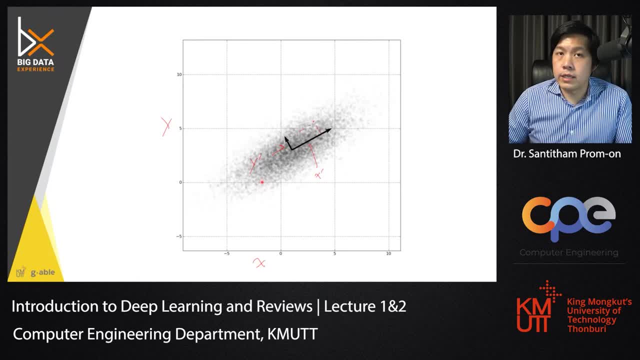 plays quite important roles in machine learning. That is because it allows you to transform the data from one domain to another domain. that is easier to use And actually, deep learning do the same thing. Deep learning transform the data from the raw data domains. 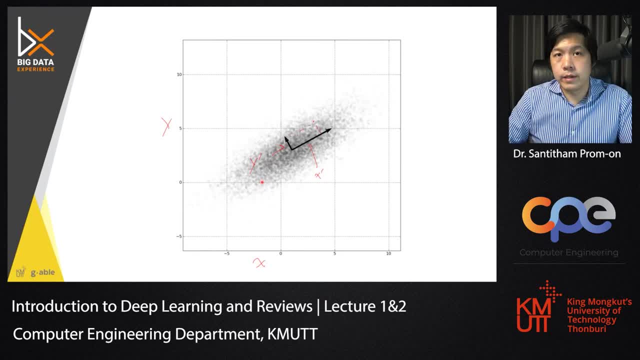 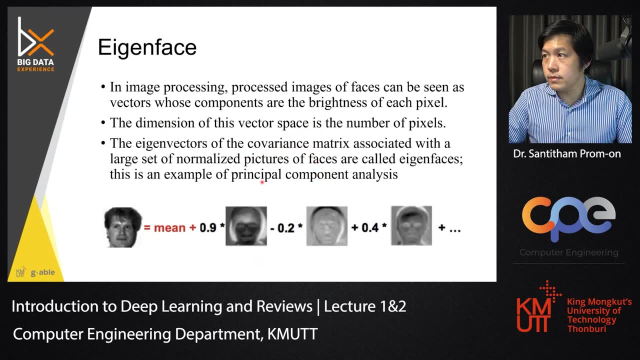 into the transformed data domain. that is easier to classify And we will see that later on in the concepts afterwards in the latter classes. Eigenvector is also used in applications like eigenphase. that is to compose the phase into the composition of the template phase. 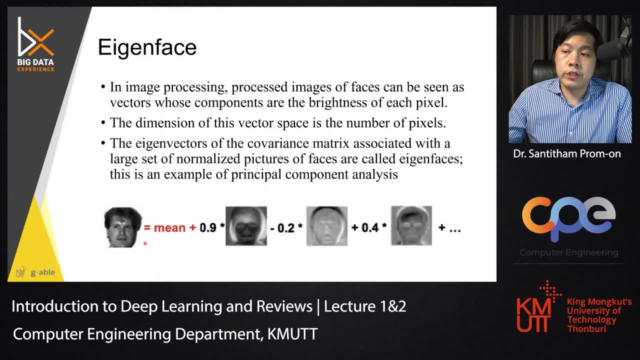 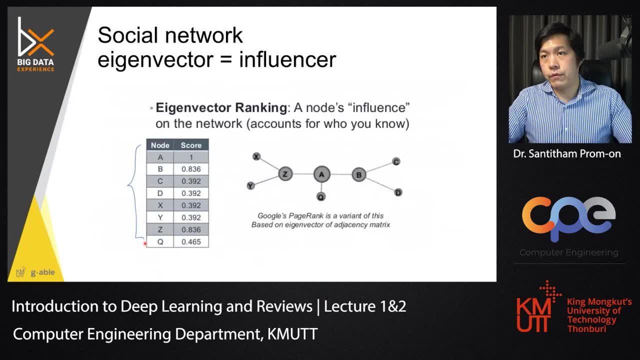 or the eigenphase, And then you can use the coefficient to identify whether the phase that you are receiving is actually similar to the phase that you are trying to compare with or not. The eigenvector is used in social network analysis to identify the nodes that are important. 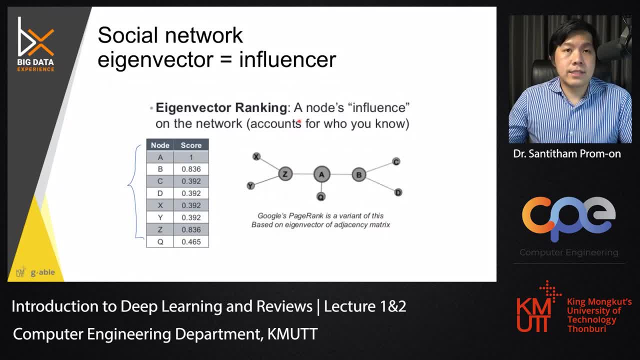 By representing the graph as a matrix, you can identify which node is likely to end up with if you were to randomly walk in the network. This is called Google PageRank. Google used this structure to identify which web page is likely to be the prominent web page. 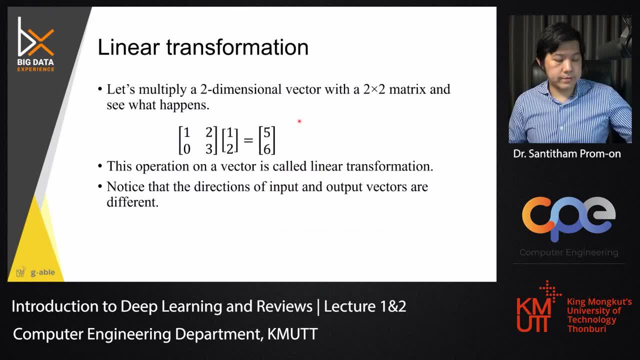 by analyzing its structure. So eigenvectors and eigenvalues play an important role in linear transformation as well. So if you transform, I have a matrix to transform. this matrix actually transforms the points 1,, 2,, 2,, 5,, 6.. 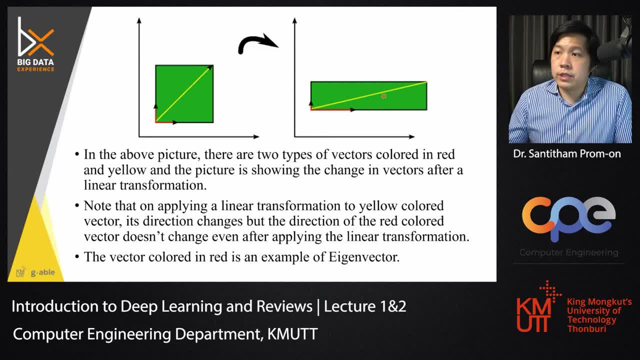 But you can see that after transformation, the matrix, even from this vector to another vector, is actually the scaling of the values on the axis of x and y axis, But the direction of x and y axis stay the same. The x and y axis are known as the eigenvectors. 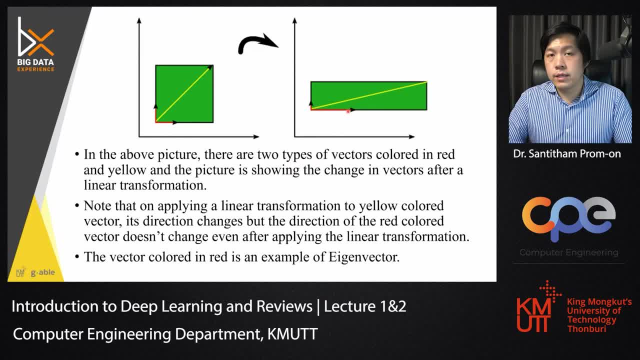 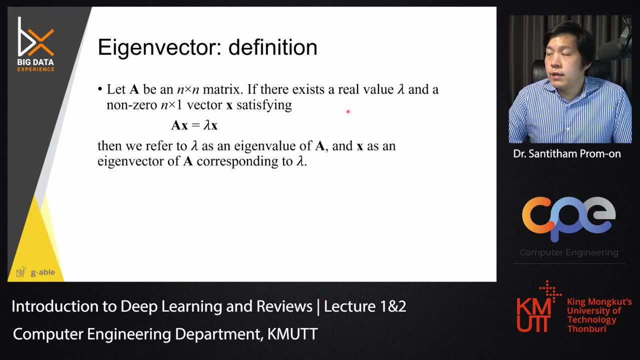 That is when you make the transformation. it doesn't change but the value at that axis changes. So in the formal definition the eigenvector can be thought of as a vector. that when you multiply the transformation to the vector, multiplying transformation A to vector x, 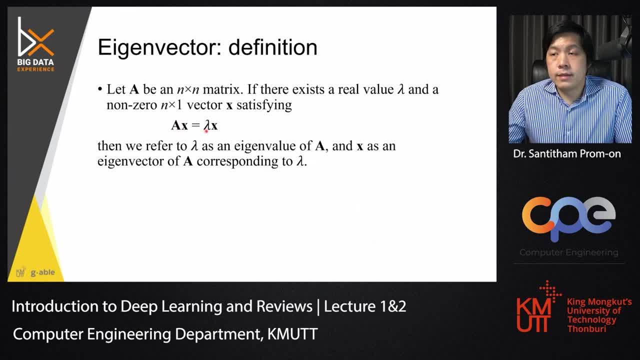 it results in lambda- x, where lambda is a square and x is a scalar value. What does that mean? It means directions stay the same, no matter what values that you multiply the vector with. It will just translate, it will just enhance. 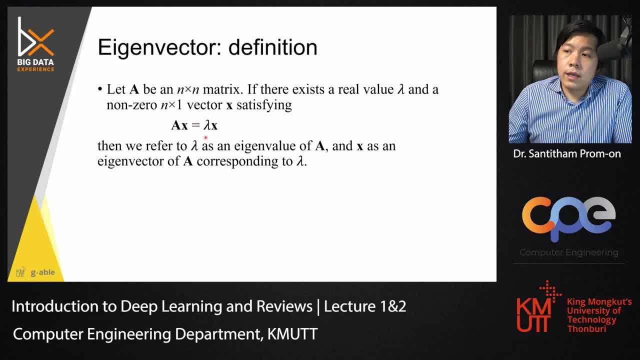 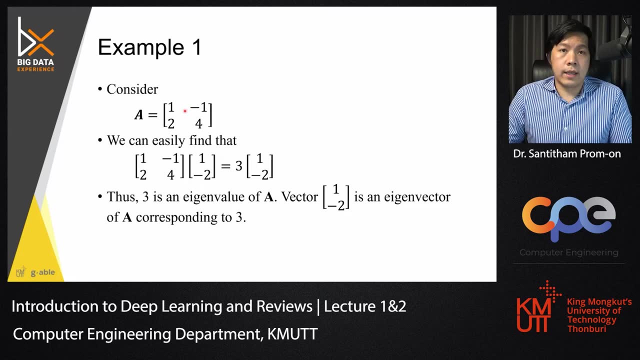 but in that same direction. We call this lambda here of A as an eigenvalue of A and x as the eigenvector. Now let's take a look at some examples on eigenvectors and eigenvalues. Here is an A. 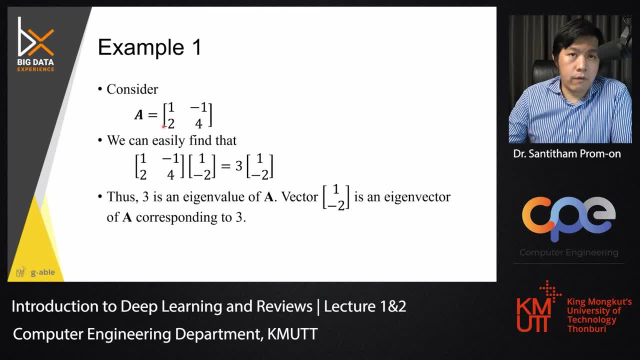 We have A as 1,, 2, minus 1, and 4.. And if we were to multiply A with 1 and minus 2, let's perform a simple calculation here. Take rho, multiply by column. This is 1 times 1 minus 2 times minus 1.. 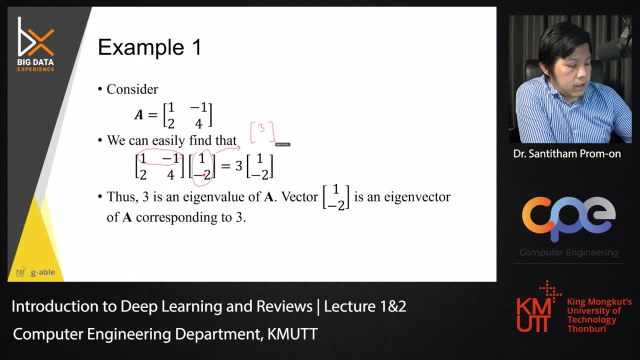 That's why we have the value of 3.. And then 2,, 4, and 1 minus 2,, which is 2 times 1, and 4 times minus 2,, which results in minus 6.. So pulling 3 out: 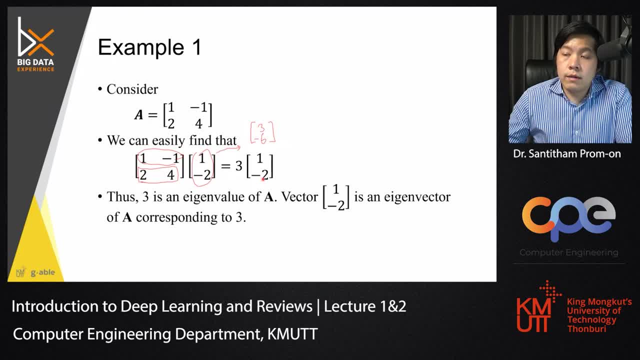 you get 3 and minus 1, 1 and minus 2.. So it means that after multiplication you end up with the same vector, but the transformation matrix transforms into just a single value. Here we call 3 an eigenvalue of A. 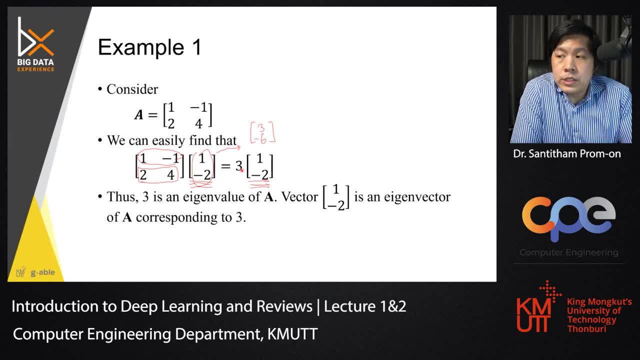 and vector 1 and minus 2 is eigenvector of A, an eigenvector of A with corresponding eigenvalue of 3.. Why do we need eigenvector, Why do we need eigenvalues And how do we find this eigenvector and eigenvalues? 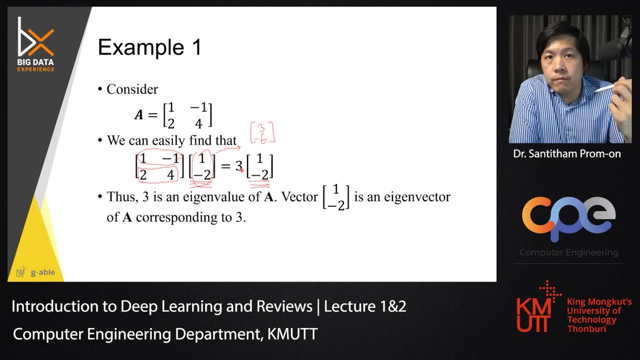 If you think back, some of you may come from engineering backgrounds and you may have, or if you take a physics course in undergrad level, you might have remembered the technique called Kirchhoff, like Kirchhoff voltage law and Kirchhoff current law. 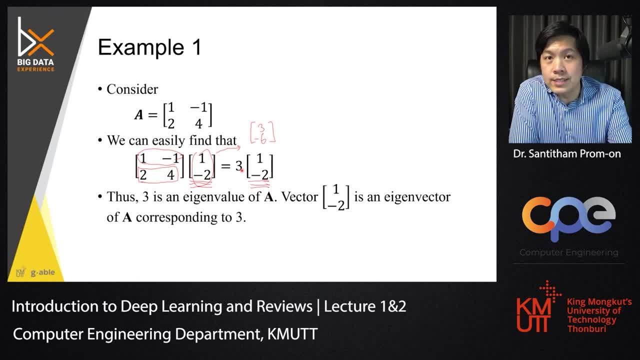 And you might have encountered a technique like node analysis and mesh analysis in the electricals, in the, I would say, in the circuit analysis course or in physics course, when you learn about electricity and the circuit, When you study about the behavior of the signal, like that. 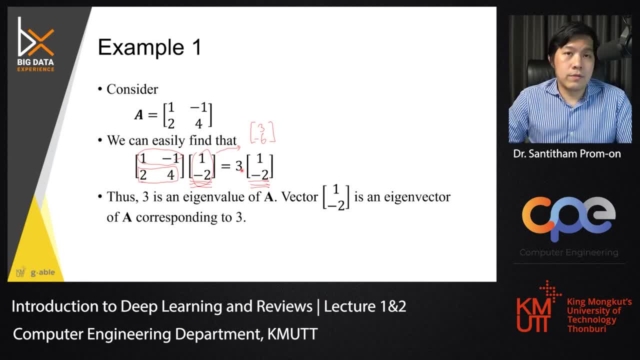 you are actually identifying the eigenvector to get the value of something like E to the eigenvalues to express the behavior of the C and the L in the circuit. But if you have come from other areas, what we are talking about is actually: 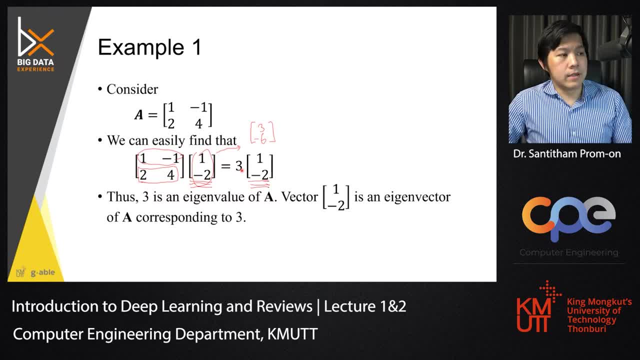 the behavior of the dynamical system, of the mechanisms in the real world, that kind of- I always say that kind of transferring energy from one point to another point and they are exchanging certain energy with one another. So that means so far for this case. 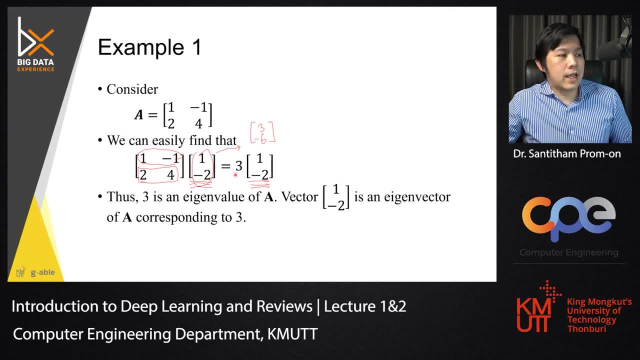 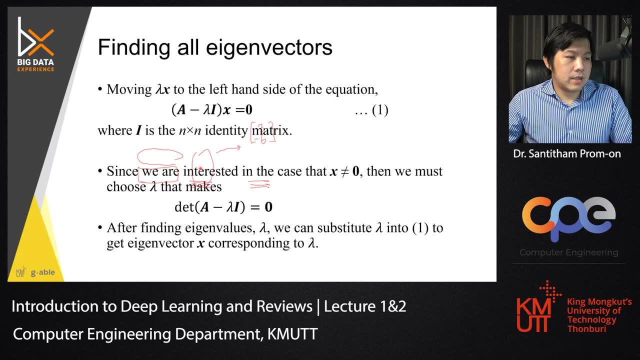 we have this matrix that can be represented as a scalar value- we call this an eigenvalue- And the vector here think about it as the core vector of this matrix. How do we find the core vector of this matrix? We can find the core vector of this matrix. 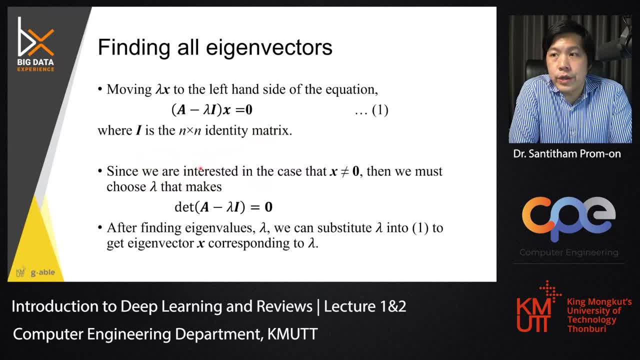 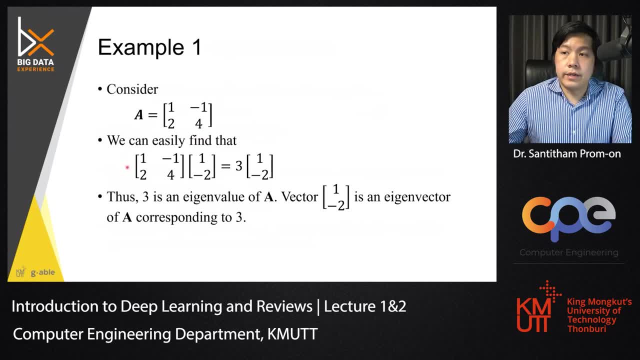 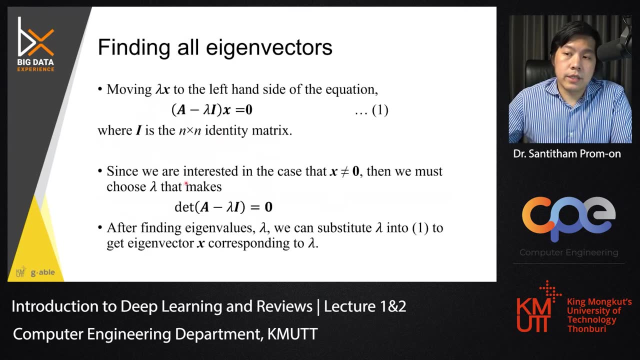 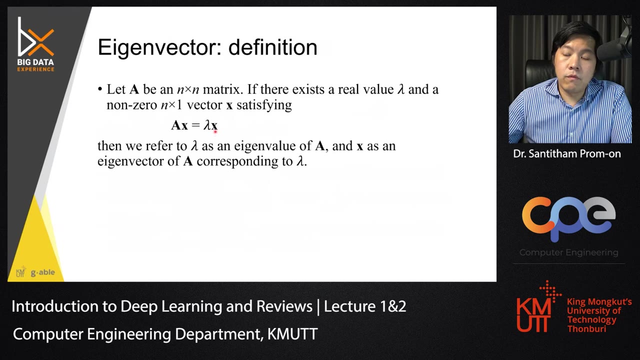 by deriving it from the characteristic equations. So once if we have this coefficient right and we want to find the characteristic equation of this matrix, we can determine it from this by moving the lambda x, lambda x from this equation to the left-hand side. 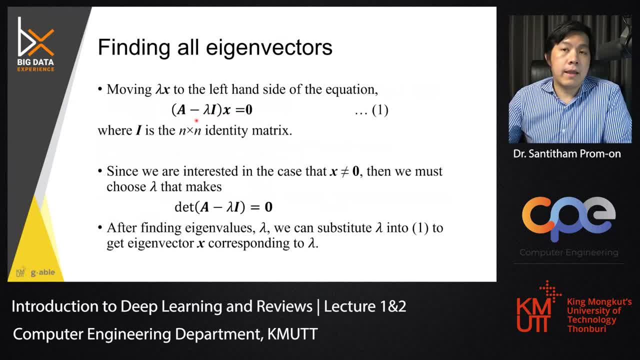 and then pulling x out, We have the A minus lambda- I equal x. For A minus lambda, I equal x to become 0, this A minus lambda I has to have determinant of 0, because it would need to scale x to 0. 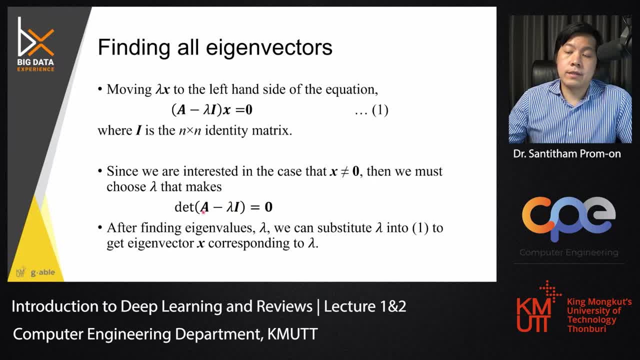 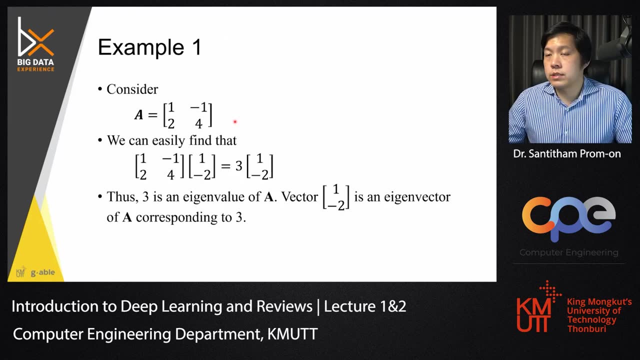 So we have the depth of A minus lambda I becoming 0.. And then, determining the value of lambda, you will get the eigenvalue, And by substituting lambda into 1, you get the eigenvector corresponding to that. Let's see if it works in our case. 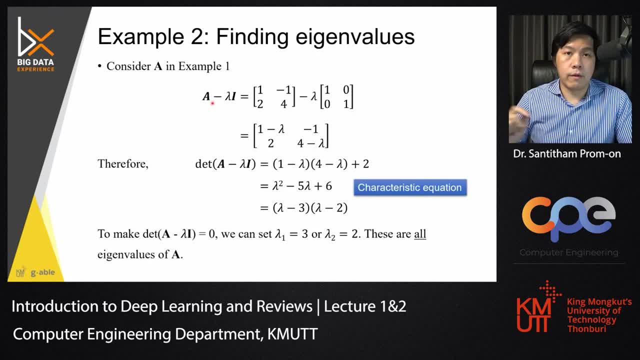 for 1, minus 1,, 2, and 4.. For 1, minus 1,, 2, and 4, we have it here and then minus of lambda and the identity matrix. This would be lambda and lambda. 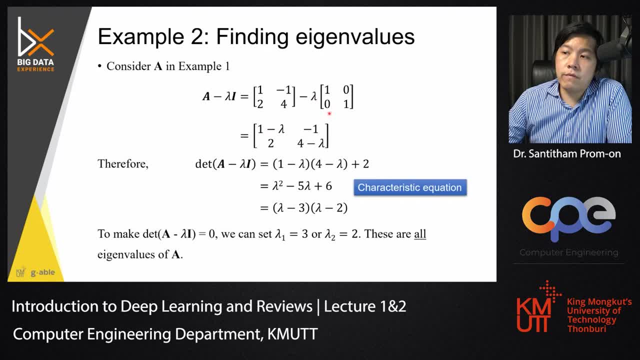 Subtracting it out, you get 1 minus lambda, and minus 1,, 4, and 4 minus lambda. Calculating the determinant of these differences, you get this. multiplying down, become plus, and multiplying up, you get minus, right. 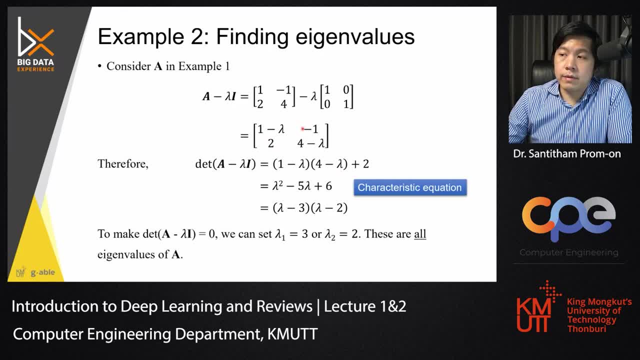 Have 1 minus lambda and 4 minus lambda plus 2, because multiplying up you have minus and with the minus you get plus. Then for this one you have the lambda square minus 5 lambda plus 6.. Just multiplying them here. 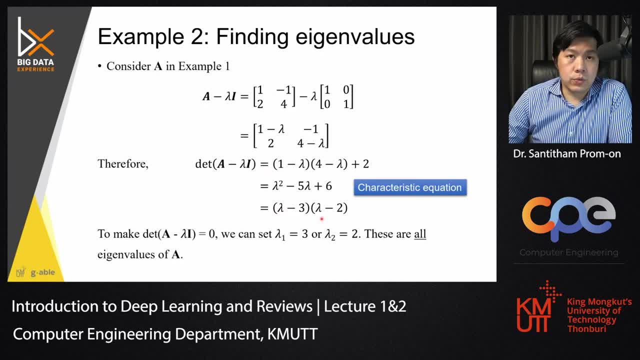 And then take factor, This is lambda minus 3, lambda minus 2.. That means there are two eigenvalues for this matrix. So you get 3 and 2, or the 2 root of this equation. Once we know this, 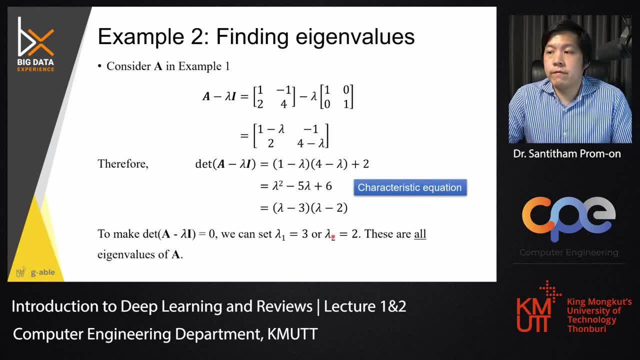 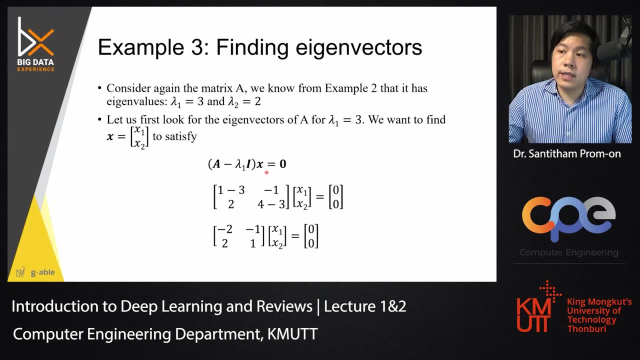 we can then determine the eigenvectors of this equation by substituting 3 and 2 into the equation 1.. So for that sense we have this: a minus lambda 1 i x equals 0. Lambda is 3.. Plug it in. 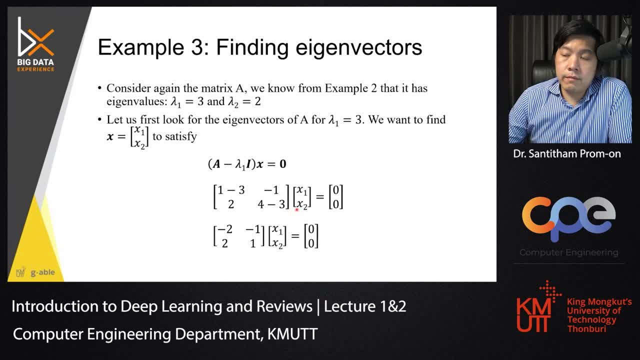 and then you get this: 1 minus 3 minus 1, x 1, 2, and 4 minus 3, and x 2.. This is minus 2 minus 1 x 1, minus 2, 1 x 2.. 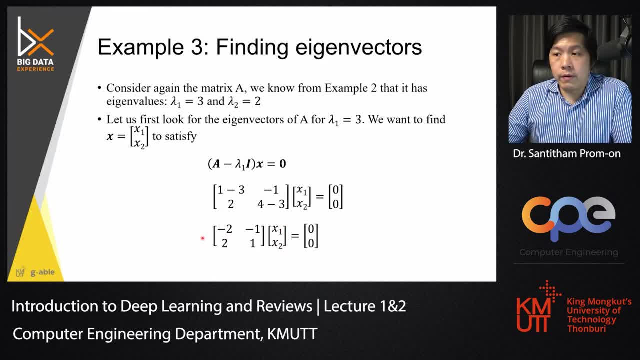 So you may wonder: well, they are the same equation anyway. right, It is minus 2 minus 1, and x 1 x 2.. When you multiply it in this way, you get minus 2 x 1, minus x 2 equals 0.. 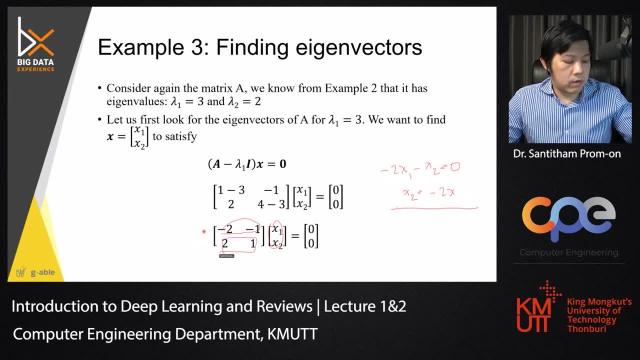 So that would mean x 2 equal minus 2 x 1. Or if you multiply it like this, you get 2 x 1 plus x 2 equals 0. So x 2 equal minus 2 x 1.. 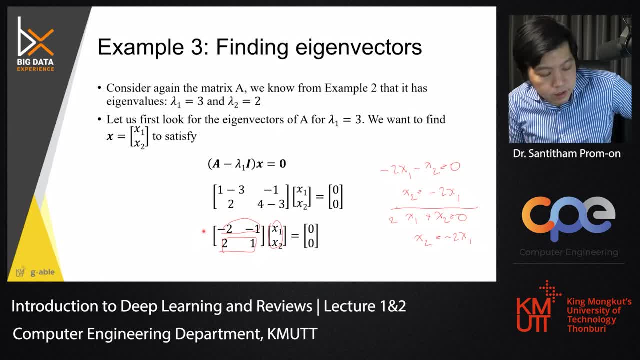 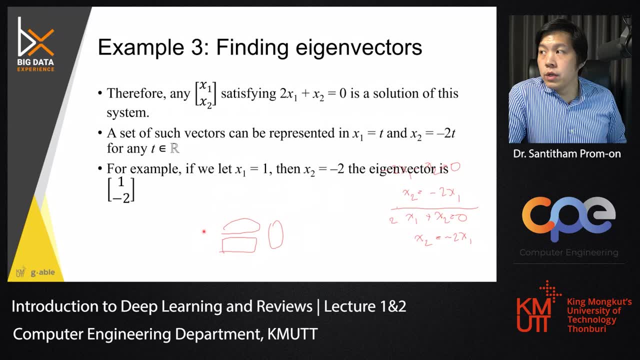 They are the same. So for this one it means that you have relationships between between x 1 and x 2.. You can make assumptions here. Suppose that you assume that x 1 equals 1, then x 2 would become minus 2.. 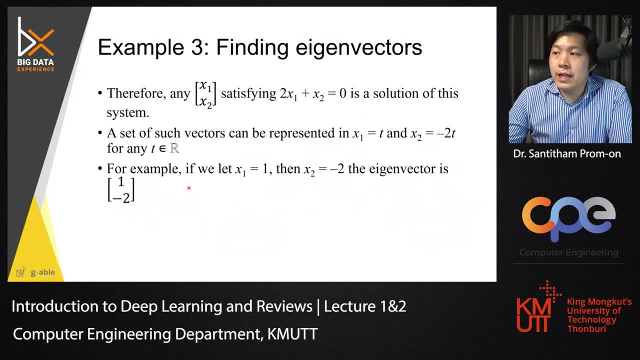 x 1 is 1, then x 2 become minus 2.. So that means you have eigenvector of 1 and minus 2.. Why can you make assumptions like this? The reason is because you need to multiply it with certain coefficient in any way. 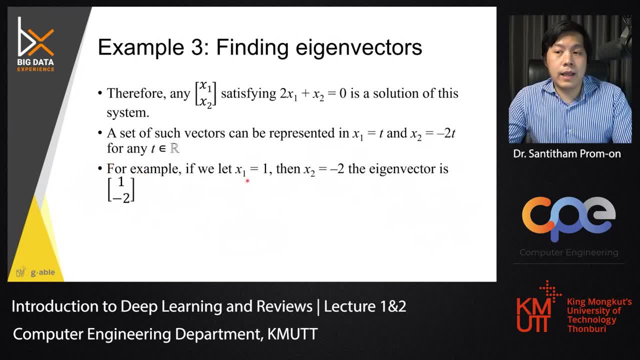 when you use it. So those scalar values multiplying with eigenvector it will scale it out. So you can just make assumptions that where one value is 1, then what would be another value here? Then you get this as minus 2.. 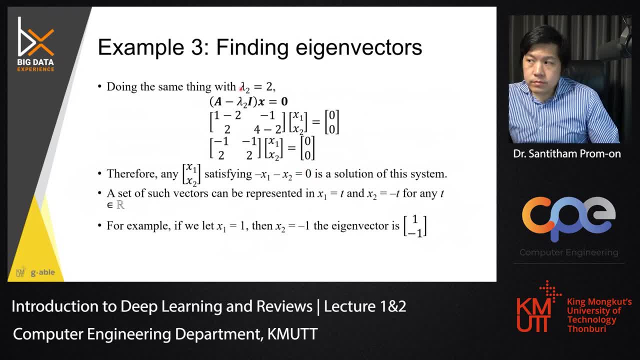 Let's find another one, Another eigenvector for this one can be found by substituting lambda 2, which is 2, into the equation 1.. Then we get 1 minus 2, and minus 1 is 4 minus 2.. 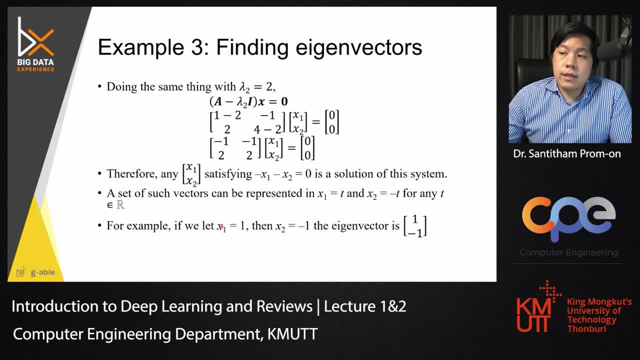 Then you get a relation like this one, which means that x 2 equal minus x 1.. If x 1 is 1, x 2 is minus 1.. So that means eigenvector is 1 and minus 1. 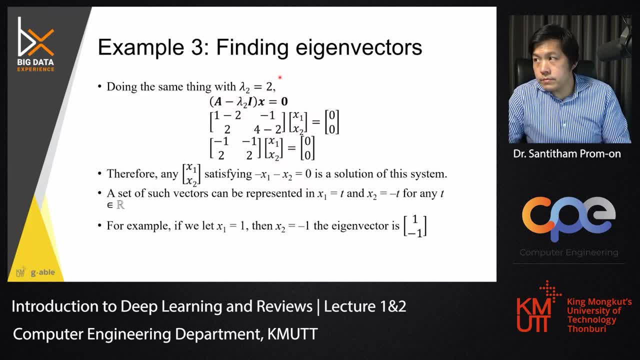 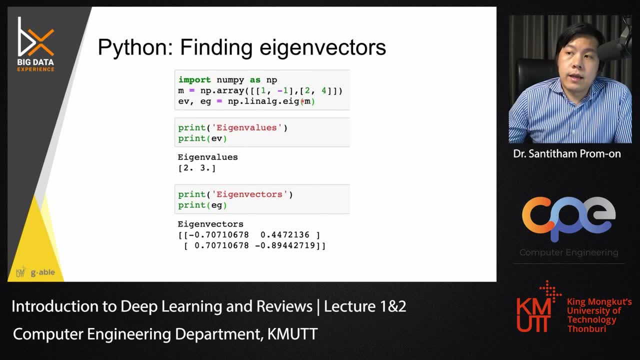 for the eigenvalue of 2.. You can use Python to solve the equation and find the acid Like the 1 minus 1 and 2, 4. using the EIG eigenvector decomposition you get eigenvalue of 2 and 3,. 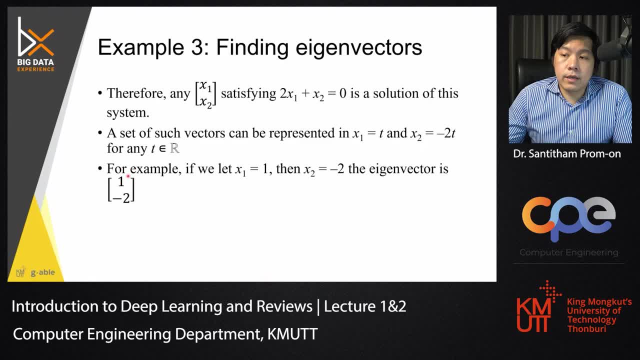 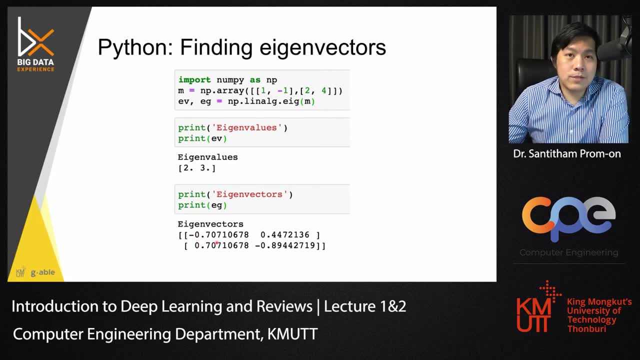 eigenvalue of 2 and 3, eigenvector of this. Now is my question: Well, we get 1 minus 2 and 1 and minus 1.. But when we use Python we get this minus 0.707. 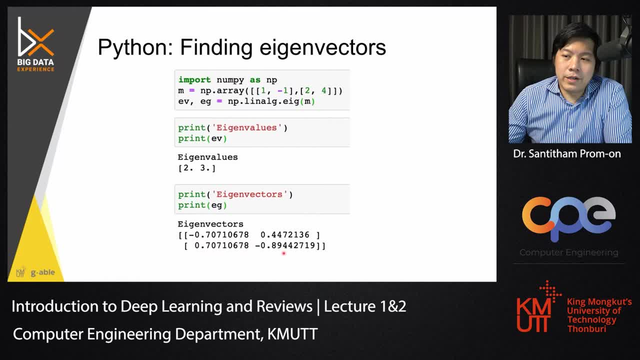 and 0.44 and 0.707 and minus 0.8 minus 0.. Oh sorry, We get this minus 0.707 and 0.707 and then this one minus 0.447 and 0.447. 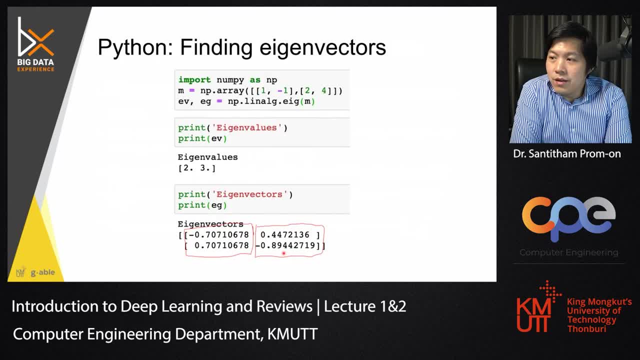 and minus 0.894.. Why not 1 minus 1 and 1 minus 2?? Can anyone answer this for me? Put it in the chat If you have question. what have I done here? So the technique known as PCA? 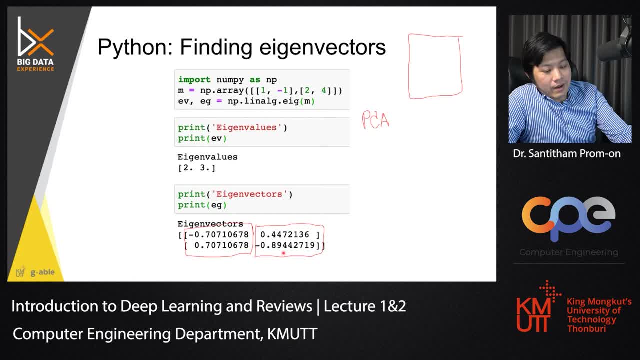 that I talk about require that you have like a tabular data. It usually reduce the data into principal component. When doing this, it need to calculate the covariance so that you have the square matrix And then from the square matrix it will perform the eigenvalue decomposition. 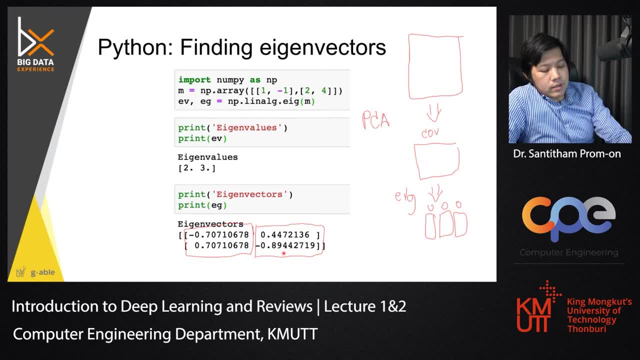 so that you have a set of eigenvalues and eigenvector according to that, And then principal component is actually the projection of the data. here with this eigenvector, Right Y minus 1 and 1.. Oh sorry, Y minus 0.7 and 0.7. 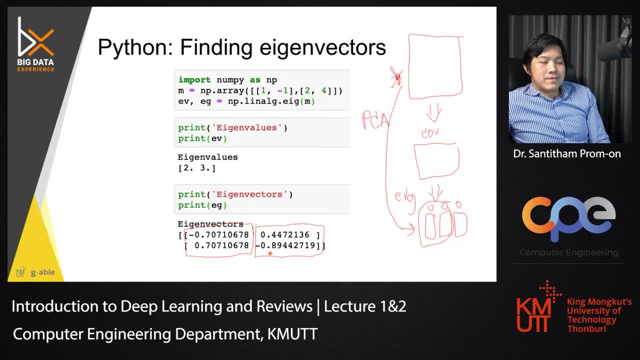 and 0.4 and minus 0.8.. Are you still there? Please answer, so that I will know that I'm not alone here. Why is that? Make a guess. Why do you think this is the case? Any idea? 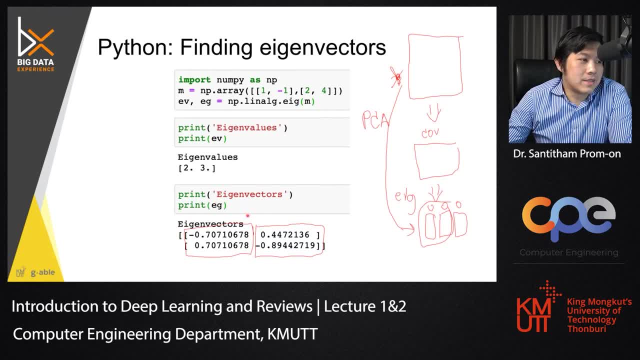 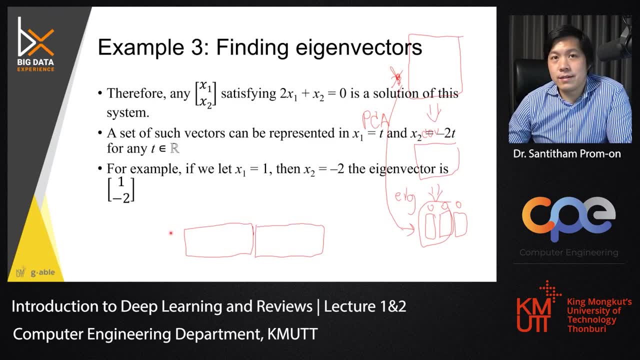 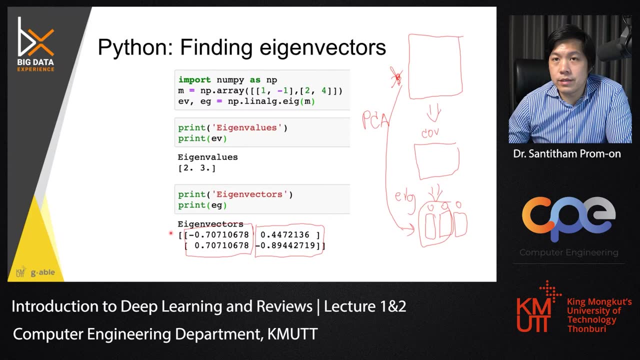 Correct Unit vector, Just because the function here would give you the unit vector. So this is the unit eigenvector. It doesn't matter, because whether it is just 1 minus 1,, 1 minus 2, or the eigenvector, 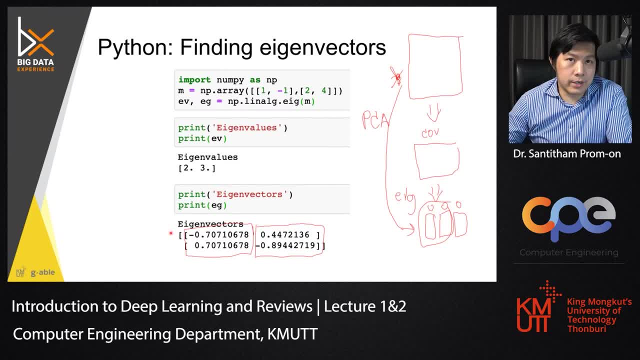 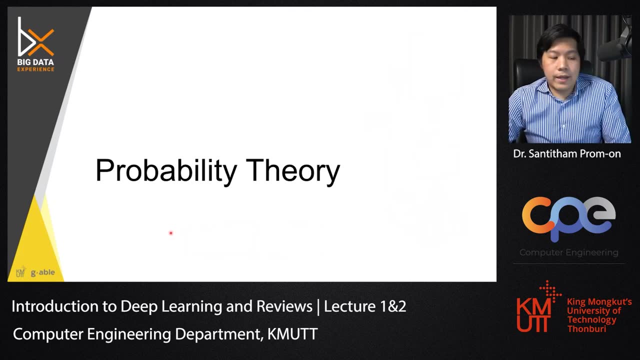 unit eigenvector. they are still on the same direction And when using with PCA, using with other techniques, directions matters more than the scaling values. Okay, Correct, Right. So yeah, These are still the review, Don't worry. 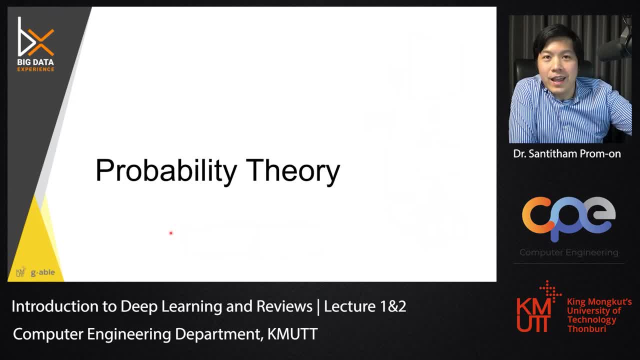 When go to the deep learning, you will definitely have to use them. Now you have to worry. You pick up the book. Come on, If you pick up the book and go to like chapter 2, you will find them here- All about vector decomposition. 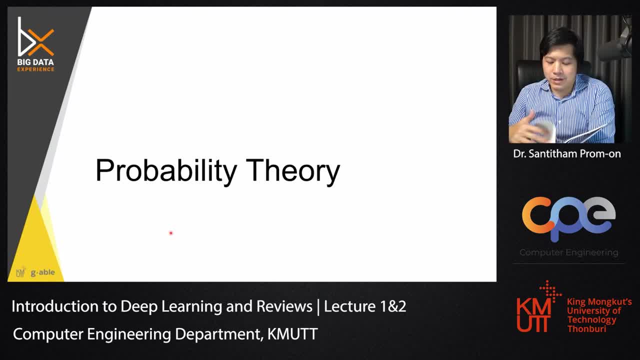 about what I'm talking about, with assumption that you have already known. You have already known certain concepts, So I'll try to kind of digest that into like a simpler version. Hopefully, Yeah, hopefully that's the case. Okay, Now the last topics. 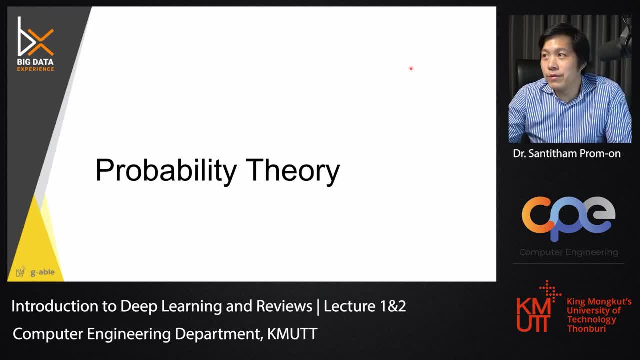 Let's take a break. I know it's quite a lot in terms of the review. Let's take 5 minutes break and 808.. We will resume on the probability theory Break. 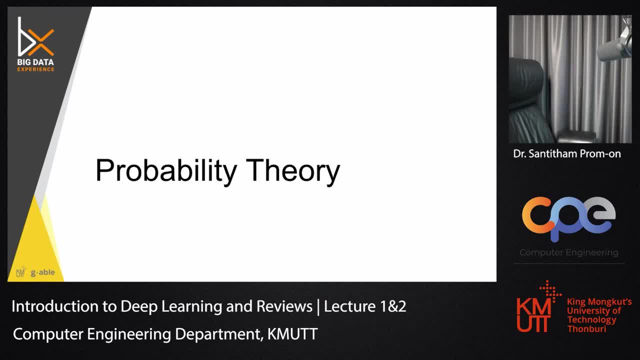 This year there are not many people in the club because the first time, the first time, they were late for the exam. They sat in the same place, They were late for the exam, so they went to the same club. When I called them, they said: let's try shopping first. 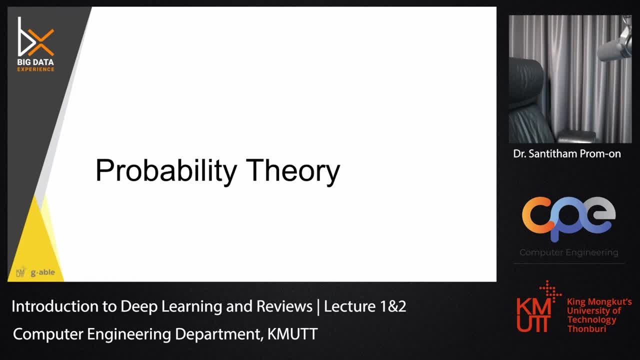 The first time. Let's try shopping. Let's sit in the same place. How was it? At first I wasn't feeling good. Then I went to the same club, then I was late for the exam, But now I'm good. 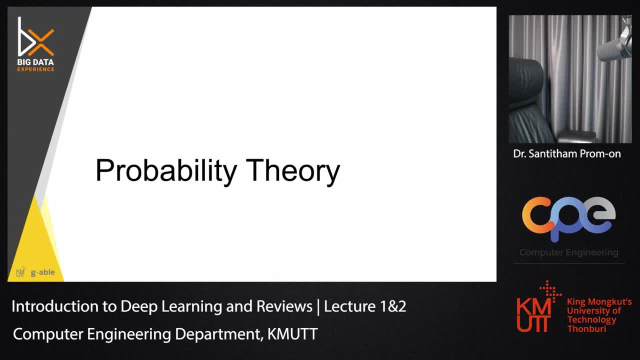 So this year it's better. I'm here for the exam then the second time. Now I'm in the same place as the first time. I'm lucky. There are 9 people in the club. I'm lucky. Are you ready for the exam? 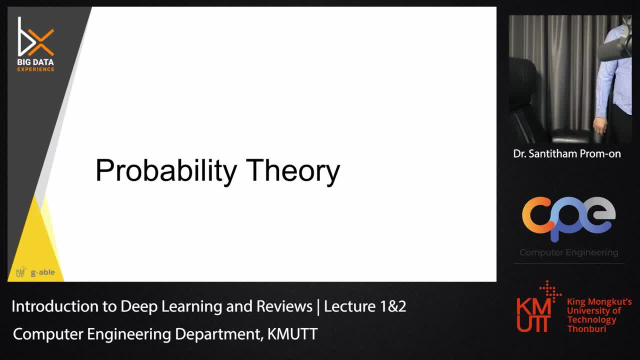 Yes, this year I need to know more about the club And I want to know what kind of club are my friends? They must be in good condition. Do you want to eat? How is it? It's very hot, But it's delicious. 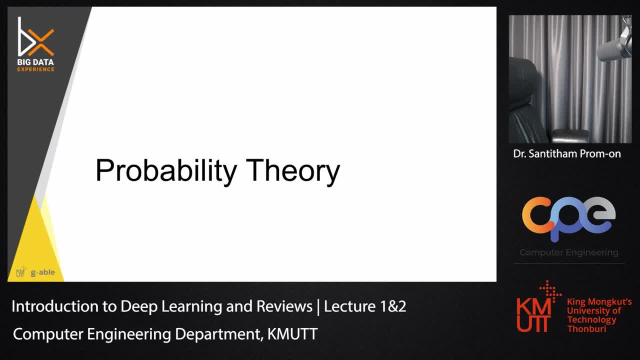 It's delicious, isn't it? Yes, it's delicious. I can't see the time I have to turn off the camera. Turn off the camera. It's 8.08 pm. 2 minutes left. 20 seconds left. 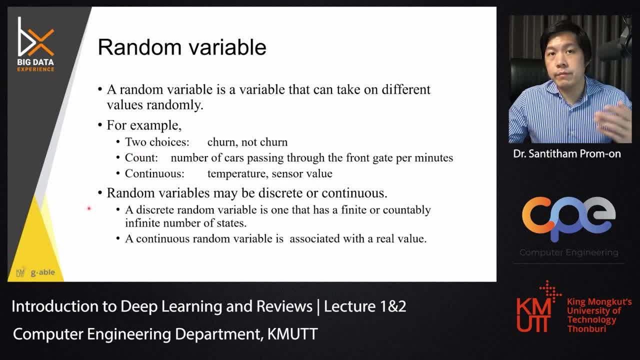 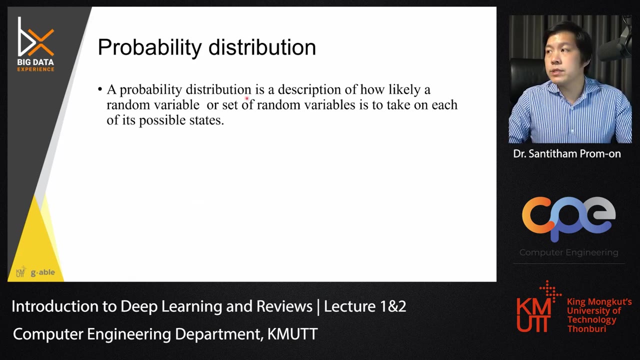 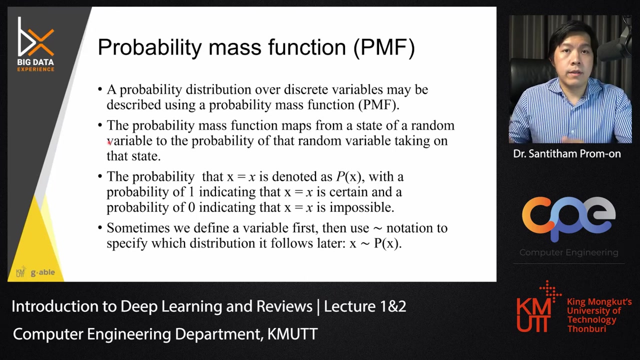 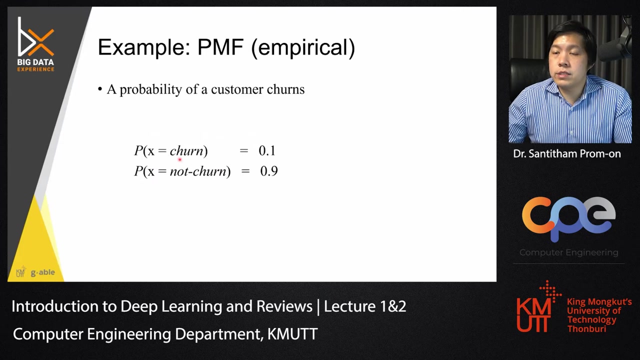 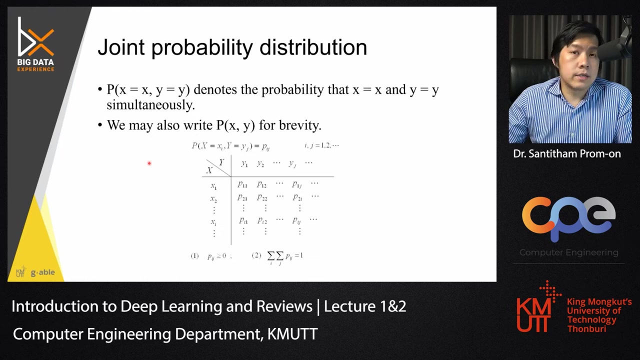 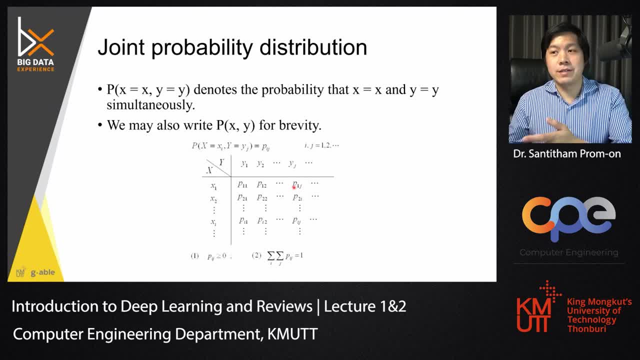 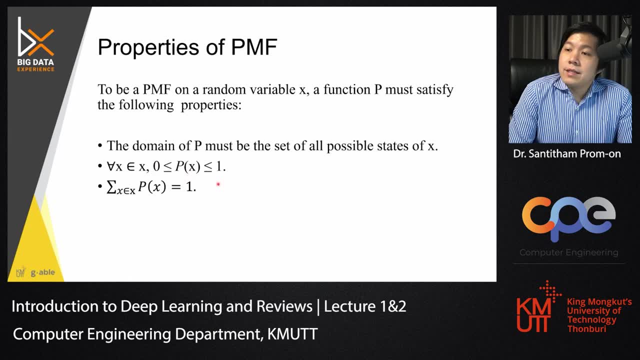 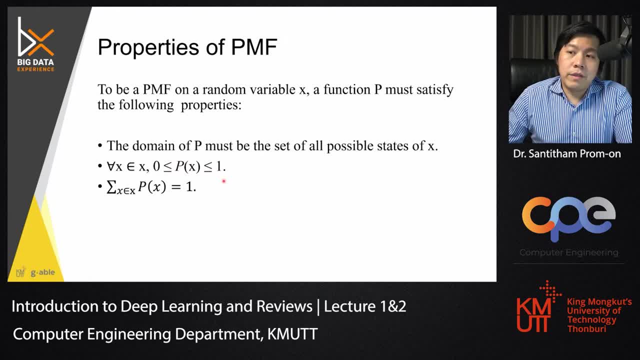 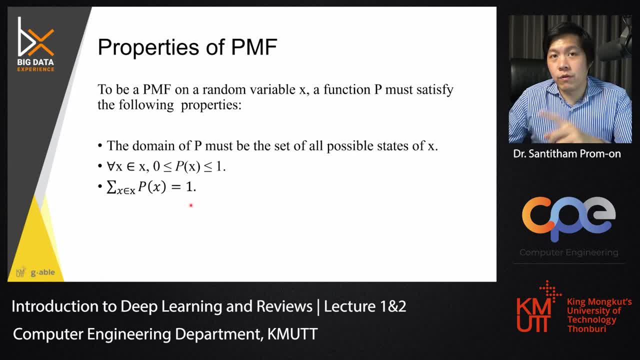 Thank you for watching the value of all of the combinations. you get value of 1.. That is the universe. The probability of the universe is 1.. Just like the thing that you learn in your statistics and probably in your undergrad degree. 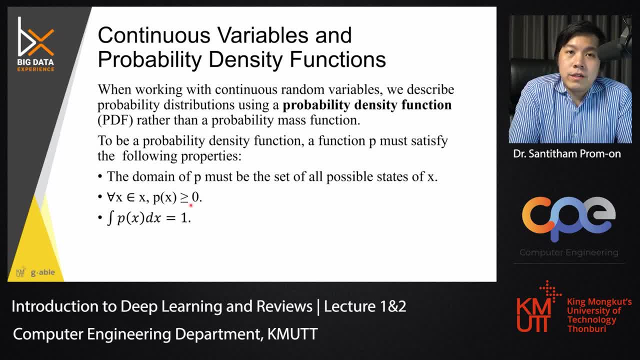 This is for the discrete variables. For the continuous variables, instead of calling it probability mass function, it's called probability density function. They are similar, Though this one would be continuous. That means value of px. px. value of probability would be more than 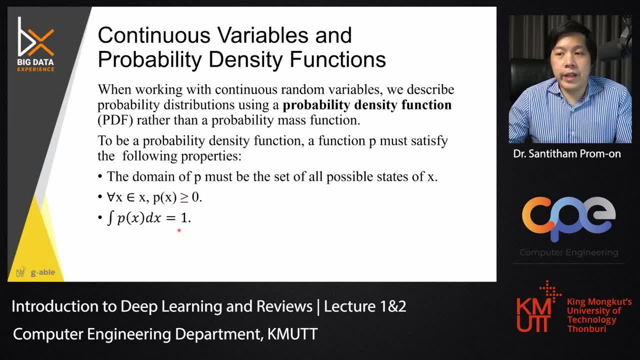 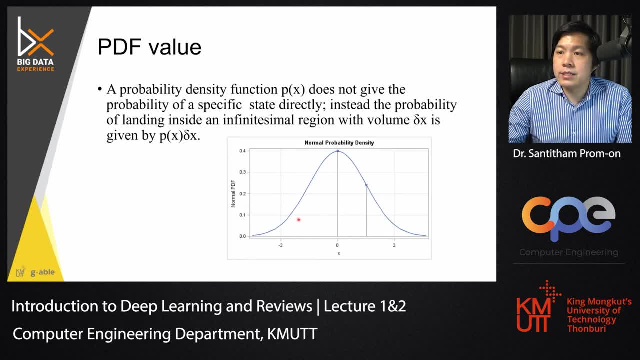 0. But instead of summation, if you integrate the density function, you get value of 1.. Examples of probability density function. pdf is the normal distribution. It looks like this one. This is the standard normal distribution, If you. 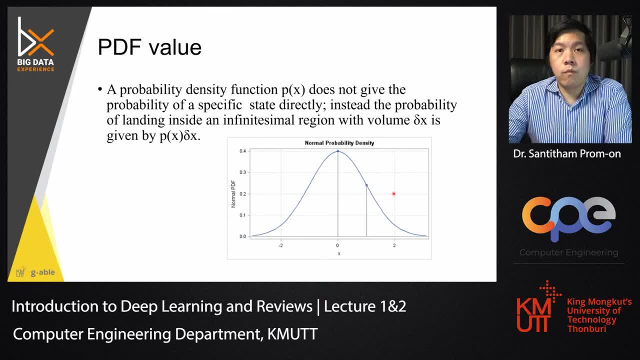 integrate the standard normal distribution, you get the value of 1.. This is the whole probability. You can find the probability of that occurring from a certain region. When you take one value out of the pdf, you are actually getting px, delta x. That means you are getting just one value here. 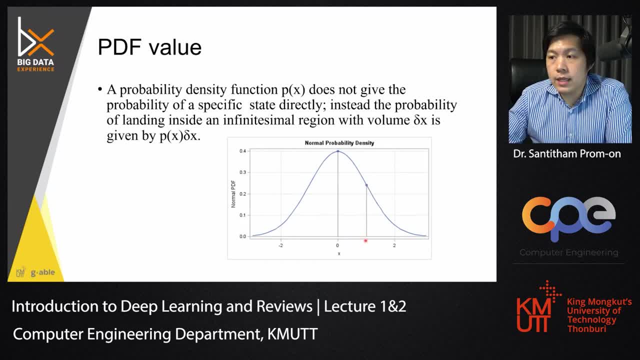 out of this. This is like the chance that this value would happen when you take it out of the distribution, But usually in the continuous value sense. getting just one slice of value is difficult, because 2.0 and 2.1 is not equal. 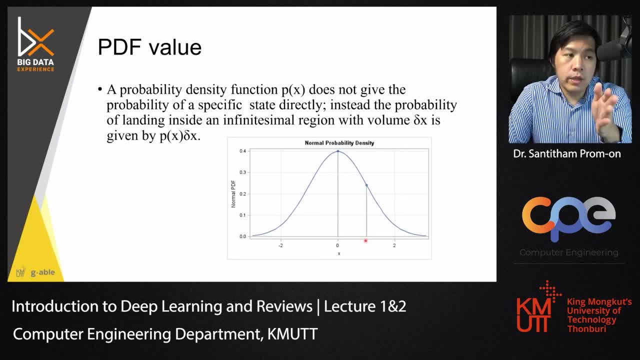 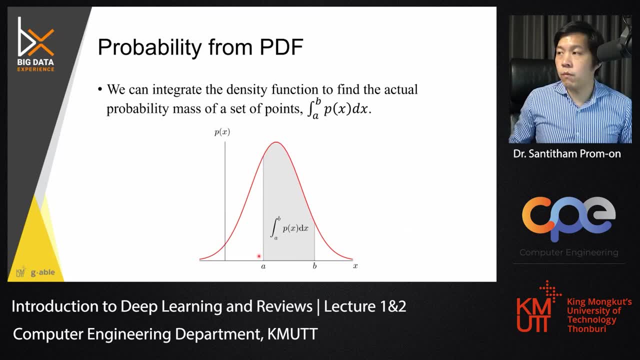 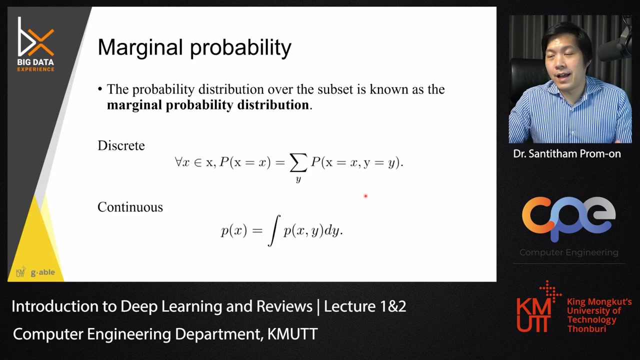 So finding probability at 2.0 is not close to 2.1.. Instead of that, we can find the probability of the range of value by integrating the area under the curve of the pdf, and then you will obtain the probability. So this is like how you obtain the probability from pdf. 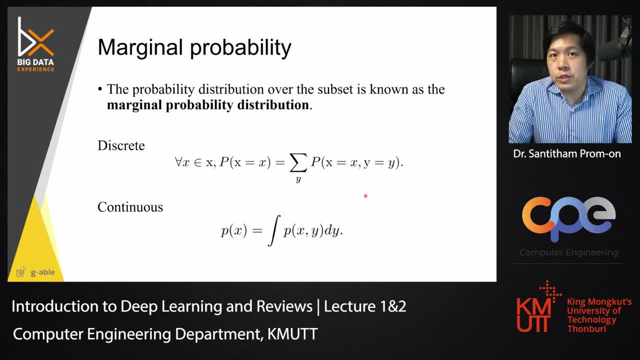 There is a probability when you have the joint distribution. if you were to eliminate one axis out, we would call this amount. This is the probability distribution, The size of the probability distribution of the system. You can see that u x is equal to u and u z is equal to u and u z x is equal to u. 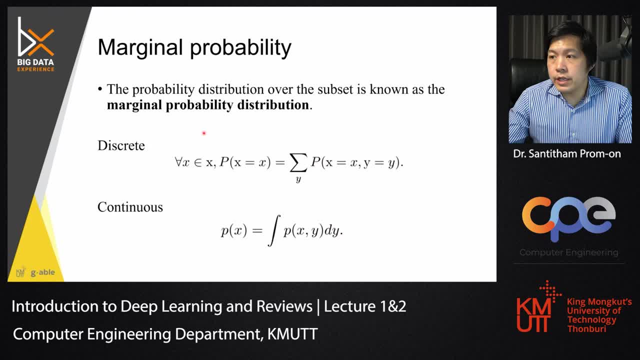 So when you consider one variable, a marginal probability distribution, it means that you are considering just one variable at a time. This is called a marginalization process. That is your kind of summation of all probability on one axis, integrating by one axis. This marginalization is used a lot in the Bayesian statistics. 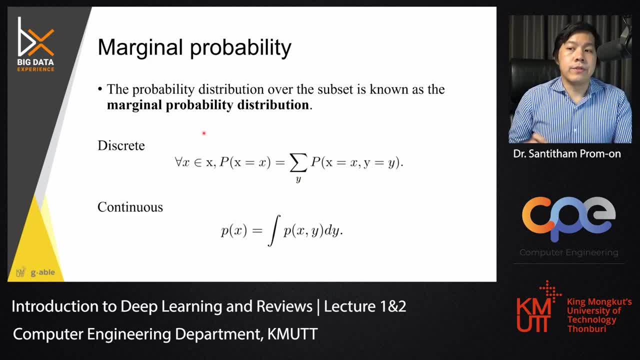 So if we do something like Bayesian belief network or the Bayesian worship approach ratio of the population, this is not going to work. Bayesian deep learning types: you probably encountering this marginalization process, But for us, luckily, we will not begin with those that will be a little bit more advanced. 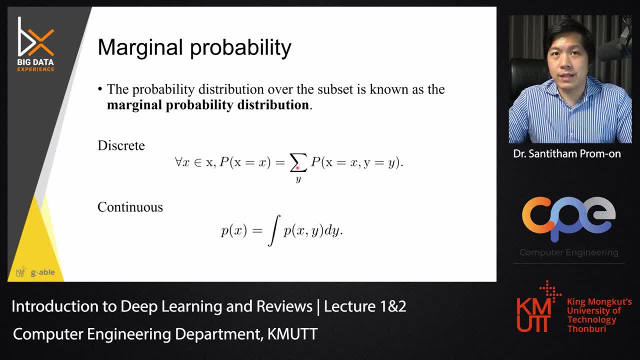 So this is supposed to be a process called marginalization, or eliminating one axis out of the distribution. then you get like, like, if you think about, think about something like going to university marginalization, you know that university is on the plane, right. 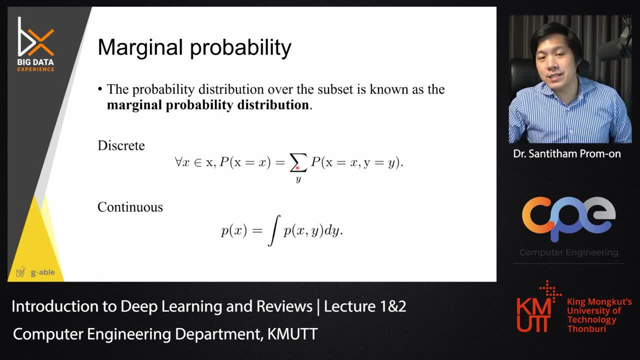 So it has x and y. marginalization is like the process of viewing the university from the front. then you are eliminating the depth because you are seeing just from the front. So it means that in computer graphic- computer graphics are we're marginalized one axis. 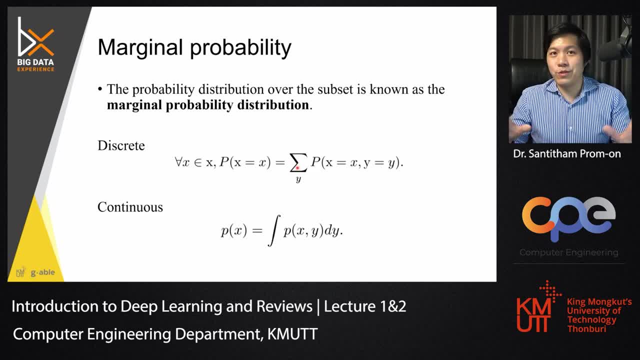 so that you can perceive it as two dimension. I don't know if this would exist- I can't explain things better or not- But yeah, the marginal probability distribution will, the same way that is supposed to have joy distribution. you want to know just how much it would change in how much thing would? 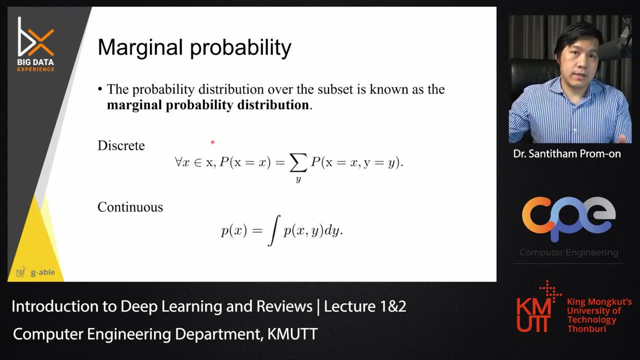 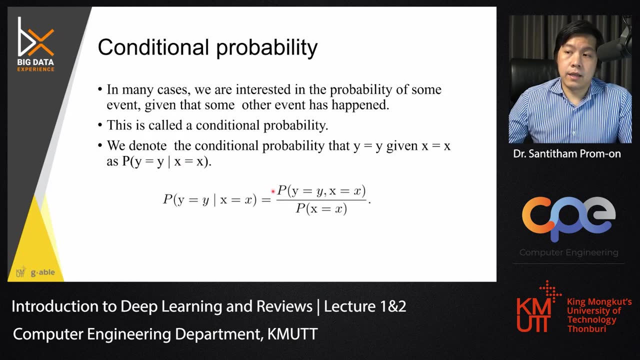 happen in one direction. you can marginalize the author out and then get just one axis right. This one is: will be p, x equal x, the, and then you just marginalized y by summing them. then you get the pop of x equal x would happen. 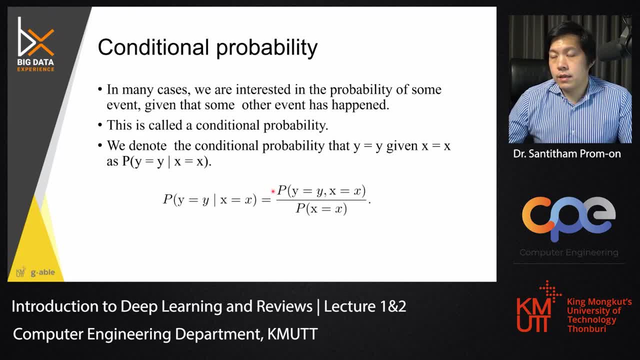 Okay, So those are the basic probability. then we now move on to a little bit more concept on probability theory. This is called a conditional probability. Conditional probability is the probability of certain events, given that you know that certain thing happens, given that certain condition happens. 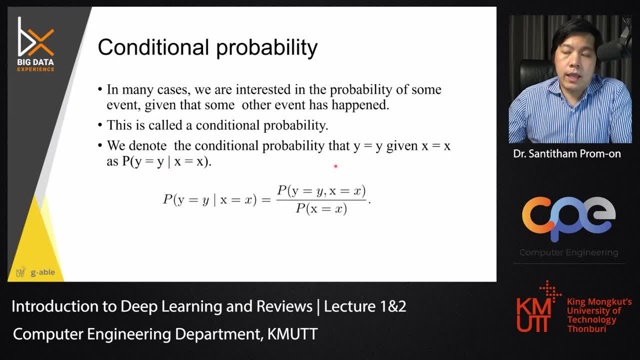 So this is like p x. This is like p y equal y, given x equal x. This comes from the joy distribution of y and x divided by. you know that x happen like p x equal x. This can be explained in in easier in the set term. 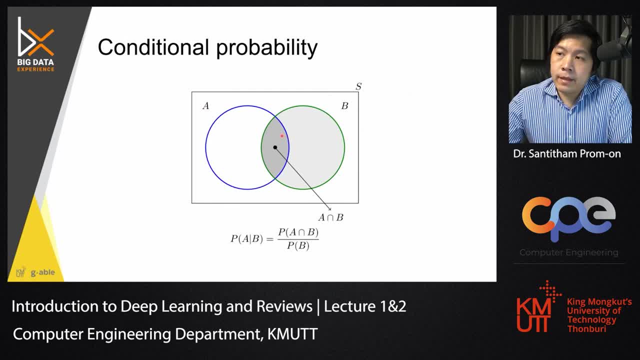 So let's look at this, this Venn diagram. In this Venn diagram you have a and b. If we talk about just p of a, p of a would be the proportion of a divided by the whole thing. right, The proportion of a divided by the whole thing. 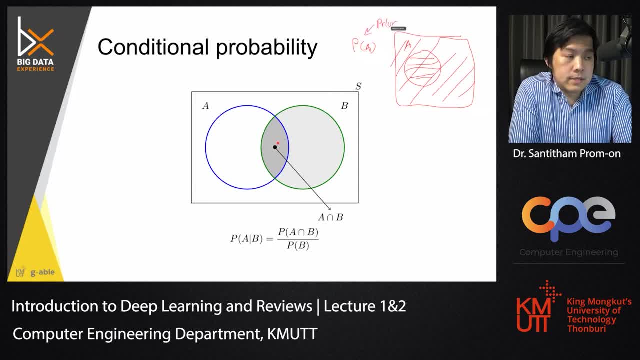 This is p of a, all the chance that a would happen. Sometimes we would call this a prior, pop The prior. Okay Now, p a given b. what is it? P a given b is still a p of a, but you know that b happens. 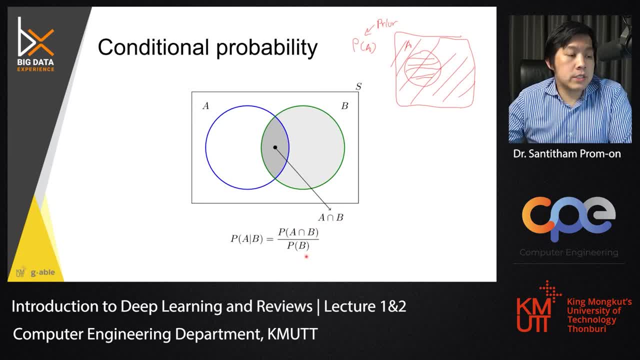 So when you know that b happens, you are trying to find the joy distribution of p a intersect b, which is the intersection between a and b divided by p b. What is p b? Think about p b as the area of b here. 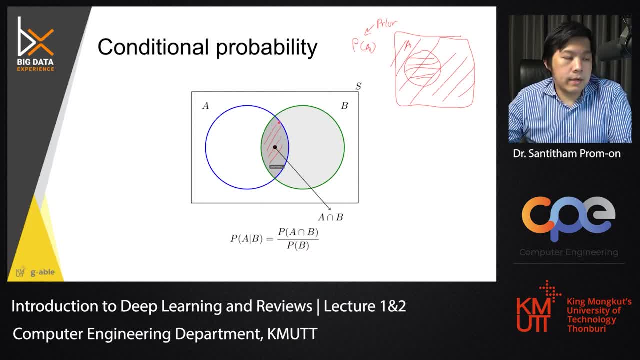 So you are taking the area of a. Okay, Dividing by the area of a intersect b, dividing by the area of b. So what you end up with would be the proportion of a that is in b, right. So this is the conditional probability. 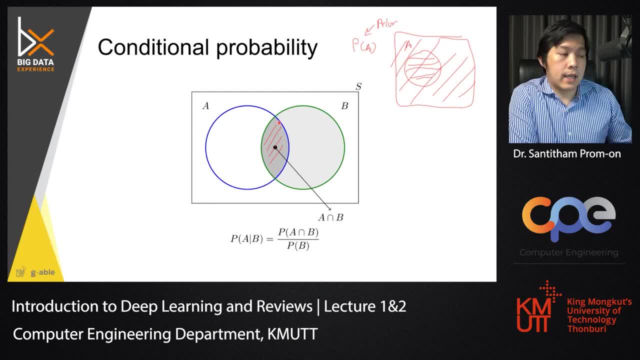 Conditional probability can be used in the latter sense that we will talk about prediction, that you want to predict even a occurring, given that you have certain data, You have the model And then compare that with the prior and then you will see whether your prediction 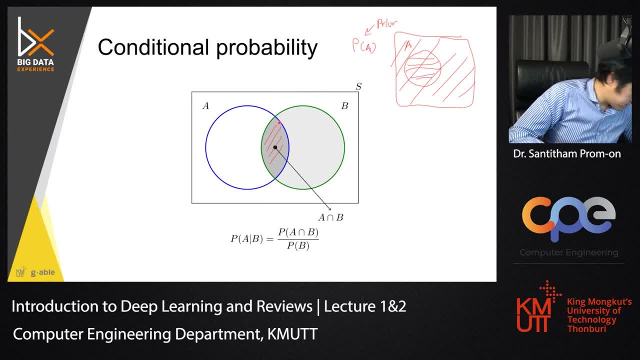 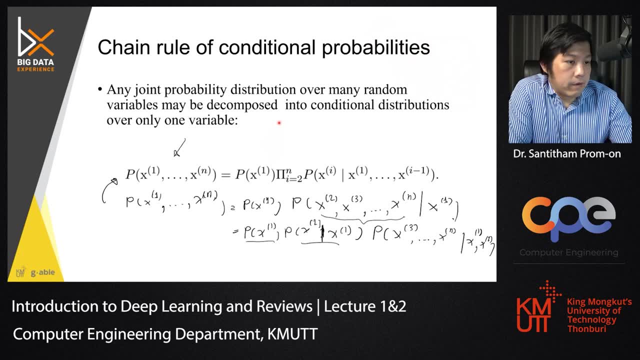 is better than the prior, or not? Okay, So here is the definition of conditional probability. Okay, Conditional probability has the chain rule. Okay, I did not erase it out here because I don't want to write it again, So this is the chain rule. 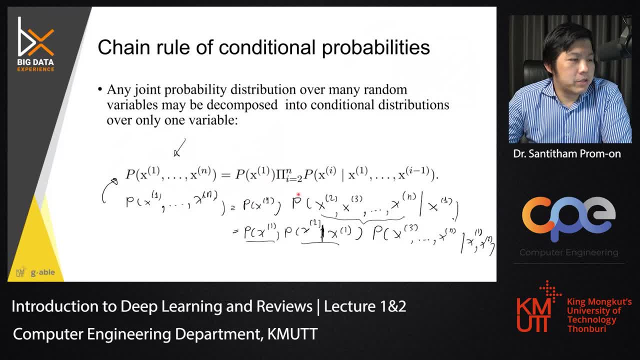 Okay, Conditional probability. So you have this joint distribution. You can take one out, You can take one out, take one prior out and then you will get the multiplication of the conditional pop of the rest of that event. i given the rest. 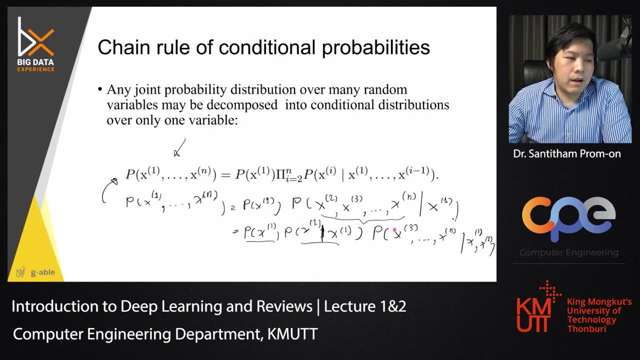 If you take another prior out, you get like p of x2 given x1. And then And then the conditional pop of the x3 to xn and then x1 and x2.. So these are like the basis of Bayesian theory and Bayesian network. 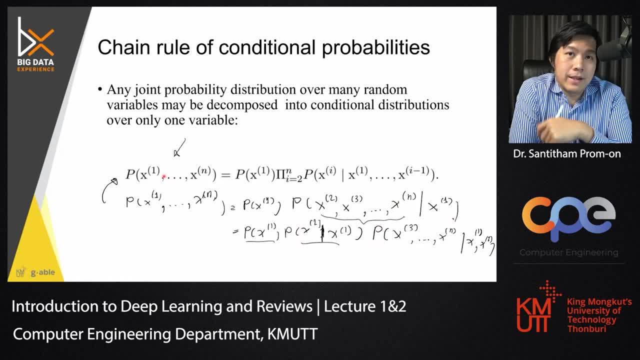 Seeing math like this might scare you, So let me explain it in terms of the table. For this one, this is like a table with n column, An n column table, An n column table. if you were to store it as 0 and 1,, you have the total combination. 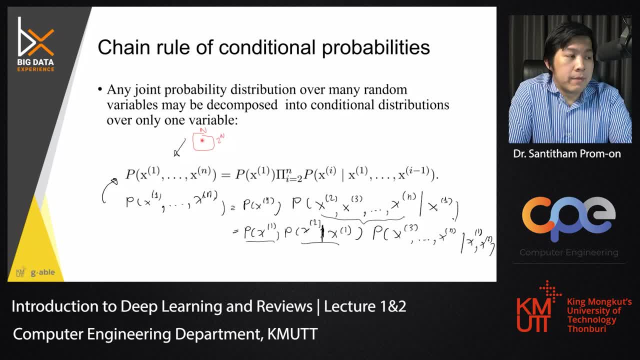 of 2 to the n right. That means this table will be quite large. if you want to store all of the combination of these variables, However, think about this table. Just one variable right, P x1.. Suppose that you have 0 and 1.. 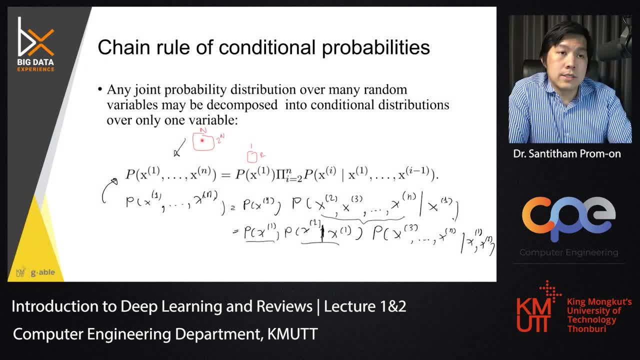 Then this is just the size of 2.. 2 to the 1 is 1. And this table will be the size of 2 to the i minus 1.. So it means that you are taking, when you take it off here, you represent, you reduce. 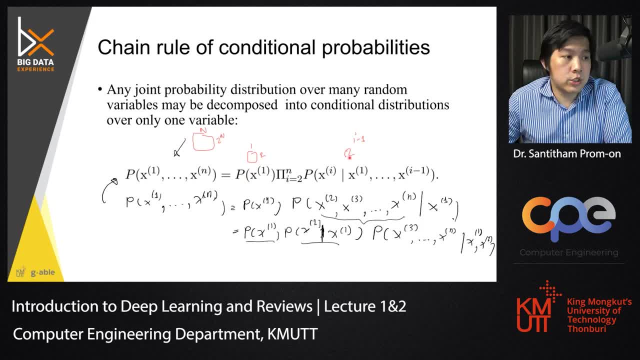 the number of or the size of the table that you need to store 2 times Instead of having the 2 to the n table. So you have this 2 and 2 to the n minus 1, which is a lot less than 2 to the n right. 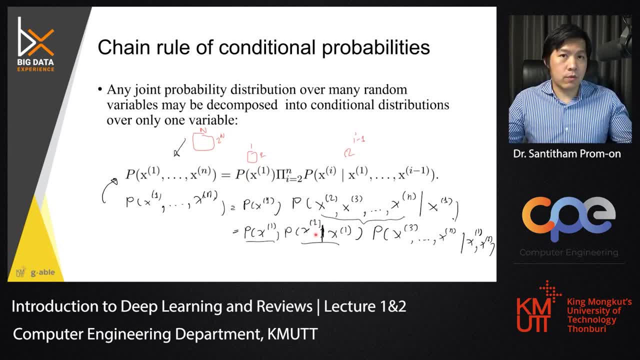 So the number of data, the size of table, that you need to store, is quite reduced. quite a lot Bayesian relies on this concept to decompose the joy distribution into multiple dependency of the table. So instead of storing a large joy distribution table, it's stored just like a piece of fact. 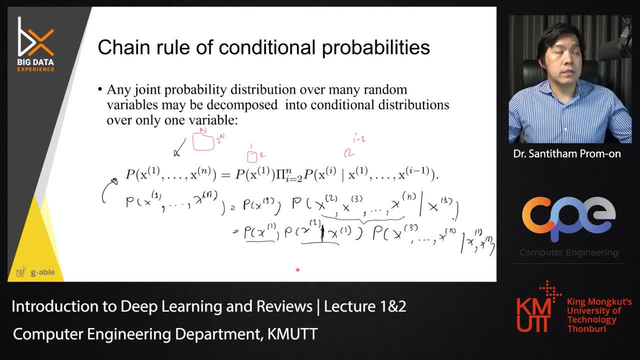 that suppose like seeing high temperature and having a lot of data. So you have this 2 and 2 to the n minus 1.. Bet you've taken a guess from what Bayesian is saying today And if you had a good idea- better gift than great joke- you give it to me in the comments. 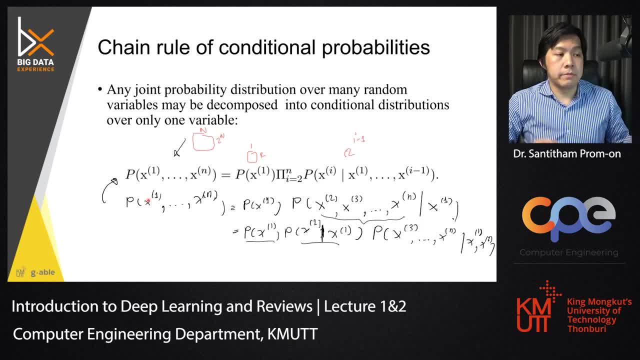 below uh-huh. So now if i asked you to do something, you can actually say kind of USA-ombudsman, move slash, come back to bYE as ateil to have higher value And then say: what do I really want? if you study Bayesian, come back to this concept and review it again. It will help. 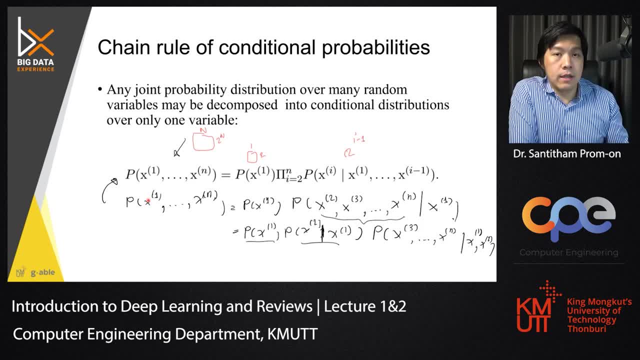 For us in this course. we are not doing the Bayesian inference or the Bayesian technique in detail yet, So this is just a review at this time. In the advanced deep learning technique there are techniques that combine the Bayesian inference with the deep learning, Because deep 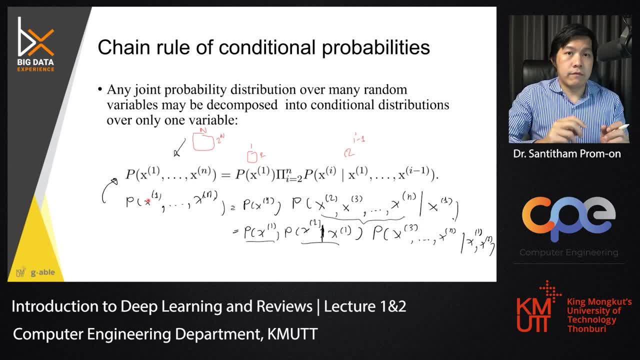 learning relies on calculation of the patterns. But if you want to make inference sometimes you need to kind of encapsulate deep learning model with the Bayesian inference And it will allow you to kind of doing the reasoning If you are, if you want to study about this more. 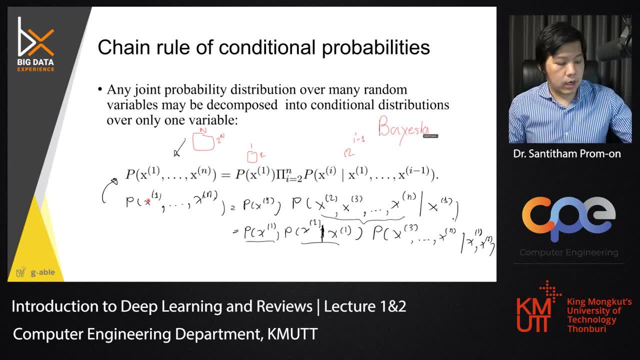 about inferencing reasoning. I would suggest the topics of Bayesian network. Try to study that topic. It's not difficult, Although mathematical is quite scary. but it's not difficult, Although mathematical is quite scary. But the in terms of data is actually quite simple. Just some table and then you just multiply table. 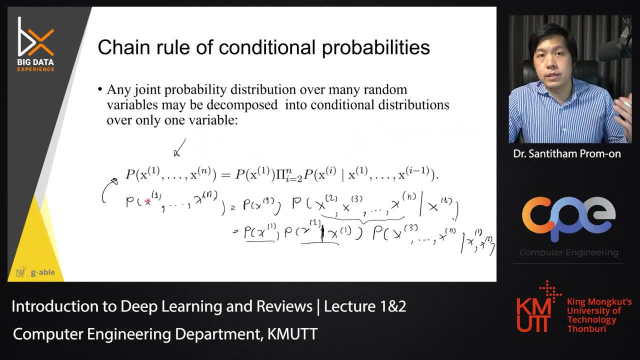 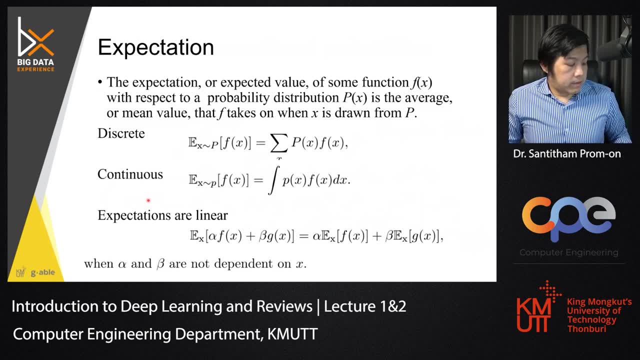 together in the end, Right, But? but the derivation of the technique is quite complicated though, Right. So next topic would be the expected value. We call the expectation of the of some random variable. some function as the multiplicative expression of the error. So expected value would be the multiplication of the probability and the 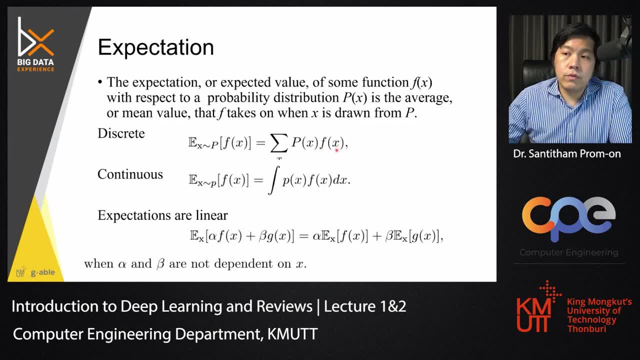 random variable. Fx is the random variable or the function that produce value, And Px is the probability of that one. So expected value in discrete sense is summation of P and the. so the chance, Px is the chance that thing happened and the outcome. 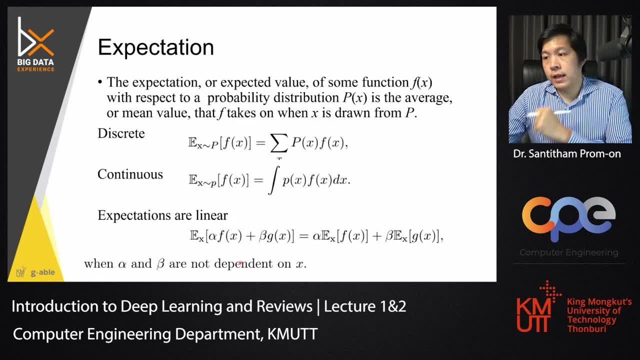 probability and the value. So this is expected value. Expected value has linear property, That is, you can find expected value of a formula of the combination as the combination of the expected value. So basically, if you add these two populations together, each has its own expected value. 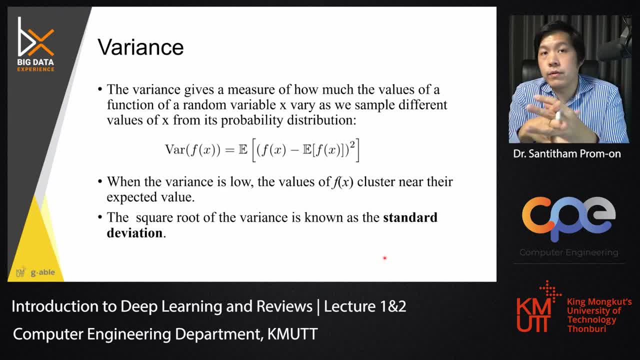 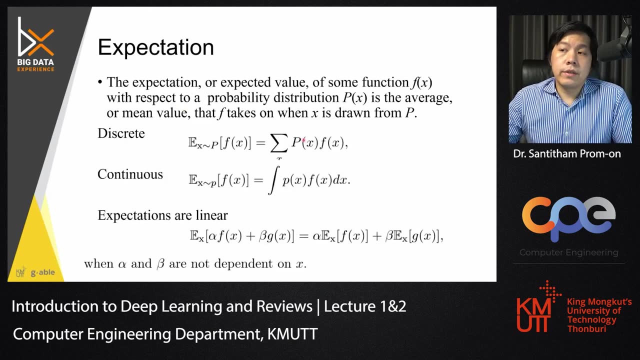 the combination of the population will be getting expected value and add them together, That is expected value. Now, if we talk about the expected value at the order of two, this is the variance. You can think of variance as expected value measures, something like the centrality of. 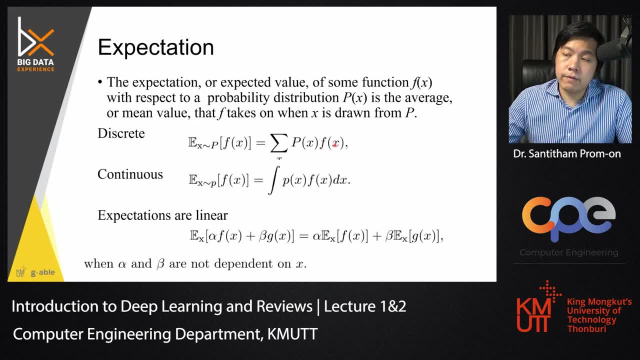 the distribution, Because you are multiplying the chance of things happen with the value. then you get the kind of estimate Of the mean, the mean of the distribution, the mean of the value of that distribution, Like if you have a chance that a customer would buy things by 0.1, not buy by 0.9.. 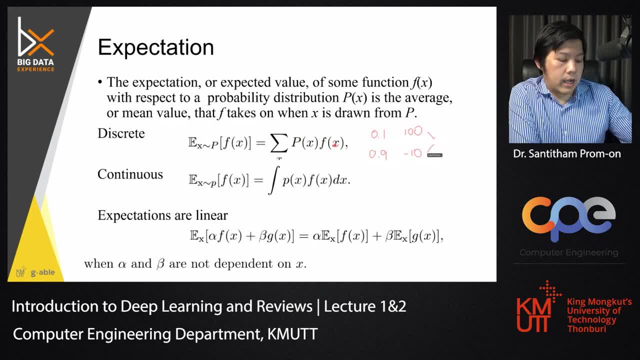 If customer buy your product, then you get 100 baht. If not, then you lose minus 10 baht. Then in combination the expected value would be 0.1 times 100.. And minus 0.1 times 100.. 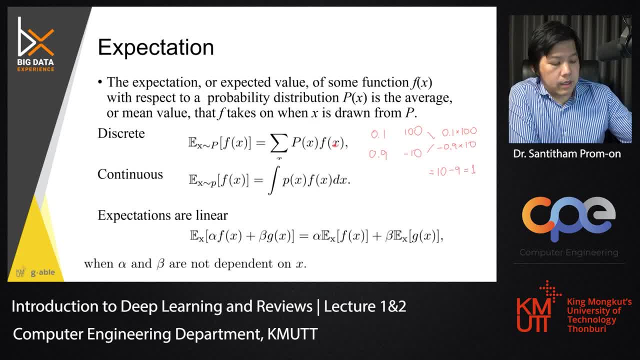 And minus 0.9 times 10.. And this would be equal to 10 minus 9 equals 1.. That means the expected value is 1.. So you can expect to get a profit of 1 baht per customer. So this is the expected value. 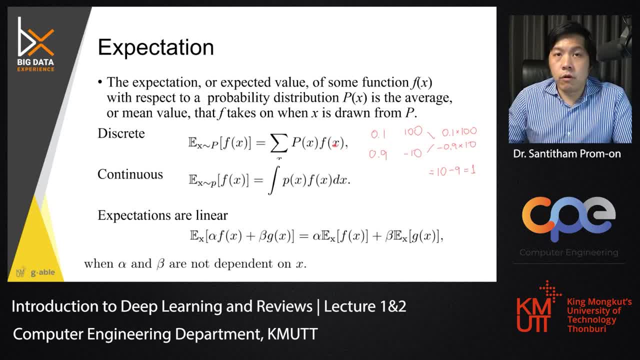 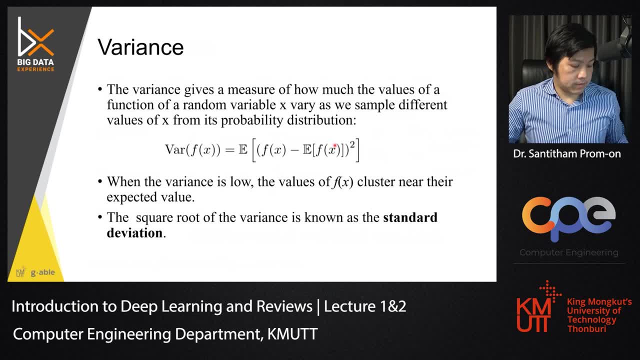 This can be applied in many sense. You can apply it to the result of the model. You can see that the technique also derive. many of them derive based on the expected values. Thank you Now, well, you know. mean then next must be the variance. to measure the variations. 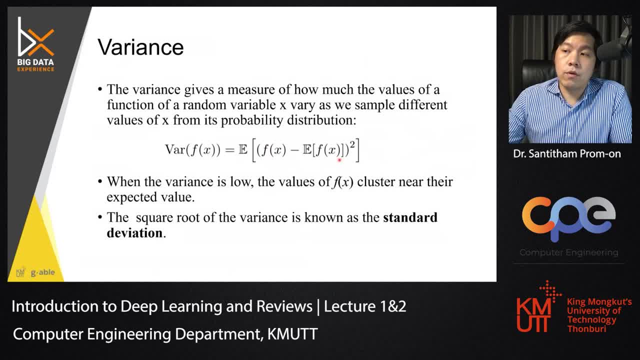 of data Variance is actually the expected value of the difference between the value itself and the expected value and the mean. So you are trying to find the expected value of the difference, square the size of the difference And this is called variance. 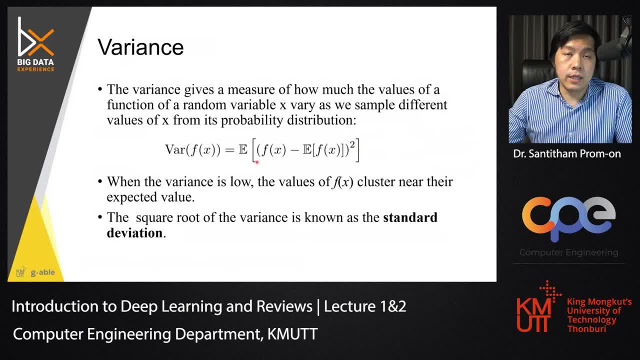 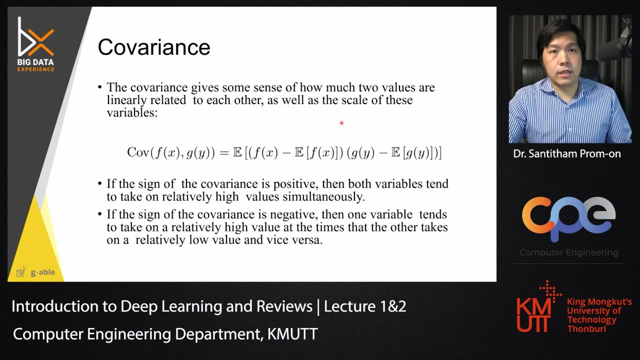 If variance is low, it means that F is closer to E. The cluster is tight. If variance is high, then it means that F is farther from the mean. So if you take the square root of variance, then you get standard deviation, as in the. 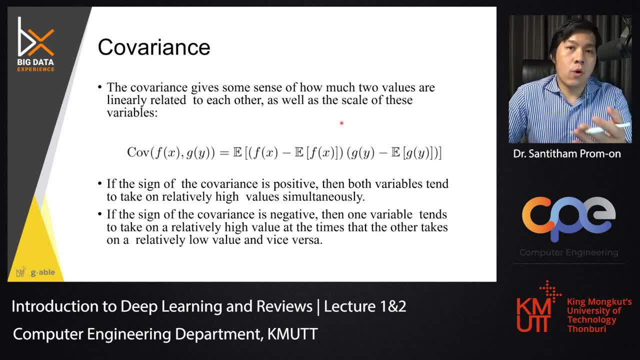 statistics And the terms covariance refers to finding variance of two things together. So covariance of function Fx and g, And the term covariance refers to finding variance of two things together. So covariance of function Fx and g, g, y of two variables is taking the expected value of comparing in one axis, f, x, to. 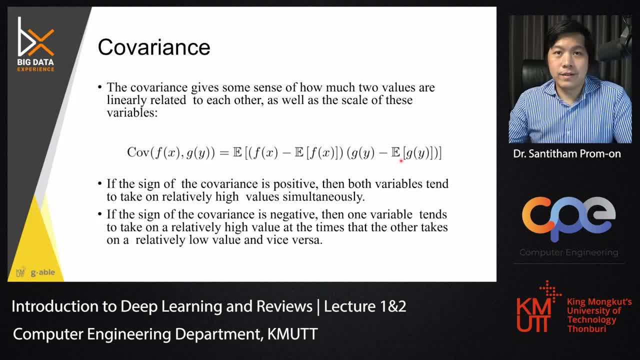 to e of f x and g y to e of g y. looking at this way you might. so for this one covariance would measure whether they goes in the same direction. for example, if the value go in the same direction like x and y, high value of x would pair with high. 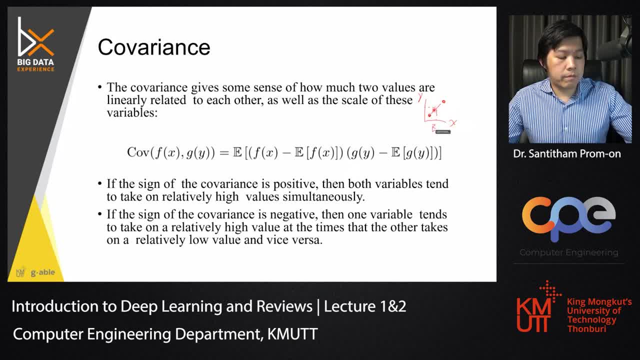 value of y. lower value of x would pair with lower value of y. that would mean, if this is the mean of x and mean of y, ignore g and for the moment, then you get a value here. if f is more than mean and y is more than mean, then you get a value of x and y. 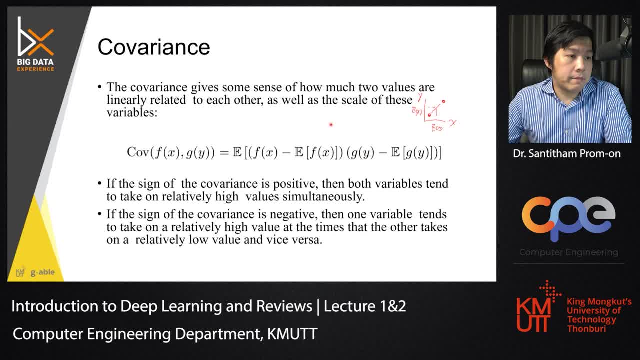 multiply them, you get positive value. if x less than mean, y less than mean, multiply them, you get positive value. right, so this is like an average of the the difference. uh, so so you can estimate whether they are co-vary together or not, or whether they are negatively co-vary with one. 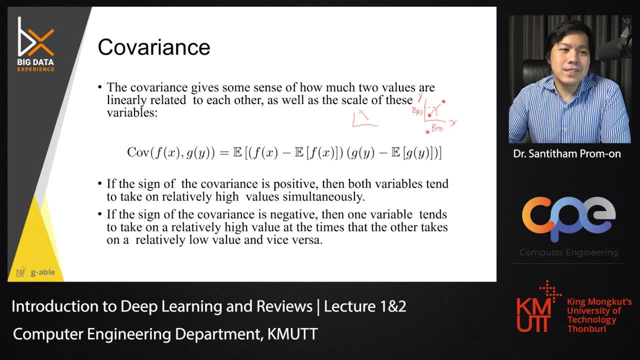 another right, this is covariance. you can see that this is like correlation actually actually is covariance in the normalized way, right? so correlation is actually measuring covariance divided by the norm of the vector in x and y axis, and then you get correlation. you can see that it's kind of tracing the root coming from the same stem. 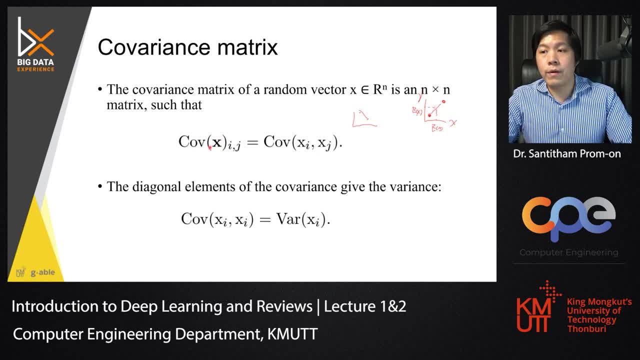 covariance can be compute to get the covariant matrix, the covariance of of x, of the matrix x. suppose that you have the matrix of multiple column, multiple, sorry, multiple- column. then the coherent matrix is the covariance of each column, right? so it's like the covariance of each column. 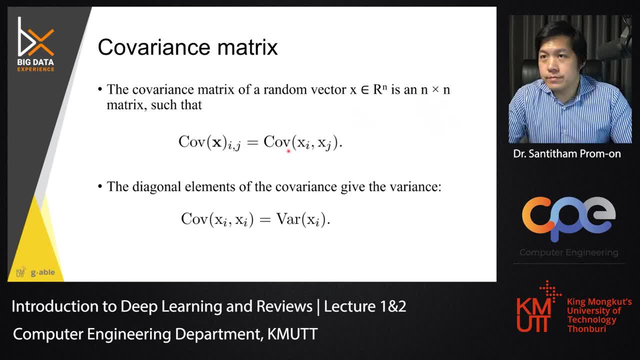 and the diagonal will be variance value, right? so this is the basic concept of probability. that well, we will use them time and times and you can see that learning, machine learning would require to definitely get into this probability theory and statistics. in any case, use it every day. 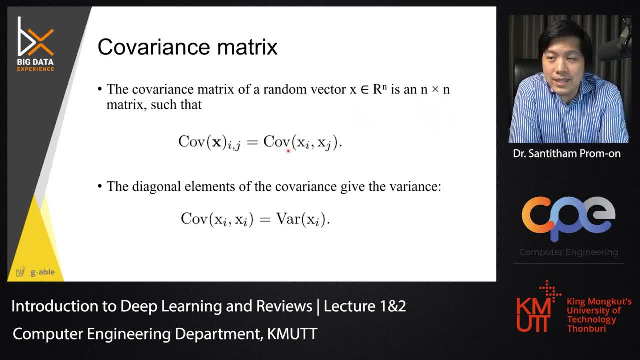 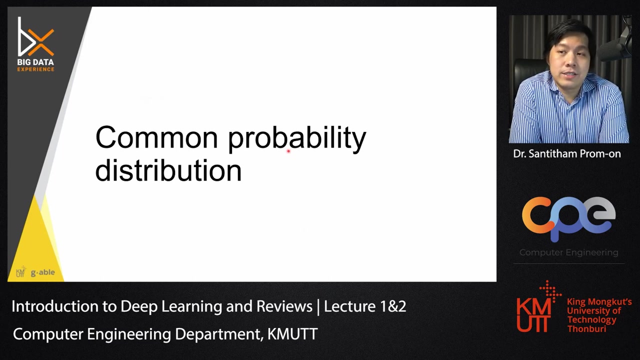 actually i just post something about statistics like a test of virus, right, that is. the confidence interval has certain assumptions that must not be ignored and, because it relies on normal distribution or the t distributions allow standard deviation and mean which, if the data is not normally distributed, that is not valid. 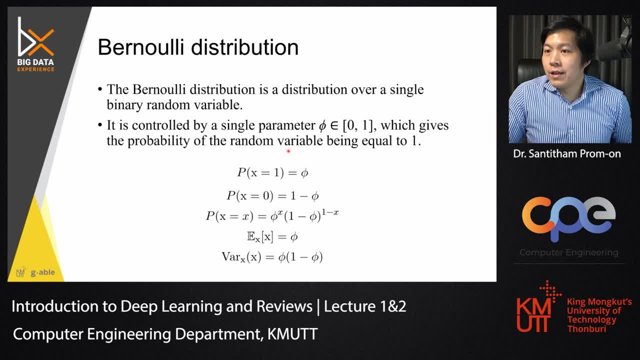 in any case, just take a look if you are interested in that. okay, let's take a look at some distribution that we will find in the deep learning class. the first one, the Bernoulli Bernoulli distribution. in the Bernoulli distribution we have a distribution that can take the value of 0 or 1, and then you have a chance to get. 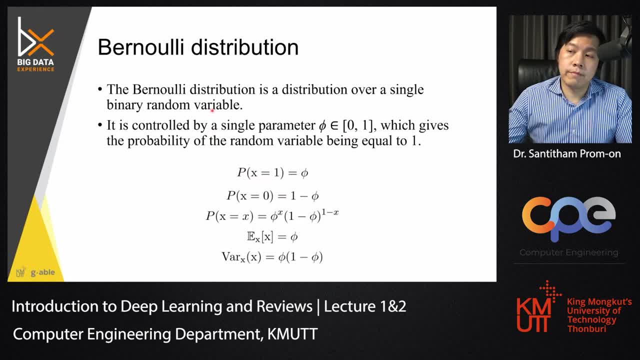 into that value. So px equals 1 would be equal to something. px equals value would be 1 minus that phi equals certain values And in the Bernoulli distribution it can take 0 or 1.. So the chance that you. 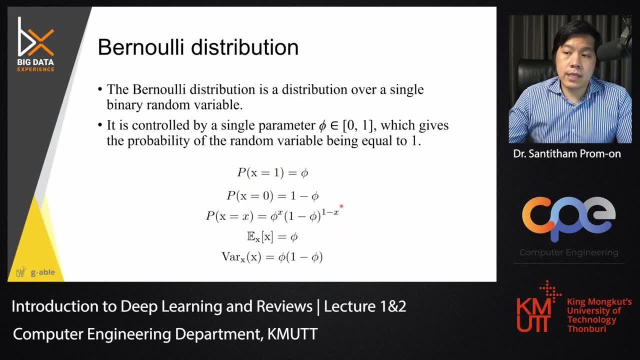 observe this would be x time would be phi of x and 1 minus phi of y minus x, depending on how many times that we are talking about here, And the expected value of x would be phi And the variance is phi and 1 minus phi. 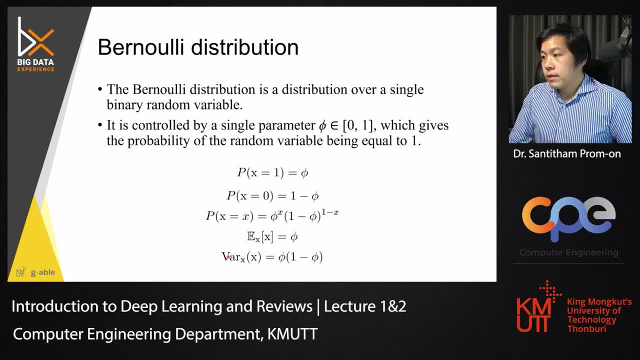 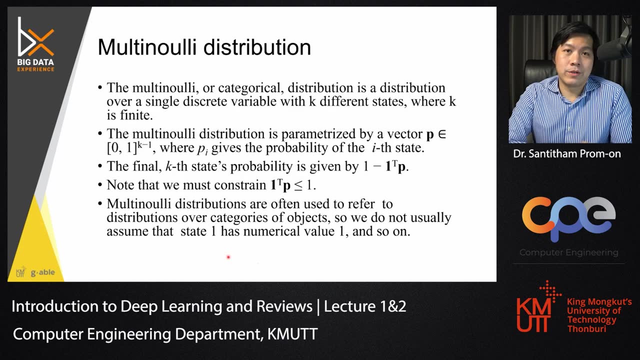 This is like the distribution for 1 and 0. But in deep learning, in machine learning, instead of calling this a Bernoulli distribution, it is called a binomial distribution taking two values, one of the two. So it's the binomial. 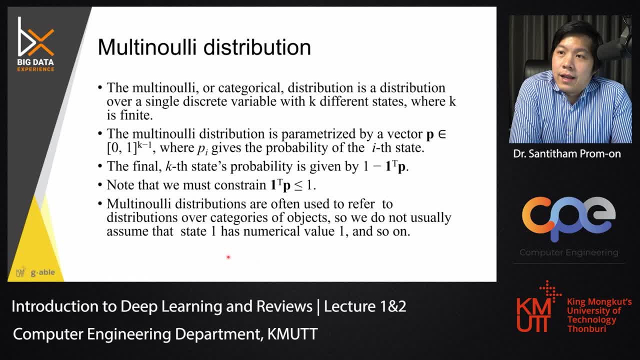 in machine learning. Then we have this, the multi-Nulli distribution or the categorical. You know this as the multi-class classification. The multi-Nulli distribution is a distribution that would take a single discrete value out of k different states. 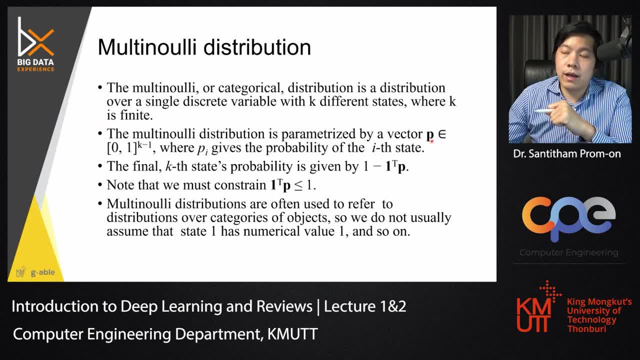 This is called a multi-Nulli, So a multi-Nulli can be parameterized as p. p would be the vector that telling pi would say that the chance that you would belong into that class. So think about this as when we learn this would be the results of the softmax function. 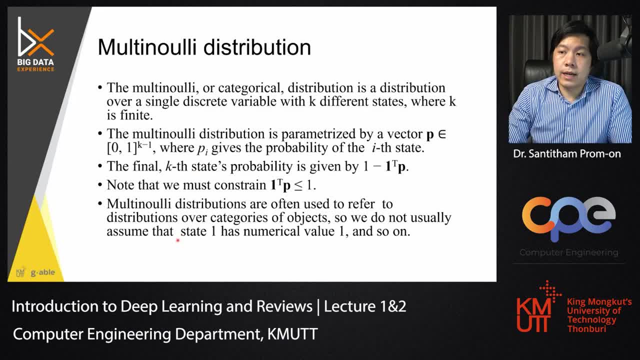 And then you get this multi-Nulli distribution or multi-class distribution And then we can pick like the highest one out. So multi-Nulli is often used in referring to the category of the objects And the highest one refers to as the most likely object that could occur. 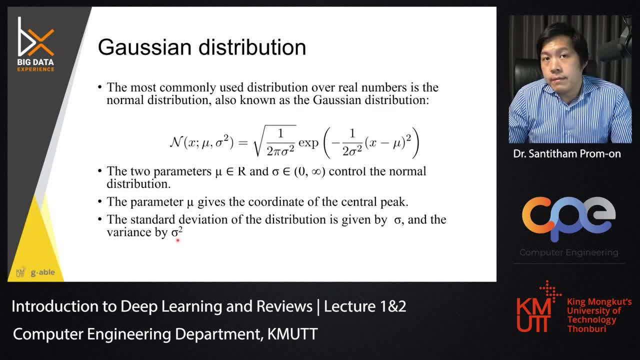 The next distribution is the distribution that has often encountered in statistics: The Gaussian distribution or the normal distribution. Gaussian distribution or normal distribution consists of this exponential representation of a non-particular structure: exponential function. Think about this: Exponential function has the highest value and the value equals. 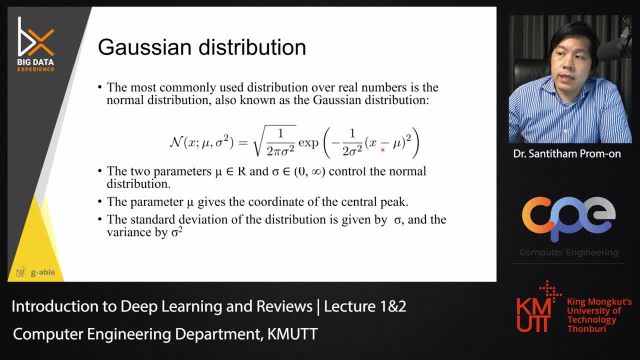 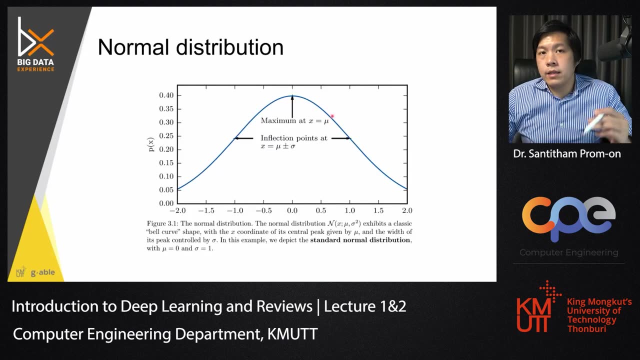 zero, That means this one will be highest. if x equals mu, right, Because x equals mu, it will be zero. If x is not equal mu, then it will take some value. Once it has some value with the negative sign, this would reduce the values of exponential quite a lot. That's why we have this. 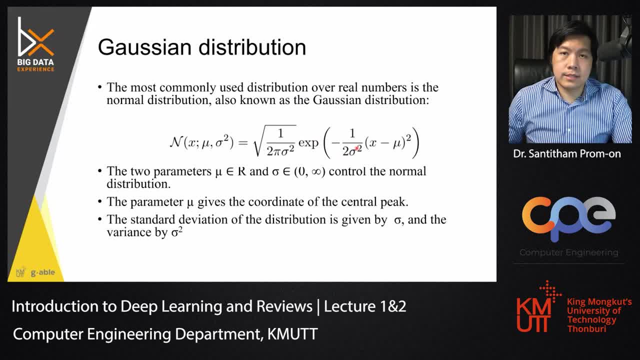 reduction here, inflection like this from these exponential values. Sigma controls the shape of the distributions. It scales the value, in this sense the value itself, and it also scales the expansion of the exponent here. So mu, then, would be the center of the peak. 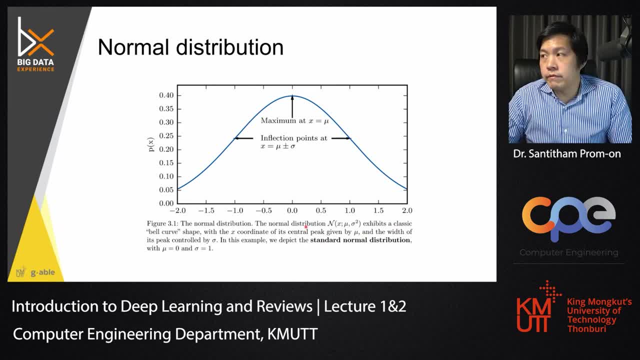 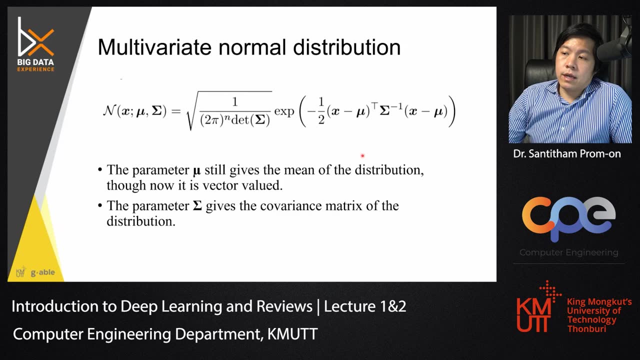 while the sigma would control The spread of the mountain. This is the normal distribution. This is a particular case called standard normal because mean equals zero and the standard deviation equals one. Normal distribution when you have multiple variables or, let's put it this way, when you 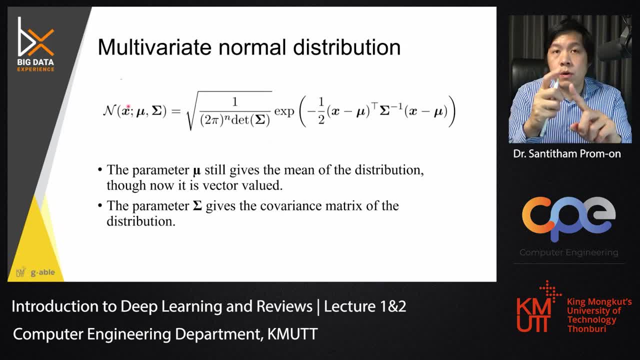 have a vector. When you have a vector, not just one value, And when we talk about distribution of the vector, it's not just one value anymore. So the distribution of the vector in the normal sense would be a mixture of, not a mixture. 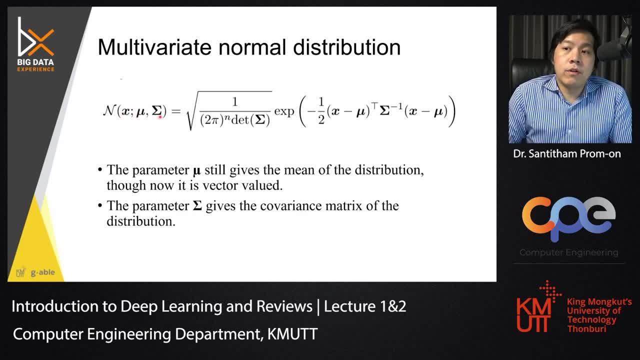 I would say multiple distribution, multiple normal distribution, And that multiple normal distribution would have multiple mean vector of mu and has certain dependency, certain covariance between them. This is called the multivariate normal distribution or the distribution of multiple variables. So the difference would be that instead of having just sigma, you have this determinant. 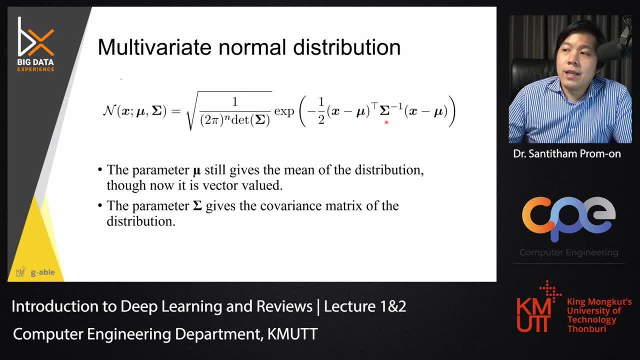 of sigma to determine the size of transformation. And here this is still X minus mu, but instead of having the 1 over sigma, you have sigma inverse. And the reason that you have this X minus mu again and X minus mu transpose this is: 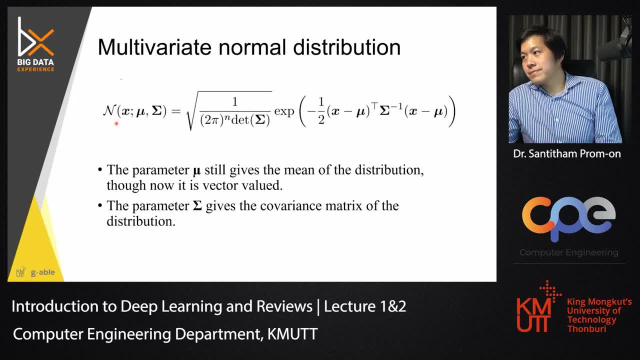 to denote the square. okay, So this is the multivariate normal distribution. This multivariate normal distribution can express dependency between the distribution by having the covariance having the value not in the diagonal line. If it has certain dependency between them, the covariance would have certain value and 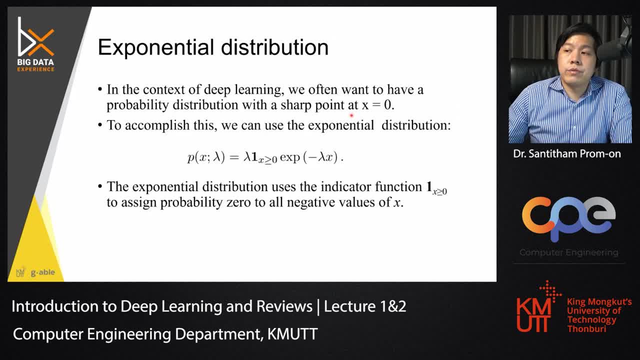 when you multiply it it's going to be 0. But if you multiply it in this sense it will contribute to the distribution. One distribution will contribute to another distribution. This is for the normal distribution, For the exponential distribution. exponential distribution refers to a distribution that 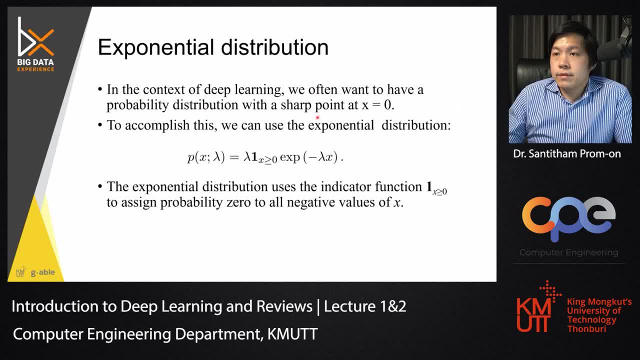 is using exponential In deep learning. Sometimes we want to have probability, have a sharp point at zero and then reduce at higher values. We can use exponent function in that case. This is exponent function. So when X increase, when X increase, lambda would. when X increase, the value would decrease. 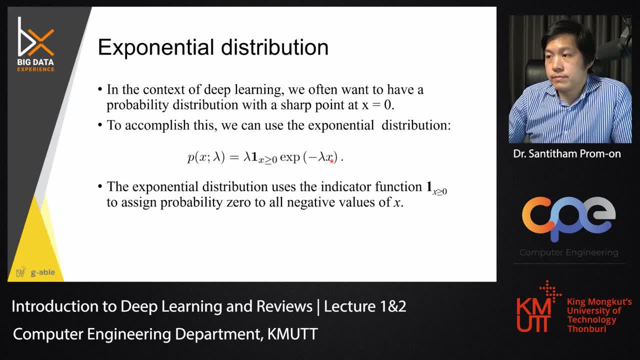 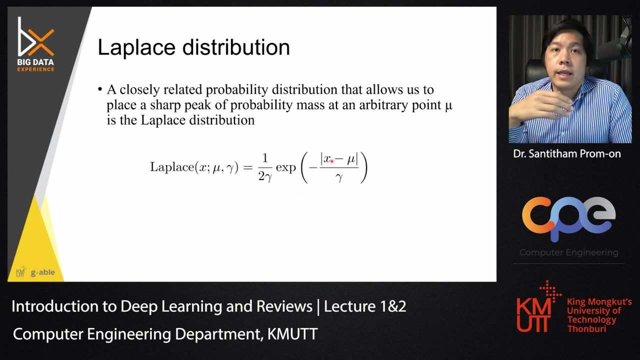 Lambda would control the rate that it would decrease. Okay, This is called exponential distribution. When to use this? sometimes we use it for, for example, for controlling the learning rate, so that you have large learning rate at the beginning, smaller at the end. Yeah, So this is for the exponential function, The 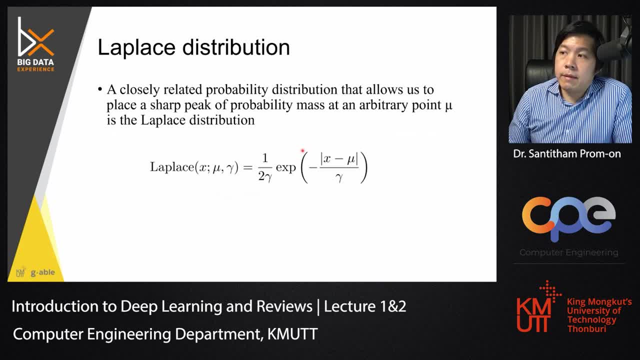 next one is a Laplace distribution. Laplace distribution has has this formula. Actually, it's quite similar to normal distribution. If you look at this case. the difference is that this is absolute instead of 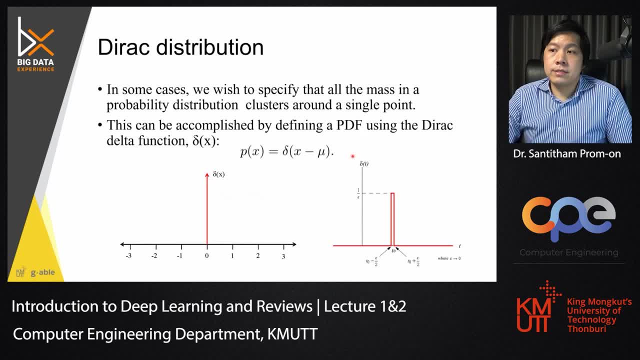 square. So when, when it's like that, Laplace distribution would be sharper than normal distribution. I think this is the last one. The last one is the Dirac distribution, also known as impulse. Dirac distribution has a special property, that is, it is the 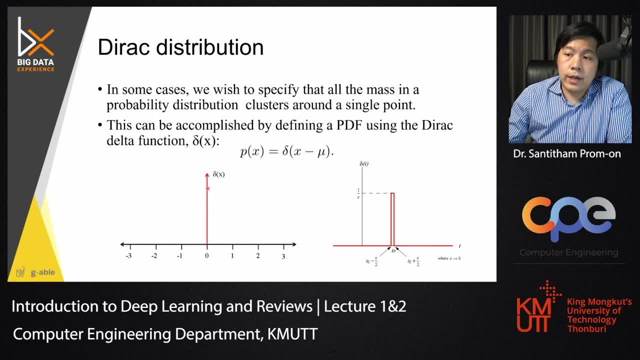 distribution that has only value in the value that is located. Sometimes this is denoted as an impulse. It means that it happens at this time, not any other time, Right? The Dirac delta has certain property: when you integrate it, It has the value of 1, and at this point it has the peak of infinity. 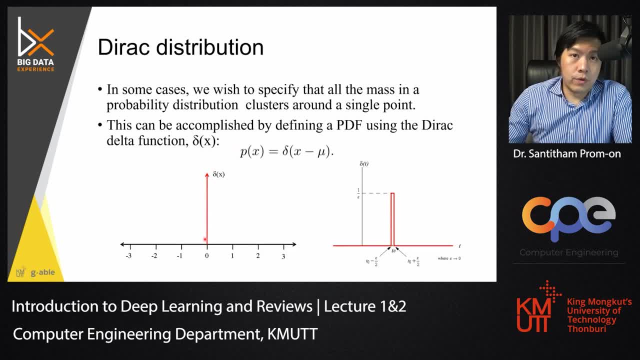 but the width of 0, approaching 0. This is usually used to denote when you take the value out of the continuous distribution, or, well, when you use something like convolution and you know it as the discrete level distribution, That's right. So there, in this case, the 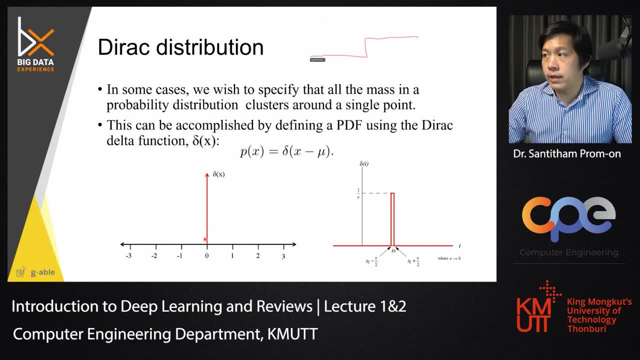 average is 0.. So you can see what this is. So this is a little bit of a delineation in the level we their Delta would come out in that way. or when you take derivative of a sharp, if you take derivative of a U function, if you D by DT of this, 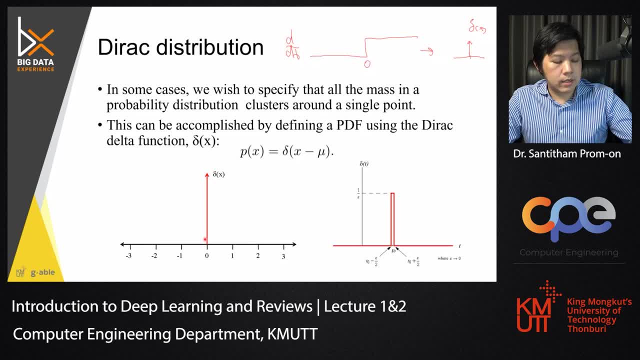 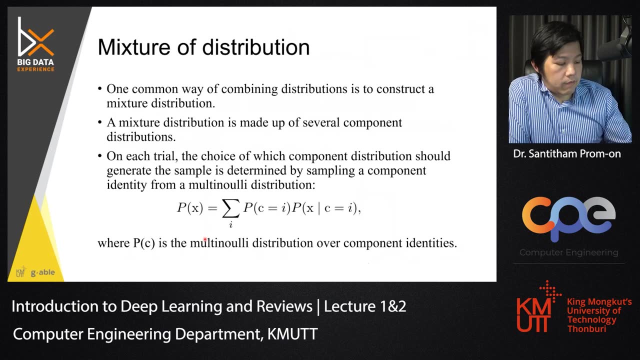 function. it gives you the Delta of X. this is at zero. yeah, so this is the relationship which which is important in, in, in the latter mathematical foundation of of the model. okay, these distribution can be combined. it, yeah, it can be combined by just add them up, right? this is look, although it looks. 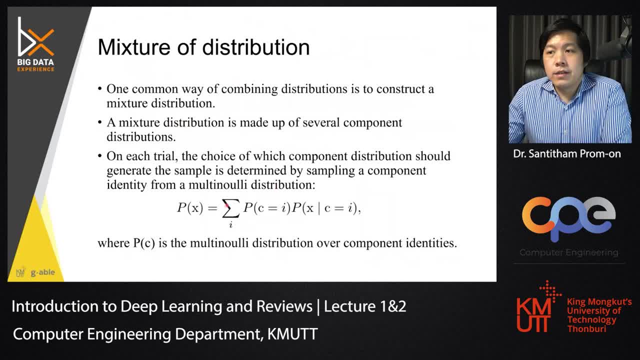 like: oh, what is the mixture of distribution? like the name suggested, mixture mean combined. when you combine distribution you need to have certain probability, so certain, certain value. so the mixture of distribution is the combination of distribution with certain weight. okay, for example, you can have like this multi newly distribution to be denoted as the combination of the Bernoulli. 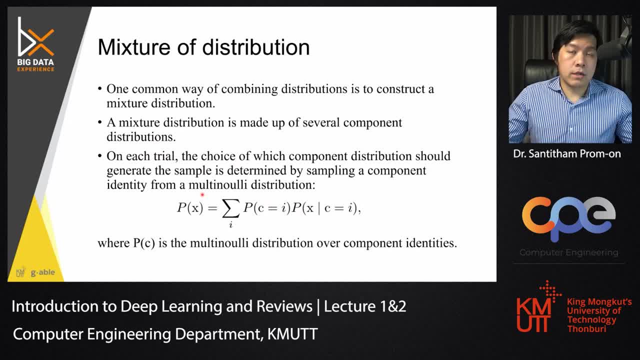 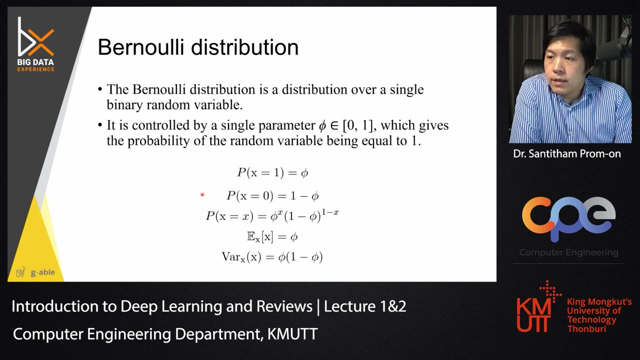 distribution. you have a multiple Bernoulli distribution. combined it with certain weight, then you get the multi newly distribution. so these example of distributions that that might arise in in deep learning, in in representing the data, we will at least take into account Gjeong we used. 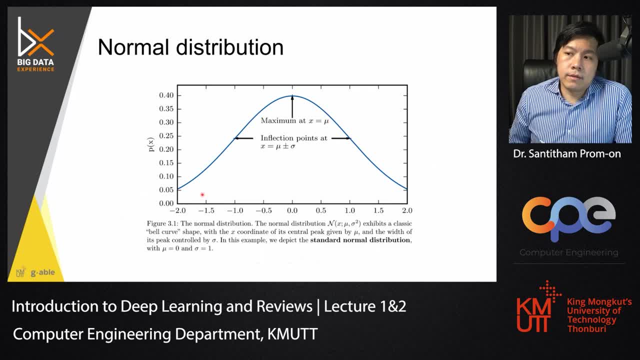 conduit machine and and and we discussed in attribution and Dale- dai vision in a graduation. are we patient off the top? this may another question you want to answer. and yeah, we can end. and the better distribution, interdimensional個ורand also at least take in the rail fija of evaluation, of evaluation of the Ledger allocation, and narelle is involved in the realm of all the innovations, which is to couch. 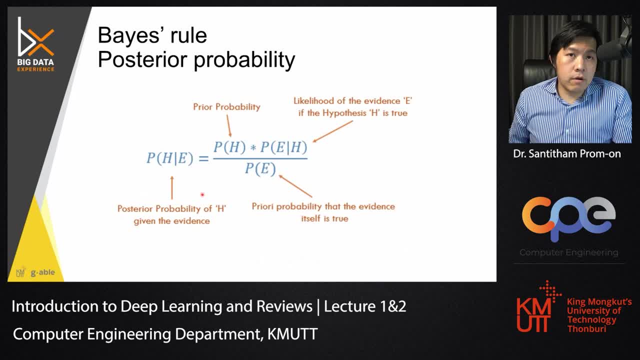 evaluation of the of the model, of the regression model using deep learning and classification model using deep learning. okay, um, now almost, i think, almost the end, right, uh, so when we work with machine learning, we are not actually just fitting data with the model and just that we are actually relying on. 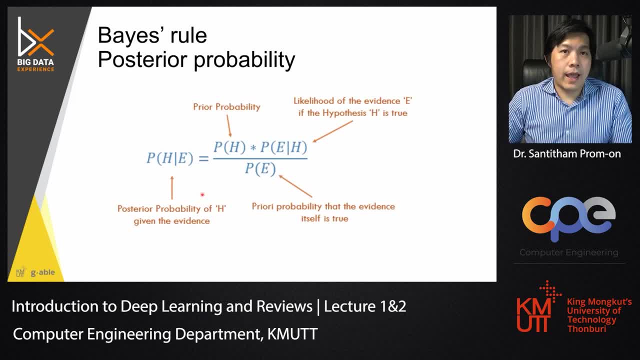 certain probability theory and that theory is called the base theorem or the base rules. in the base rules, usually when you you have a chance to observe even- and we call that the prior probability- for example, in population, there might be a chance of one in a million that you get covered. right, but the posterior probability, right. so so if you see some person, 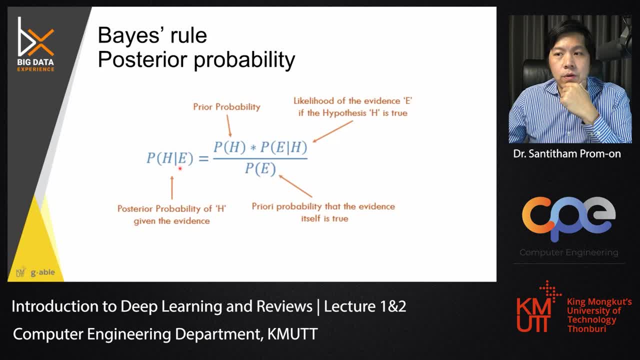 pass by. no, there's one in a million that that person get covered. but suppose that you see that person. e is an e, it an evidence you see that person not wearing mask, then the ph given e might increase to one in a thousand right. one in a thousand that that person might get caught right. and and this is 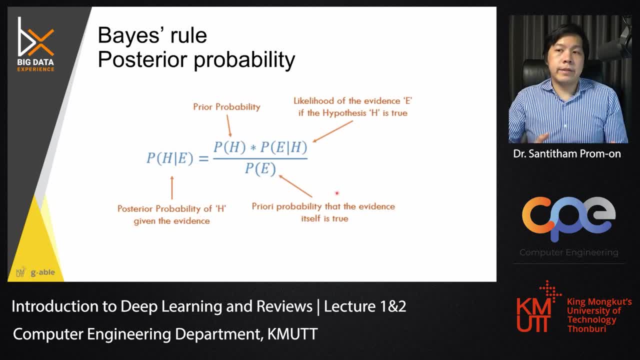 called the posterior probability. posterior probability is the property of the event after you observing the evidence and this comes from the it's come from the conditional probability equation. this is prior pop and this is the likelihood that you observe e given h, like e is like not wearing a mask and then get covered. this is the call, the evidence. 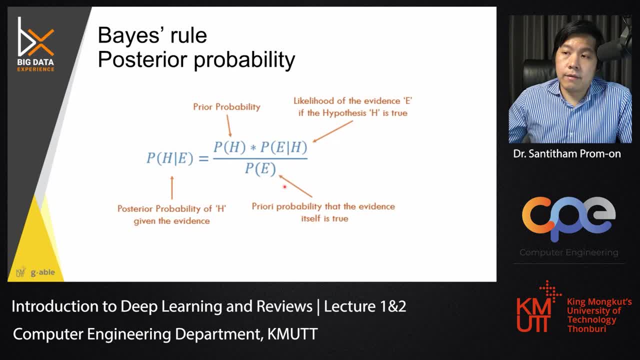 sometimes you get this from the model. this is the uh priority pop that come from the evidence, then chance of wearing mass. sometimes this is ignore, so base rule. it comes from this because we know that p of a given b equal p of a intersect b divided by pb and p of 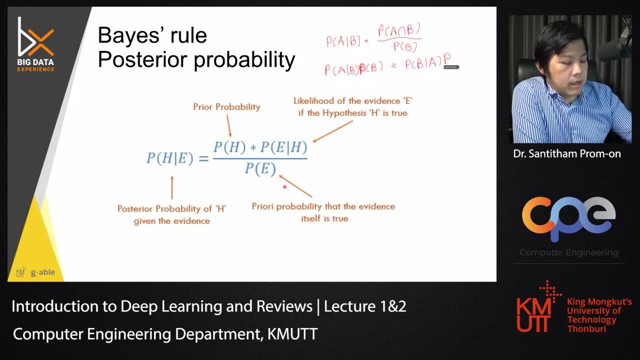 that mean p of a given b time pb. time pb would equal p of b given a time pa equal p of a insect b. so that means if i were to move this p of a given b and then p of a of b given a divided by pb, i would have this base rule derived from conditional probability. okay. 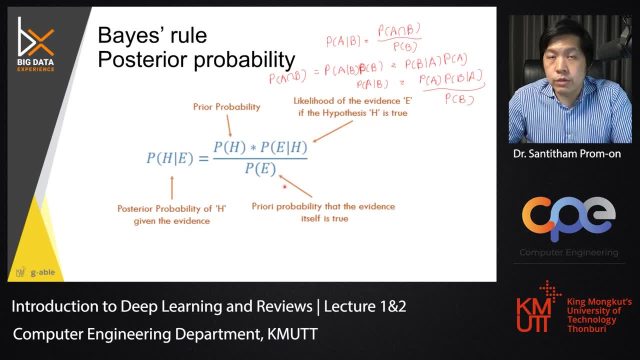 so this bear rules play important role, a crucial role in machine learning, because machine learning is this equation. yeah, you will see that in the machine learning lecture, that the machine learning that we know is actually this equation. and when you train the model sequentially, when you train the model that is balanced. 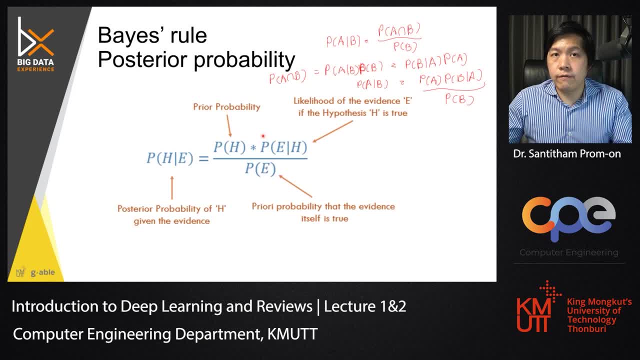 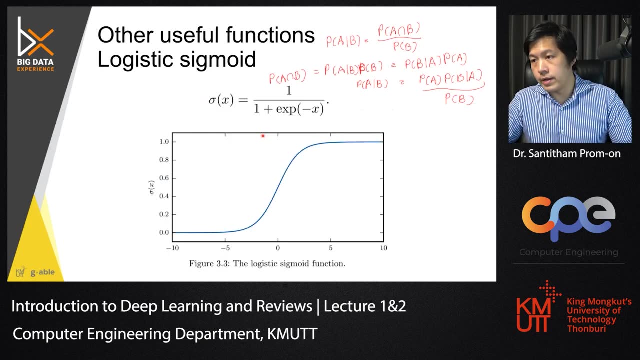 you need to multiply them with prior pop, otherwise you would have unbi, you would have the bias model. okay, so this is the base rule. we will use it later on anyway to associating posterior pop with the, the model that is, it is stranded, and also to derive the lost function in in. 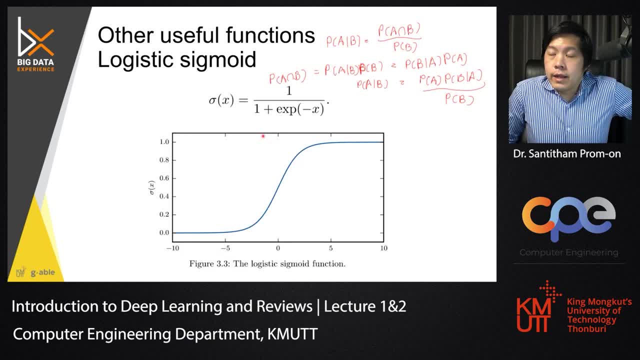 training, the model right uh, let's take and also, i think, just a few more slides. we will take a look at some important uh functions. first is sigmoid function: logistic function. sigmoid function has a smooth transition and it has a very nice property which we will talk about next time. 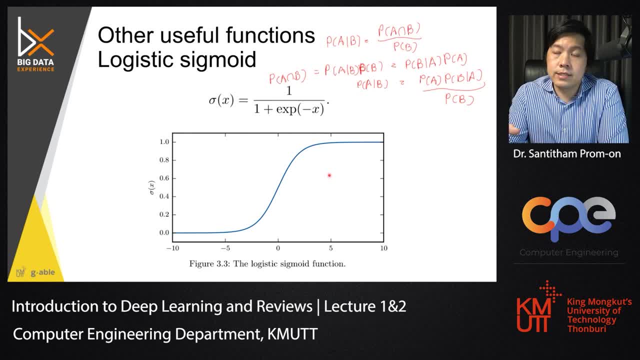 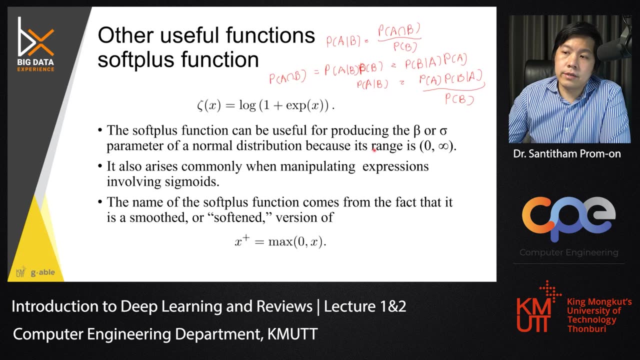 that allow us to calculate gradient and optimize the, the deep learning model, the perceptron, with the with, by using mathematics in combination with coding. this is the logistic function or the sigmoid function. as x increase, the value transit from 0 to 1.. another, another function, that is: 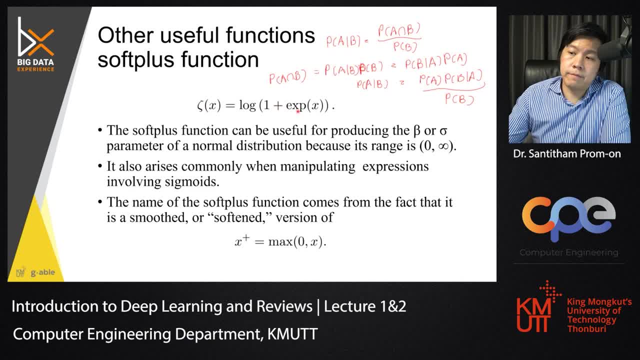 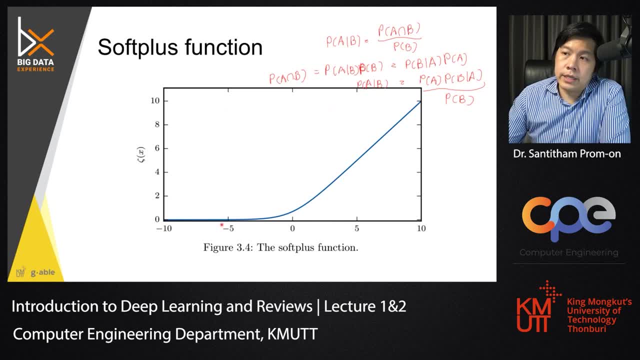 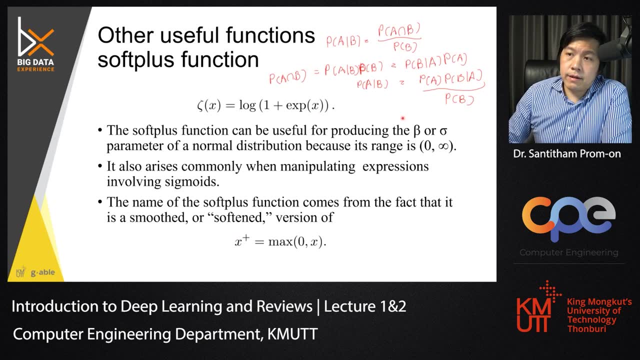 quite important is the soft plus function. the soft plus function. here the zeta of x is log of 1 plus exp of x. this is a soft plus function. so plus have the value of 0 and then increase and become linear after it passed 0. this is soft plus function. the top plus can be used to. can be used. 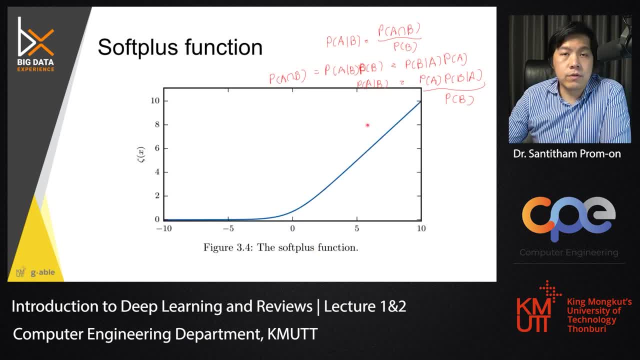 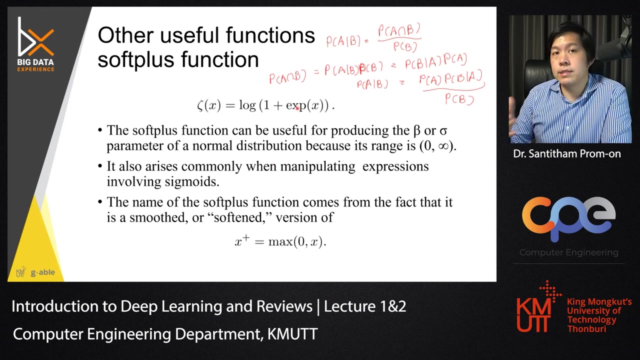 to represent the like, the value that has that is like 0, or has the value of x when it's more than 0, and this can be well in in deep learning. there is a technique called the, the activation function, called the raylu rectify linear. it can soft plus can replace that, because this is differentiable. 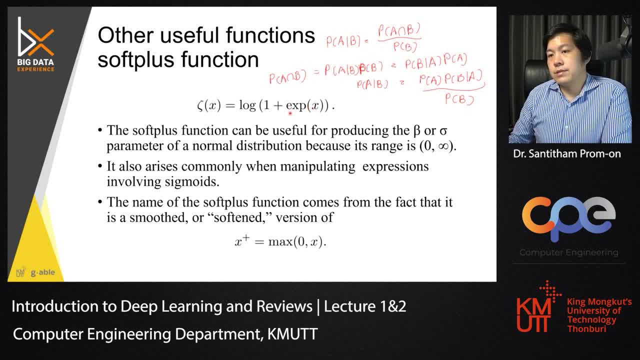 lay lou- is not differentiable, right. so, and this might arise later on, the soft plus. this is log of 1 plus exponential of x, um, log of exponential, it's just that value. okay, that's the soft plus function. that means when the value closer to 1, it will behave like log when the value is a lot more than. 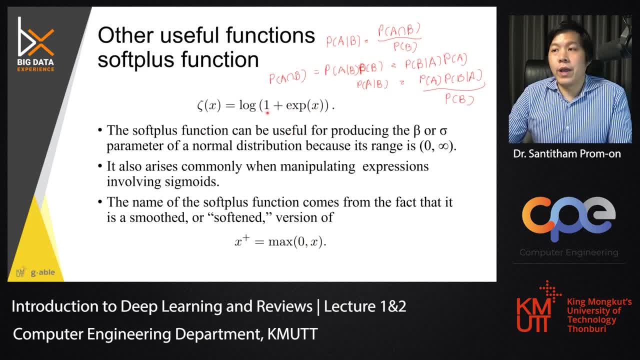 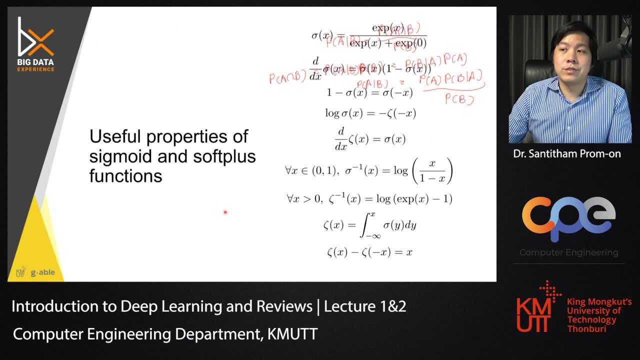 1, it will. it will behave like that value. when x is less than 0, then it has to be a value of 0. so that will be log 1, which is 0. okay, so sigmoid soft plus has certain relationship, that is. this is the. 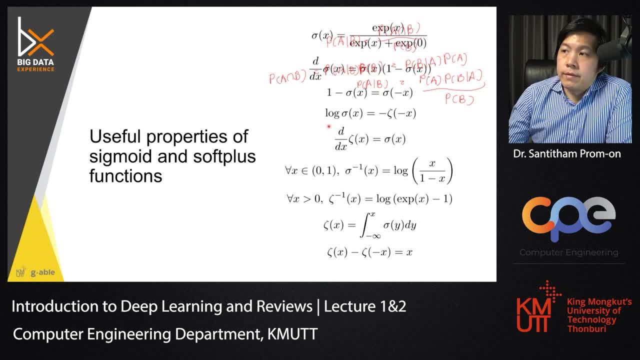 sigmoid function. um, if, uh, we dip the sigmoid, we get sigmoid and one minus sigmoid, and we will talk about this later on- and uh, we take the, uh we, if we dip the, the soft plus, we get the sigmoid. this is like the: the function is convertible from one to another. 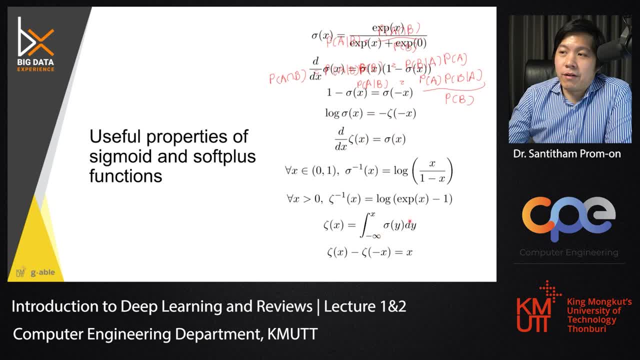 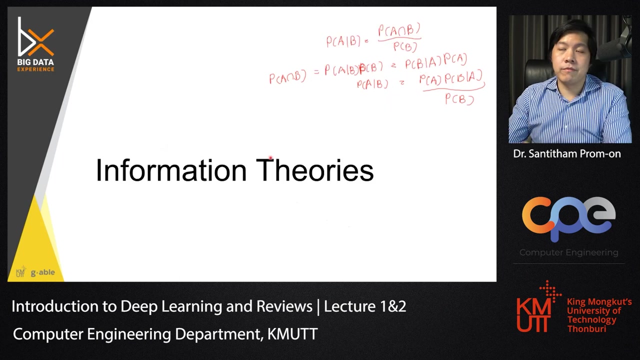 um, and and what else. take log of sigmoid and you get the soft soft plus on the flip side and if you integrate the, the sigmoid to a certain value, you get soft plus and the soft plus, minus, minus, surplus, reflecting out to get value of x. so this is quite a useful formula. it is useful properties, although we will not use all of them. we. 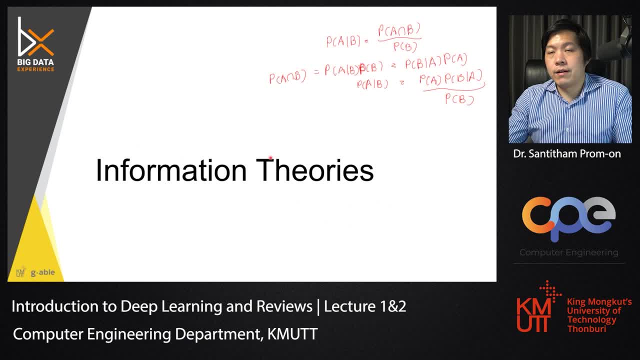 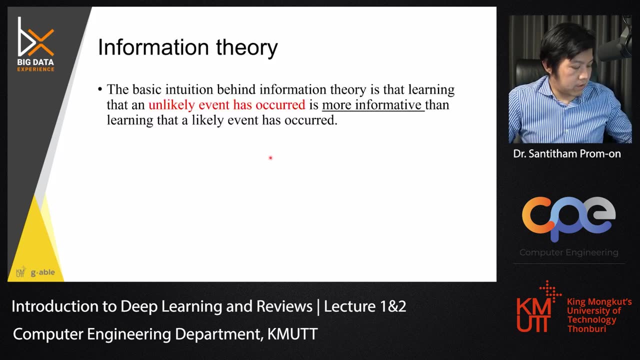 will at least use the sigmoid and then see later on how it works in gradient derivation. okay, this was about without". now this is a very complex theme. i hope you don't think this is too much, right, as am waiting for my comments in this webinar. tips over in this class, moving on to the next topic. today. in this video, i will tell you what is 모양èmeagrammetim ini. it's called Hohenschopp's theorem. i will see you donate eternity to the hobbrell, as said in this class, Temporarily. now it comes to the last topics that we will cover tonight. is wishes info- i forgot to remove this out- which is information theory. um, information theory refers to, uh, the learning that how even occur and when even occurred. that should be certain information that can be toilet, that can be learned, that should be certain variables, and i will explain, would mean certain statements.